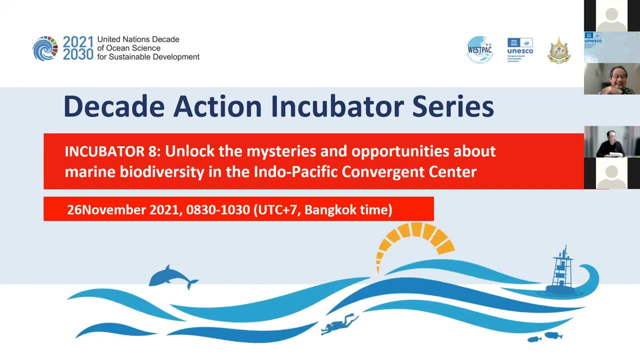 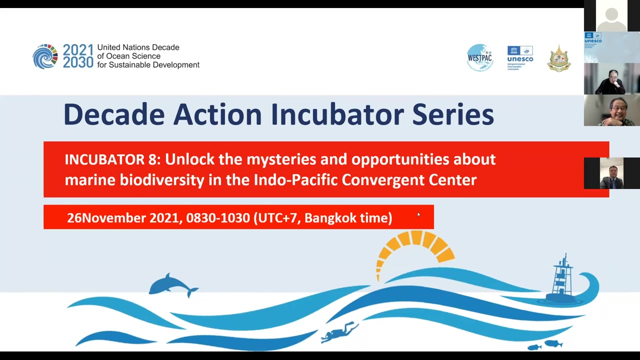 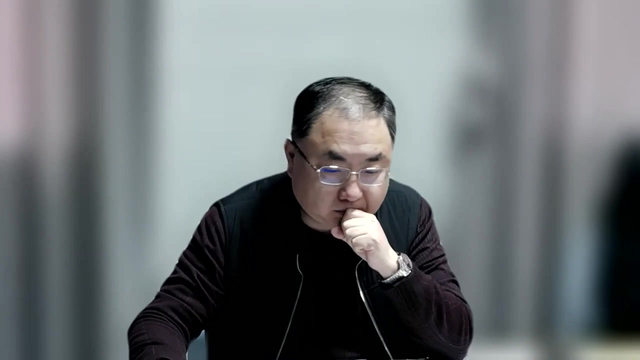 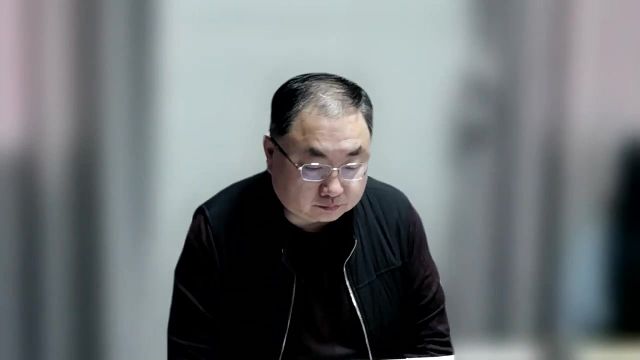 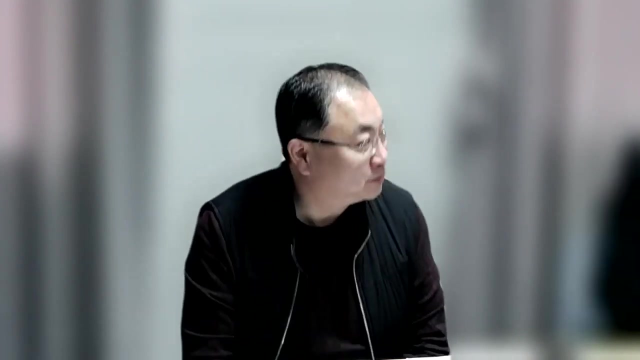 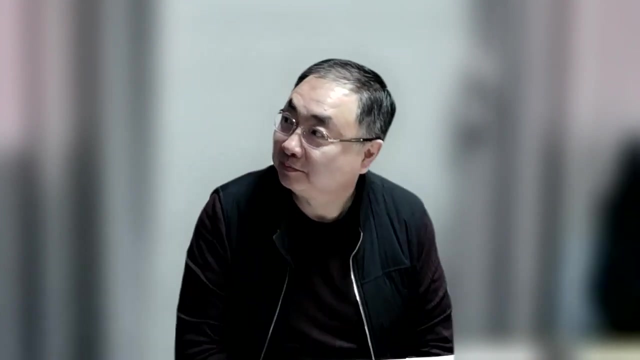 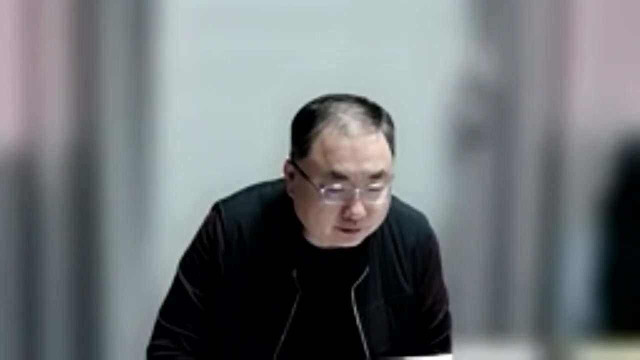 Thank you, Thank you. Thank you very much, Hi Ellen. Could you hear me? Yes, yes, Morning, morning, Hi, I can hear you. Meet you again. Yeah, yeah, I can hear you clearly Good. 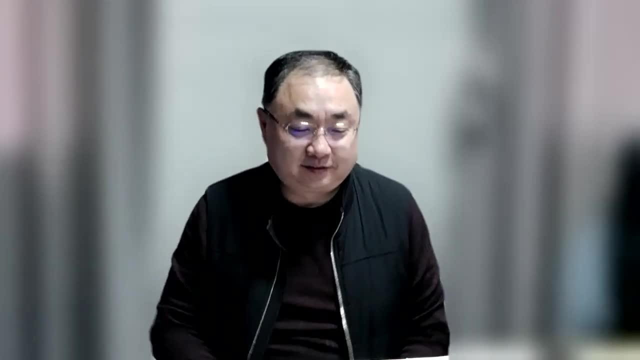 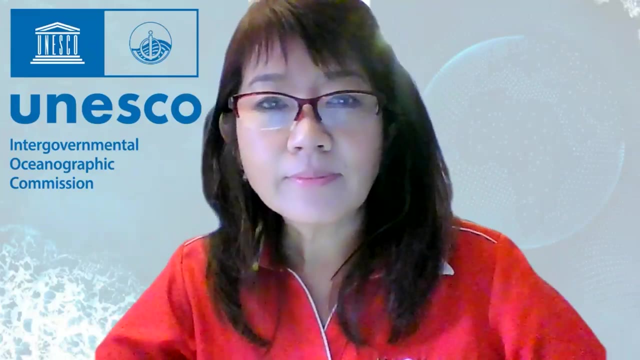 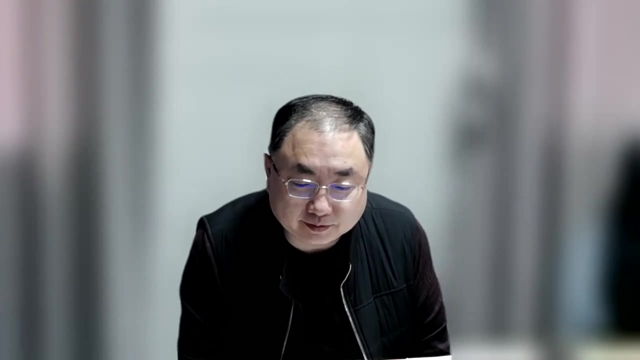 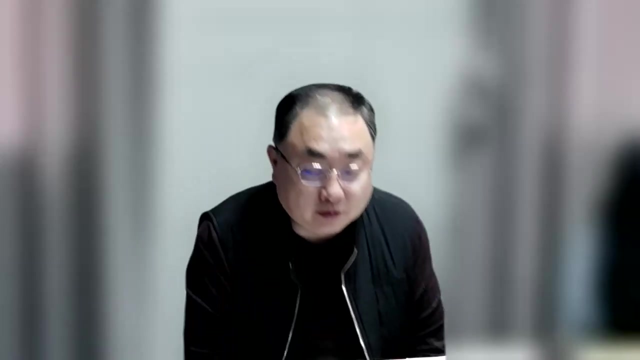 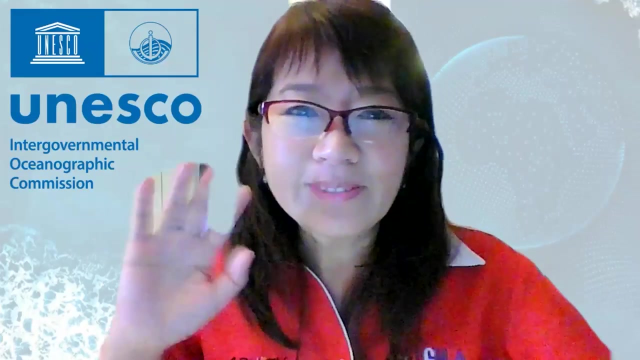 Good, good, Hi, I can hear you clearly. Hi, how are you doing, Prof. Hi, how are you doing? Zainal Nice, to meet you? Morning, Pak, Zainal Morning, Prof. Aileen. How are you? 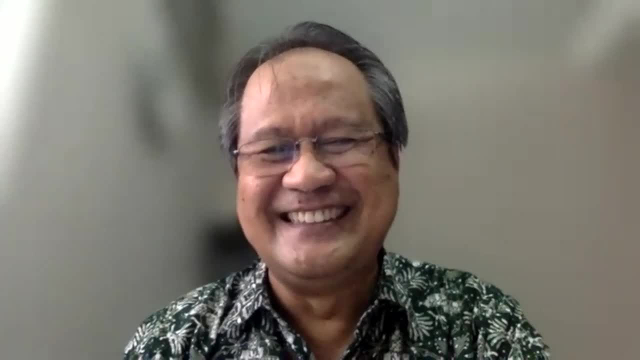 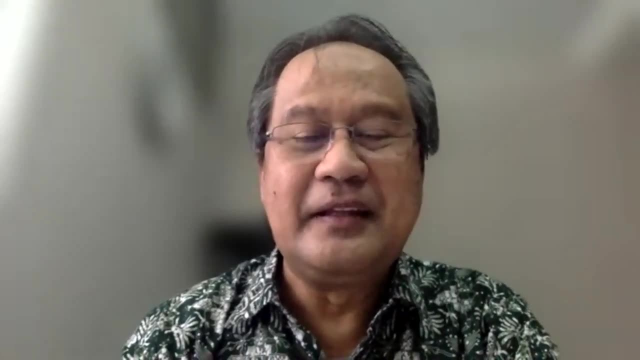 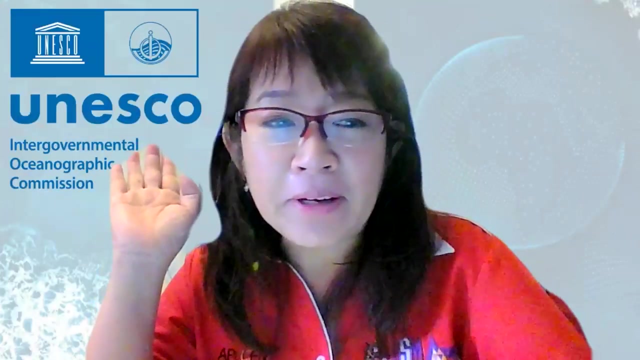 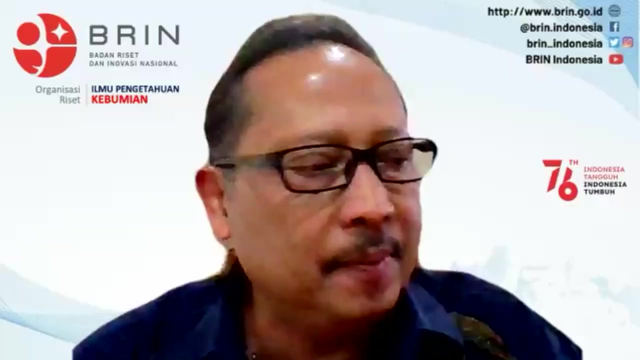 How are you? Good good, Very good, Good good. I tried to find a background. I couldn't find it. In this background, I asked for Menzi. Hey everybody, Hey, good morning, Prof Oki. 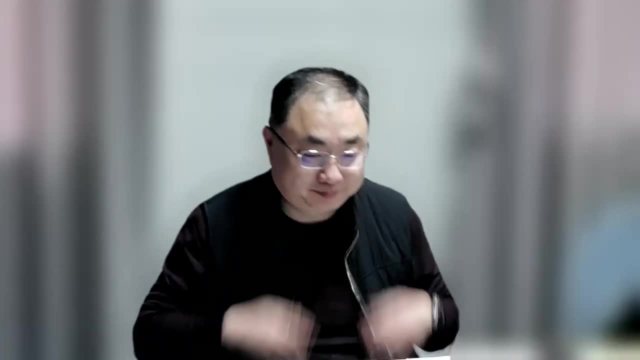 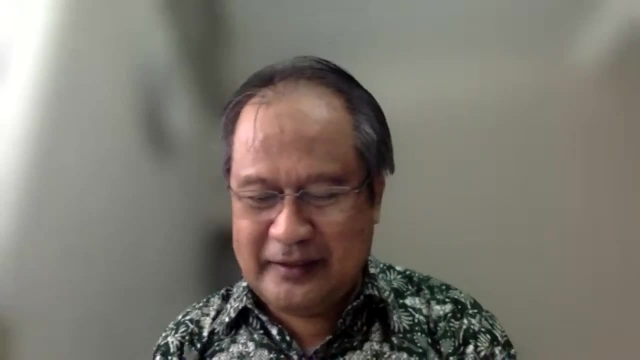 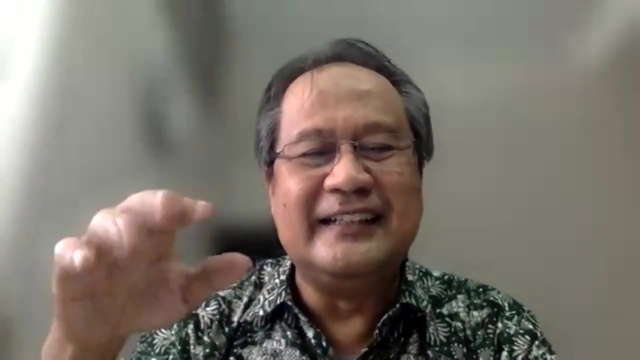 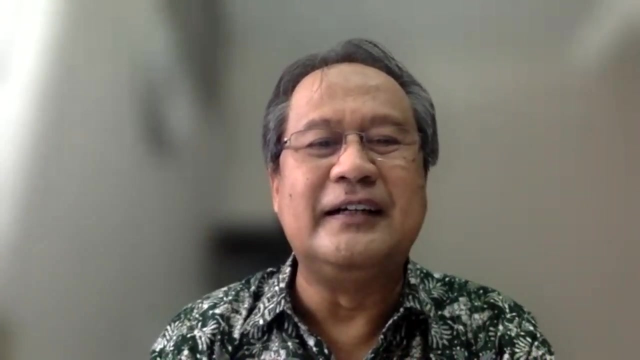 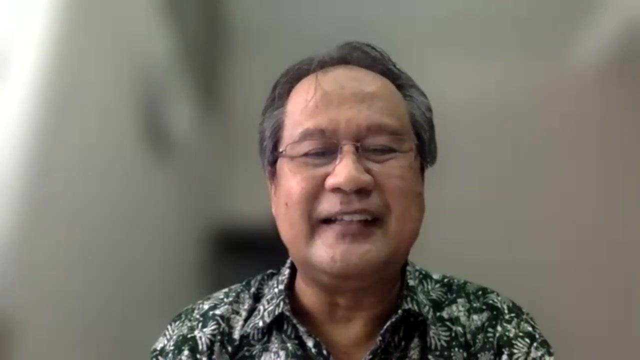 Hi, Prof Oki. Nice to meet you, Nice to meet you too. So how is the? what do you call the list of the speakers? right, So we start from you, and then Prof Oki, and then Dr Krishnan. 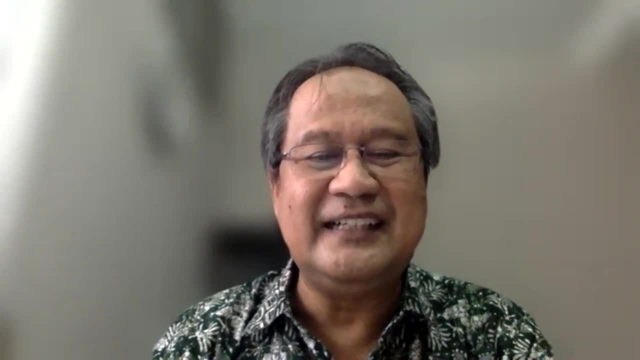 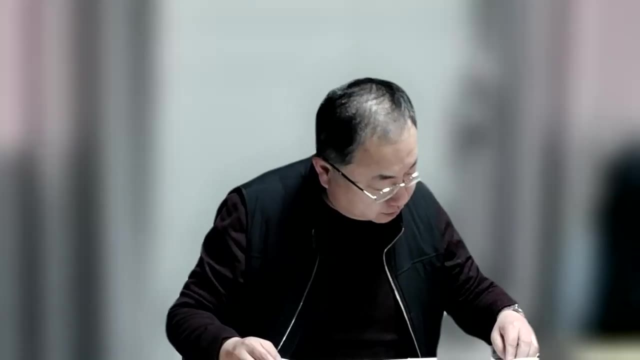 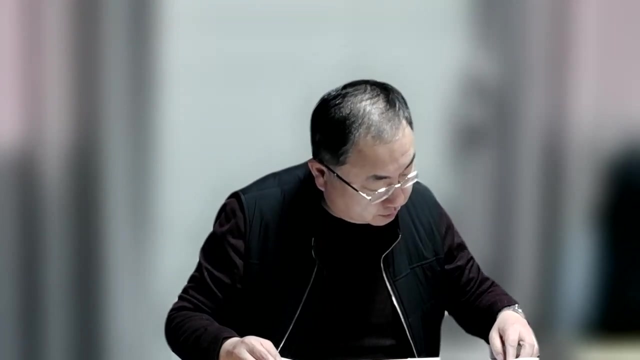 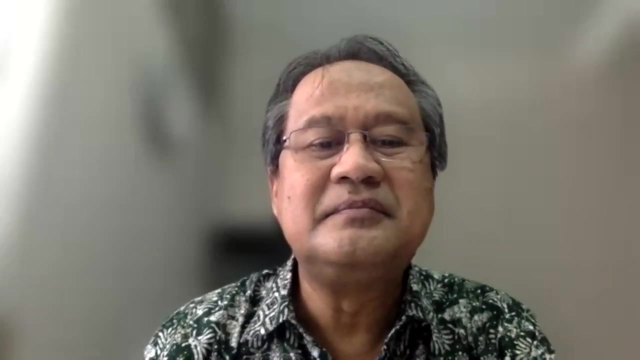 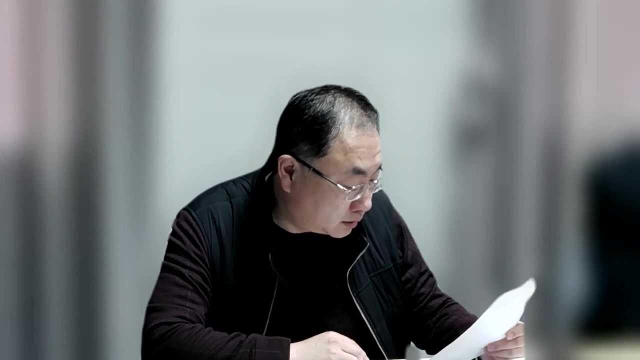 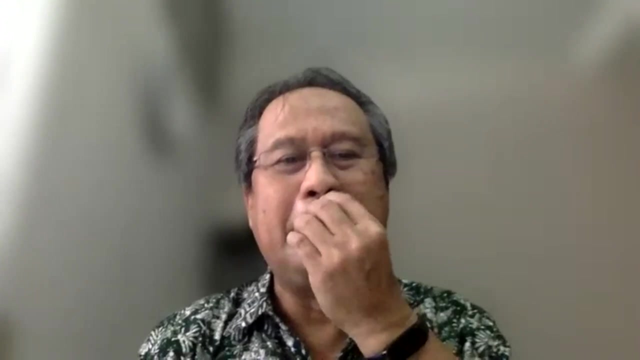 and Dr Zainal Jichang and Prof Yuandia. five speakers right, Five. See, according to the agenda, we have four invited folks. Yes, there are Oki Paoki and Andy and the ranger and myself. right, all three of you. yeah, yeah, and, and, and there are other. 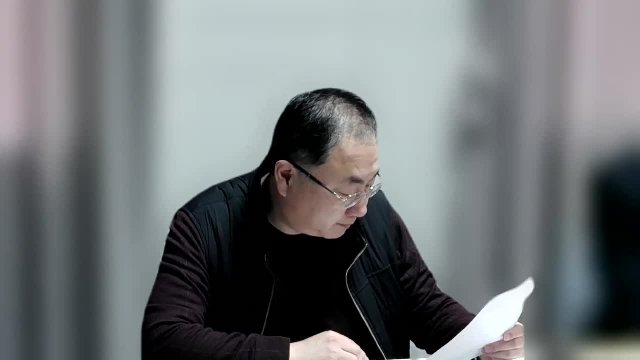 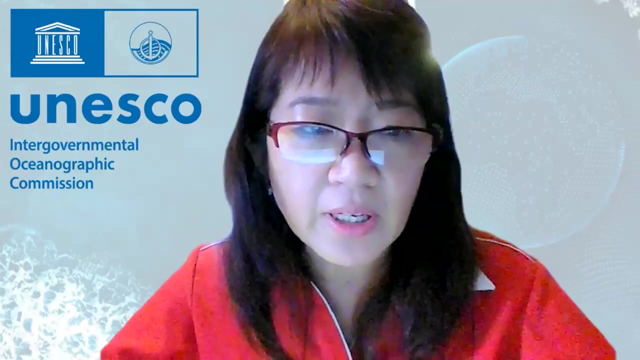 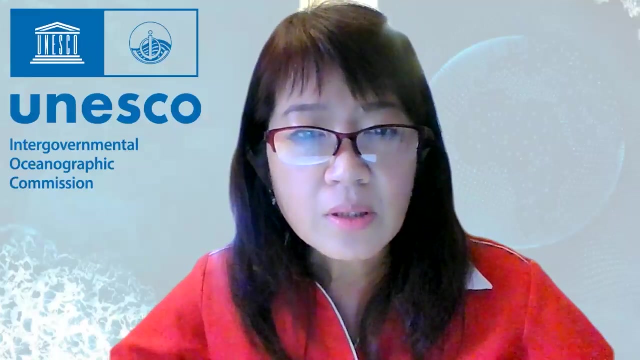 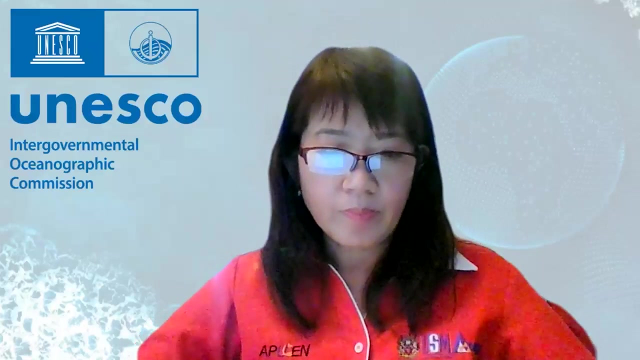 three mini talks. um, from mr uh christian, yeah, and uh, and the young chan yang, which is a mini box, yeah. um, uh, professor, uh, just to confirm the mini talk. we have two speakers or three speakers. three, three speakers for the mini talk. yeah, yeah, okay. so from uh fangwang, can you repeat it again? the speaker. 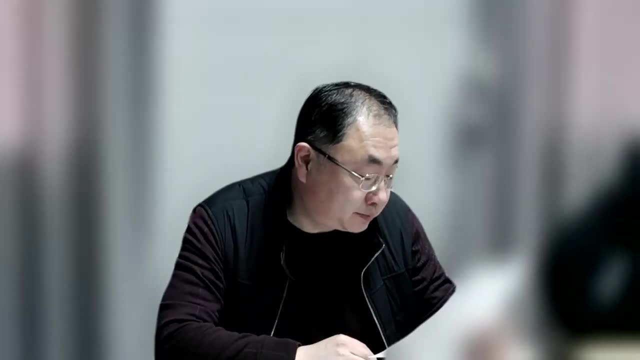 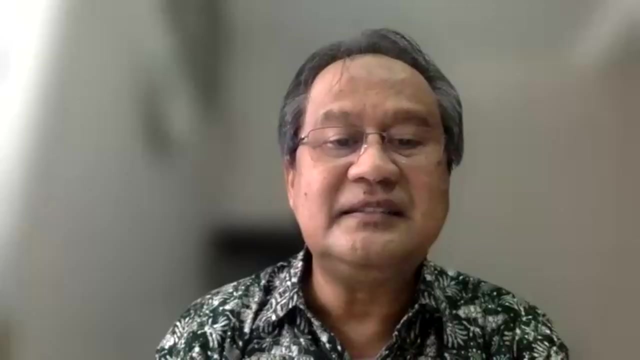 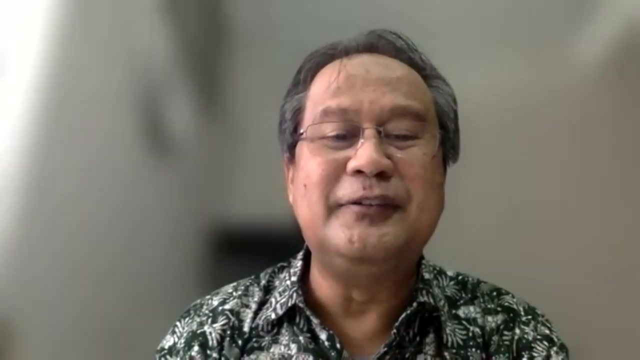 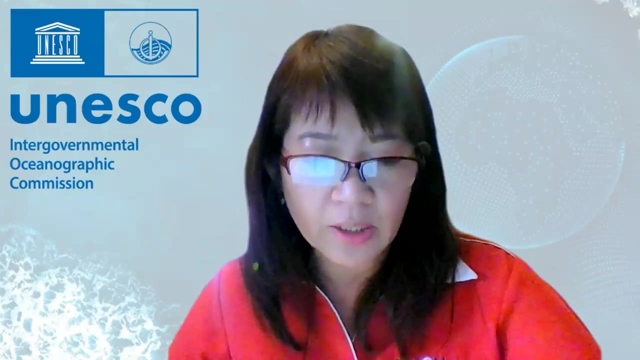 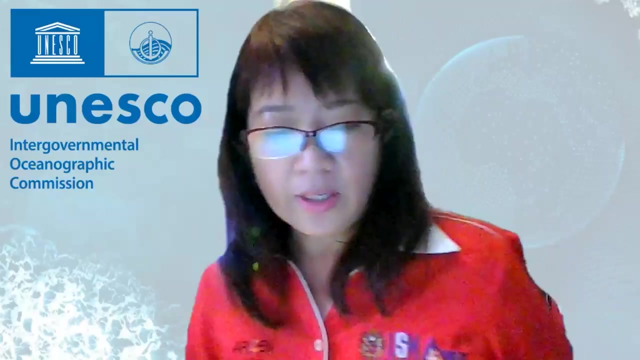 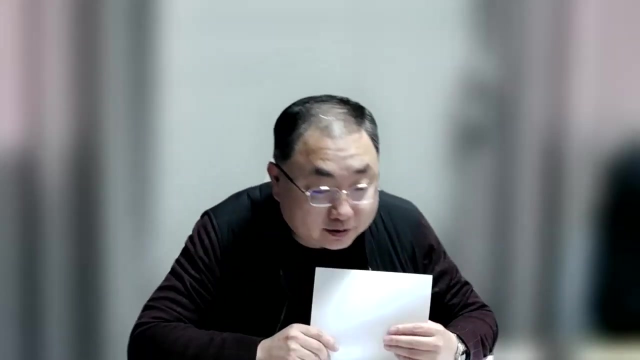 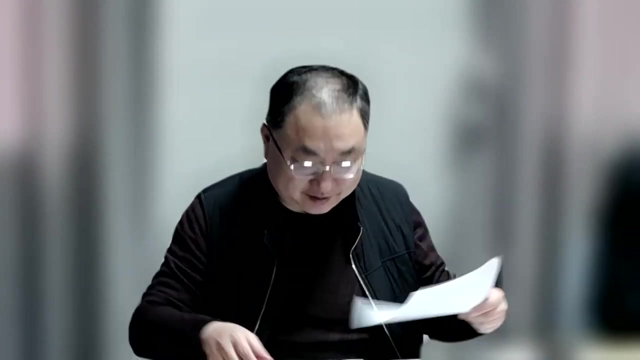 uh, yeah, the uh. invited speaker is uh, uh, the uh. the first is uh is me and the second is uh. okay, yes, the young one uh for the mini talk, right, yeah, yeah, yes, okay, okay, yeah, okay, um, okay, shall we start uh? hold on a minute, okay. 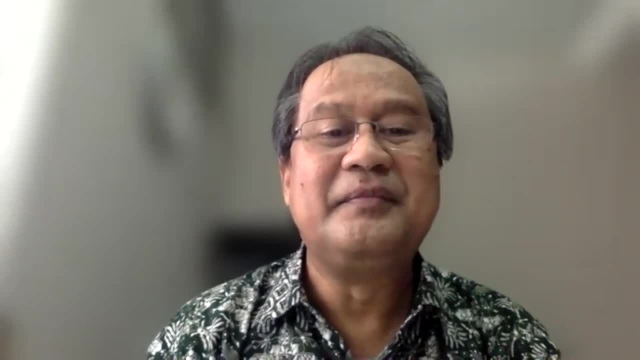 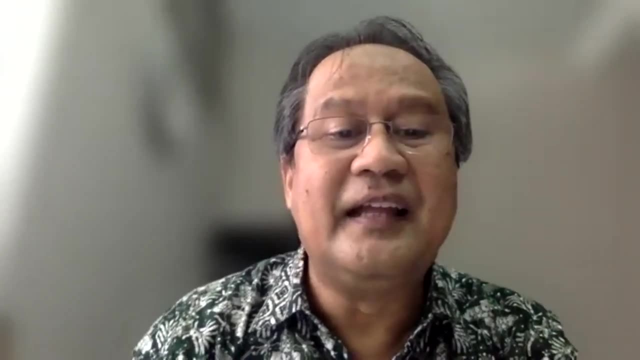 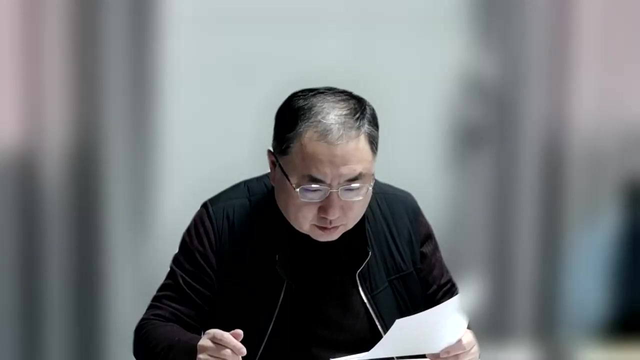 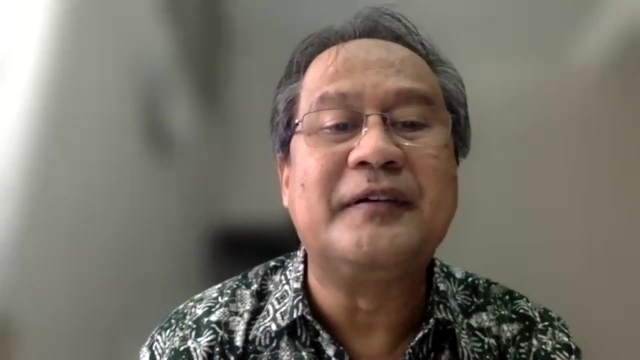 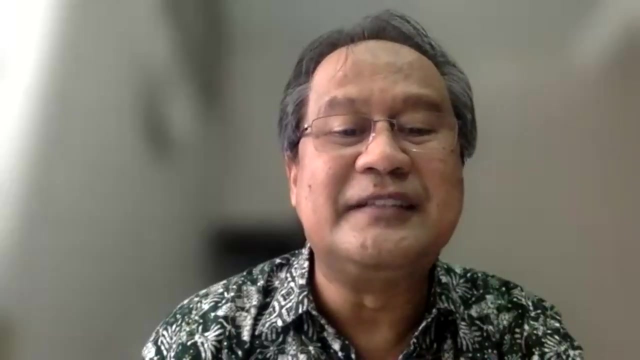 professor, you, yeah, okay, speaker, i can i repeat again? first uh from fangwang, and then uh from okay, yeah. and then uh, prof. eileen, yes, yes. and then number four: uh from uh, you, yes, yeah, yes, yeah. one, two, three, four and then the three minutes. 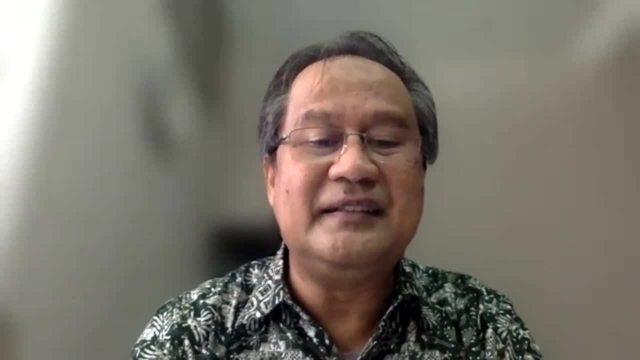 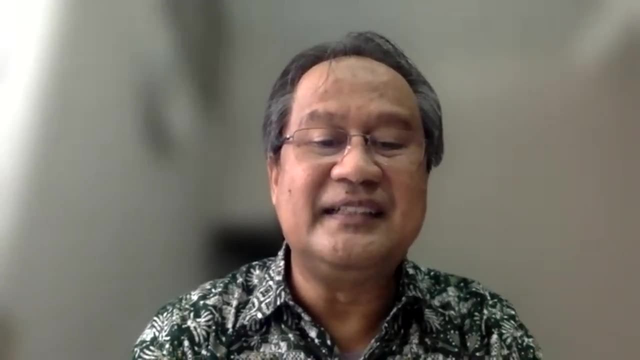 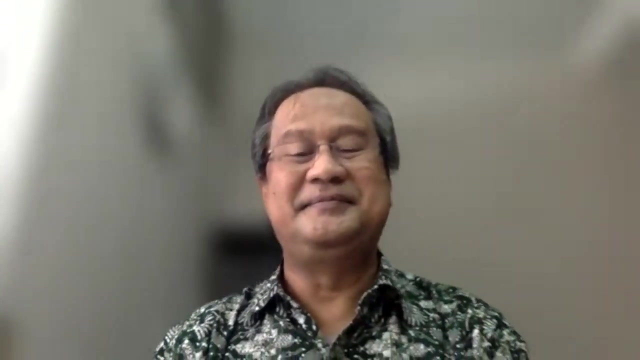 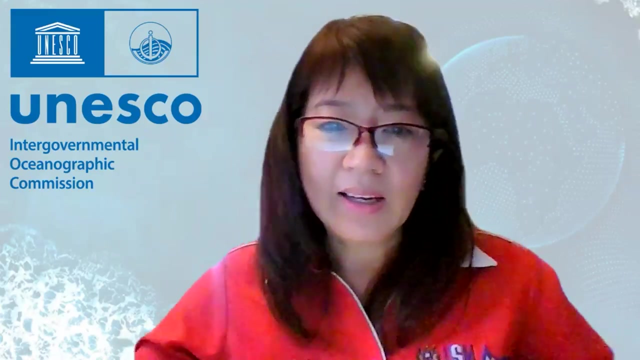 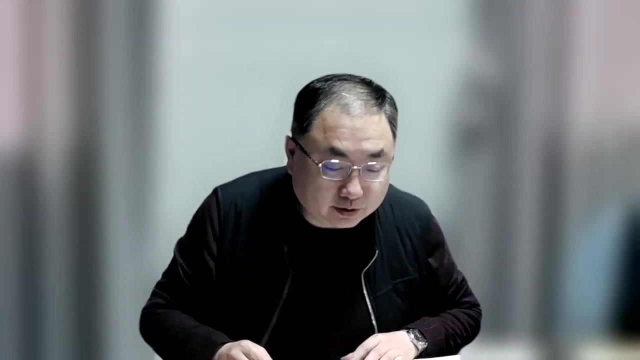 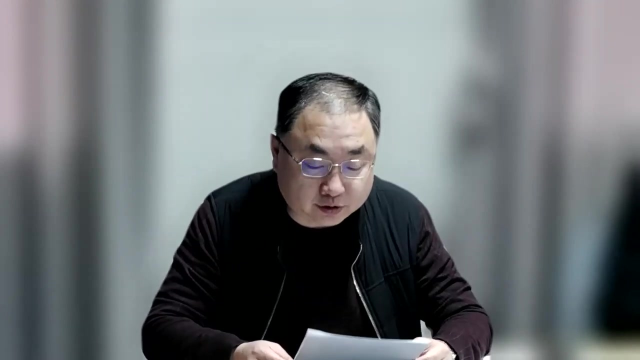 um three minutes is okay? yes, we can start okay. thank you. yes, we can start okay. thank you. yes, we can start okay. thank you, so, so, Good morning, ladies and gentlemen. This is Fan Wang, from Institute of Oceanology, Chinese Academy of Sciences, On behalf of the organizing committee and the program committee. 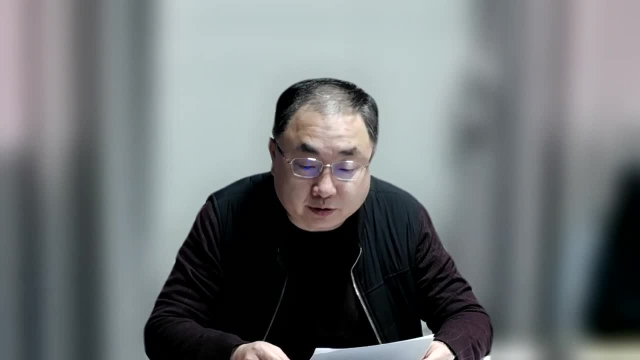 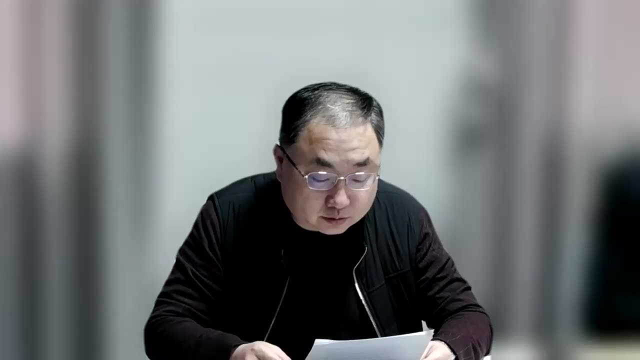 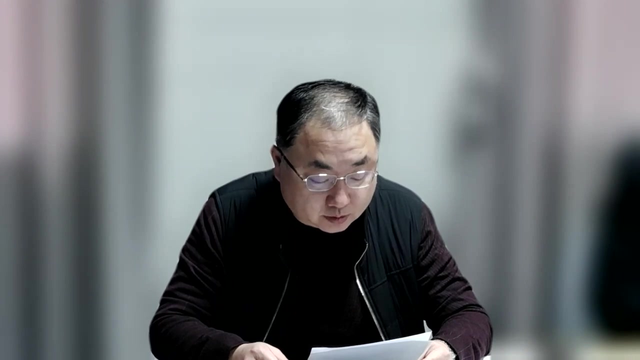 I'm happy to welcome your participation in DECADES Action Incubator 8,, which unlocks the mysteries and opportunities of marine biodiversity in the Indo-Pacific Convergence Center. The integrated investigation in the Indo-Pacific Convergence Center: Marine Ecosystem and Biodiversity- short for TRIPOL, IPCC, MEP. 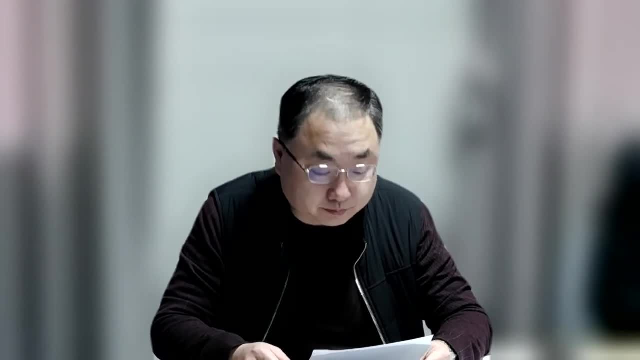 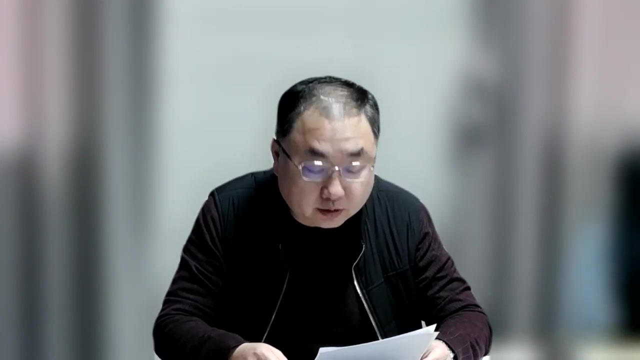 Initiative was firstly proposed at the regional consultative and planning workshop towards the UN Decade of Ocean Science for Sustainable Development for the North Pacific and the Western Pacific Marginal Sea in 2019 to Q to identify the priority issues on marine ecosystem and the biodiversity reach in the IPCC area and the development solution to reverse the 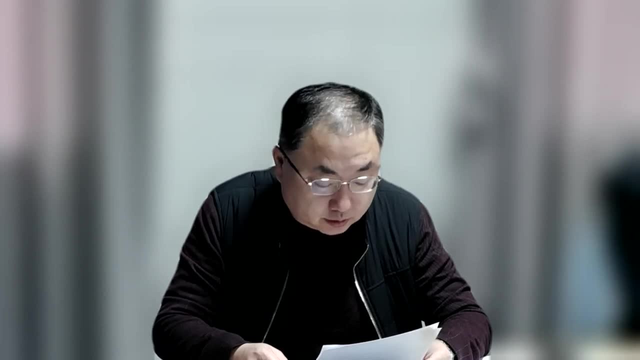 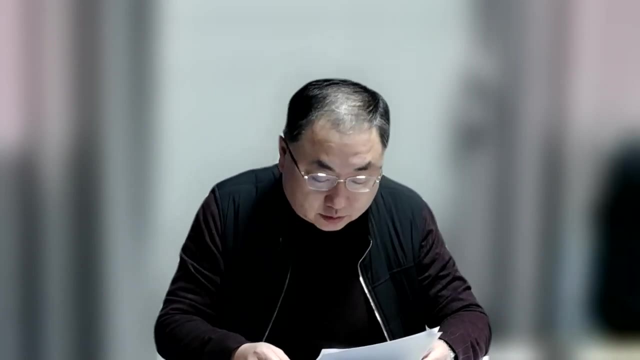 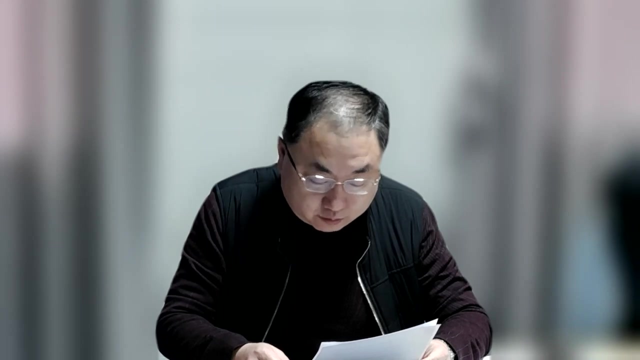 deterioration of the marine biodiversity from multi-layer and multi-disciplinary perspectives. With the support of IOC, Westpac, a TRIPOL IPCC MEP Working Group was formally established in April this year to strengthen the regional collaboration and development programs, The IOCAS, CMAC's. 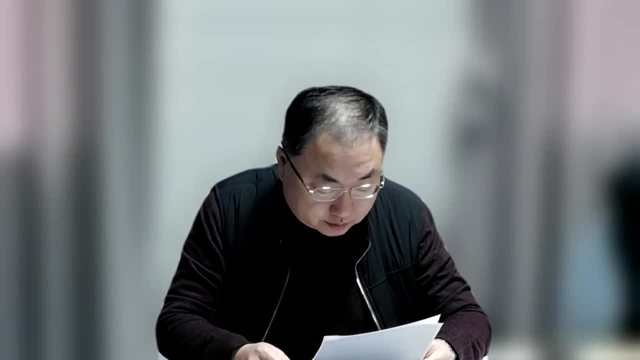 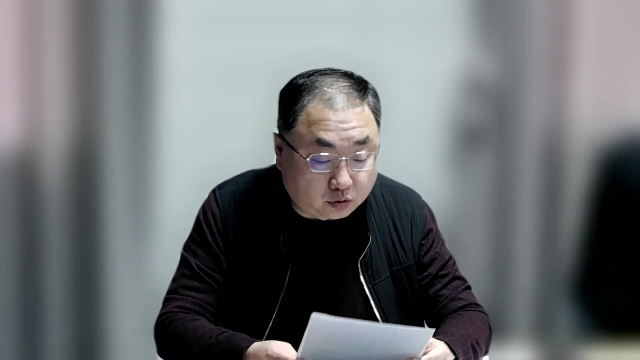 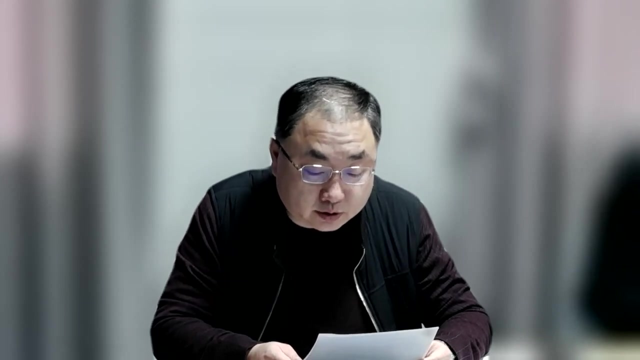 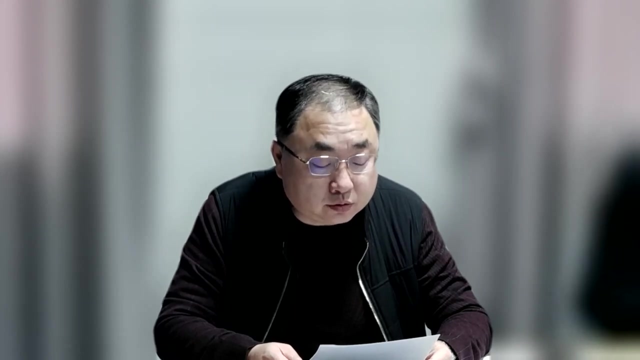 USM and the RCO brand want to jointly propose the unlock the mysteries and opportunities of marine biodiversity in IPCC area. side event to dissemination. to disseminate the concept of TRIPOL IPCC MEP Initiative and engage the science-based community and the society in this region for further collaboration. 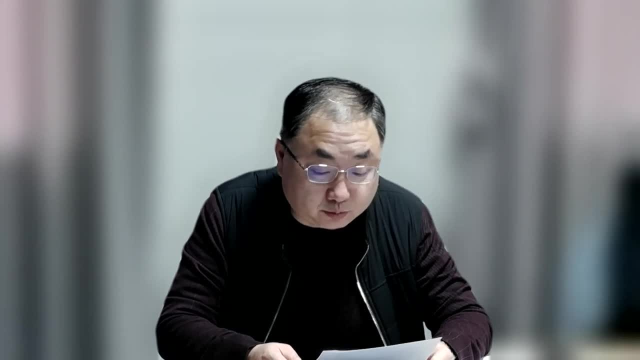 This side event will provide a platform for promoting the co-design process of TRIPOL IPCC program amongst ocean science, community policy makers, private sectors and civil society, towards the identification and the development of science-based solution to protect the and preserve the marine biodiversity in this region. 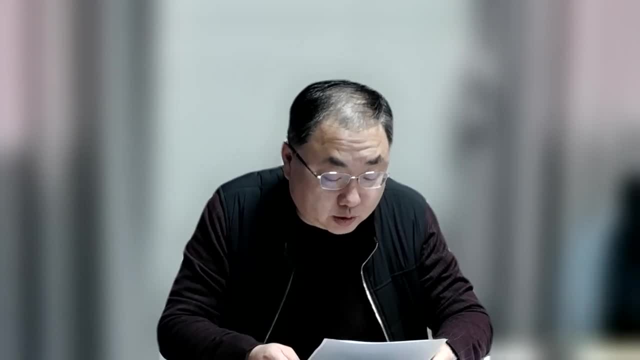 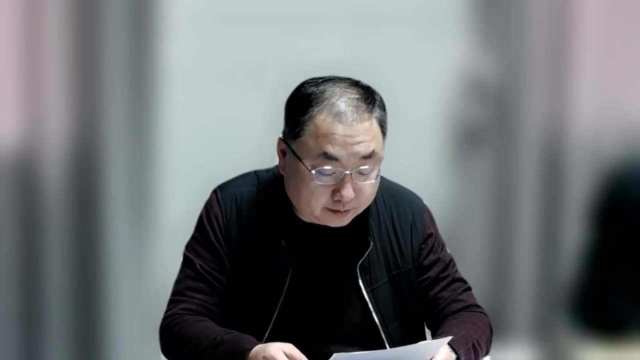 And today we are honored to have invited the professors and various stakeholders to attend this side event. Firstly, let's warmly welcome Mr Wen Tao Wang from the Administrative Center for China's Agenda 21st. Mr Wen, welcome to China's Agenda 21st. 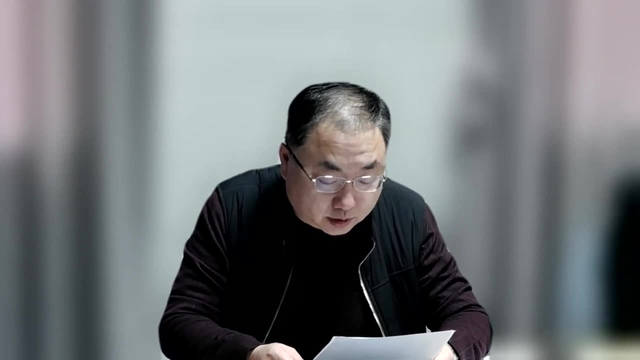 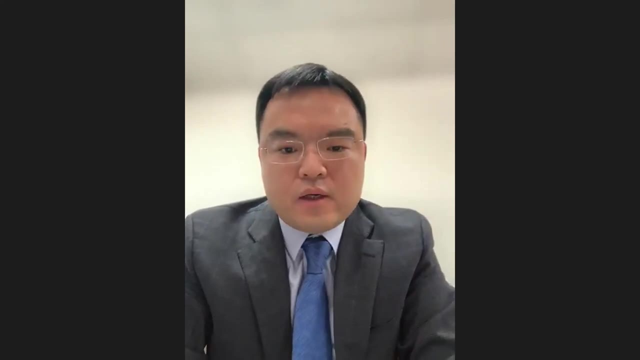 Mr Wen, welcome to China's Junta for Center for China's Agenda 21, Ministry of Science and Technology. I would like to express my sincere gratitude to the organizer, the Institute of Ocean Knowledge, Chinese Academy of Science, and also my great thanks to all the online participants As an once-in-a-lifetime 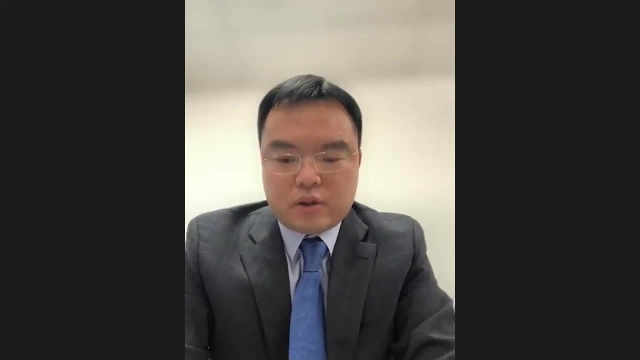 opportunity. UN Decade aims to lead a revolution in ocean technology and global ocean governance. Three goals and seven outcomes have been proposed. I noticed that the slogan of this kick-off meeting for the Western Pacific is to join the collective global movement, engage with various stakeholders. 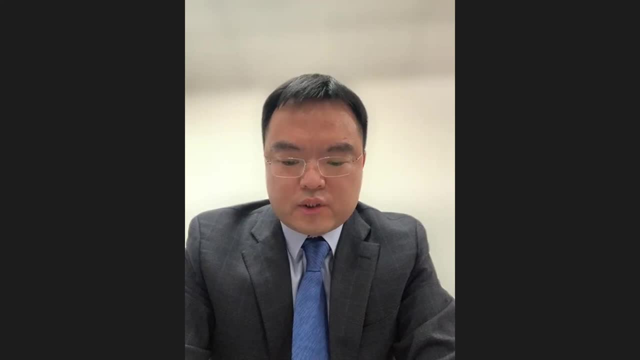 in this region and develop ocean science solutions for the ocean we want, which I think fits very well with the goals of UN Decades. Indo-Pacific region is deeply influenced by many oceanic activities. So far as I know, Indo-Pacific Convergence Center is recognized as the global center of marine. 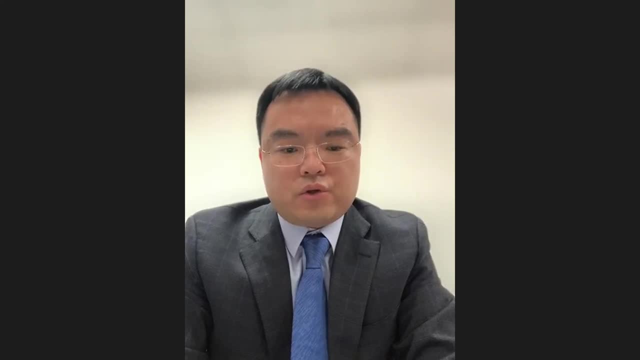 biodiversity. Many scientific issues associated with the biodiversity center, however, have not yet been explored, including species and geographic distribution patterns, region and evolution of marine organisms, diffusion regularity and driving factors, and so on. As stakeholders in the Indo-Pacific region, how to reverse the trend of ocean health decline. 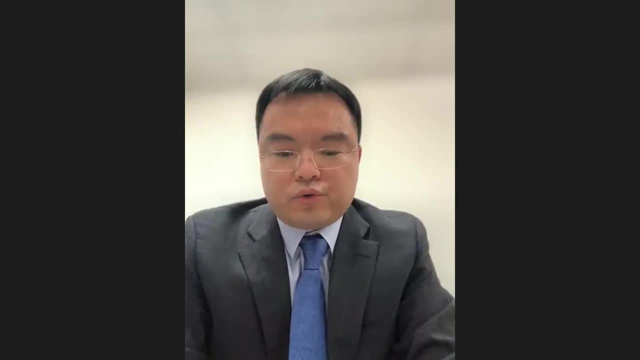 how to protect marine biodiversity and how to rationally use marine resources. we need to give scientific answers and make more research works. Our center acts as a pioneer and driving force for China toward sustainable development. During the 14th Five-Year Plan, the budget managed. 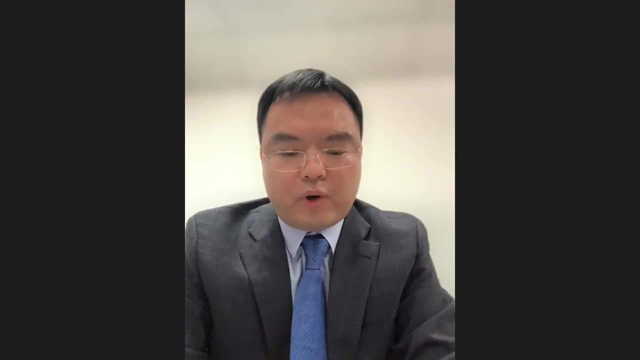 by our center for R&D in ocean and polar fields has reached more than 6 billion Chinese yuan, which carries most of the SDG 14 targets, like reduced ocean pollution, geotrification, ocean acidification, overfishing, ocean prediction, ecosystem health and so on. 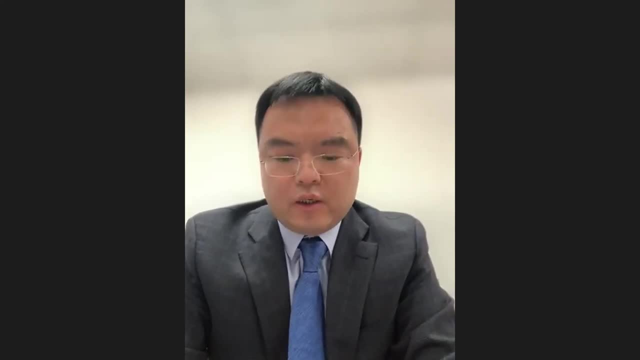 ACCA21 also has more than 40 cooperative partners from all over the world in the fields of climate change, ocean and polar science. We take the lead of the BRICS country's working group on the ocean and the polar fields, actively participating in the IPCC, LDP, the Arctic Circle and other. 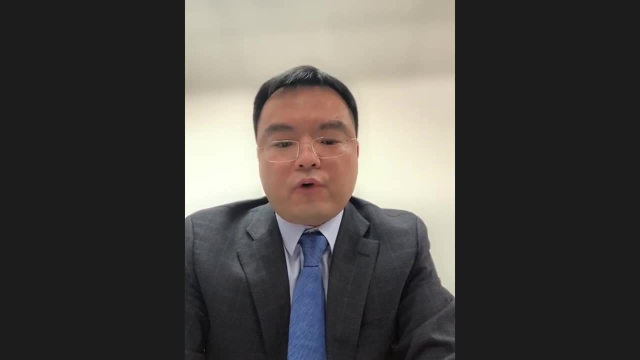 cooperation in this field. Our center fully supports the UN-dedicated actions activities and our activities. We also support the UN-dedicated activities activities and our activities In the incubator eight. it is great to see that scientists from Indonesia, Malaysia 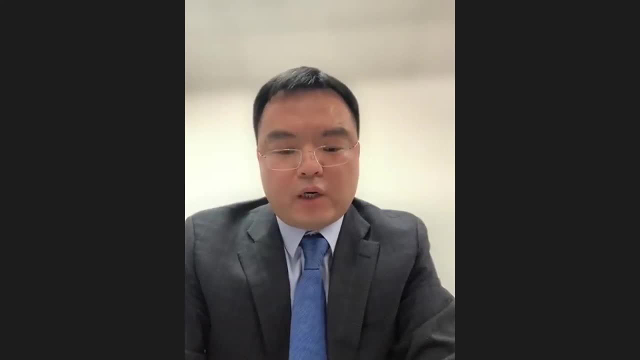 and China are working together to focus on the marine biodiversity in the Indo-Pacific Convergent Center. Scientists research on different aspects from climate change, chemical perspectives to protection and design international programs. I wish the incubator eight a big success. Thank you. 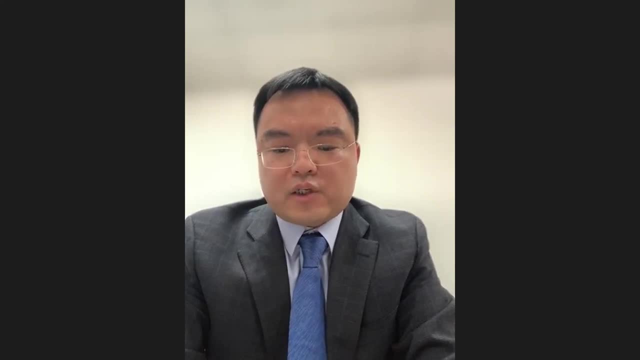 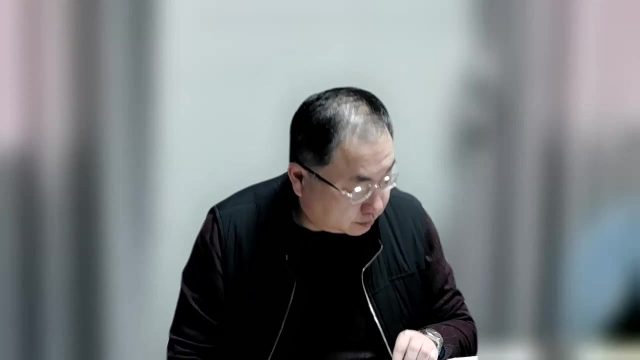 and wish our international scientific team discovers the marine biodiversity mysteries and sees the great opportunities to develop more collaborative activities. That's all, Thank you so much. Okay, thank you. Thanks for Winter's speech. So next please welcome Ms Dongyao Wang. 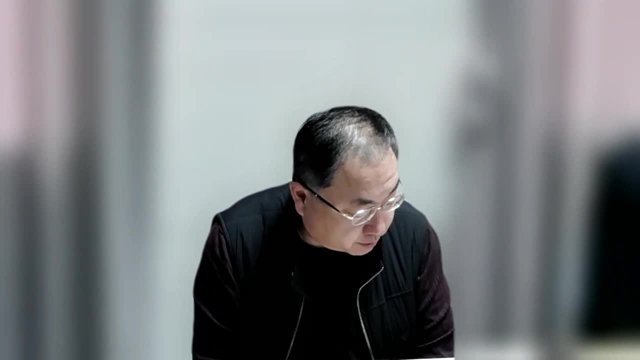 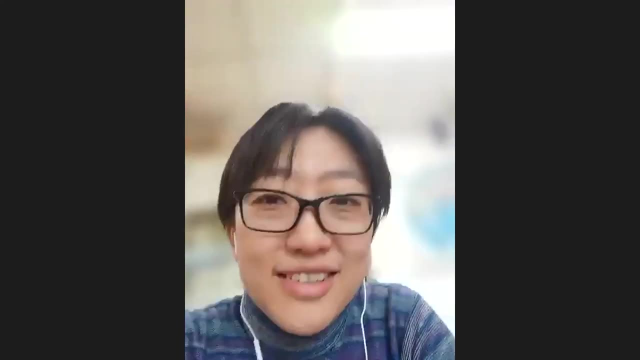 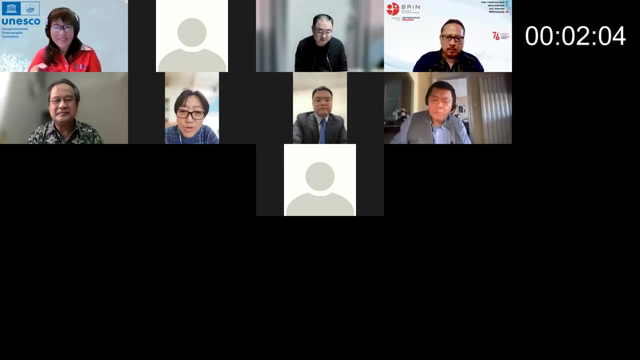 from Bureau of International Cooperation, Chinese Academy of Sciences. Dongyao please, Yes, hi. Thank you, Professor Wang. Long time no see. So, dear colleagues, ladies and gentlemen, good morning. I'm Dongyao Wang, from the Bureau of International Cooperation of Chinese Academy. 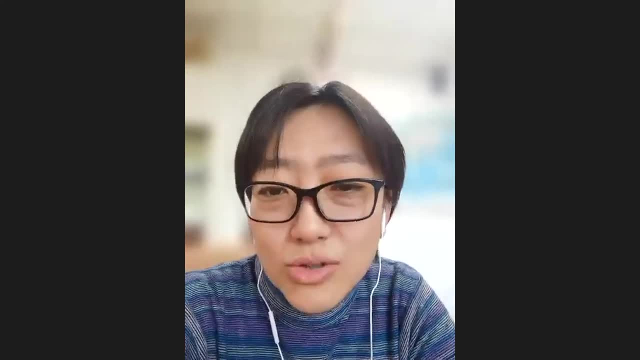 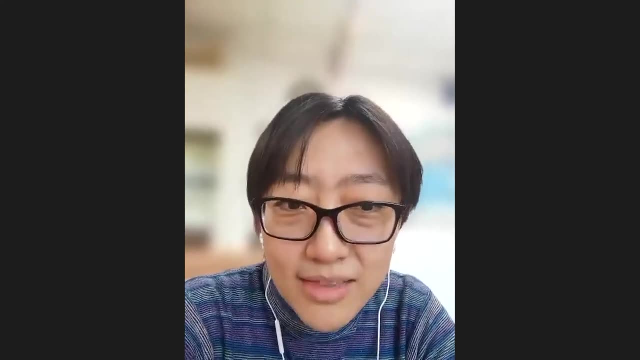 of Sciences, It's my great honor to be invited to participate in this meeting. As you know, the ocean is crucial to all the life on Earth and the prosperity of human society. In the past decades, the ocean has been the most important source of life for human beings. It is the 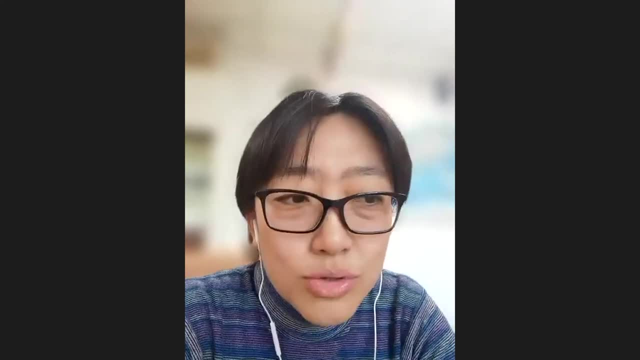 most important source of life for human beings. It is the most important source of life for human beings. It is the most important source of life for human beings. Human activities brought huge stress to the ocean, which caused obvious degradation of marine environment and adversely 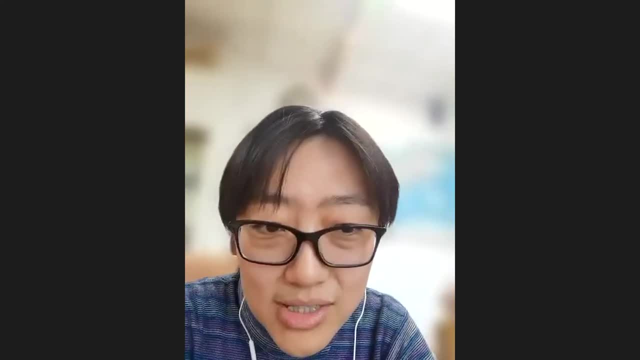 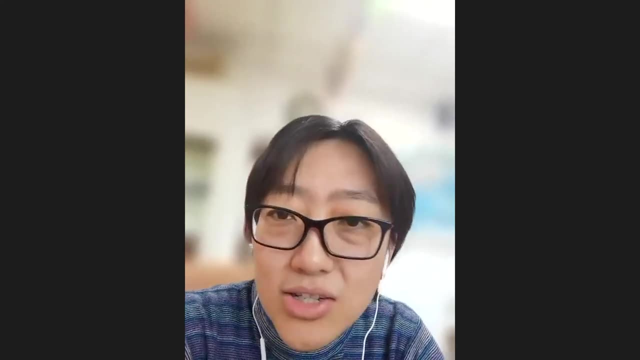 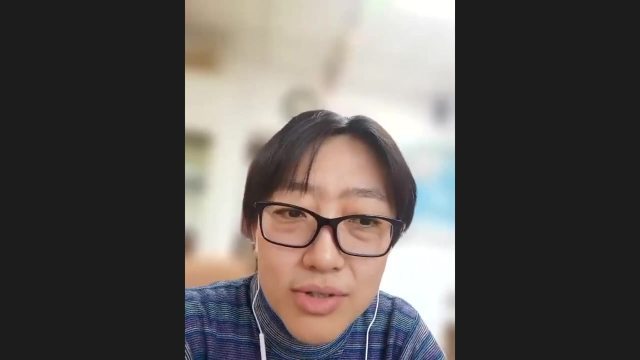 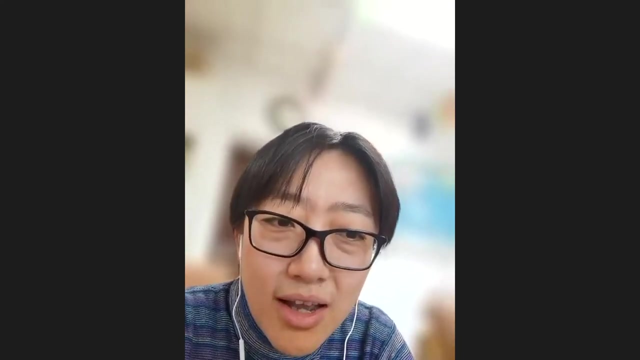 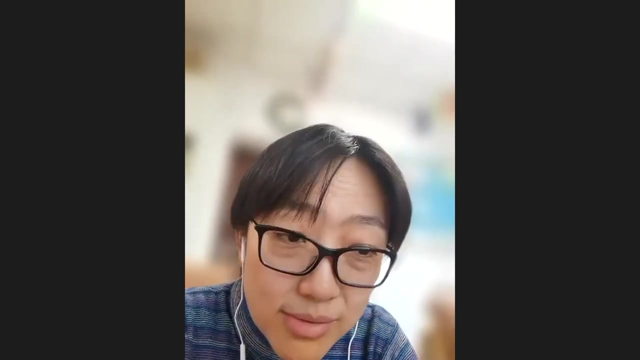 affected the marine ecosystem. As one of the national academies in the region, the Chinese Academy of Sciences has always attached great importance to the study on the sustainable development and protection of the marine environment and always highlighted the importance of the international communication and cooperation to tackle this trans-borderly and interdisciplinary challenge Nowadays. 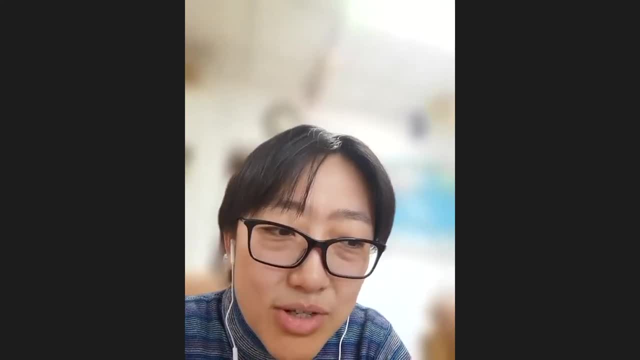 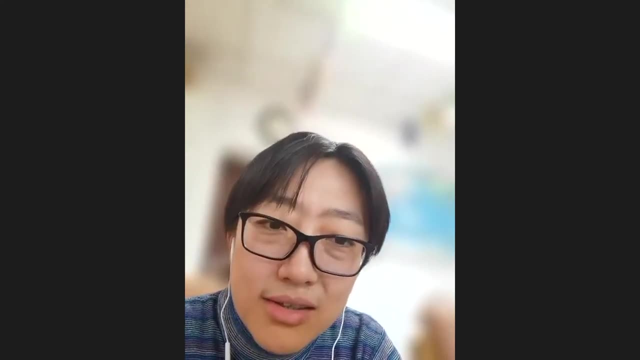 the scientists from different countries have established extensive collaboration and achieved many valuable results. I think the IAEA and the Chinese Academy of Sciences have been very successful, and I think the IAEA and the Chinese Academy of Sciences have been very successful and very successful. Nonetheless, they are not just the foundation to the social development. 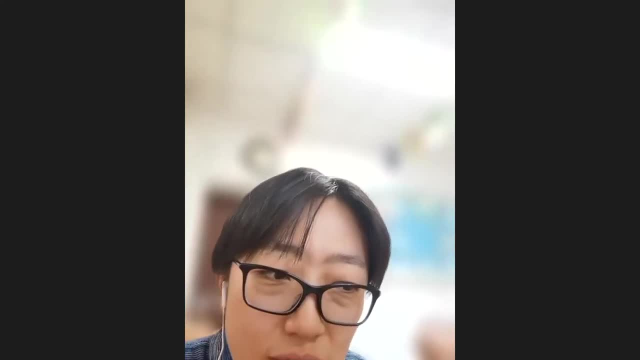 They are also the foundation of the human resources and the cultural development that the Chinese Academy has developed over the many years of the Chinese economy. I am very proud to present today my triple PCC MEB initiative, which proposes a very practical and inspiring action plan. I know Professor Yu will give more details about it later. I wish this 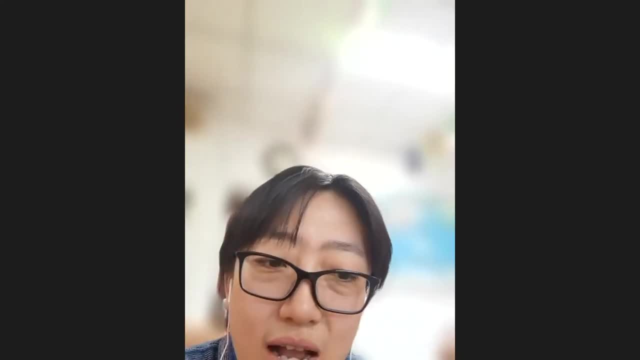 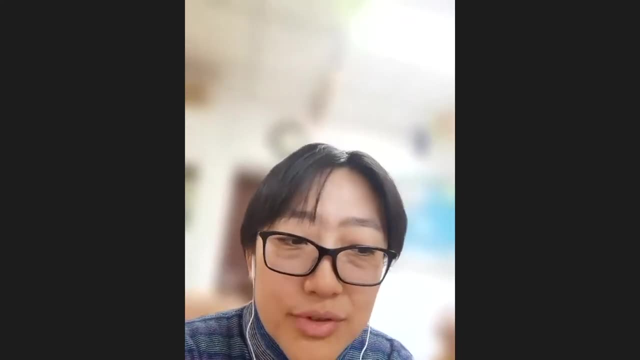 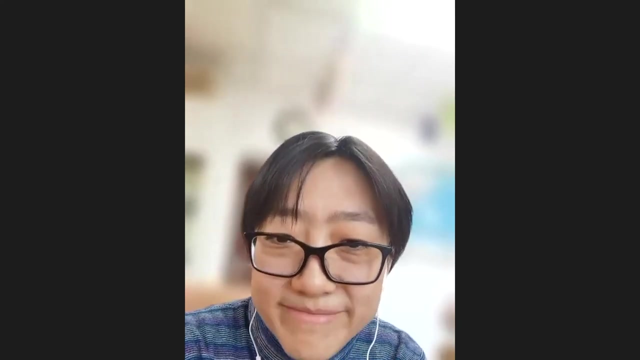 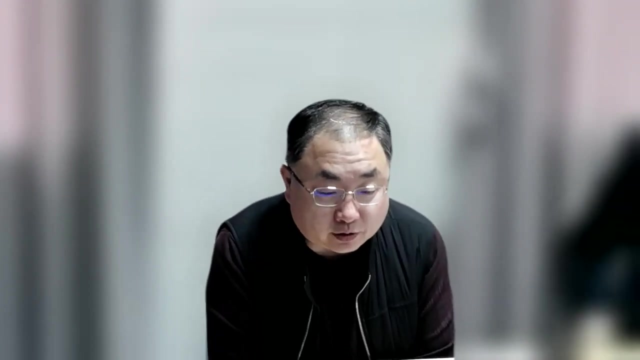 initiative will attract more stakeholders and scientists from the different countries to work parties. we will make a greater contribution to the UN decade of ocean science for sustainable development. I wish the meeting a great success, Thank you. Thank you very much, Dongyang. And according to the request of 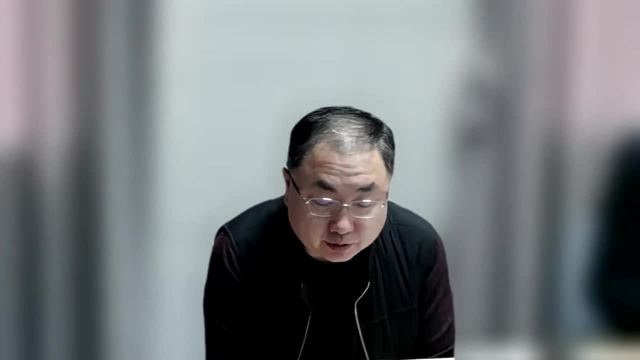 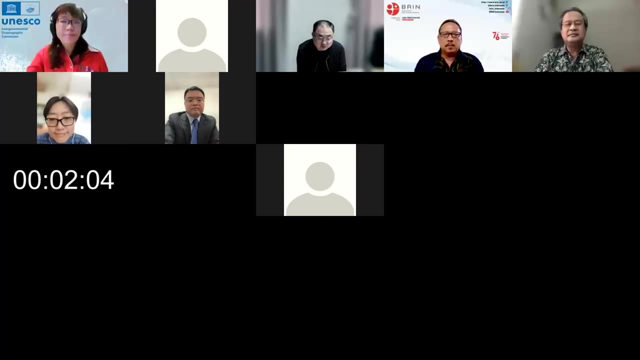 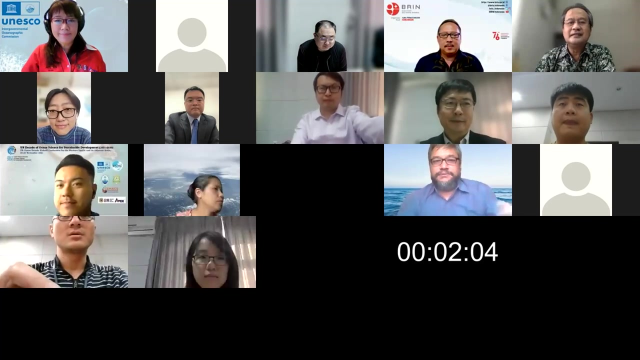 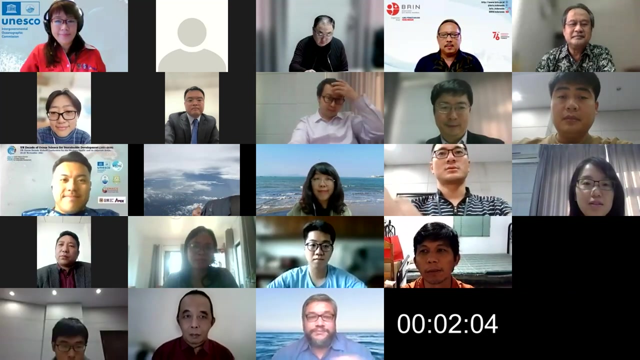 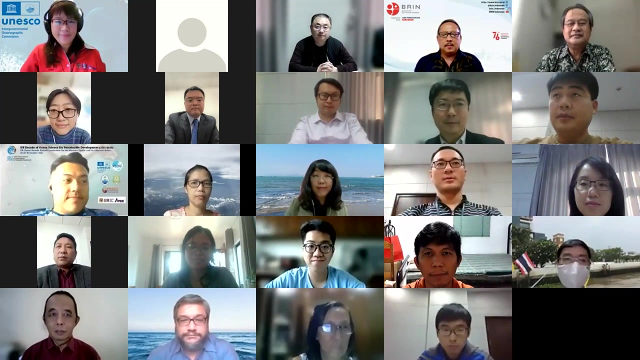 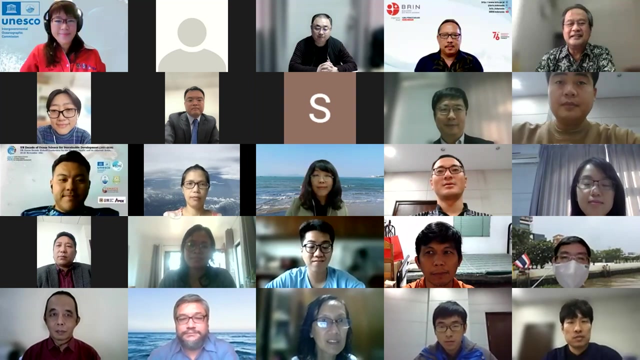 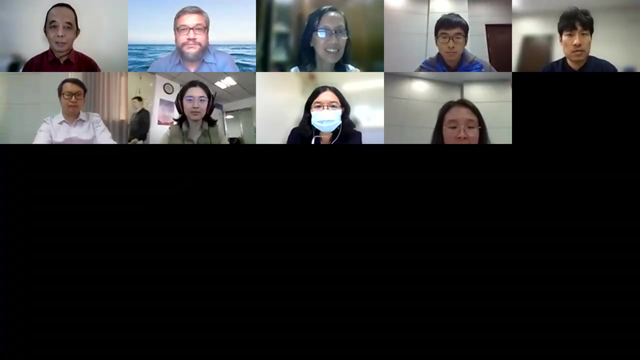 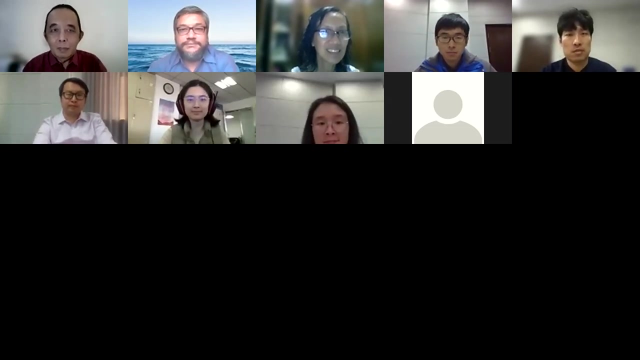 the kickoff conference. we should take a group photo, And could you please open your camera? All right, everyone is ready. Okay, one, two, three, Smile. Yeah, Okay, another pitch. We have quite participants today. One, two, three, Thank you so. 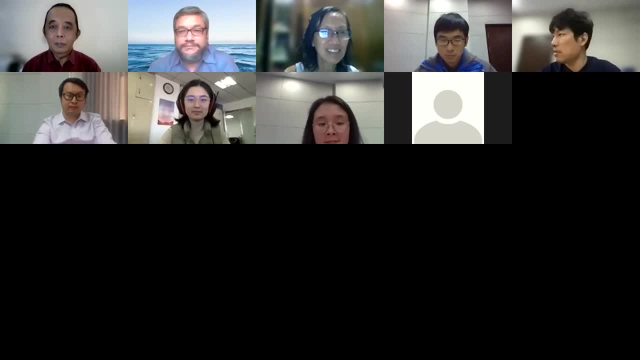 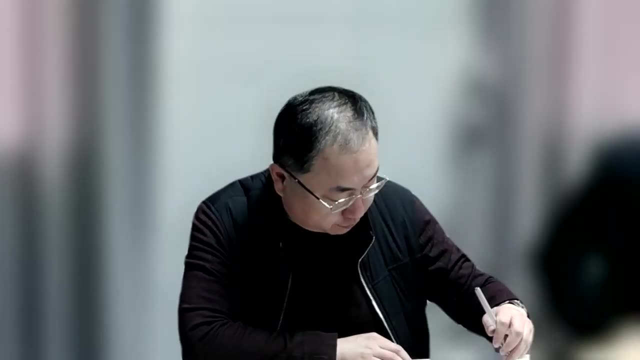 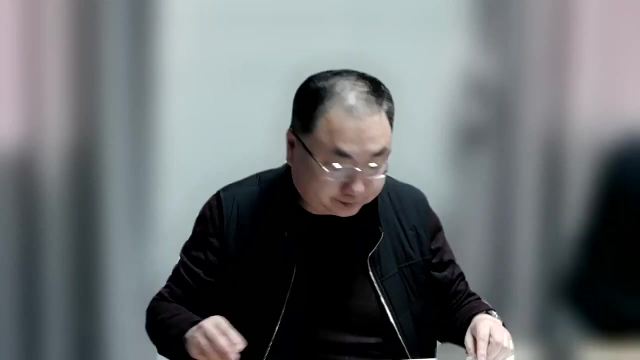 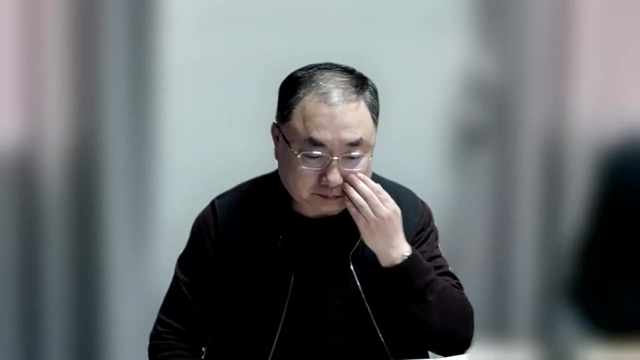 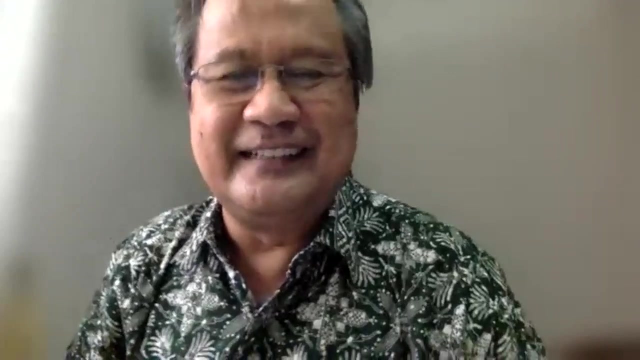 much, Hey, wonderful. So thank you very much. And now, according to our agenda, I will give my the host right to to part center. please, Now, please. Thank you very much, Prof Wan, for handing me to chair this 60. 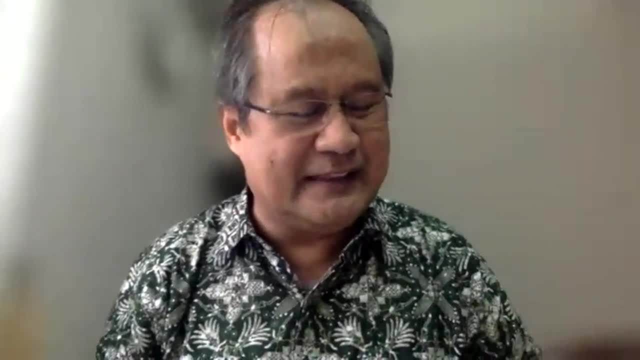 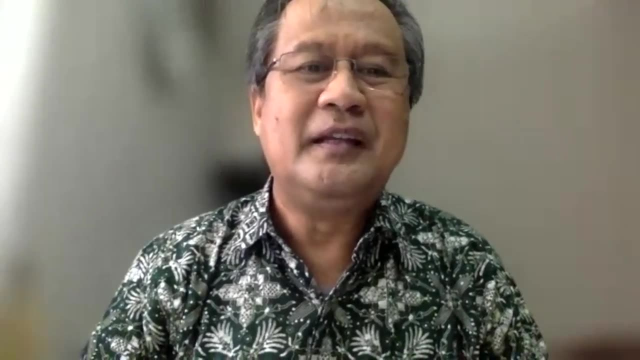 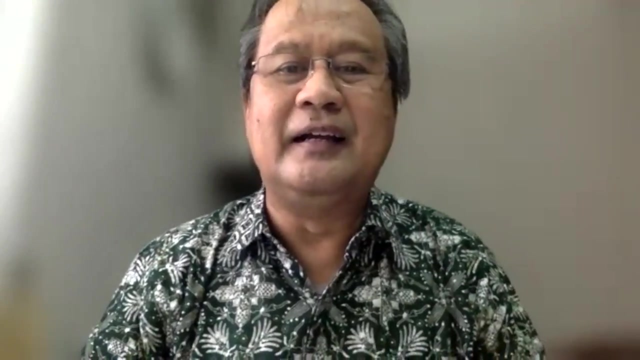 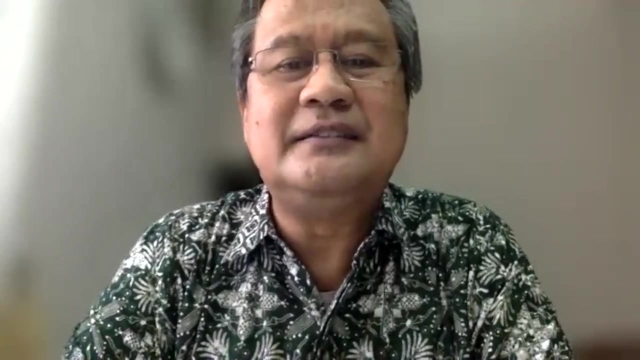 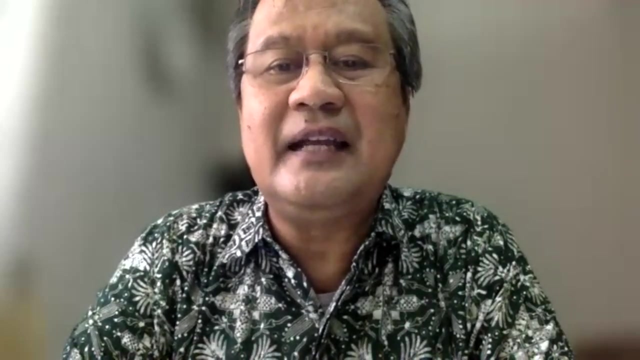 minute presentation or discussion later on. So the first speaker today will be Professor Fan Wang from Institute of Oceanology China Academy of Science. So he is a director of the Institute of Oceanology China Academy of Science and Yantai Institute of. 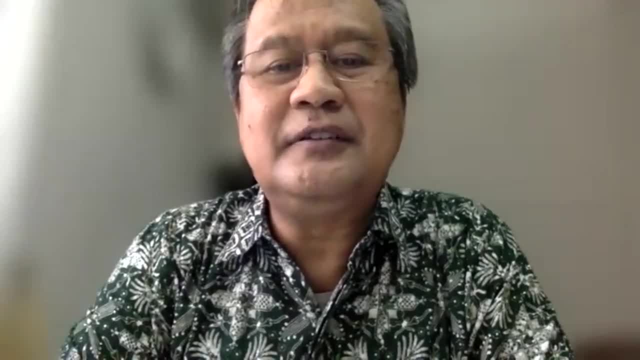 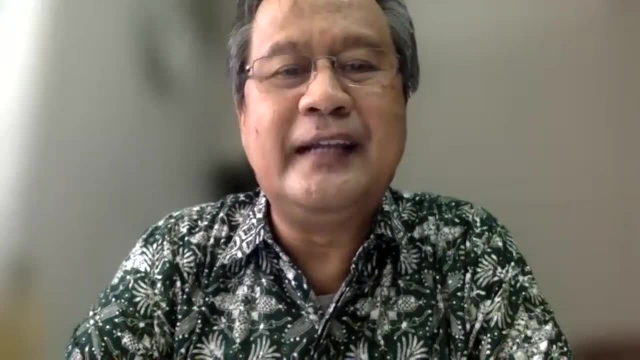 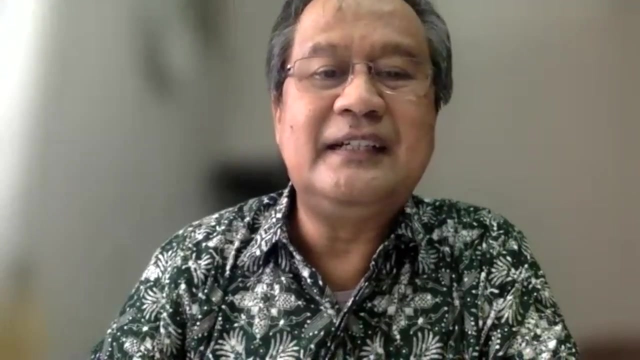 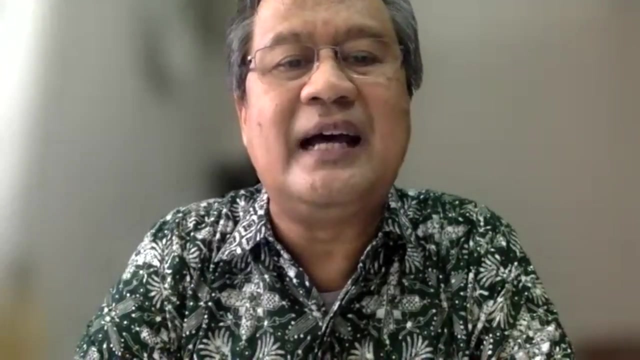 Coastal Zone Research. He is also Dean of Marine Science College, University of China Academy of Science, So for the next 15 minutes, Professor Wang will present the talk on climate change impact on marine biodiversity in the IPCC area. So the time is yours. 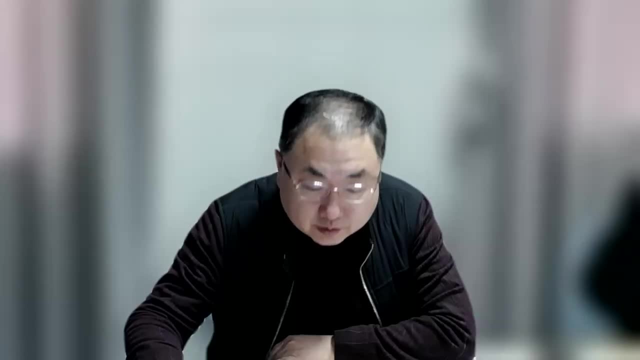 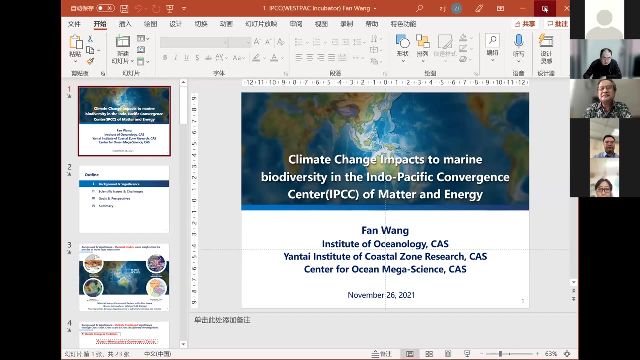 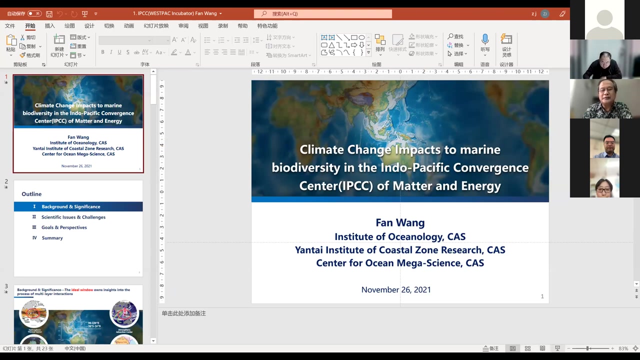 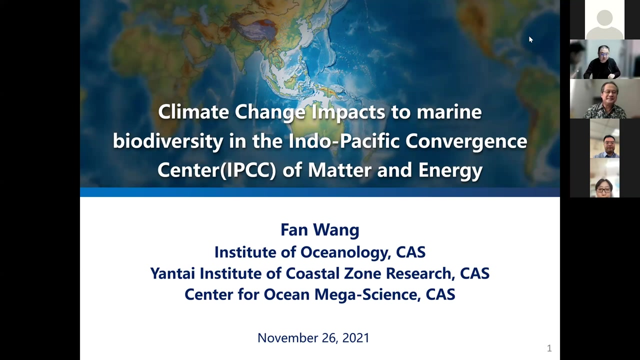 Professor Wang. Okay, thank you, Let's share my screen, Would you see? Could you see it? Yes, it's clear, But could you? could you please use Right? Okay, that's good, Okay, Okay, Thank you. part center And ladies and gentlemen, today I would talk about the multi-layer or multi-sphere interactions in the Indo-Pacific Convergence Center. 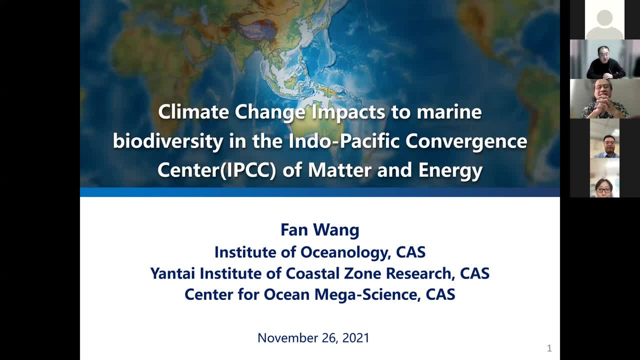 Today I would talk about the multi-layer or multi-sphere interactions in the Indo-Pacific Convergence Center of matter and energy, especially the climate change impact to marine biodiversity, of matter and energy, especially the climate change impact to marine biodiversity. My talk includes four parts. The first one is about the background and the significance. 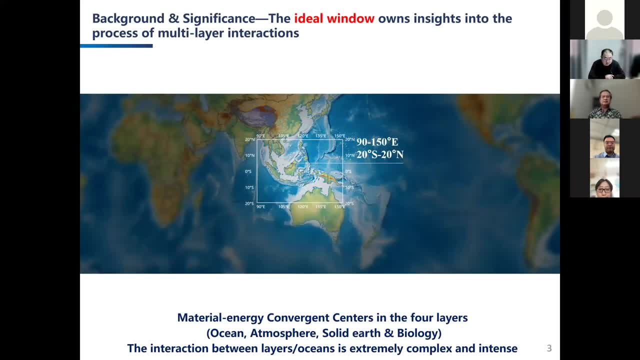 The Indo-Pacific Convergence Center is located between the Pacific and the Indian Oceans and there is the Indo-Pacific Warm Pool as the thermal Center of the ocean, the atmosphere and the environment вокруг it. In this context, the Indo-Pacific Convergence Center, or extensively partout at the ocean, up to the nations living on the surface, then there is the Indo-Pacific Warm Pools. 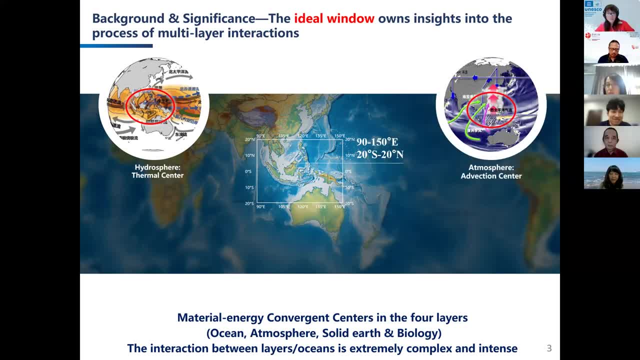 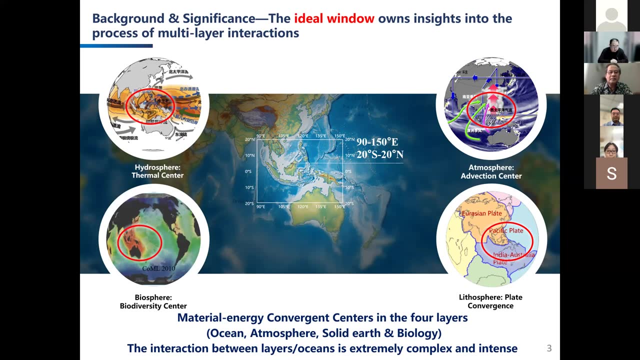 as a thermal center of ocean and there is a very strong advection center in the atmosphere over the warm pool and there are three, please uh, converging to this area. and, finally, there is a bio diversity center over the whole, uh, the global ocean, even though the whole globe. so there are material energy convergence centers. 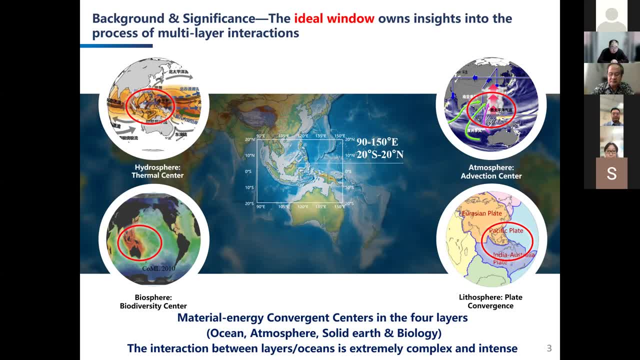 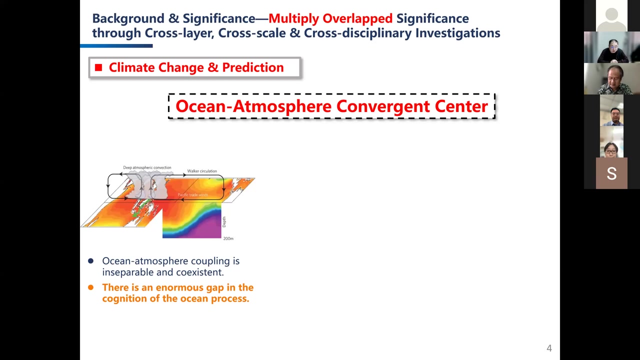 of the four layers of the earth system. the interaction between layers and the oceans is extremely complex and intense, so this area study give us an ideal window on insights into the processes of multi-layer interactions, and the comprehensive study in this area has a multiply overlapped significance. 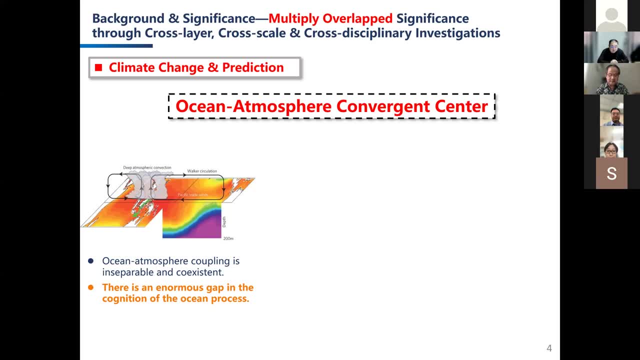 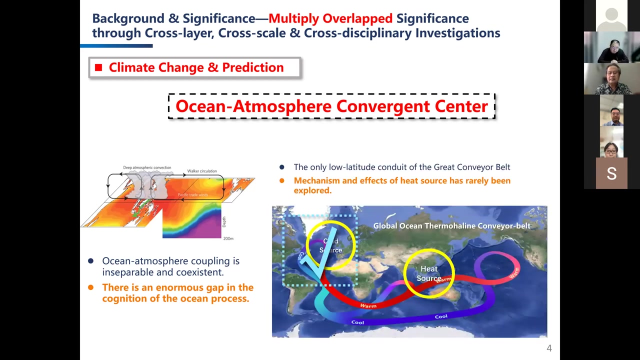 through closely across scale and across disciplinary investigations about climate change and prediction. the ocean and the atmosphere convergence center was formed is formed, uh, by the full coupling between ocean and the atmosphere. however, there is a enormous gap in the cognition of the ocean processes meanwhile, as the print source of the global thermohelium reconvert. 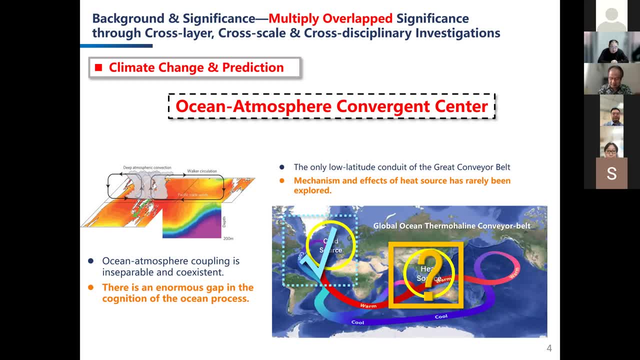 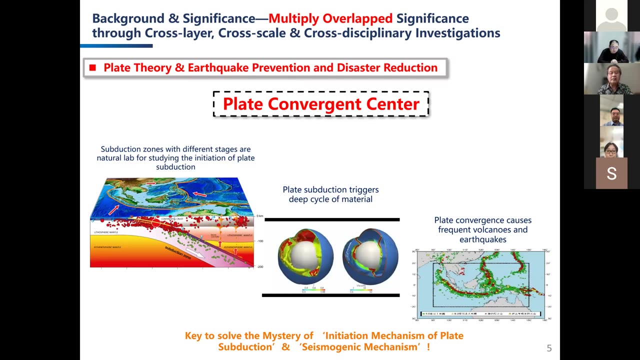 belt. the mechanism effects has really been explored, comparing to the code source in north atlantic ocean about the place theory and the earthquake prevention and disaster reduction. there are lots of subduction zones with different stages as natural lab for studying the initiation of plate subduction and plate subduction triggers. 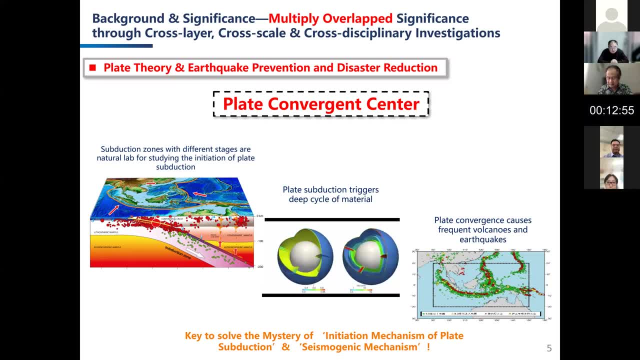 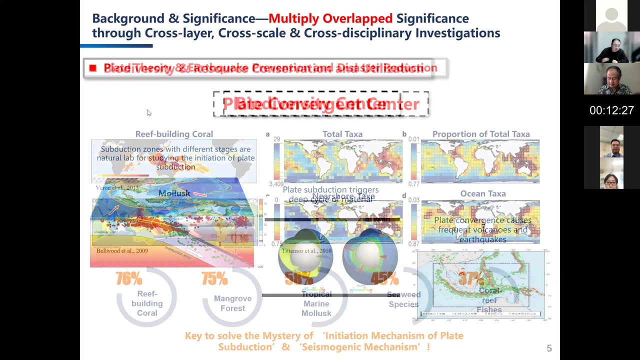 deep cycle of energy, energy and material, uh. among the uh, the solid earth, the ocean and even atmosphere. plate convergence causes frequent volcanoes and earthquakes in this area, so the study will offer us a k to solve the mystery of initiation mechanism, of plate subduction and seismogenic mechanism, and about biodiversity and resource conversion, conservation and utilization. 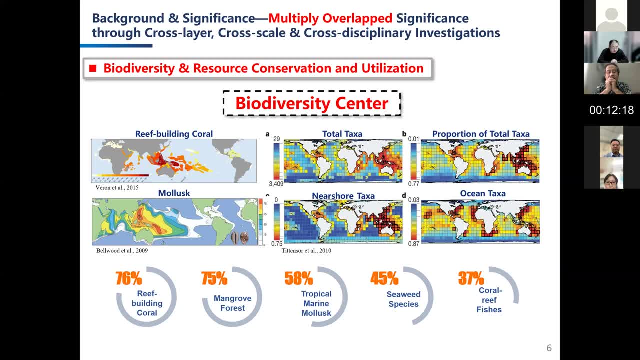 this area holds about 76 percent ree Lights power, about 76 percent refined temporal resonance, while展 dark tanks are shaking but mummies have to make cattle and help them adapt position, behaviors and structure the flow of dry soil along the wall한 building coral, 75% mangrove, 58% mollusk, 45% seaweed and 37%. 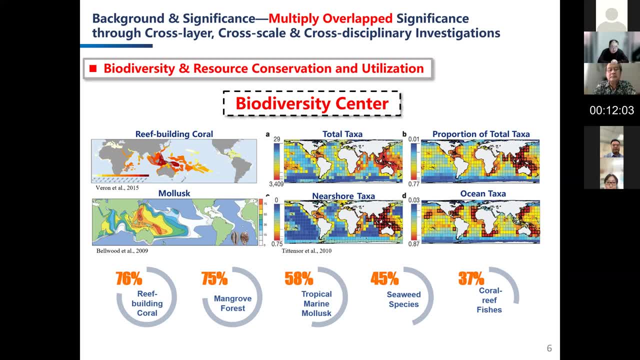 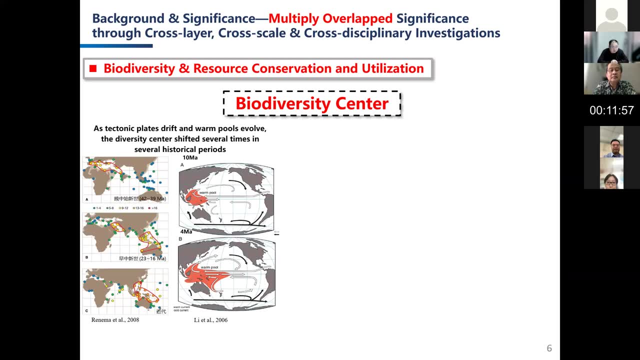 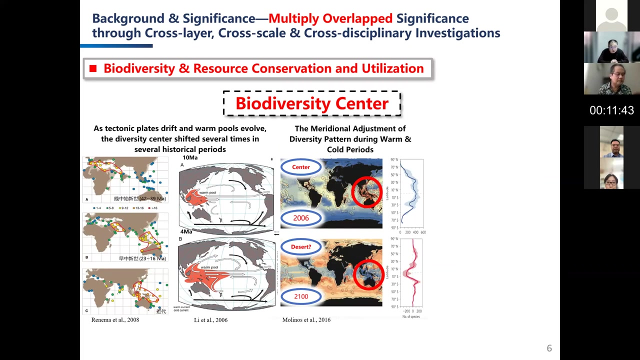 coral reef, fish species among the global ocean And as a tectonic place shift and warm pool involved, the diversity center shifted several times in several historic period And between the grisal and intergrisal period the diversity pattern adjusted meridional and at present the distribution 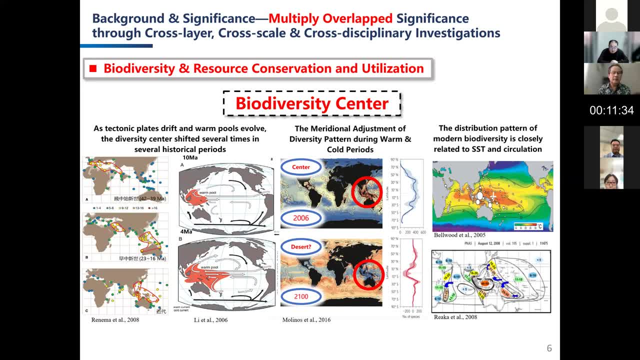 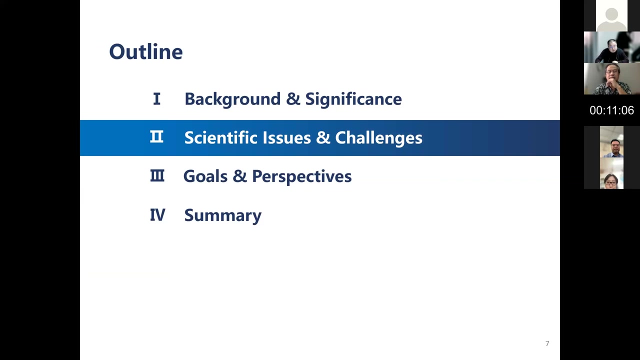 pattern of modern biodiversity is closely related to the sea surface temperature and circulation, So the climatic, environmental and biological relationships is crucial to solve the mystery of the formation and evolution of the biodiversity center and the latest scientific foundation for diversity conservation and sustainable utilization of resources. The second part is about the scientific issues and 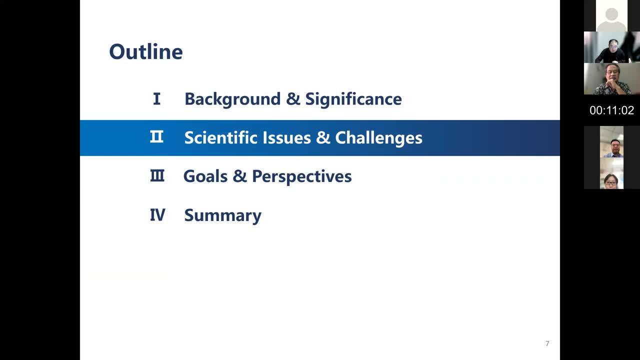 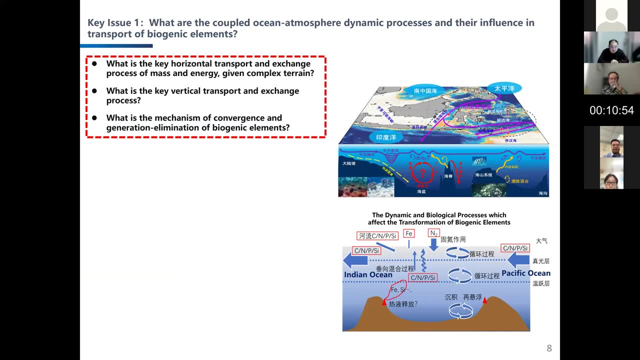 challenges we will face to. The first issue is: what are the coupled ocean atmosphere dynamic processes and their influence in transport of biogenic animals? The second is question about the role of biogenic elements, including the key horizontal transport and exchange process between oceans. given the very complex terrain, The key vertical 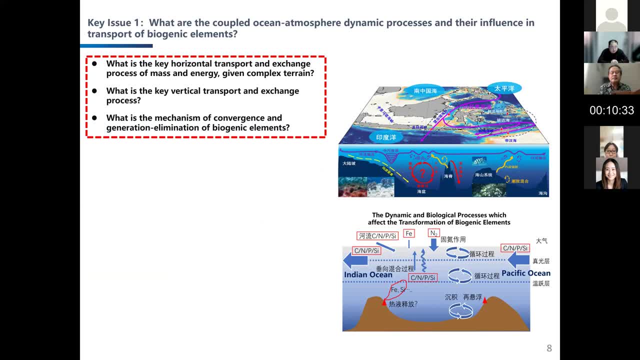 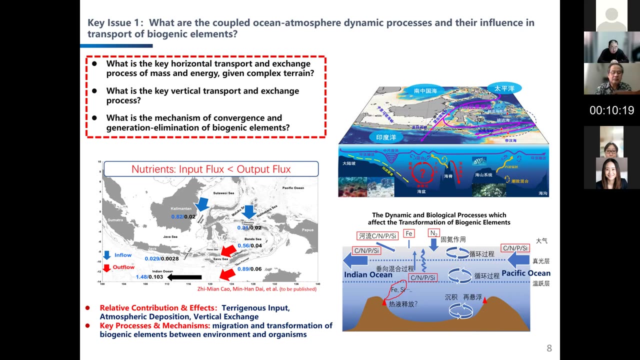 transport and exchange processes between the upper and the deep ocean and the mechanism of convergence and generation. elimination of biogenic elements: The key factor. we should include the terigenous input, atmospheric deposition and oceanic vertical exchange, especially the migration of transformations of biogenic elements between environment and 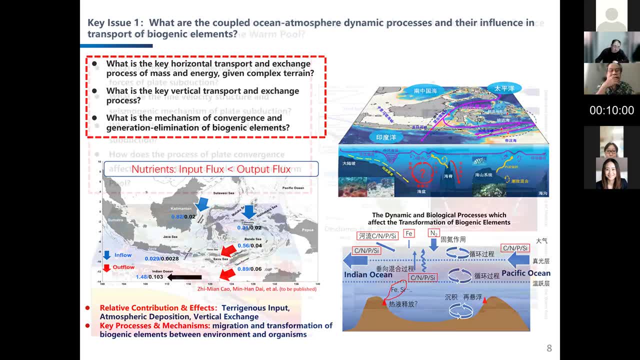 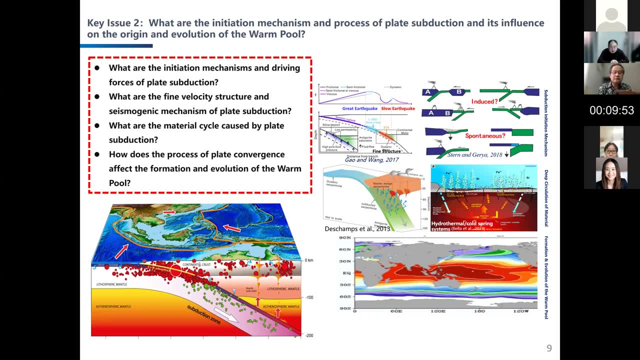 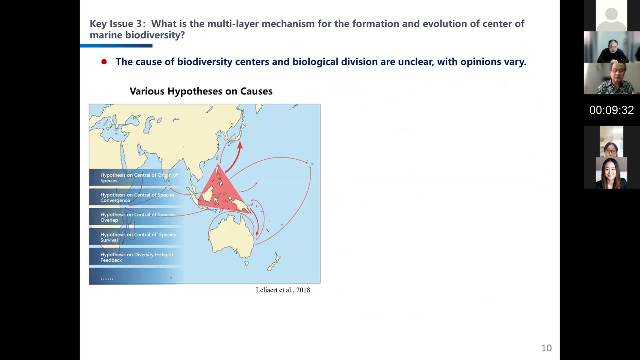 organisms. The second issue is: what are the initiation mechanism and process of plate subduction and its influence on the formation, evolution and the worm pool and, firstly, the center of marine biodiversity? And the third one is: what is the multi-layer interaction mechanisms for the formation and 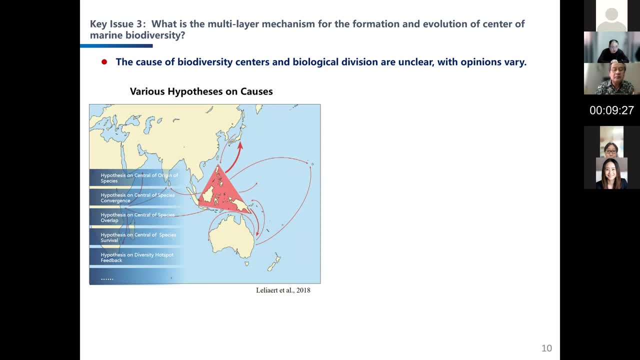 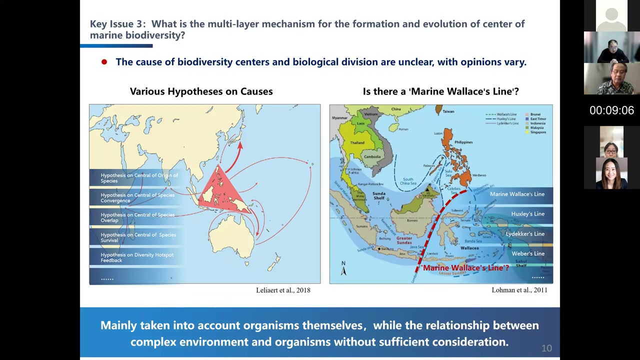 evolution of the center of biodiversity. As we all know, there have been several different hypotheses of the center formation, but they are unclear and even controversial. Is there a unique mechanism or is there a marine wireless line? And the previous studies have mainly taken into account the organisms themselves, while 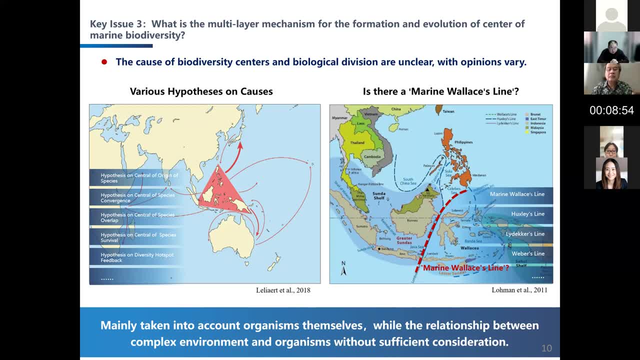 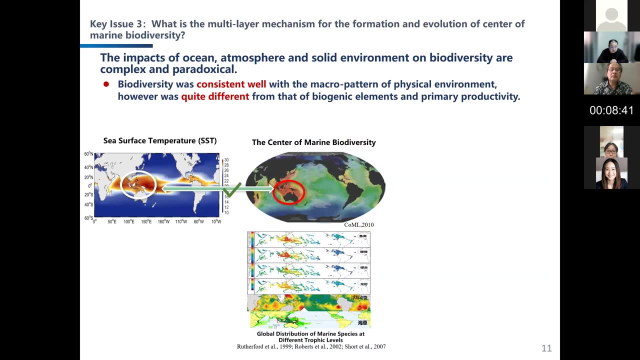 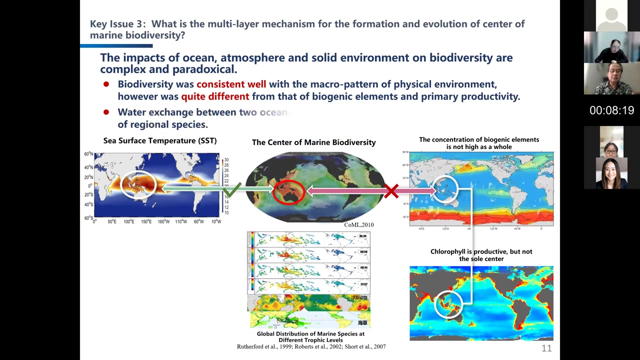 the relationship between the complex environment and the organism. It may alsokry cylinder of paleontology. Now we will go on to the next your slide. So already the unprecedented texts used the amp on Baldwin, genic elements and primary production and water exchange between two oceans. 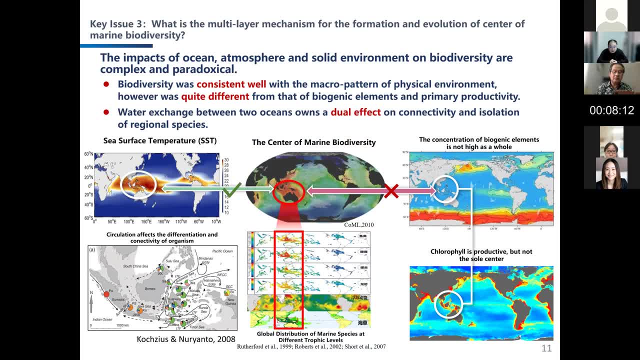 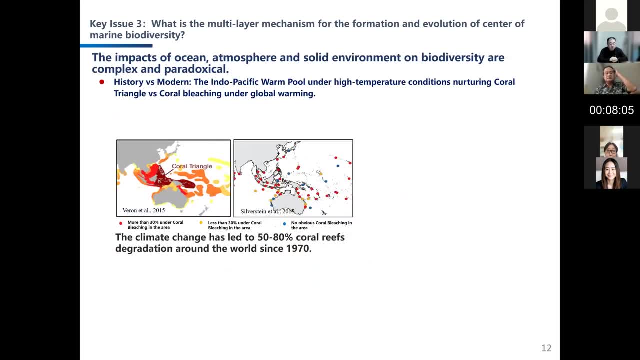 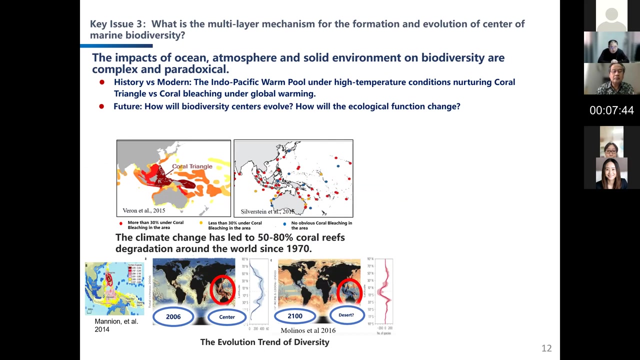 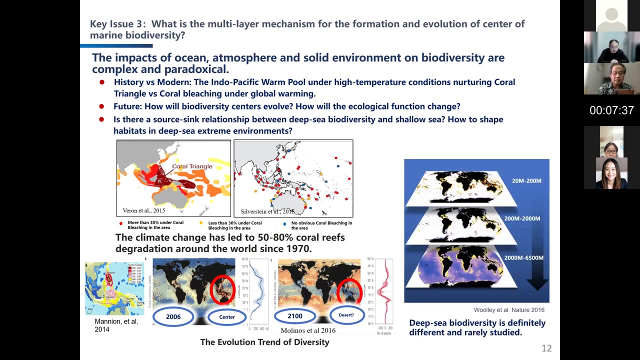 owns a dual effect on connectivity and isolation of the regional species. the indo-pacific warm pool conditions, the coral triangle: coral breaching occurs under global warming, as many studies show. and in the future, how will diversity centers involve and how will the ecological function change? is there a sourcing relationship between deep sea biodiversity and shadow sea? how to ship? 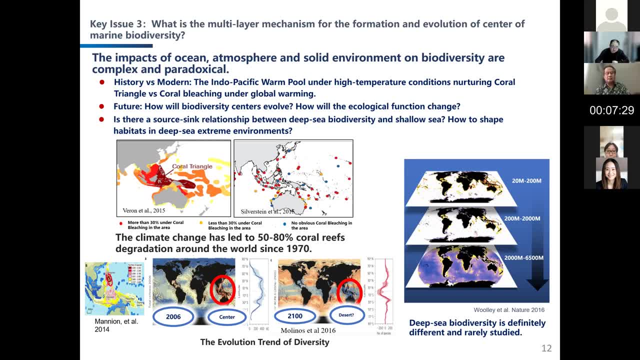 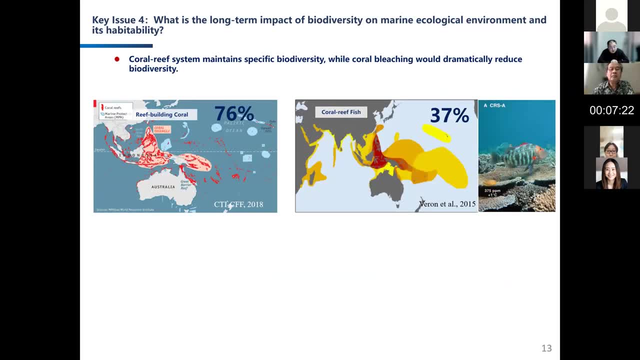 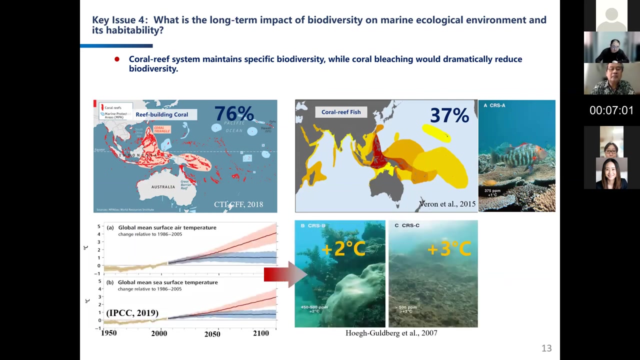 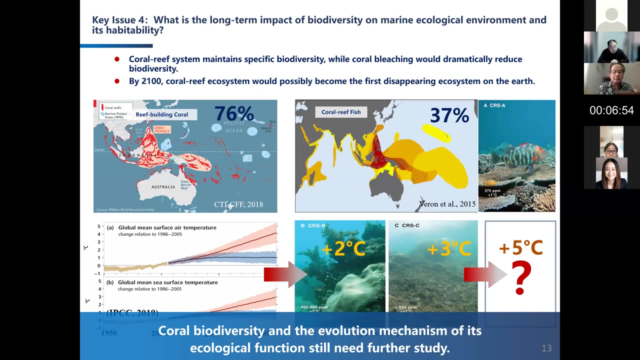 heavy case in deep sea extreme environment. and the fourth issue is about the long-term impact of biodiversity on marine ecological environment and its ability. the coral reef system maintains specific biodiversity well. the coral breaching would dramatically reduce the biodiversity and, as some studies show, by 2100. 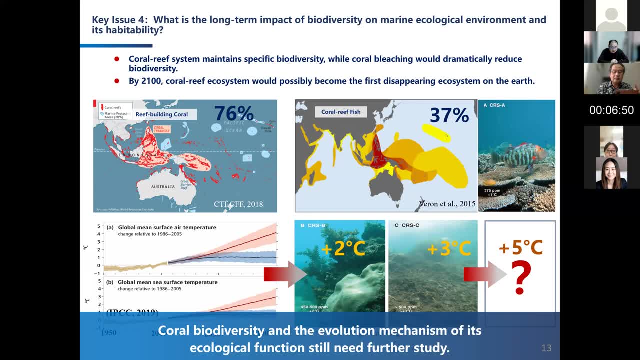 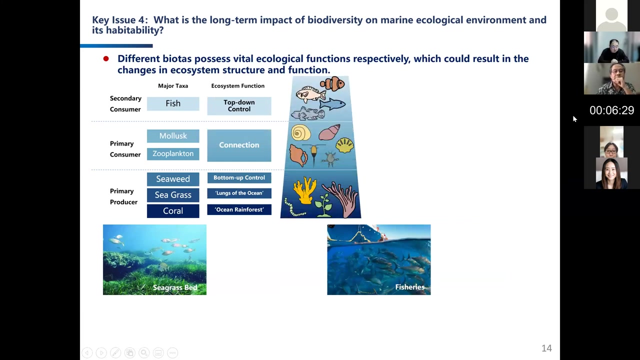 the coral reef ecosystem would possibly become the first disappearing ecosystem on the earth. so the coral biodiversity and the evolution mechanism of its ecological function still need further study, and the different biotas possess vital ecological functions respectively, and which could result in the changes of ecosystem structure and a function. 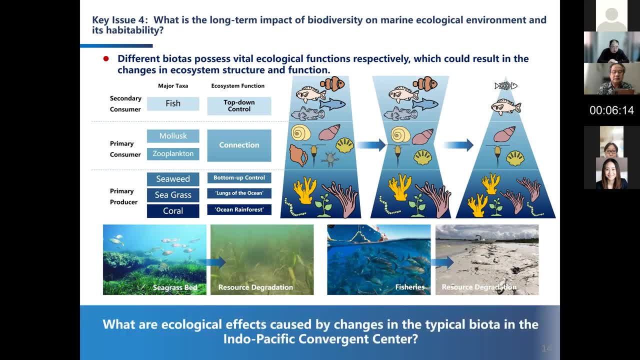 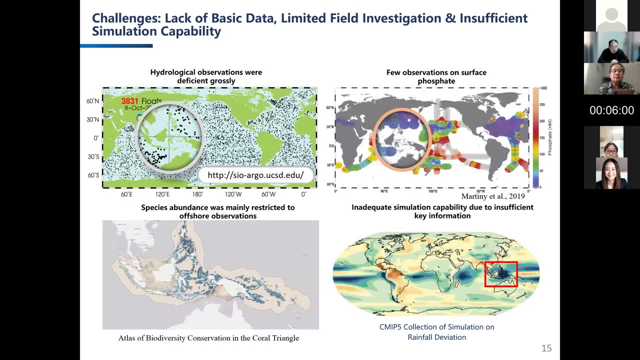 so what are the ecological effects caused by changes in the typical biota in this area? to address the above scientific questions, i would like to start with the first question. so one of the first questions is about the environmental impacts that the coral reef has. that is discussed in the network studies. 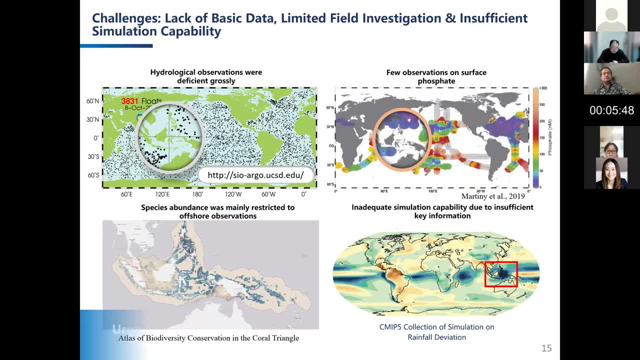 the coral reef has a huge amount of enormity. the coral reef is a very important natural resource and a very important Алексia, and we have to acknowledge that. coral reef is a very complex ecosystem. it has one of the largest marine ecosystems in the world. 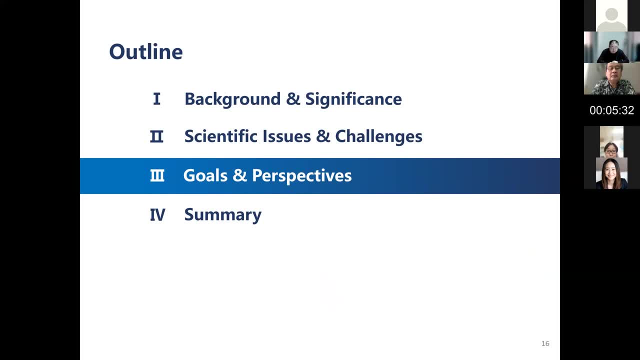 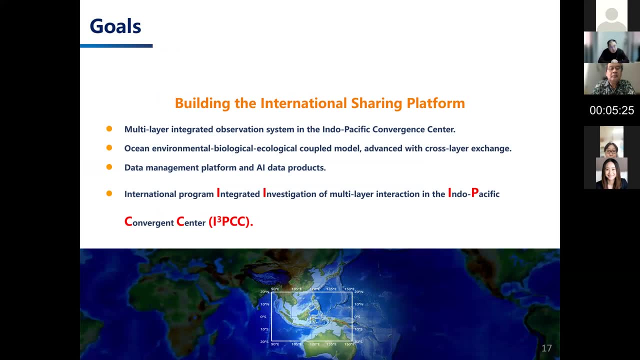 and it's based on three principles: perspective for future cooperation. and through the international cooperation we try to build the international sharing platform, including the multi-layer integrated observation system in this area: the ocean, environmental, biological, ecological, coupled model data management platform and artificial intelligent data products. and the international program, the triple ipcc. 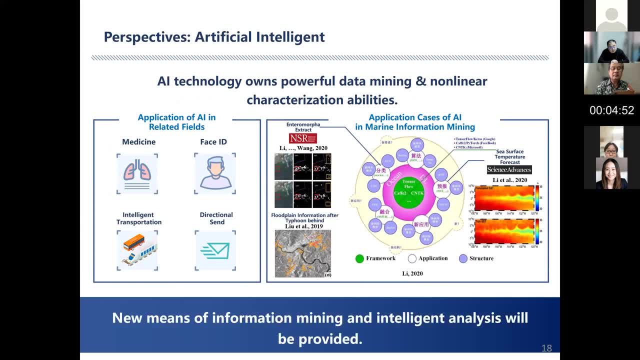 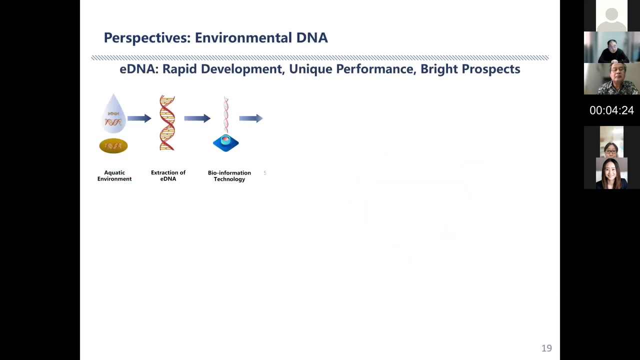 and we have some very potential solution for our future work. the first one is for artificial intelligence, which can offer the new means for information mining, intelligent analysis, because the ar technology owns powerful data mining and non-linear characterization abilities, and also the environmental dna is a very useful tool for us. 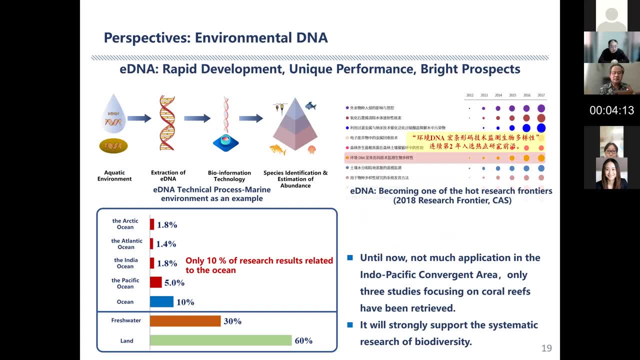 because it is rapidly developed in the past several years, with unique performance and bright prospect. however, there are only 10 percent of research results uh related to the ocean among the total environment science and up to now, only three paper focusing coral reef in this area have been achieved, so it will strongly support the systematic research of biodiversity. 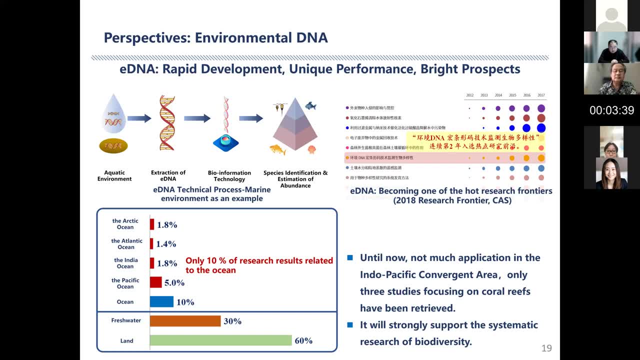 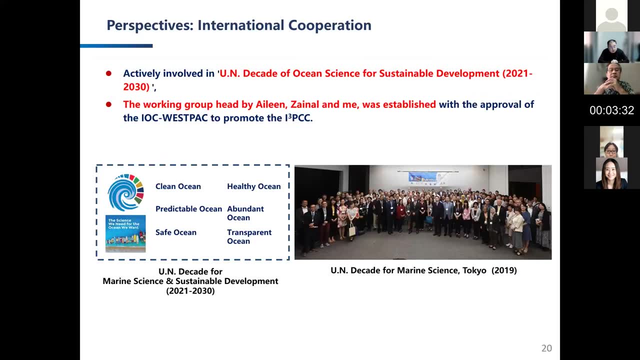 not only in this area but also in other oceans and seas. the most important thing is the international cooperation, the uh, some scientists actively involved in you in decades- of social science forces, cinema development, and a working group held by alien jana and me was established, established with approval of the ireland. 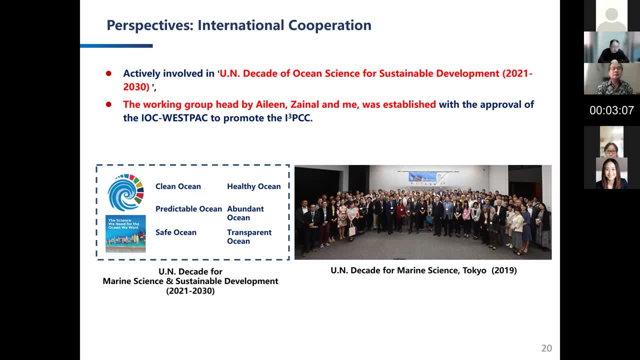 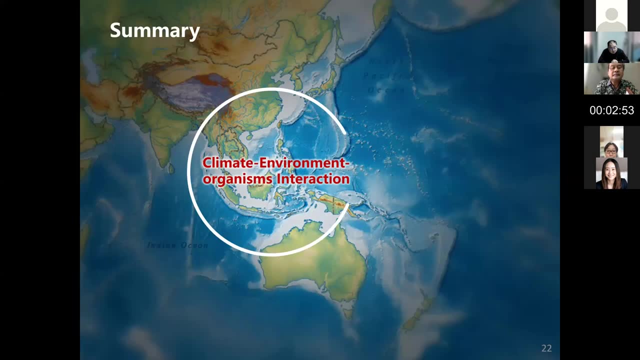 research and ecology team, and the project was conducted in the international cooperation, the Westpac, to promote the triple IPCC. So a new international program is on the horizon vividly. Finally, I will summarize my talk, Focusing on the climate, environment, organism interaction. 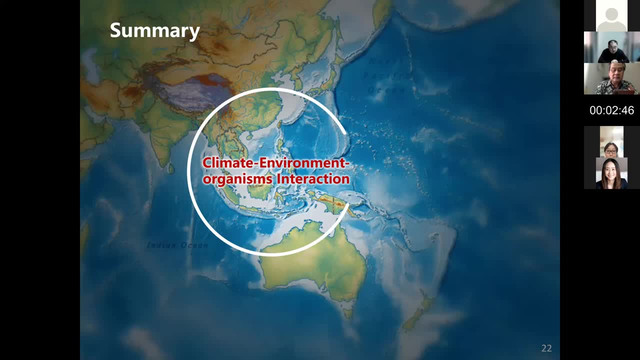 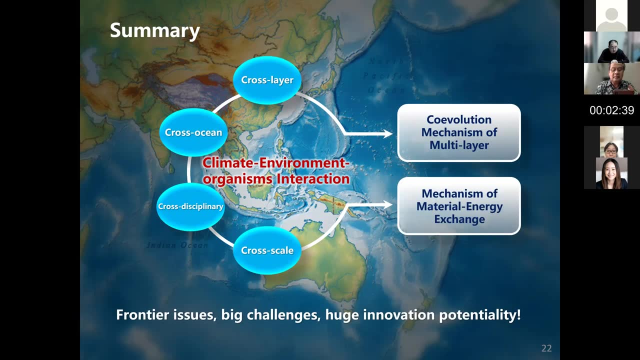 we will organize the international cooperative study through the cross layer, across ocean, cross disciplinary and cross skill study to understand co-evolution mechanism of multi-layer, especially the biodiversity center and the mechanism of material energy exchange among them. And this area has so many frontier issues, big challenges and huge innovation potential. 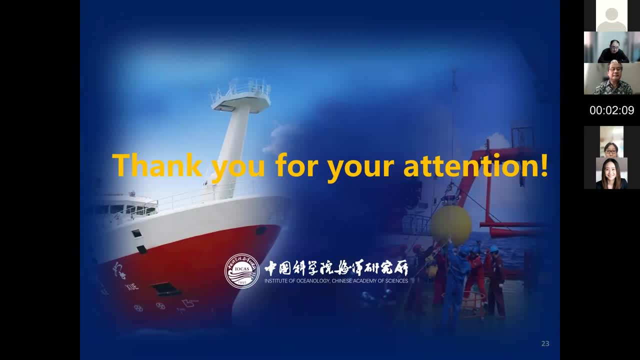 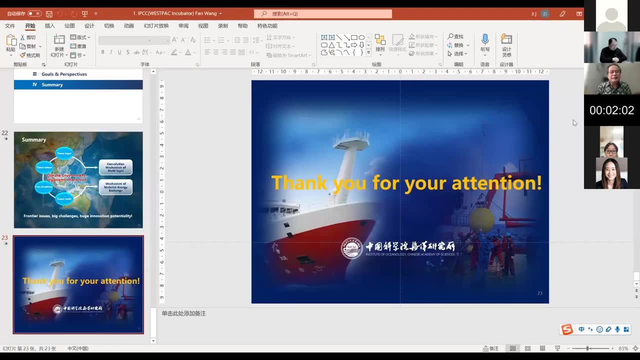 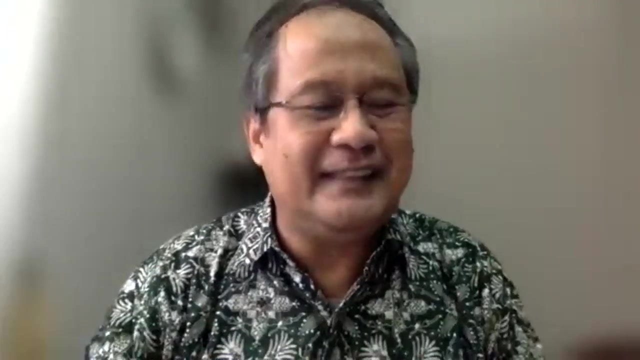 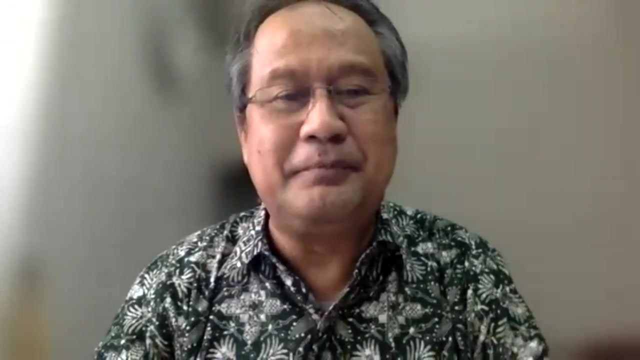 editing. So thank you for your attention and welcome to join us. Thank you, that's all. Thank you from Fan Wang for your presentation. I think it's a very exact time. yeah, So we still have around two minute time left, but for all of you. 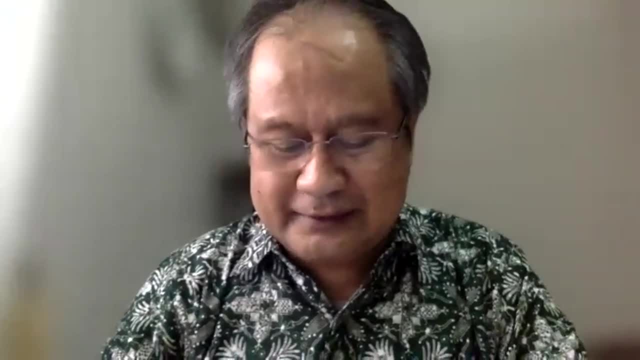 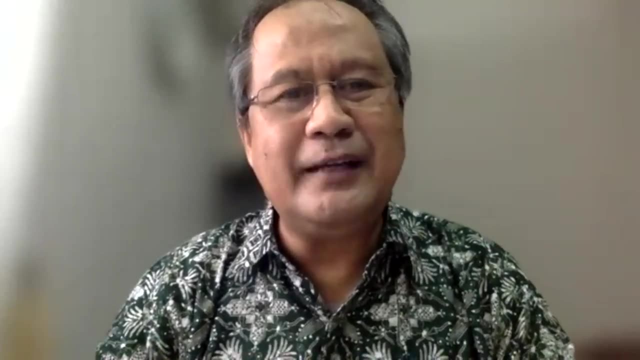 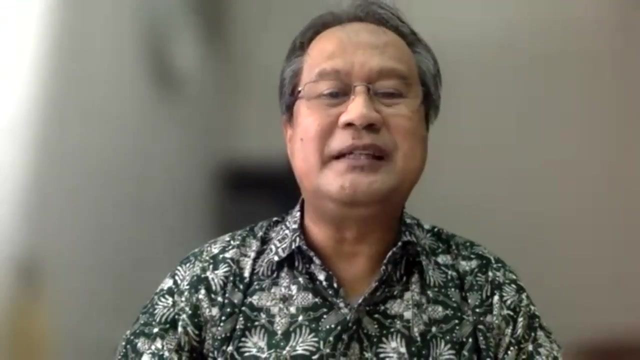 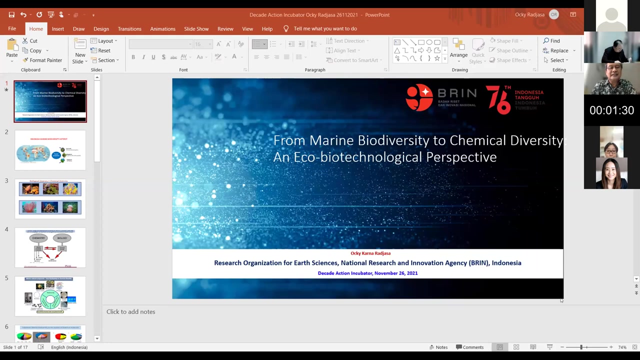 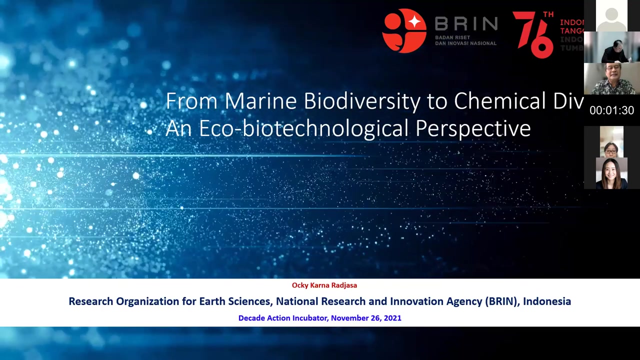 who have question. please hold on your question until the end of this discussion, So I will move to the next speaker. The next speaker is Professor Oki Karnarajasa. he is from Indonesia. He will talk on issue related with biodiversity. the title is on: from marine biodiversity to chemical biodiversity. 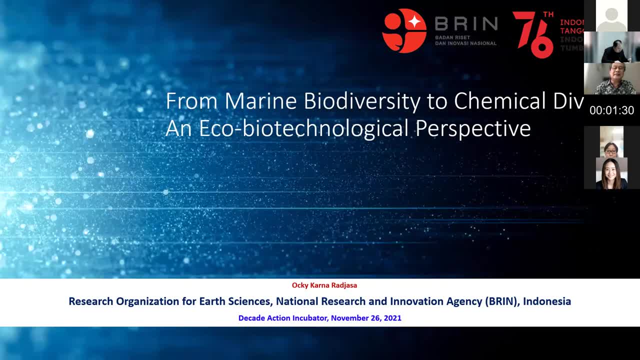 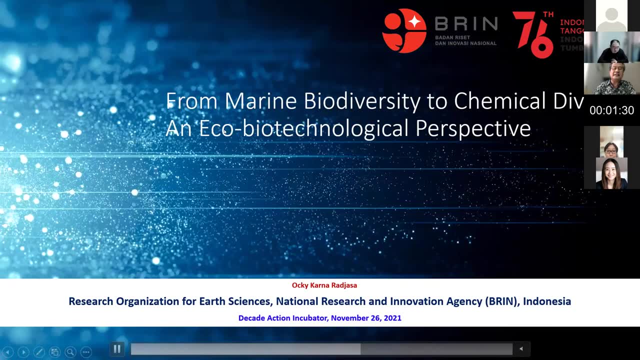 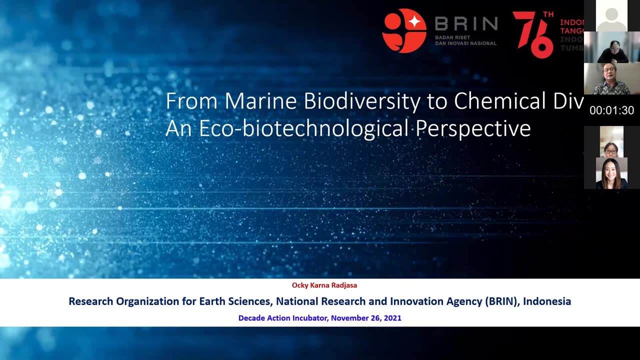 and eco and eco biotechnological perspective. professor oki is head of research organization of earth science at national research and innovation agency. it used to be indonesian institute of sciences, so his expertise is microbiology and biotechnology so he led paul research center currently. so we will have a 15 minute from oki to present your idea and 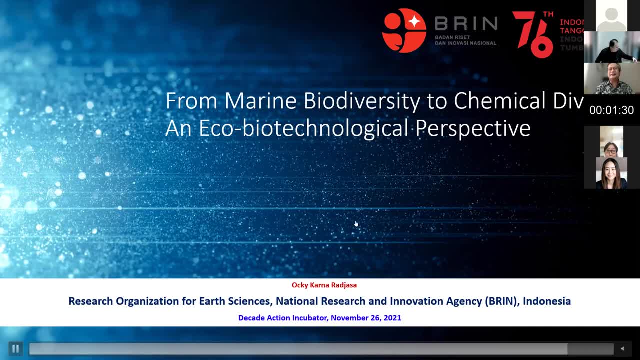 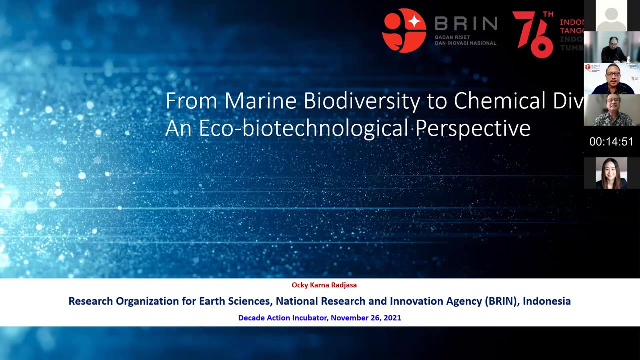 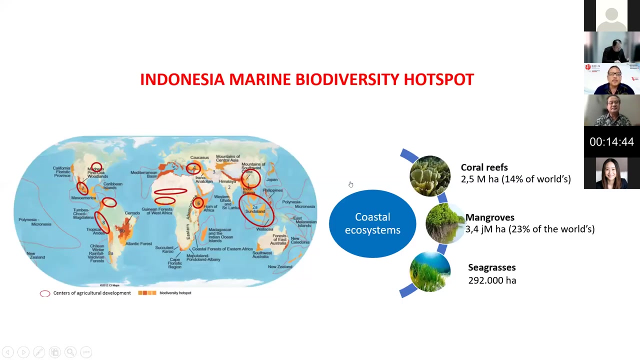 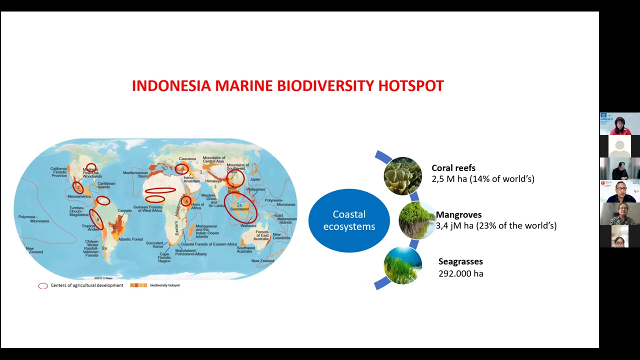 idea and solution for what professor fanwang stated earlier. please your time now, thank you. thank you, ladies and gentlemen. please allow me to briefly talk about from marine biodiversity to chemical diversity and eco biotechnological perspective. indonesia is regarded as the one of the mega biodiversity country and has been known as a. 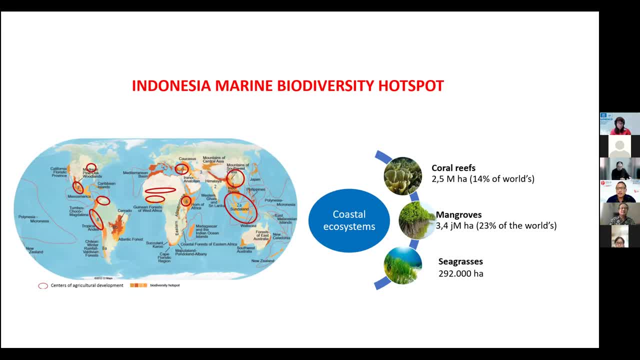 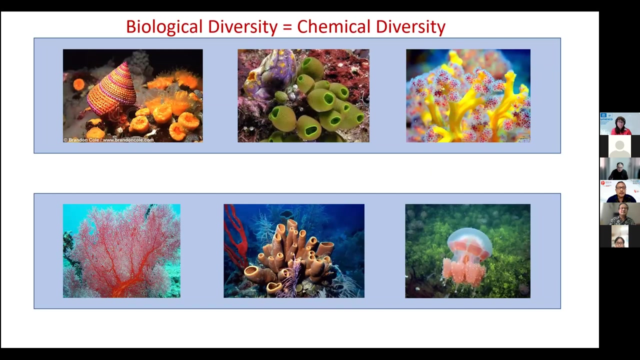 marine biodiversity hotspot. we are lucky enough to have a different, diverse coastal ecosystem, such as coral reef- representing 14 of the world's coral reef- and then mangrove- 23 percent- and also, as we all know, that biological diversity means chemical diversity. so by maintaining our biological diversity, basically, we will be able to also maintain our chemical diversity. 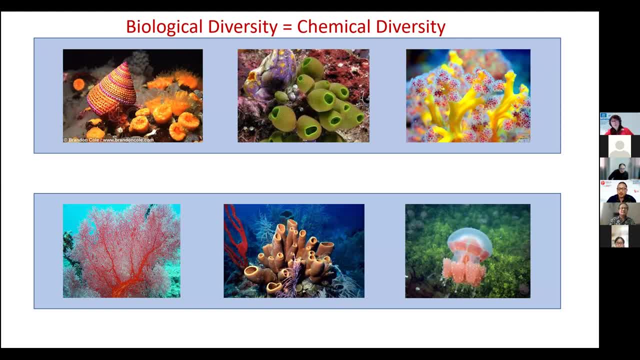 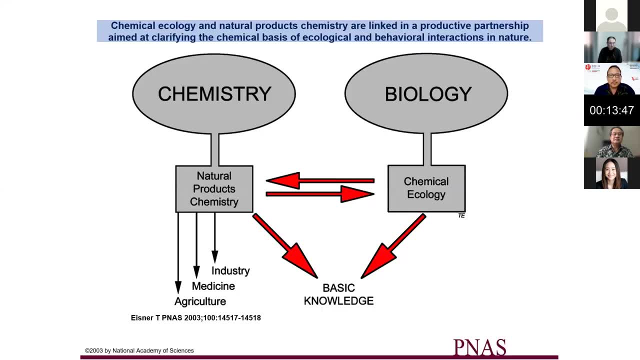 which is also important for us, especially to support our life as well our health. and when we talk about the development of a marine natural product chemistry especially, we need also to consider about the sense of biology, which is known as a marine chemical ecology. that means an interaction between 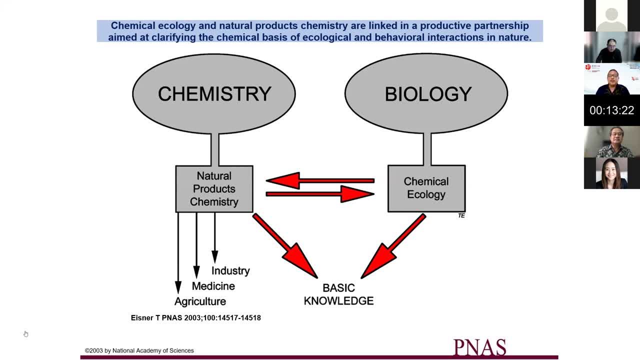 microorganism and environments through chemical interaction. that means there is no physical interaction in this matter. so i consider that this really chemical ecology is quite immature in our region and there is a need to strengthen our understanding on the marine chemical ecology to support our development on. 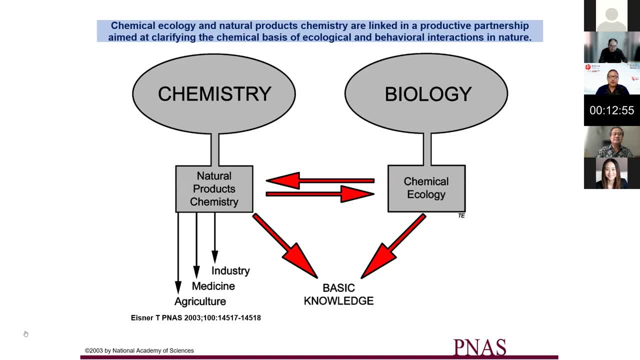 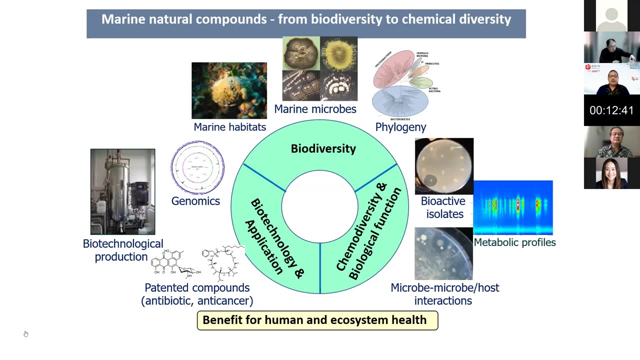 marine natural product chemistry that are useful for industry, medicine and agriculture, etc. so, basically, there is a need to strengthen our capacity on this matter. when we talk about marine natural product, especially from marine biodiversity, so we will talk about our benefits not only for human but also for ecosystem health. 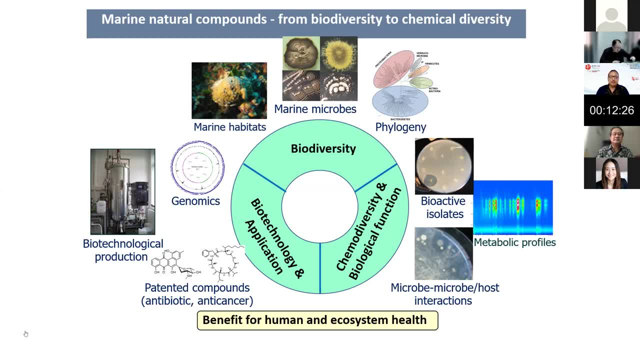 that means we have to maintain also our ecosystem for the future generation. there are at least three big themes regarding this topic. number one is a biodiversity itself- it could be from marine habitats or marine microbes or their phylogeny. and secondly is chemo diversity and 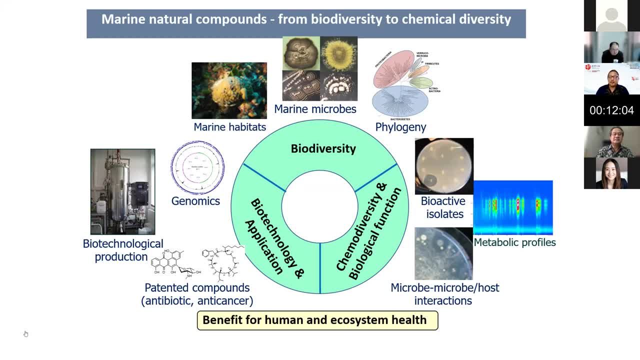 biological function. that is very much interesting for us in order to study some basic understanding how this active azure, for example, will produce certain products that are benefit for ourselves. the third one is a biotechnological and application. we can talk about the genomic biotechnological production as well as our products, such as. 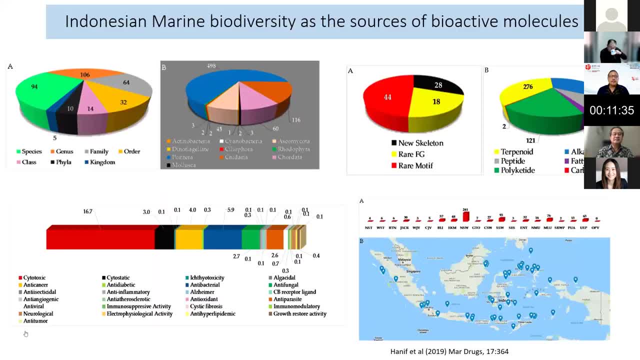 antibiotics and anti-cancer. this is an example of indonesian marine diversity as a bioactive compound has been reported. as you can see here, it's very diverse function from cytotoxic, anti-cancer, anti sucidicidal and then anti-tubor, cytostatic and then alzheimer antioxidant cystic. 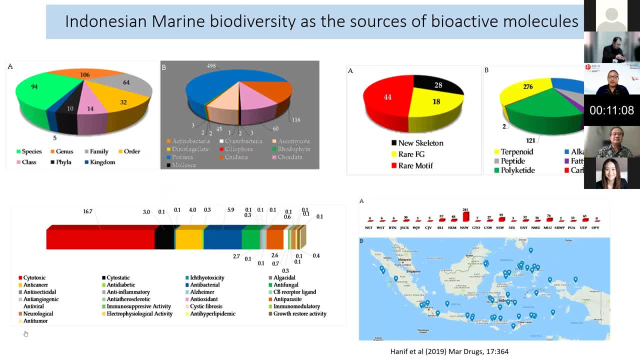 alga-cidal and antifungal, and you can see here from the map that most of our bioactive compound mostly come from the center and the eastern part of indonesia and it is very much related to the level of biodiversity in this region region especially in the central and eastern part of Indonesia. 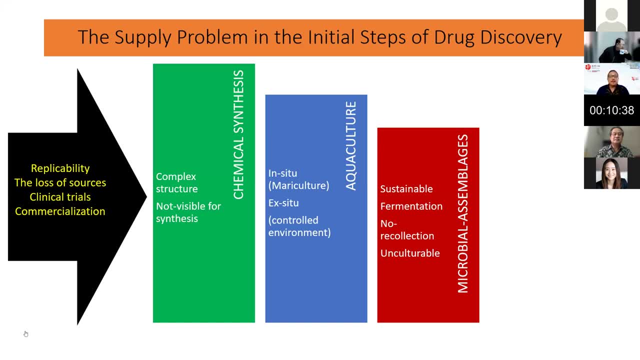 When we talk about the development of natural product, we talk also about the supply problem in the initial step of drug discovery. This is very much true, especially when we are talking about the preclinical as well as clinical trial for the commercialization. It is well understood that marine natural product is quite complex structure sometimes. 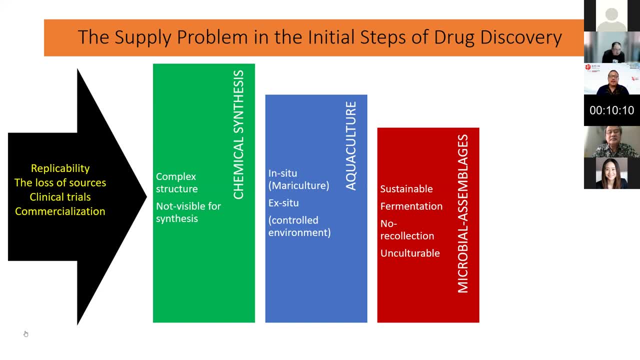 it is not feasible for the synthesis. On the other hand, our option on aquaculture, either in situ or ex situ, also sometimes support the growth of the producing organism, but the true bioactive compound do not produce. That's another challenge for the aquaculture. 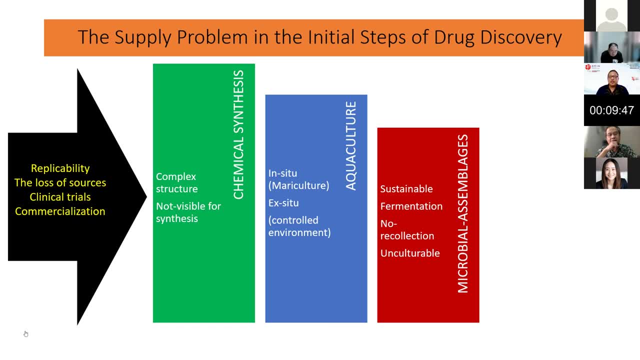 Lastly, is the development of marine microbiology or marine biotechnology, especially through the sustainable fermentation of microbes that are associated with the host organism. This will offer no recollection and possibility, but, on the other way, it also represents our difficulty In terms of culturing the marine microbes, because so far, based on our technique and 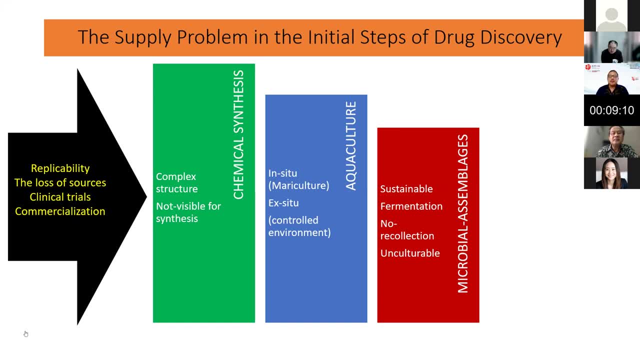 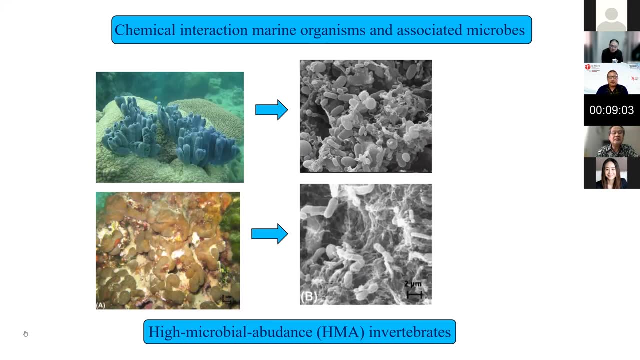 media, only 1% of the marine microbes has been successfully cultivated. Now there is another phenomena that represents chemical interaction between the host microorganism and their associated microbes, which is well known as microbial synthesis. So important is that these microbes are integrated into the natural extinction biome. 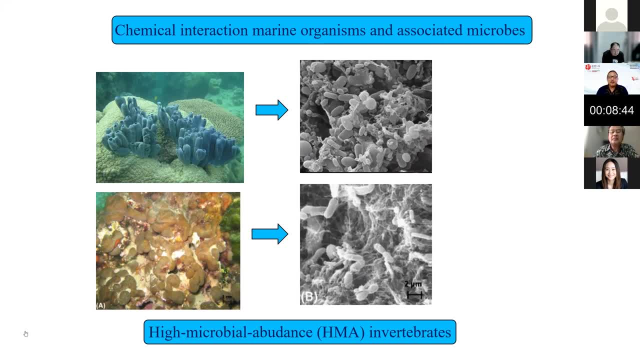 So in certain invertebrates we have what we call it high microbial abundance invertebrate. As you can see here, about 40 to 60 percent of their biomass are represented or occupied by their associated microbes. So by doing isolating and screening of this potential microbe we will be able to have 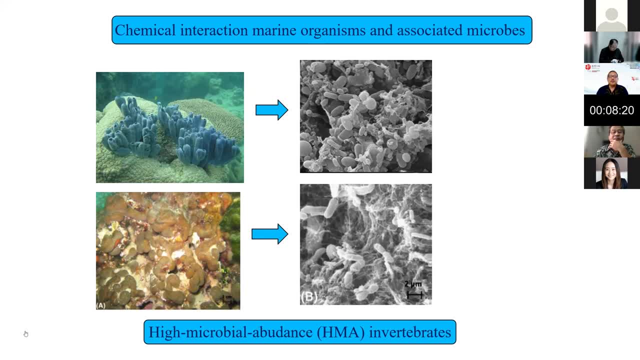 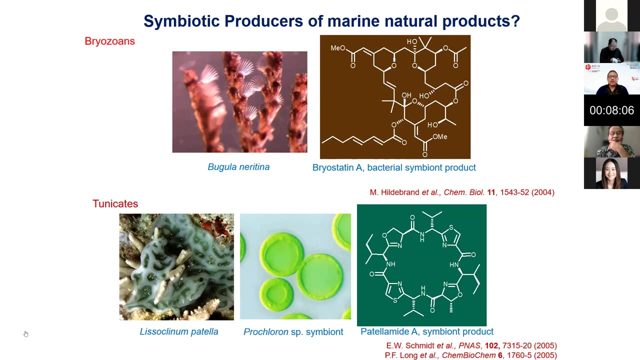 alternative mechanisms which are able to take the potential microbe and use it in for searching for the marine natural product from reef invertebrates, for example. The symbiotic microbes are the true of natural product. I can see you here, I can show you here, at least there are two accumulating evidences. 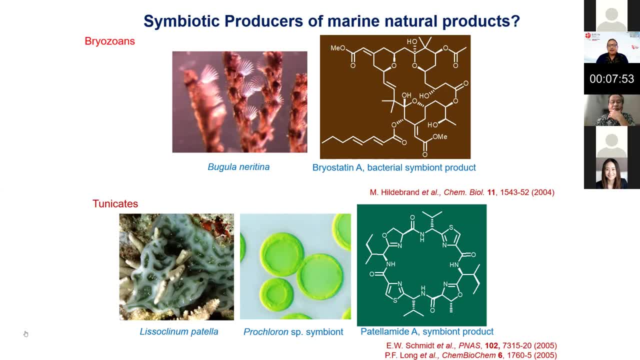 that, indicating that bacterial symbiont are the true producer of the natural product In this regard, Bugulan erythina that produce bryo-satin A. when their larvae treated by antibiotic, this Bugulan erythina was not able to produce the bryo-satin A. 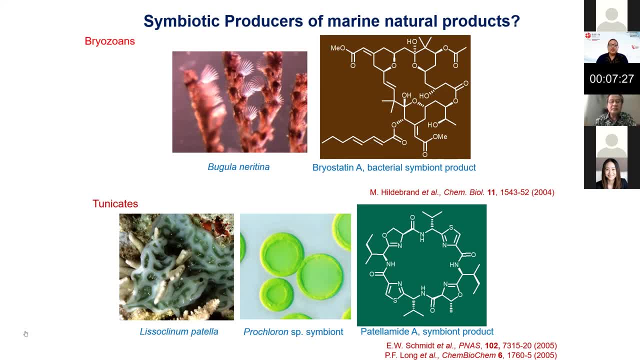 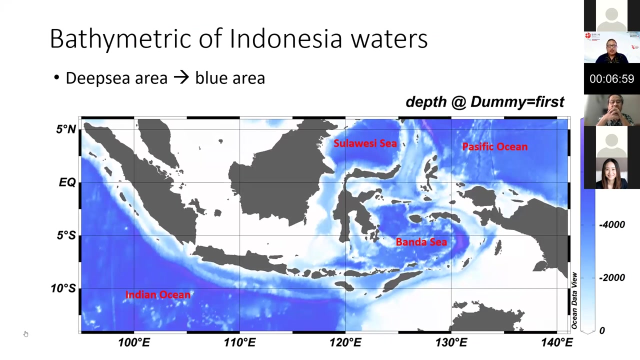 So there is an independent interaction between the bacterial symbiont and our host microorganism. Of course, this will represent another challenge for marine chemical ecology, especially for clarifying how this microbe and their host microorganism are interacting. Indonesia. 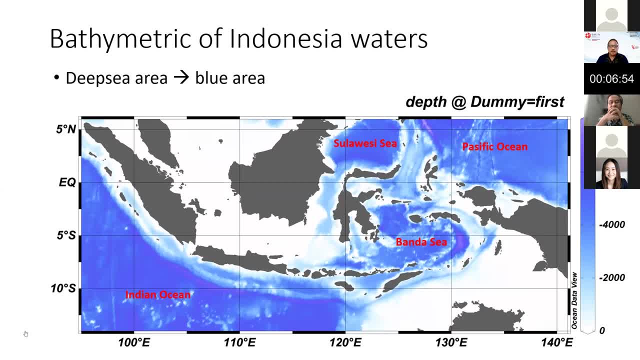 besides having such very productive coastal ecosystem, indeed, we have several deep sea water. as you can see here from Bandar Sea area, it has the deepest part, up to 7,700 meters. That means this represents another untouched biodiversity from the deep sea environment. 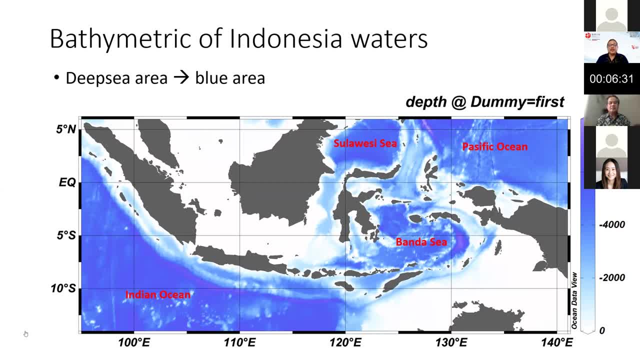 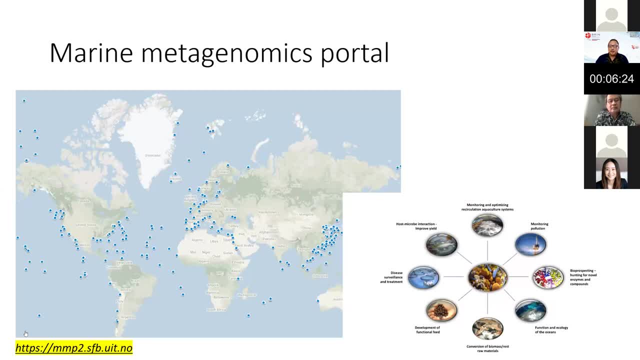 And we have some difficulties, of course, for collecting and isolating the microbe or macrobe, but there is. there is another study that representing the potential, as mentioned by Professor Wang, the study of environmental pool DNA, especially by using the marine metagenomic. 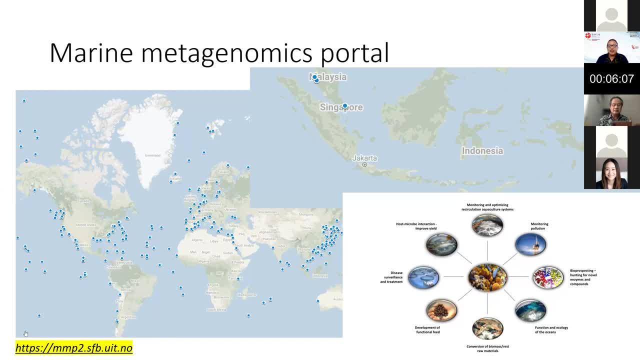 as you can see here, there is no single dot representing the study of metagenomic marine metagenomic from Indonesia, despite the fact that there is an increase on the use of metagenomic. This portal is was online in 2017,. 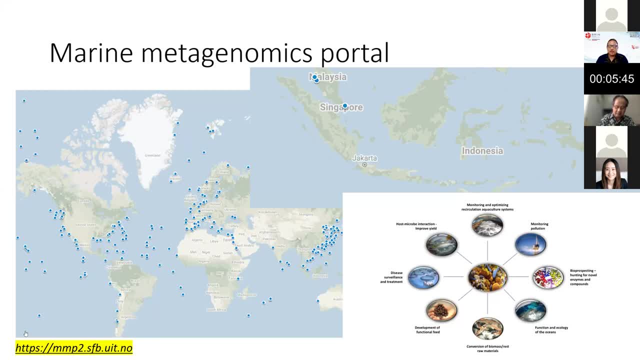 until now and maintained by the Center for Bioinformatics the Arctic University of Norway. And you can see here there are several use of metagenomic study, especially for a range of scientific and industry application, from monitoring pollution and recycling water system. 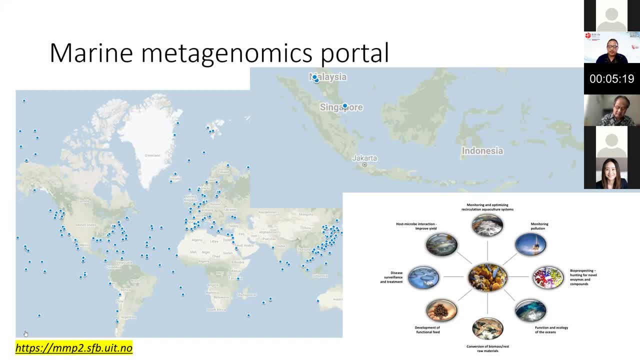 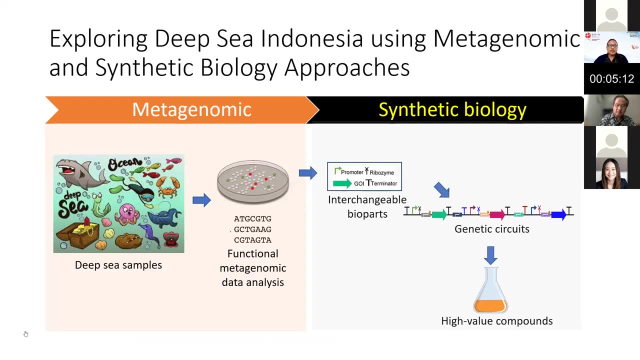 bioprospecting and also disease surveillance and development of functional feed for aquaculture. Now there is a possibility to explore deep sea Indonesia using metagenomic and synthetic biology approach. So basically, our study here will depend on the functional metagenomic data from the environmental pool DNA. 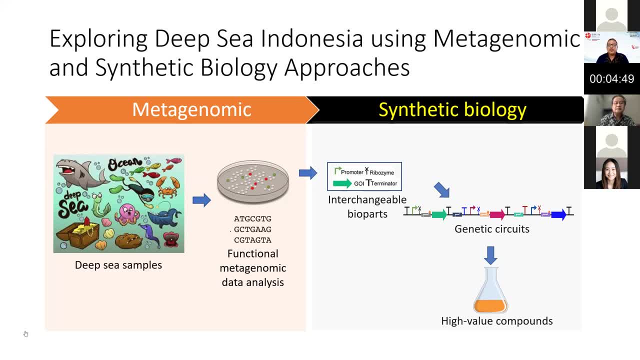 and we use synthetic biology, which is very much really on biopart, a sequence of DNA that represent functionalities of certain function. So in this regard we can use different part of uh gene from functional metagenomic data to establish and to construct certain interchangeable biopart. 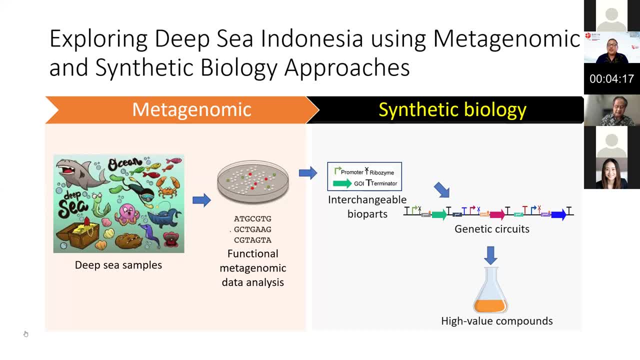 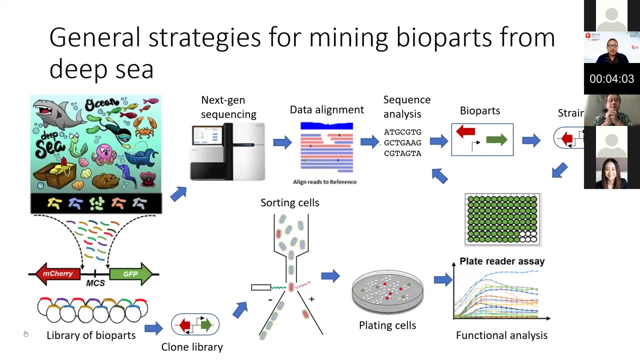 in order to build up a genetic circuit based on different biopart from metagenomic study, so that it can be used to produce a high value compound And for general strategies for mining biopart from deep sea at least, we can use two different approach. 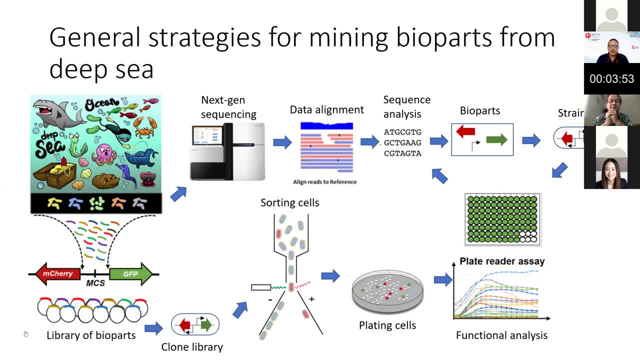 Number one is the whole genome. shotgun sequencing is performed uh for environmental pool DNA sample for gene and species discovery, And secondly, we can uh chop. the DNA fragment then will be cloned with plasmid which has green and red fluorescent protein. 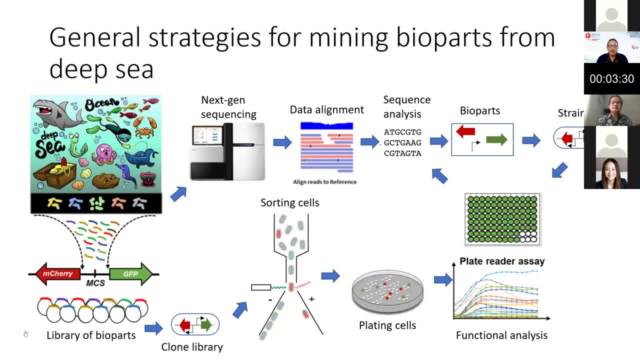 Then it will transform into equal life. So basically we will be able to screening the equal line and then, using cell sorter and potential colony can be uh further analysis and pick up to be compared with the uh security that we open from. 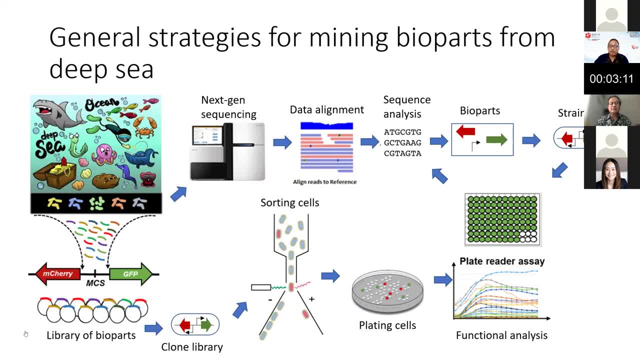 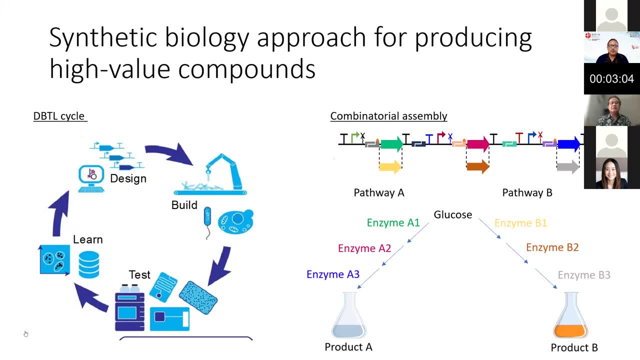 uh ultimum sequencing Synthetic biology approach for uh high value component, especially from marine and deep sea, can also be conducted by uh dbt cycle, which mean design will test and uh learn cycle to obtain the base assembly to express in the pathway and produce. 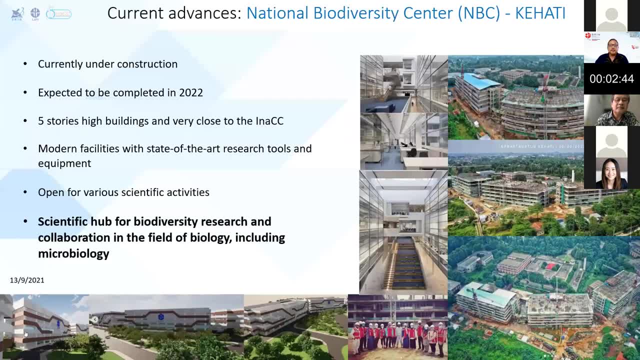 desired product in different, And we are now at the uh national research and innovation agency. Currently, we are also uh uh constructing new building for uh facilities. regarding the biodiversity, that can be used as a scientific hub for biodiversity research and collaboration in the field of biology. 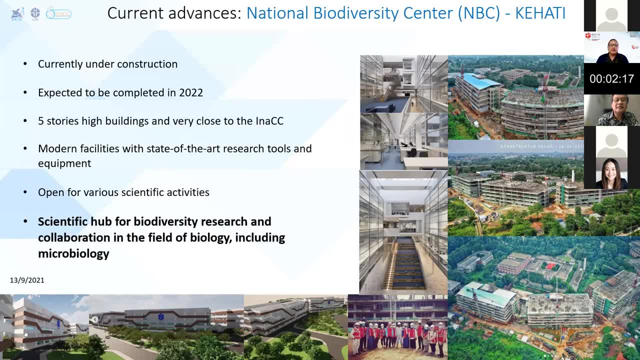 including uh my marine microbiology, So hopefully by 2020, we will be able to complete. So, as mentioned by professor Wong, we are also uh launching uh global platform, including for biodiversity, So hopefully this will also. 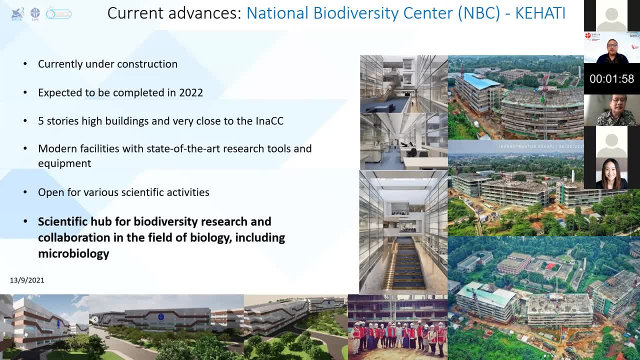 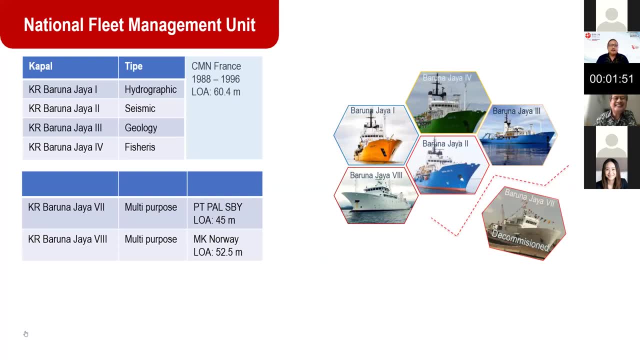 uh allow our international partner to be able to join our initiative. Two minutes more. Yeah, this is the final slide. We are also uh just constructed national fleet management unit that will also uh support our marine and deep sea research. 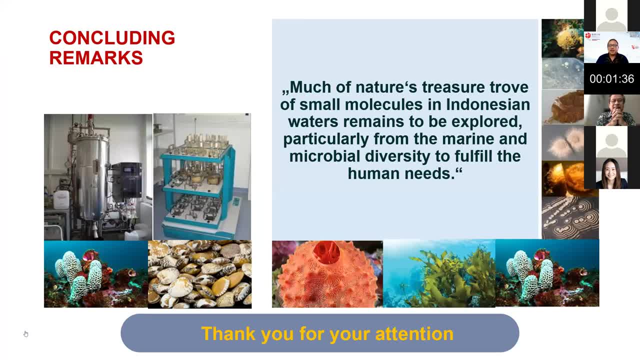 And, as concluding remark, much of nature treasure trove of small molecule in inhibition water. they meant to be explore, particularly from rain, and microbial diversity to fulfill the human needs. Thank you very much for your kind attention. Uh, thank you. 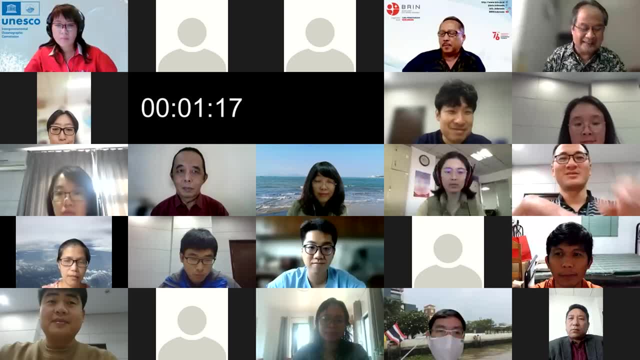 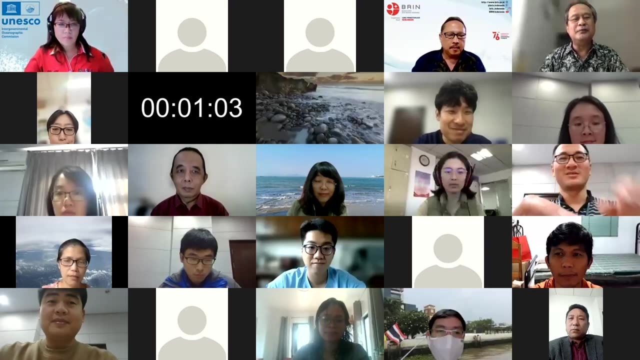 uh provoking Uh, it's uh an excellent uh talk, I think- uh uh presenting uh eco biotechnology perspective. So we move to Malaysia now, So we will invite a professor, Eileen Tan. 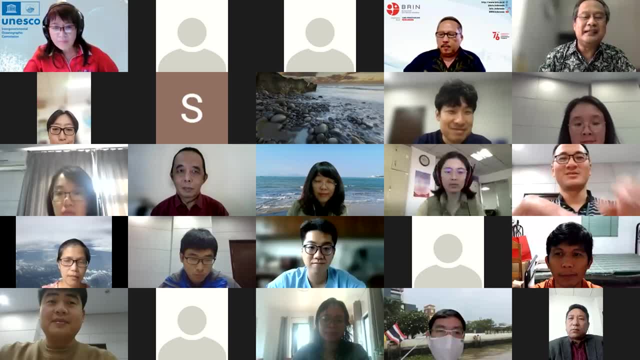 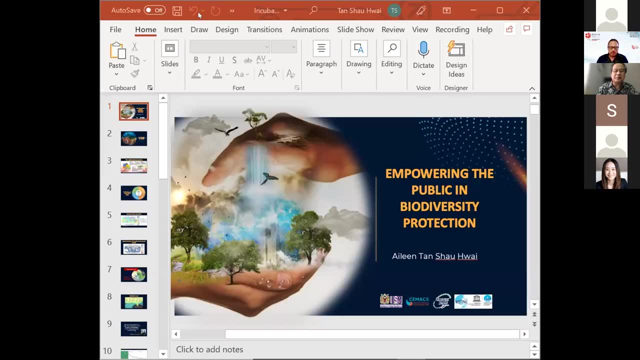 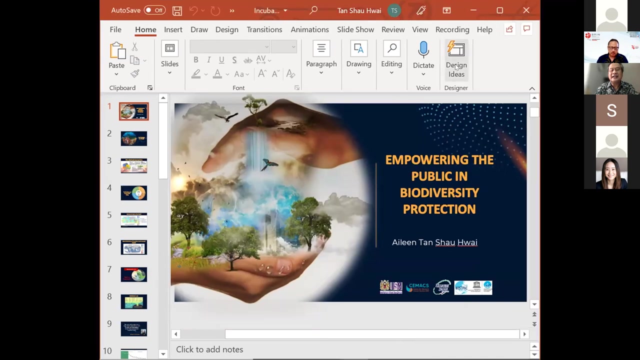 Uh she will present topic on empowering the public in biodiversity protection. Uh, Professor Eileen uh Tan is uh uh director of center for Marine and coastal studies uh at the University Science Malaysia. So his research uh. 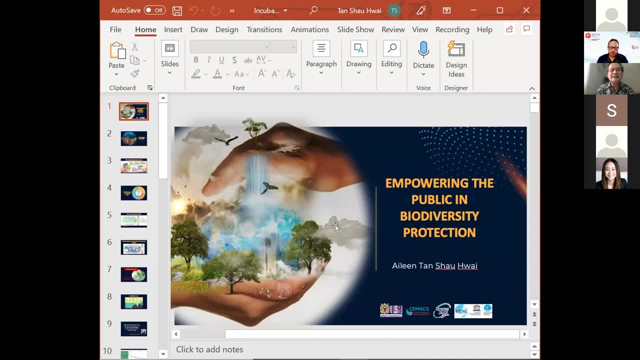 her research interest is on issue related with marine biodiversity, aquaculture and uh also related with the human uh activities. So, Professor Eileen, uh, you have a 50 minutes presentation. Uh, please, uh. 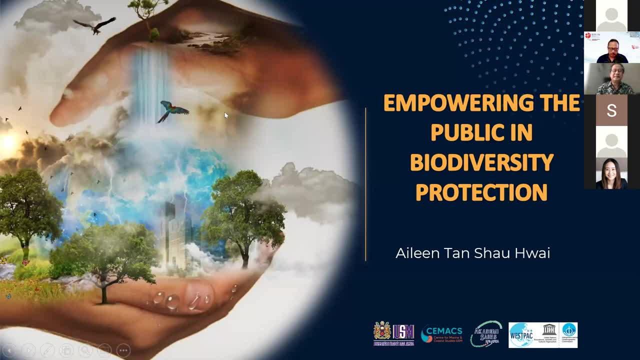 floor is yours. Thank you, Uh, thank you Uh. can you see my slides now? Yes, indeed, Okay, Thank you very much. Yeah, Good morning and good day to all Uh the uh, ladies and gentlemen. 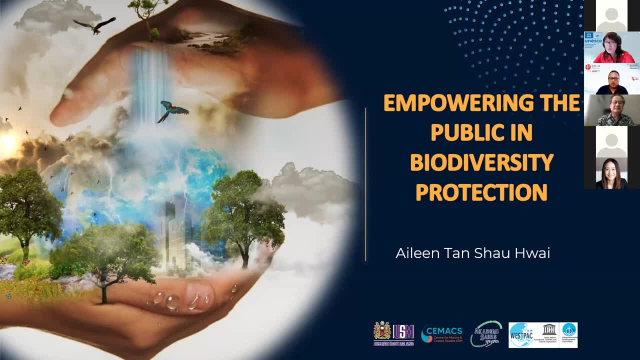 wherever you are. Um, we're having today. uh, this morning would be slightly different from what been shared by professor, from one and prof. Okay, This is very much science-based talking about the, the whole, uh, triple I, PCC and also on chemistry. 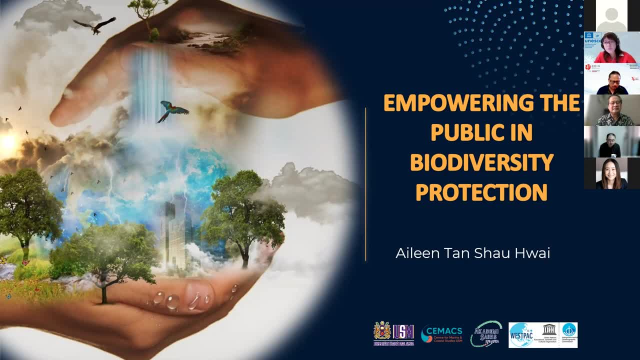 biodiversity. Mine is more on how do we actually involve the public in biodiversity protection? Um so, uh, I think, uh, in the last decade of the 20th century, what's the first time? a sense of urgency about the global scale? 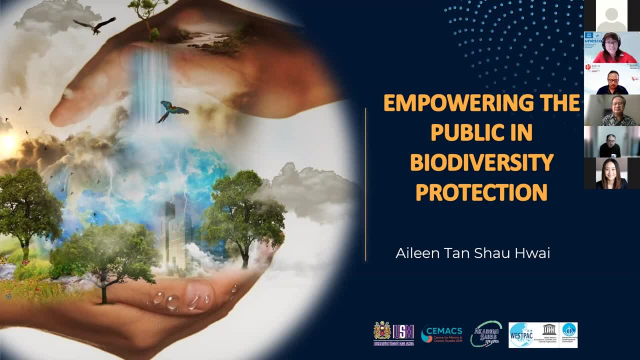 degradation of natural habitats and the resultant threats, uh, to potentially millions of species. government nice effort to both study and conserve was at race. The obvious question is: why has a massive international effort to deal with the biodiversity crisis crisis still fail to launch? you know why is it still fail to launch? you know, are the scientists. 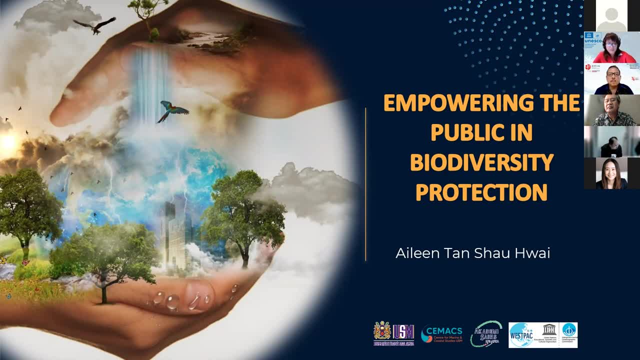 not doing enough or the government not doing enough. the power of people is well demonstrated as a primary force to protect our biodiversity. the power of the people. but how do we translate all the science that has been generated in the institution, in the higher learning institution, to the public for their understanding and to get them involved in playing a role? 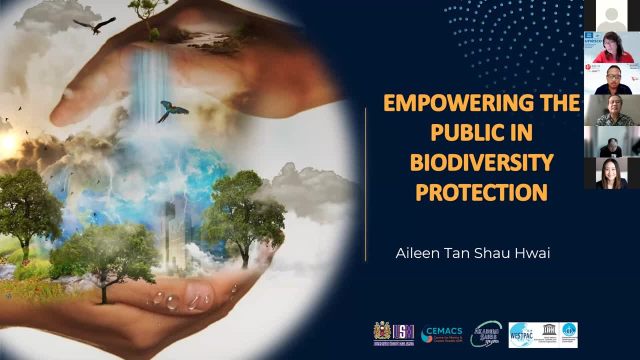 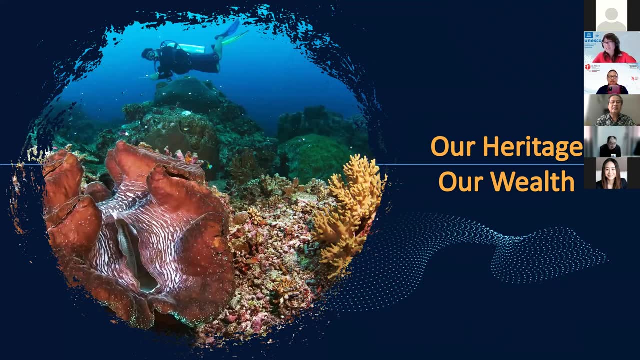 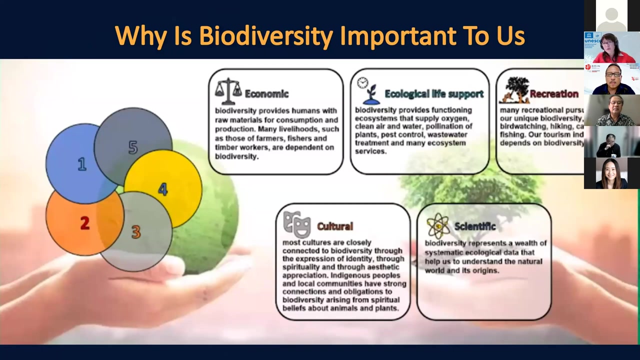 in in biodiversity protection. when we talk about richness, many would think about dollar and cents, without much focus on our vast ocean heritage and translating our ocean heritage to our wealth. what is biodiversity important to us? you know, um uh i i. i know most of us would already know, because we are all from. 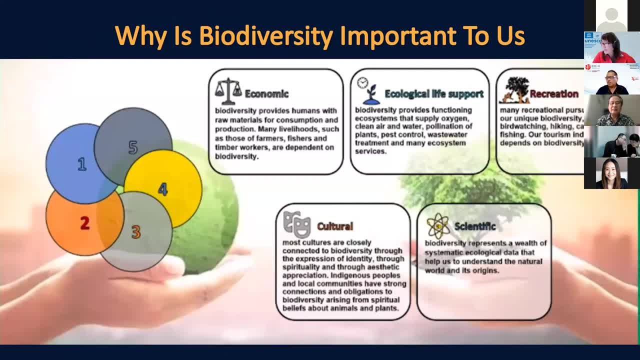 the scientific background. i'm trying to bring this matter out for the benefit of those who are not from the scientific background. you know, biodiversity provides to our economy, provides life, ecological support, supports recreation, cultural and scientific needs. biodiversity represents a wealth of systematic data that helps us to understand the natural world and its origin. this, this importance, this fact is well known to us, but this is not well known to the general public, especially to the communities themselves. 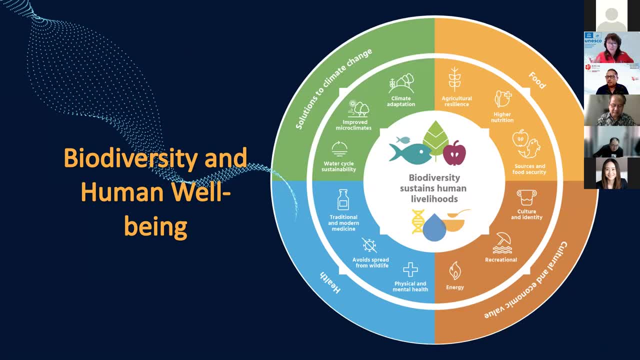 so biodiversity not only supports, giving us the advantage that's been shared earlier, but it actually supports our economies and enhances our well-being, the human well-being, and has the potential to do even more. the five main roles of biodiversity to human well-being: you know some of it has been shared by uh prof oki earlier on. biodiversity ensures health and food security. 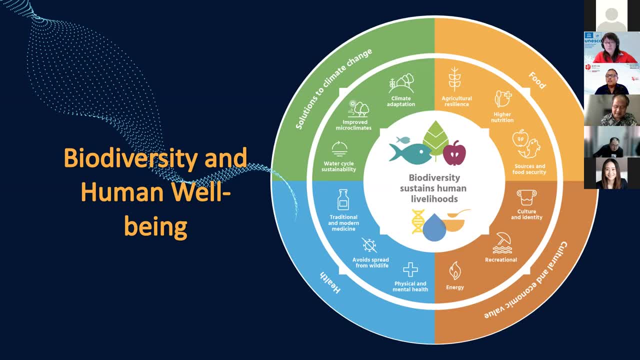 like what we are moving to forward now with the blue food agenda. and biodiversity helps fight diseases, like, for example, the pharmaceutical pharmaceutical products. biodiversity benefits business- businesses, for example, food, seafood and tourism- and biodiversity provides livelihood- the, for example, value from ecosystem services. and biodiversity protects us, such as nature-based solutions that buffer us from natural. 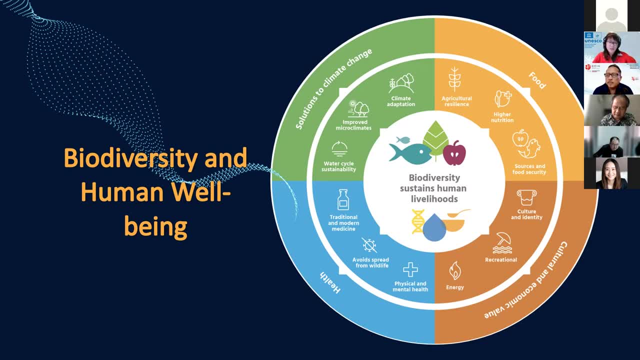 disaster, such as floods and storms. as ecosystems are increasingly threatened by human activity, acknowledging the benefits of biodiversity is the first step in ensuring that we look after it. we know biodiversity matters now. as a society, we should provide, protect it and, in doing so, protect our own long-term interests. this slide shows the global distribution of cumulative. 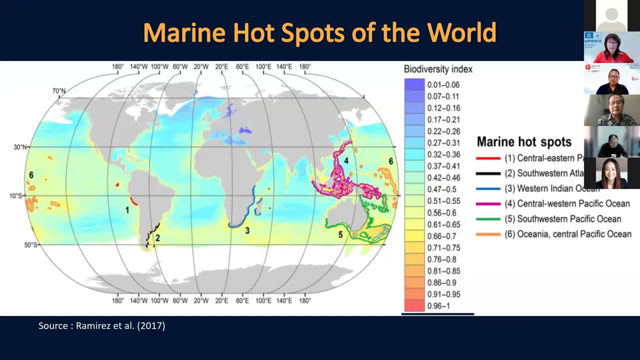 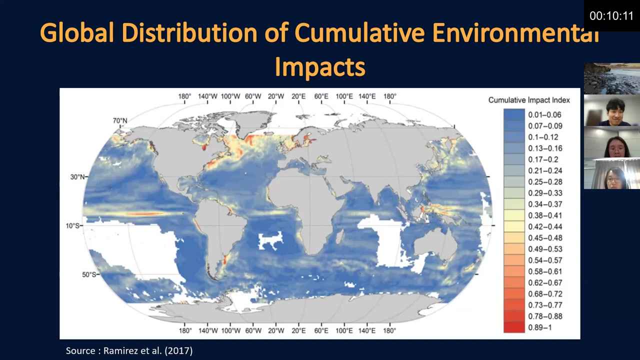 environmental impacts. um, no, no, sorry. these slides show the marine hot spots of the world, with the highest marine biodiversity hotspot concentrating at the western pacific region. similar style has been shown, also has been shared by professor fang wang earlier, but you compare with this slide. this slide shows the global distribution of cumulative environmental impacts, with highlights. 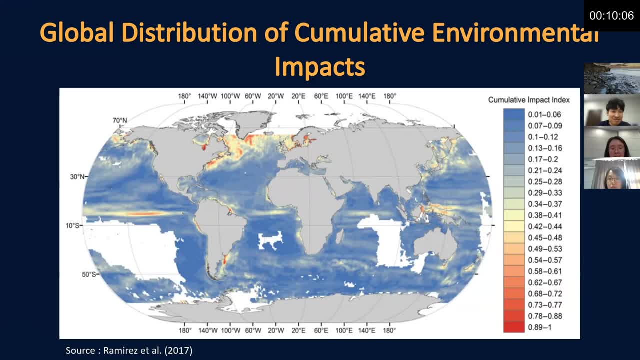 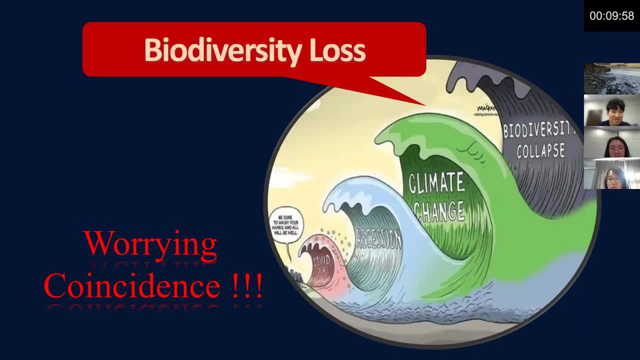 of high cumulative impact index, also around the western pacific region. this is indeed a worrying coincidence due to the biodiversity loss, added impacts from climate change and anthropogenic factors. you know we are rich and yet you know this area, the western pacific area, is also subject to. 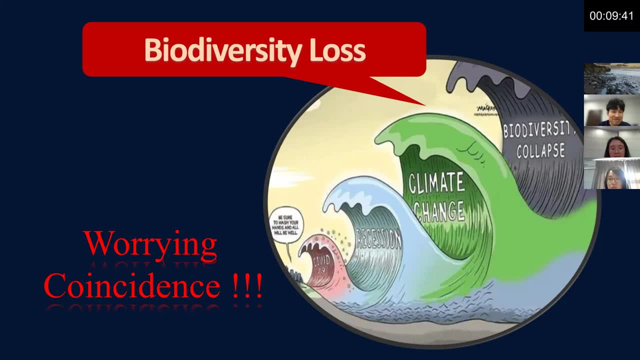 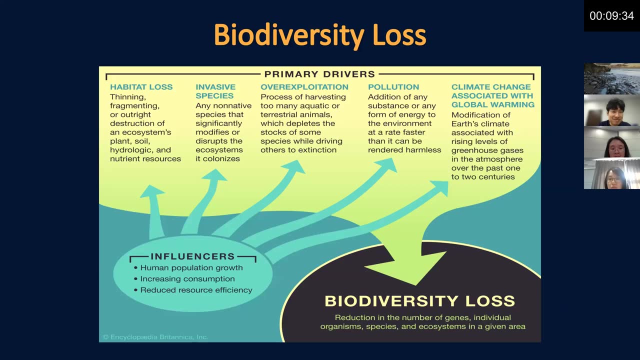 very high impact of of our stresses. but biodiversity is critically important to our health, to our safety and probably to our business or livelihood. but biodiversity the bike. the diversity within species, between species of an ecosystem, is declining globally faster than any other time in human history. this slide shows the primary drivers of biodiversity loss, which includes: 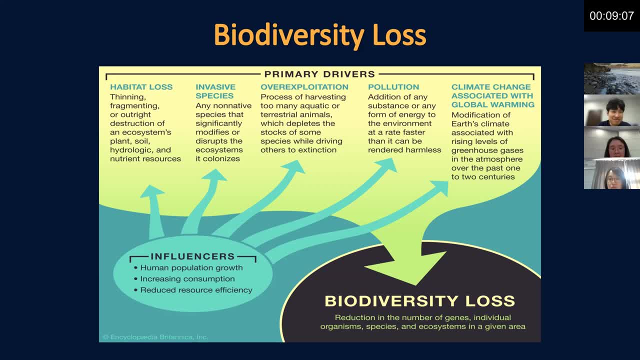 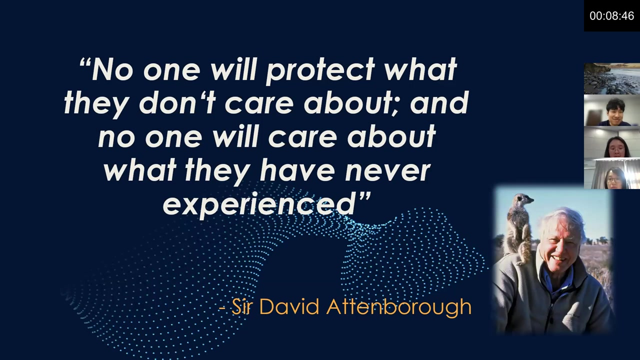 habitat loss, invasive species over exploitation, pollution and climate change associated with global warming. the influencer are human population growth. you know human population growth are increasing rapidly, also increasing consumption and reduce resource efficiency. to engage people in environmental issues such as the biodiversity crisis, one has to inspire a connection with nature. that linkage should be built from a clear and 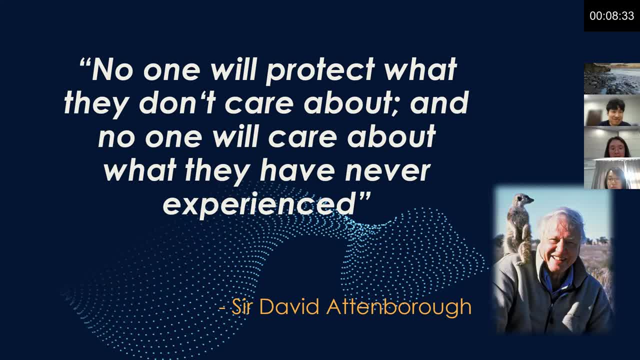 compelling message about the importance of biodiversity and what we risk in depleting it. sir david attenborough, the famous naturalist, has quoted: no one will protect what they don't care about and no one will care about what they don't they have never experienced. this is very important for us to 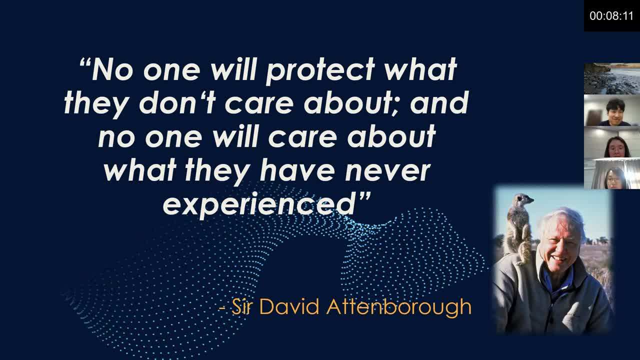 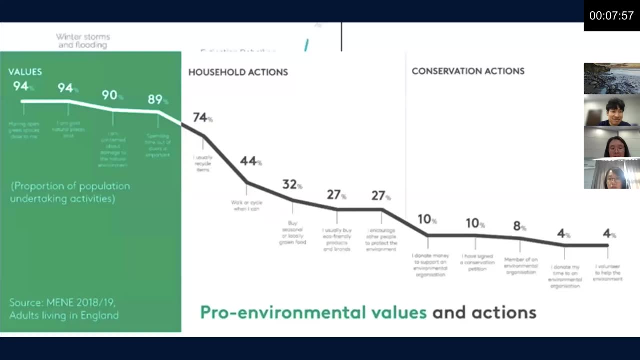 to keep in mind, because when we talk to the community, this is something we must understand. at the moment, the community do not really understand what is biodiversity is all about. in a study done by monitor of engagement with the natural environment, uh, in year 2018 and 2019, yeah, the survey found that around 90 of the adults in 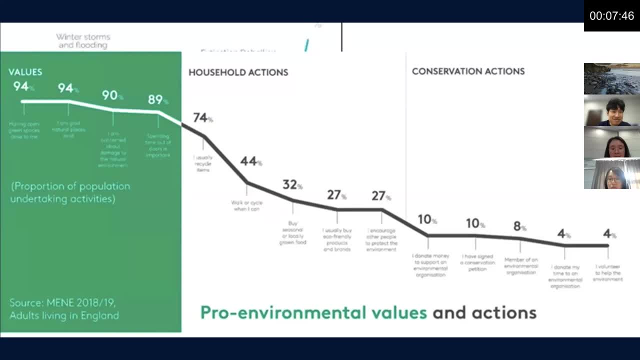 uk. we have not done such study in our region, so i'm i'm using the, the template, the, the example from uk. the adults in uk do do understand and concern about the natural environment. if you look at this, you know when, when it comes to natural disaster, they do have actions they do have. 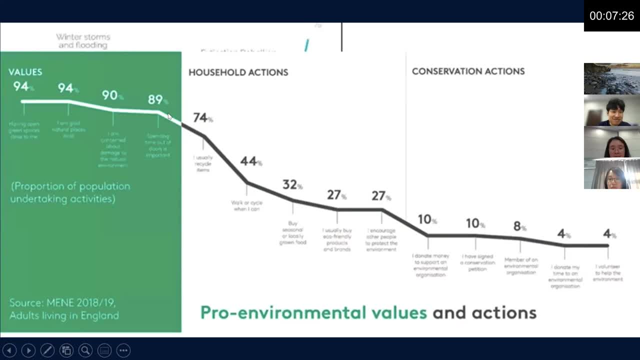 activities, but when, as it goes, the understanding is there. the knowledge is there as it goes to how much being contributed by households actions. you can see a drastic drop from 74, which is involving cycling. you know our community also understand and introduce the the carbon image emission. they 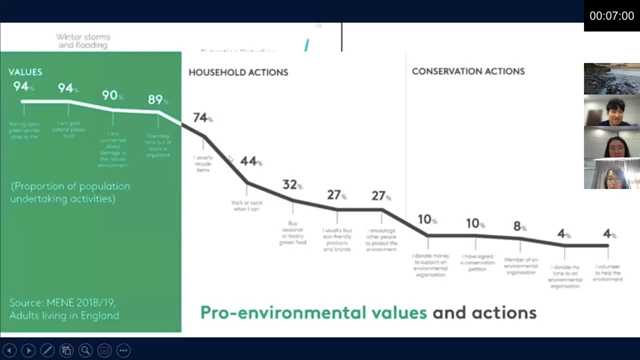 do cycles, the population do, the community do cycle around. but when it comes to more other things- you know more other things, which is expecting the, the, each household to take action, it actually drops when, when we look at it, into conservation action, into volunteering, into actual practice. it 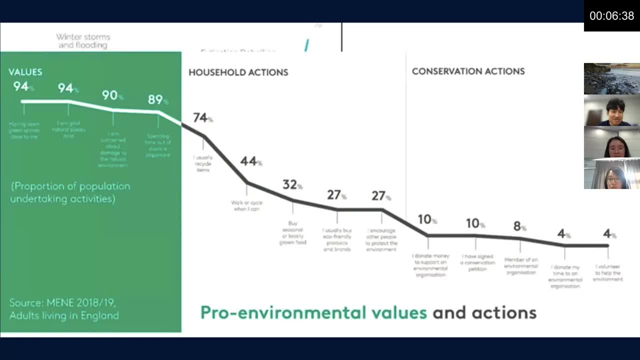 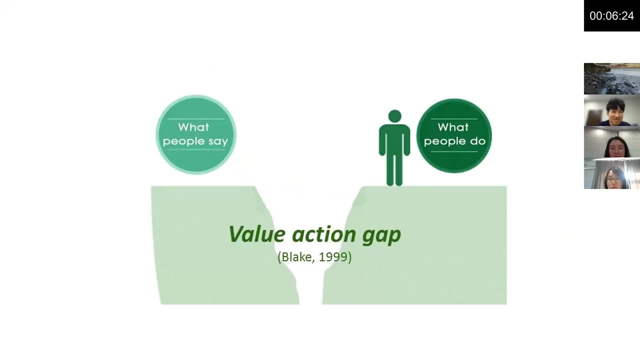 actually only goes down to four percent. who is actually, you know, in the general public, who is actually involving in conservation action? this is this is a reflection. this is a Reflection of the value action gap, showing the gap between what people say and what people do. 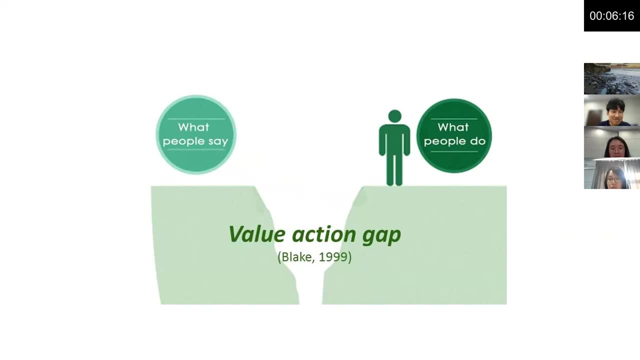 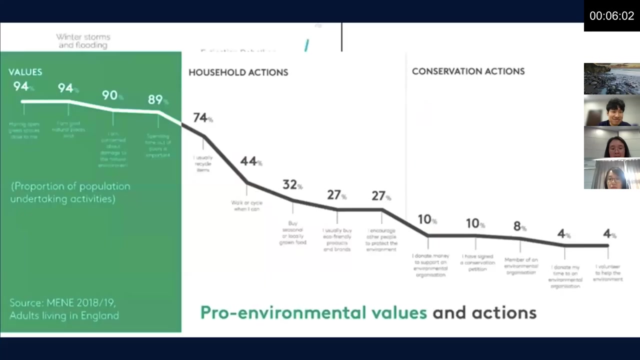 Many of us are very good in saying things we know and we explain it, But how many of us, you know, really go down to the ground and do what we believe in and what we understand? Now, that is a huge gap. you know from the earlier slides. 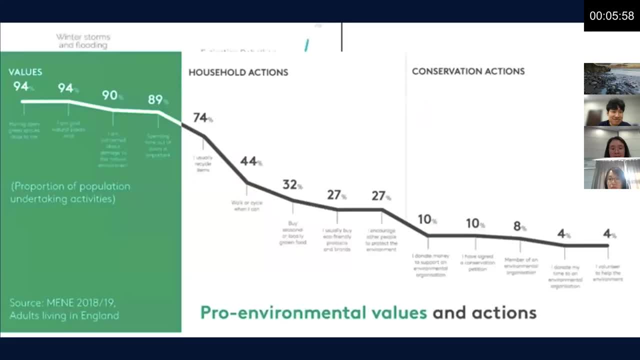 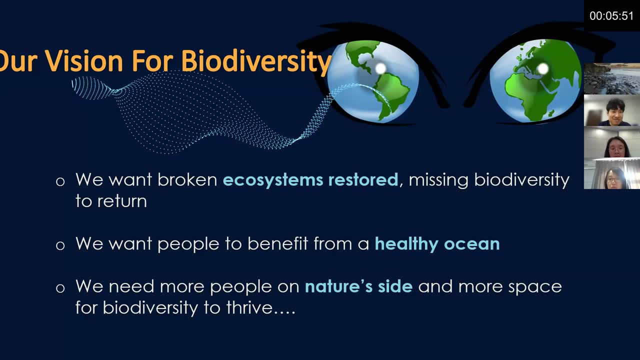 from 94% to really action is only 4%. So what is our vision for biodiversity? You know, we want broken ecosystems to be restored, Missing biodiversity to be returned, We want people to benefit from a healthy ocean And, most of all, we want more people on the nature's side. 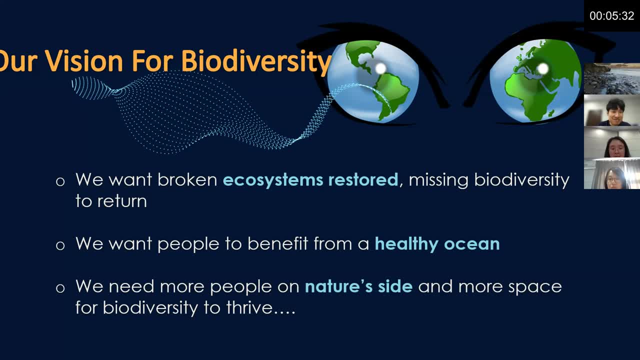 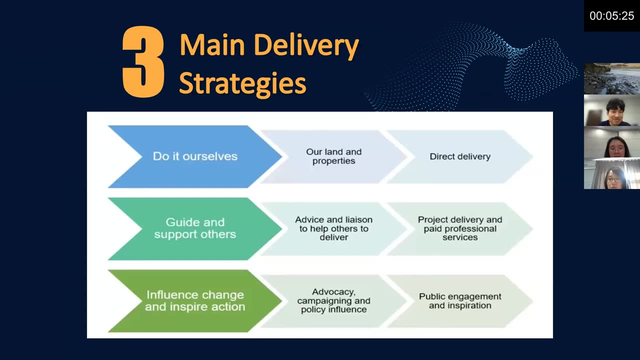 and more space for biodiversity to thrive. There are three main delivery strategies. First is do it ourselves. You know, each and every, each of us will have to do it ourselves. Secondly is to guide and support others. And thirdly, influence change and inspire action. 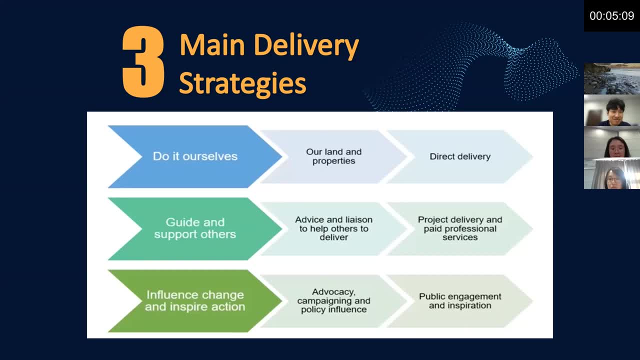 I mean as a scientist, we are not just doing science Now. we are more talking about how do we translate our knowledge, our findings, into good use, Into empowering the community, the public, into making them be involved and playing a role also. 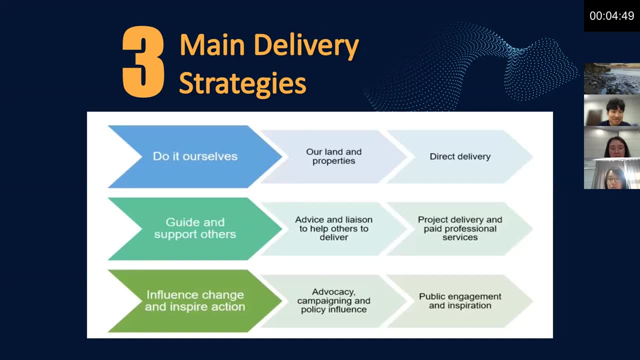 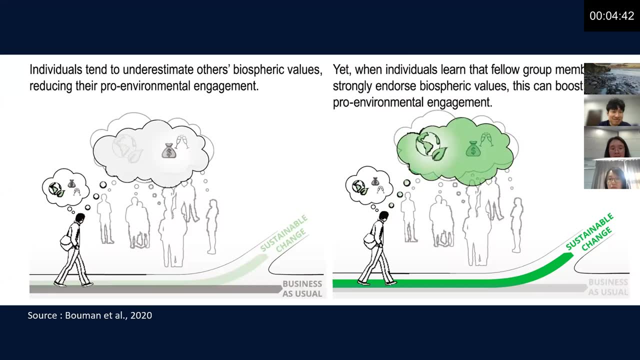 in protecting our marine biodiversity or even biodiversity in general In general. many of us knows what are the right things to do, But commonly people want to fit in what most people do and what should be done. We need social influencer, Yeah, to empower the public without the social influencer? 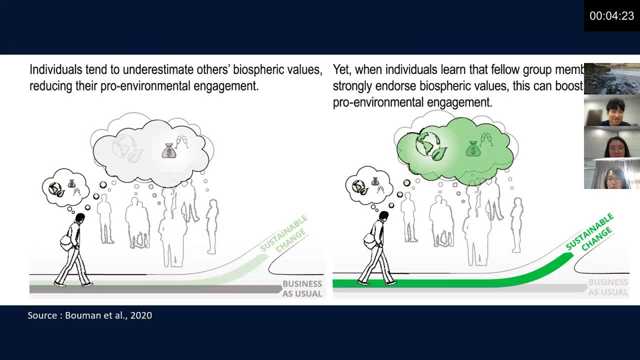 The knowledge is there, The understanding is there, But then business will be as usual without the social influencer, The public. we have to have the social influencer to empower the public for protection of biodiversity, to create a sustainable behavior. Then only we can achieve, we can map our roadmap to sustainable change. 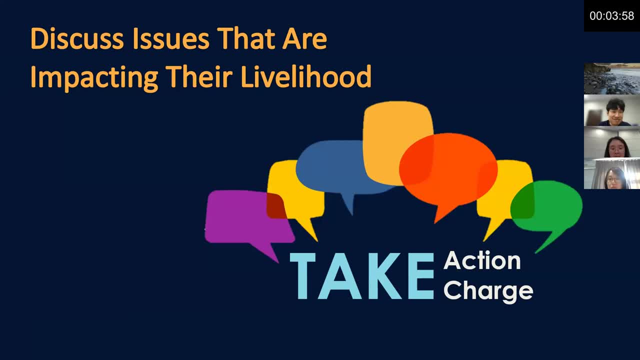 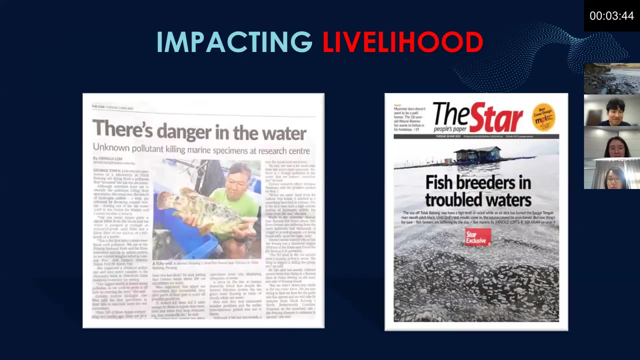 To empower the public, we need to discuss, or make them involved by discussing issues that are impacting their livelihood. We need to empower the public to take action and to take charge of their own environment- Issues that impacting the livelihood, such as fish kills affecting the livelihood of fish farmers. 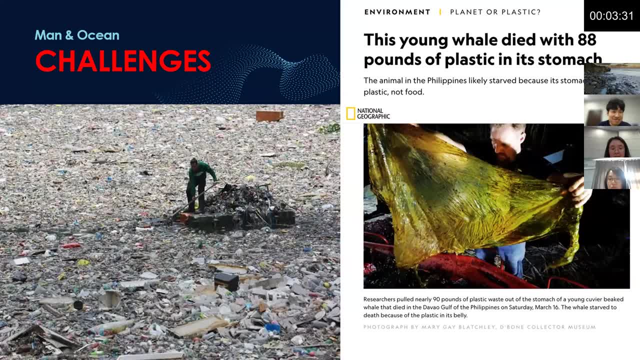 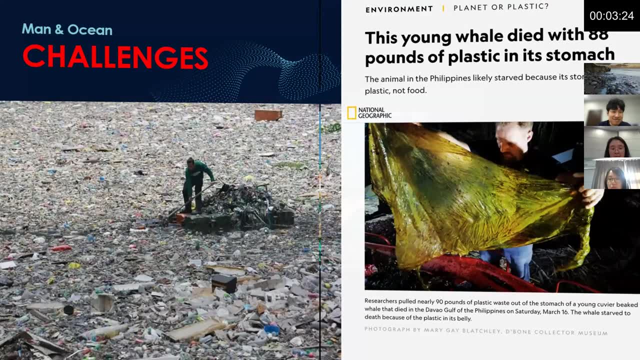 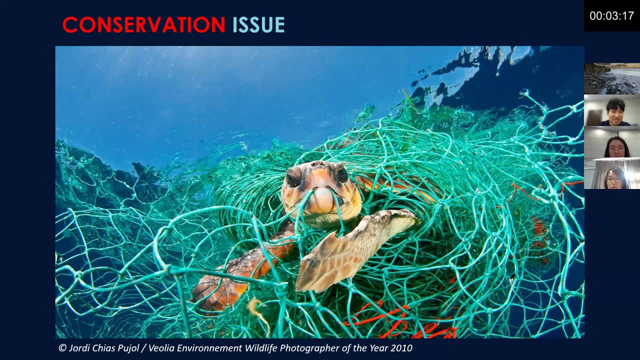 Issues such as plastic pollution, impacting the livelihoods, environment and organisms that we care for, Like the endangered species, Issues that touches the hearts of the public, such as this endangered species be caught in the abandoned fishing nets. you know, Pictures like this actually can give a lot of impacts. to engage. 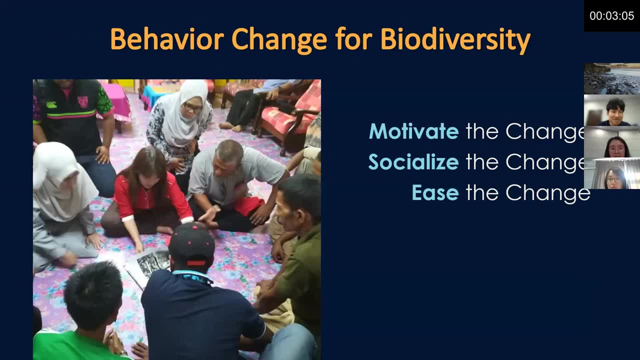 people in biodiversity and other environmental issues. One must provide the opportunity and the opportunity to engage people in biodiversity and other environmental issues. One must provide the opportunity to engage people in biodiversity and other environmental issues, the opportunity for enhanced understanding that empowers individuals to make choices. 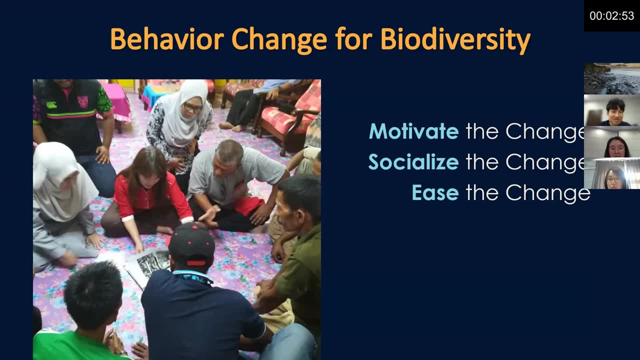 and to take action based on sound science and reliable recommendations. we have to use our, our findings, our data to actually translate that to the understanding of layman, understanding of the public. we must encourage behavioral change for biodiversity among the public. the approaches to be taken are: motivate the change, socialize the change and ease the change. the the social. 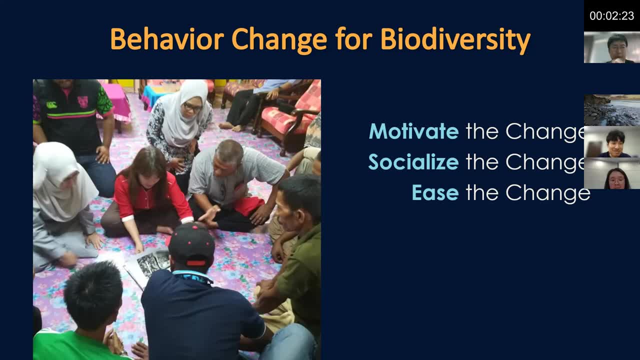 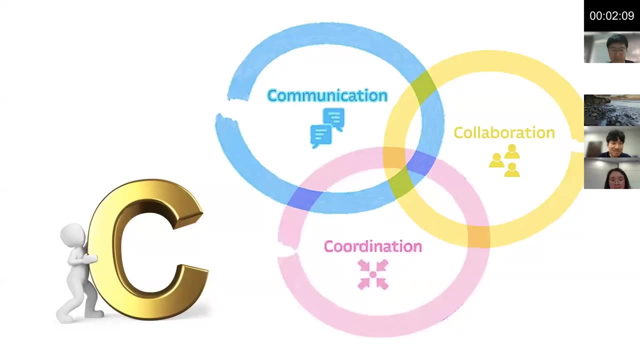 influencer, it can be from the scientists. you know, we have to come out from our comfort zone, from the ivory tower, and share what been shared, you know, in platform like this, with other stakeholders, which includes the public. and to empower the public, we must implement the three c's communication. 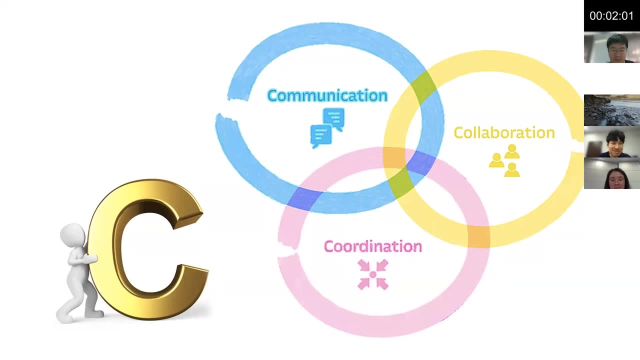 collaboration and coordination. it will be wonderful if we can incorporate the public, the stakeholders, into our triple i pcc program. you know, that is. that is fantastic because we need you know, in order to make things happen, to make things better as what we believe, we need the cooperation. 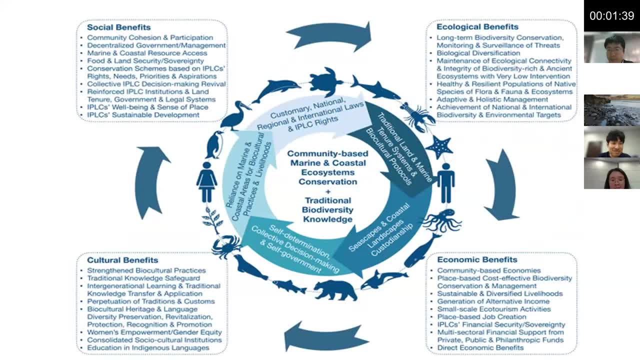 from all the public or the community should be made aware of the betterment of. what we need to do is including the support of large and small organizations, both from local and regional level, and to assist with the customers and the Seal and theھی fandom, and to 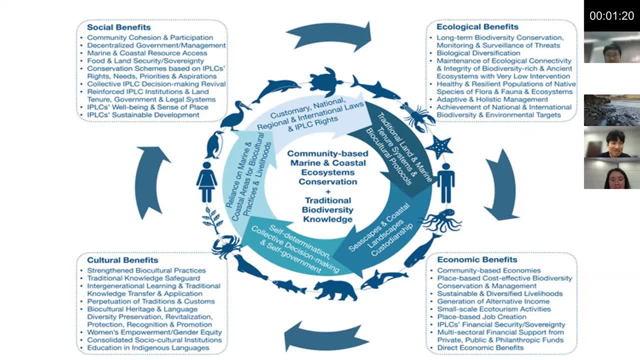 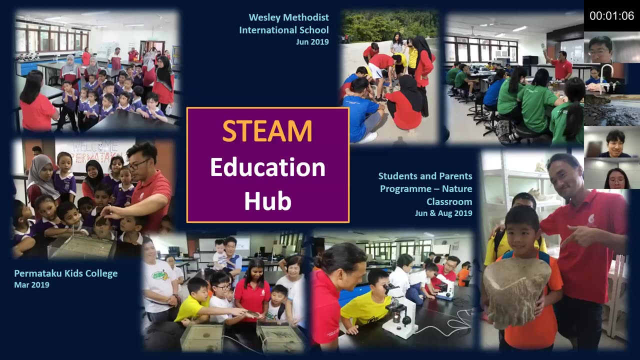 create a friendly rapport with all of our stakeholders, which is important. first of all, in addition to the community-based economic benefits, additional savings and benefits that we need to have for the future, we need to have the benefits of community-based and coastal conservation and traditional okay and traditional biodiversity knowledge, which includes social benefits. 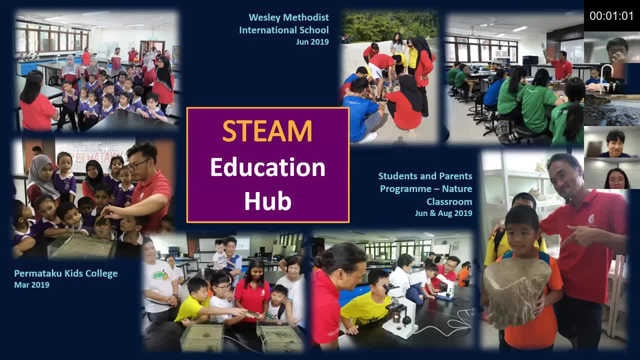 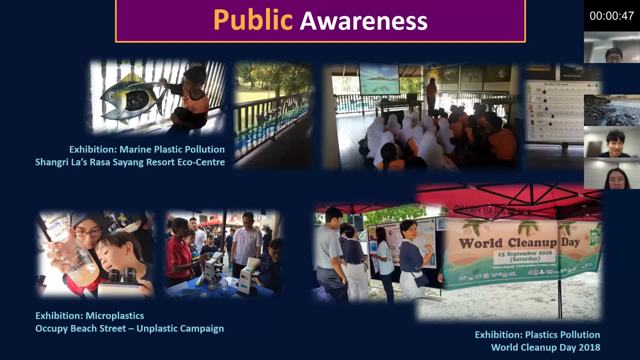 education. we have to groom our youth starting from a very young age. they were, they will be, our ambassador of the environment. they will be the caretaker of the environment. yeah, so empowerment through public awareness and involvement. we should look into creating more citizen science activities with the public, such as getting school children involved in collecting reliable data for 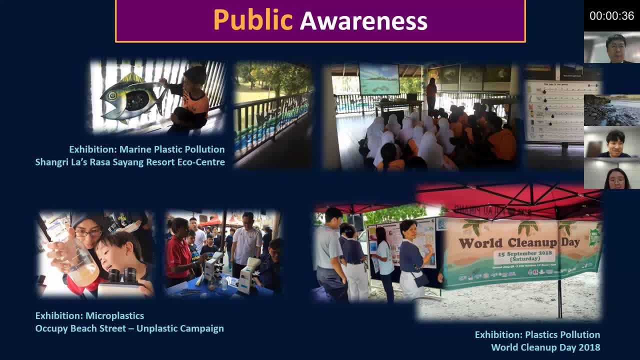 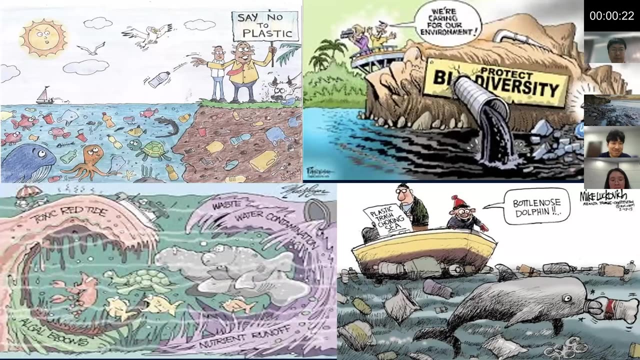 management and decision making. citizen science involve public professional partnerships that allow people of all ages an opportunity to participate in real scientific research. empowerment through stories. you know, in recent years, in our hectic lifestyle, people are reading less but are more engaged with social media. the media has an important role to play to disseminate. 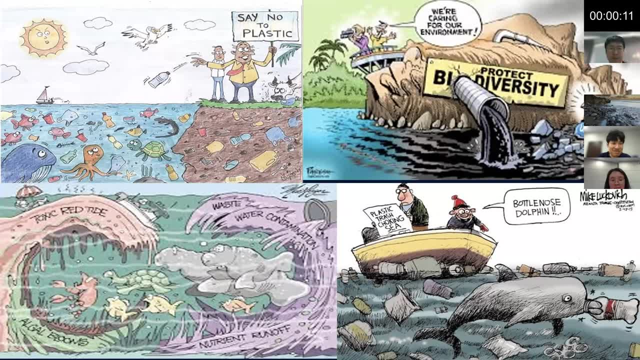 the awareness message to the public. the public can remember better about conservation or diversity and other issues better through stories, cartoons or comments, and more impactful message if it's been shared through short videos, for example, like youtube's or tick tock. you know, now it's getting more popular. there are many things we still do not know about our vast ocean. 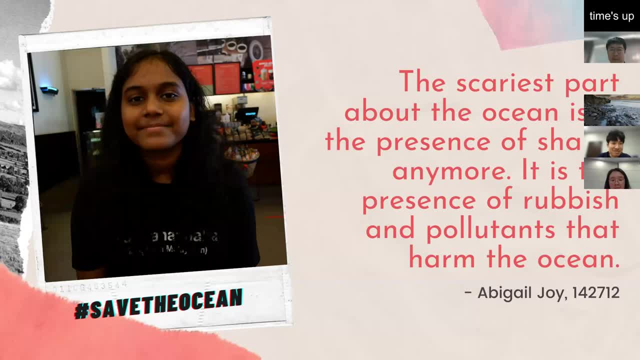 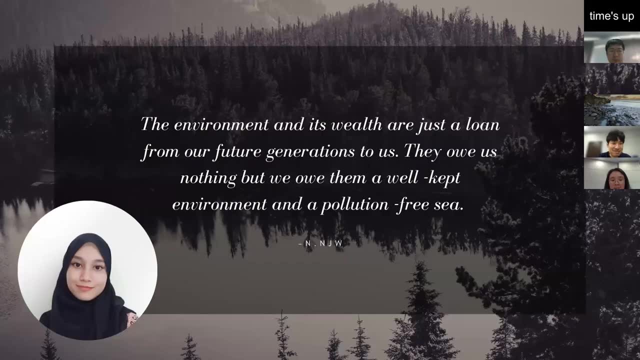 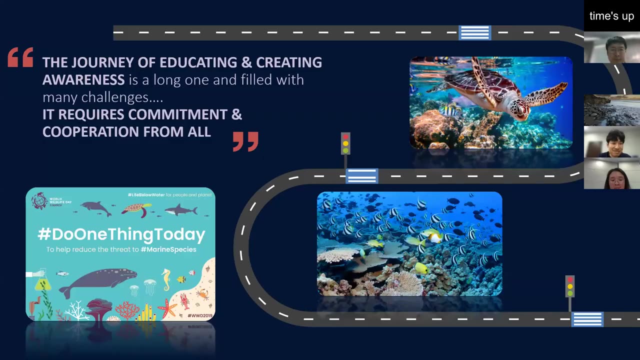 you know these are the the concern of our youth today. their voices should be heard in terms of protecting the environment. you know, this is another example of the youth concern you know. so it lies on our shoulder now. so the journey of educating and creating awareness is a long one and filled with many challenges. it requires commitment and cooperation. 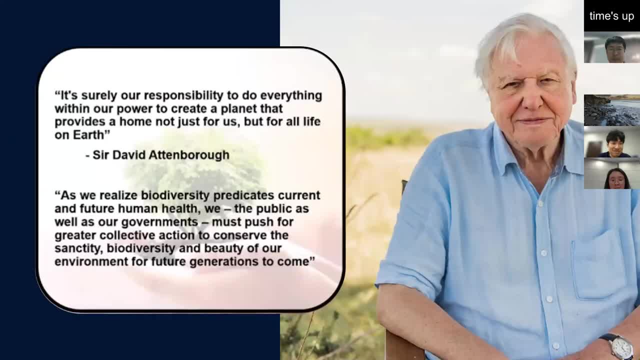 from all. as a closing remark, i quote the statement from sir david edinburgh again: it is surely our responsibility to do everything within our power to create a planet that provides a home not just for us, but for all life on earth. as we realize, biodiversity predated. 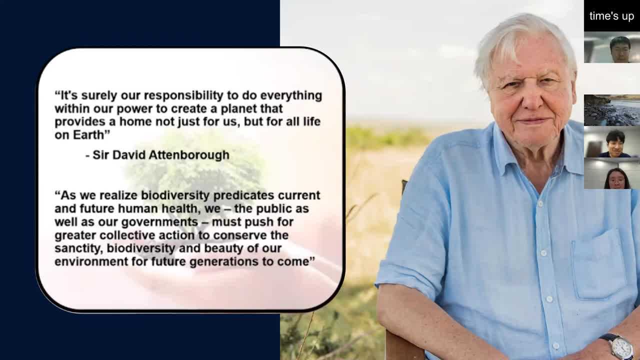 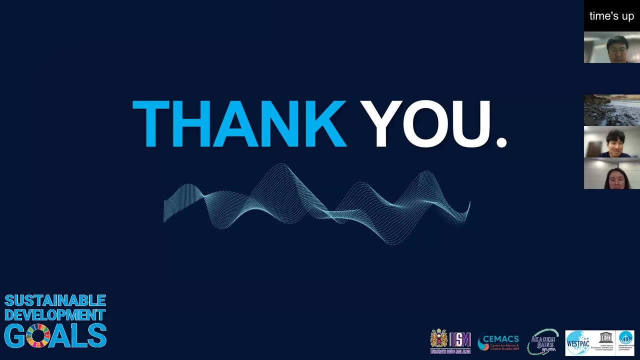 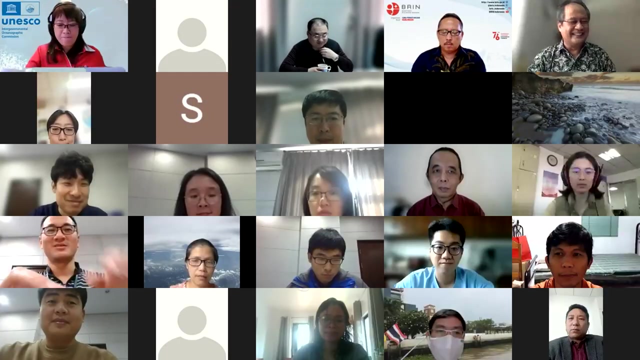 current and future human health. we, the public, as well as our governments, must push for greater collective action to conserve the sanctity, biodiversity and beauty of our environment for the future generation to come. thank you very much for your attention back to you, pak zaina, thank you. thank you, prof eileen. i think it's very inspiring uh from uh professional island talk right. 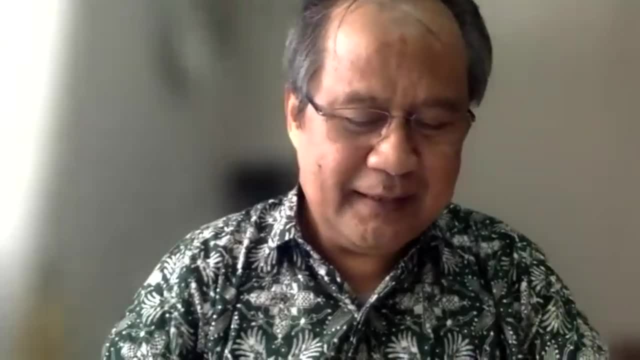 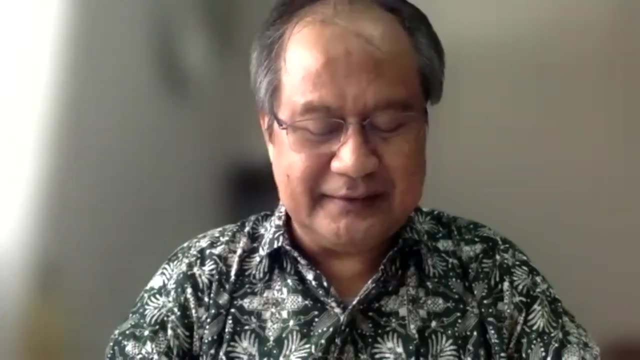 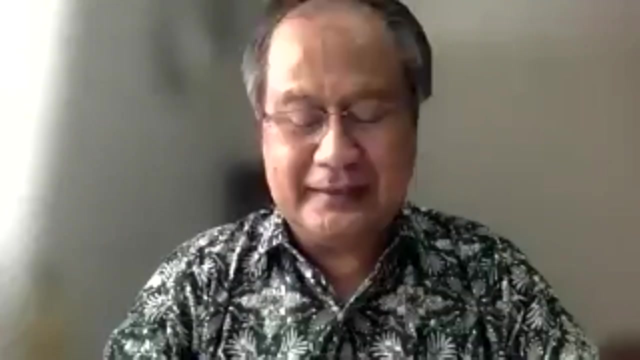 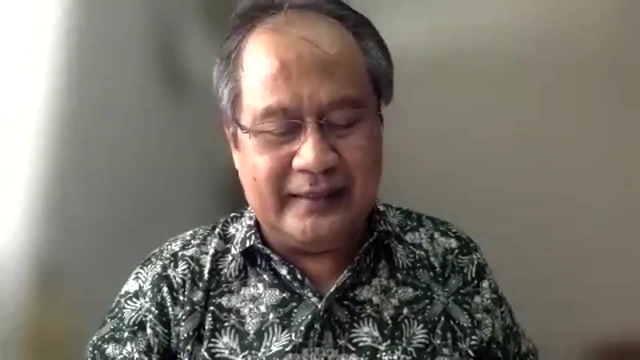 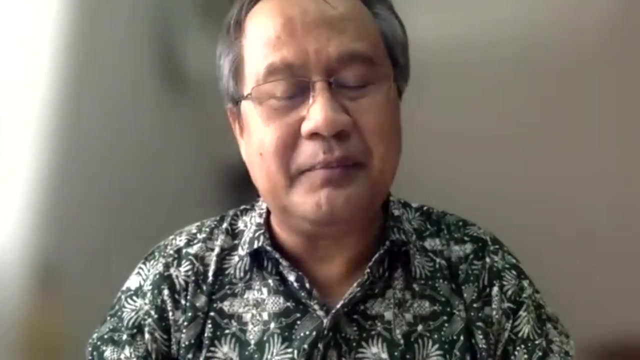 so we have passed 45 minutes. we have already listened professor hwan wang on scientific issue and challenge on marine biodiversity, professor oki on how to approach this utilization of biodiversity sustainably. prof elder eileen has been providing the importance of protection of marine biodiversity for the benefit of environment and also the people. so the next 15 minutes. 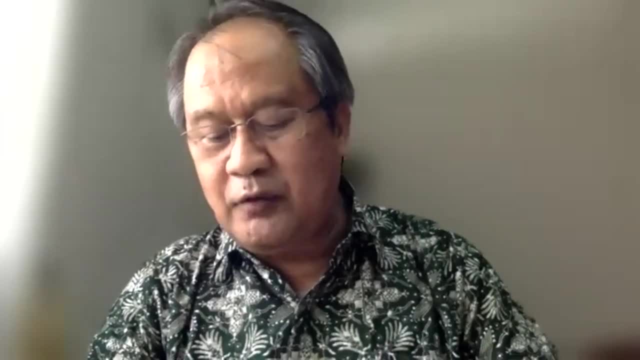 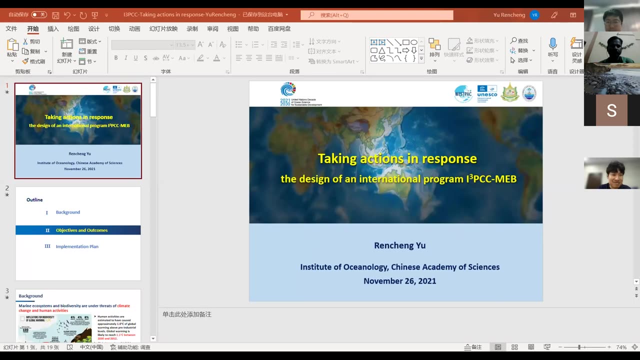 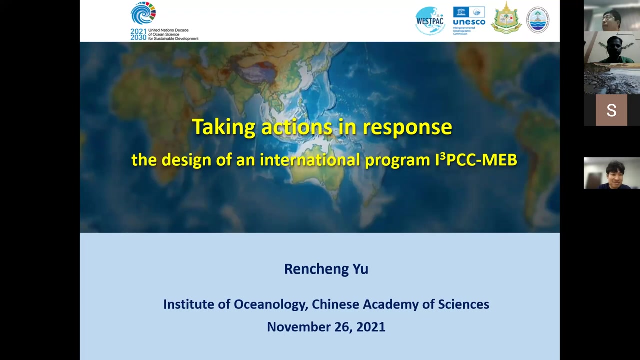 the final 15-minute talk will be on how we taking action of uh research and at regional level. professor reaching you will give a talk. so he is a professor at institute of oceanology china academy of science. he is also assistant director of uh eocast his expertise in marine ecology and harmful algal bloom. so the next 15 minutes 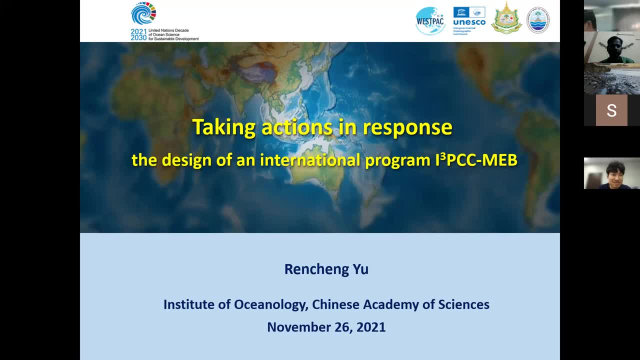 will be yours, from you, the floor is yours. thank you, uh. thank you, pakistan. can you hear me clearly? yes, yes, yes, thank you, uh, yeah, uh. just now we have a uh three present, uh three presentations about the challenges and also the values of marine biodiversity and the ecosystems in the. 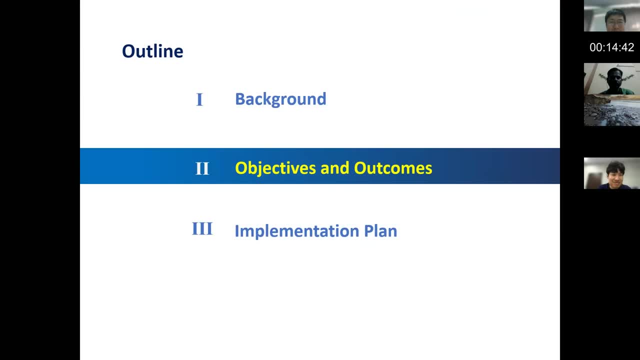 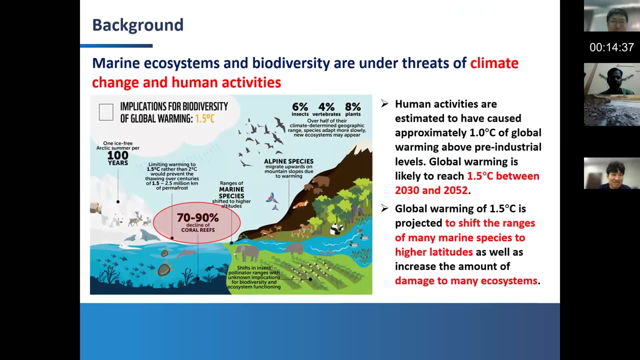 ipcc region are a, and i would like to give a talk on the actions we should take uh to protect the marine biodiversity and also marine ecosystems in this region. we all understand that uh the climate change has posed significant threats to the sustainability of marine ecosystems and also marine biodiversity. it was projected that there will be around 1.5 to 2 centigrade. 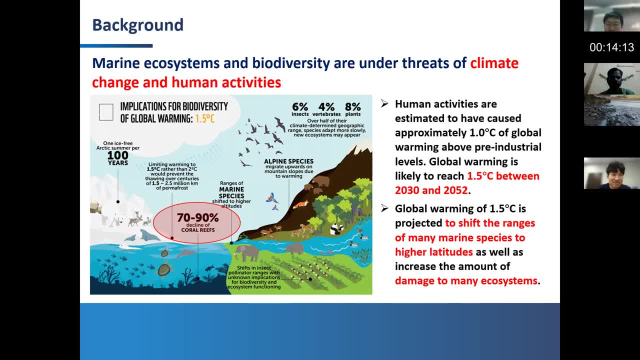 between 2030 and 2050s. so this increase of temperature will have significant impacts, particularly on the marine ecosystems in the polar region and also the ecosystems based on coral reefs. uh, and this is uh extremely important for for the ipcc region, sorry uh, as just mentioned uh this: 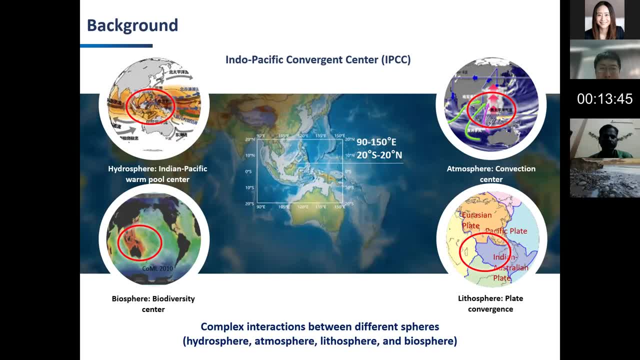 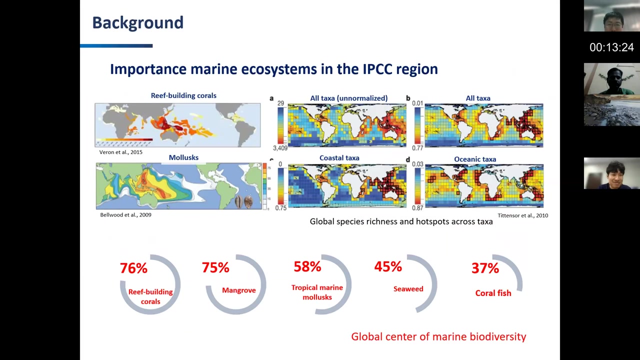 region uh is a very important region for the uh multiple sphere interactions. it's a hot spot of marine biodiversity and it's also a region with significant impacts of ocean circulation and future climate change. so we all understand that the marine ecosystem biodiversity is very rich here in this region. 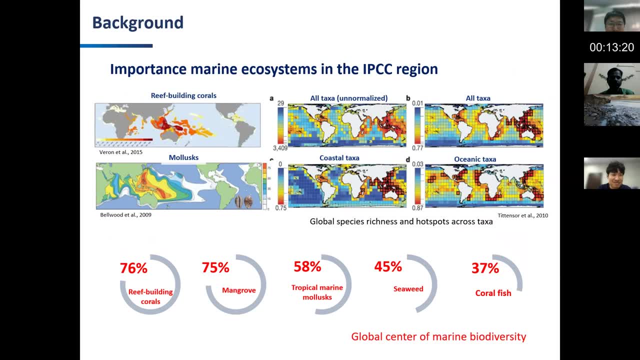 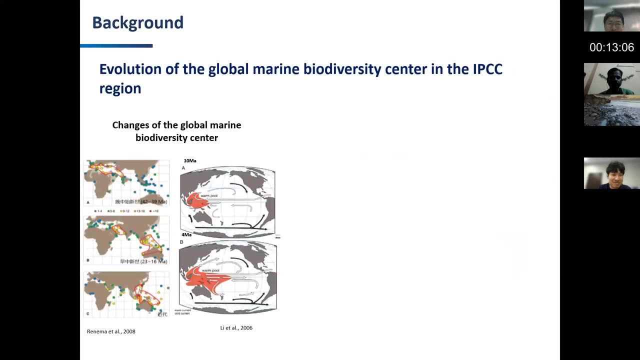 and- and this is of high value not only for uhenges, but also for the potential chemical resources and genetic resources, as just introduced by professor oki- and we all understand that uh, the future evolution of global warming uh will have significant impacts on the biodiversity in this region, because we understand that the formation of marine biodiversity center. 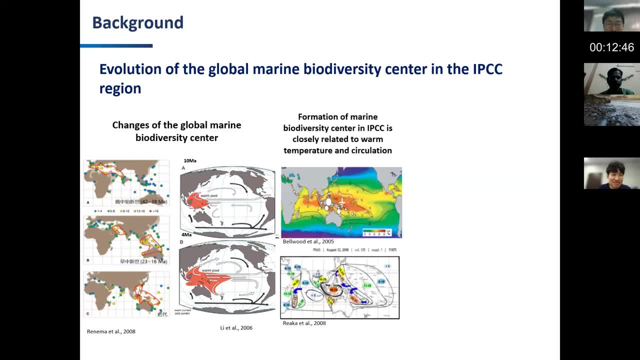 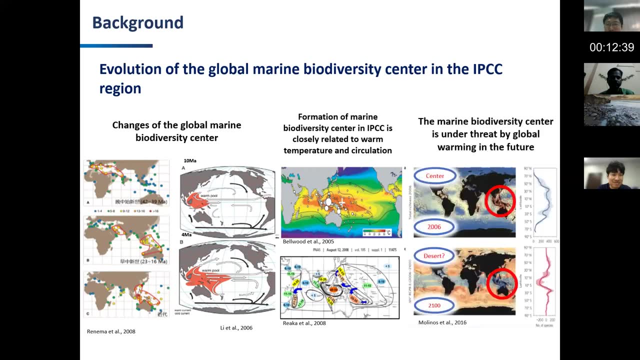 in this region is closely related to the geological evolution and also the effects of warm pool. But the future increase of temperature will significantly affect marine ecosystem and biodiversity in this region and thus affect the values and services of marine ecosystems. But more than that, in this region most of the countries are developing countries and people. 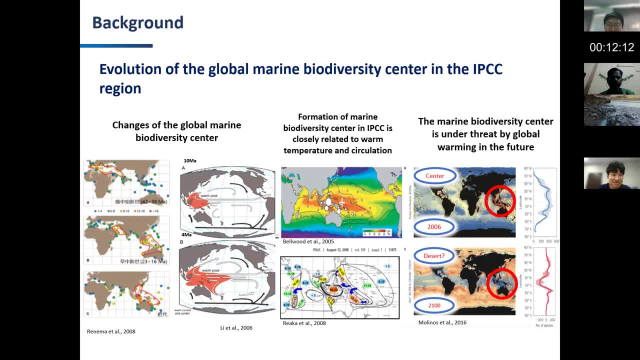 are relying on the marine ecosystems to have their food, have their resources and have their working opportunities. So the pollution and other issues, together with climate change. climate change will significantly affect the health of marine ecosystems in this region and led to many issues like, for example, hamburger blooms, which will there will be. 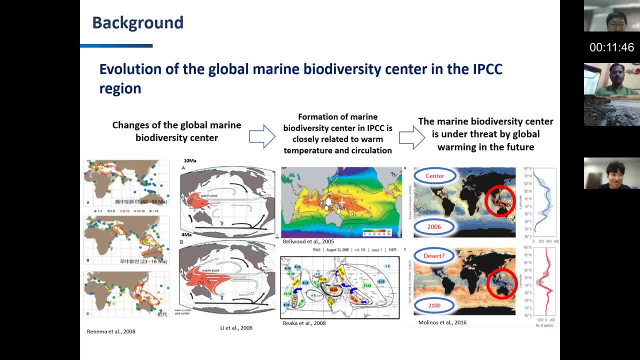 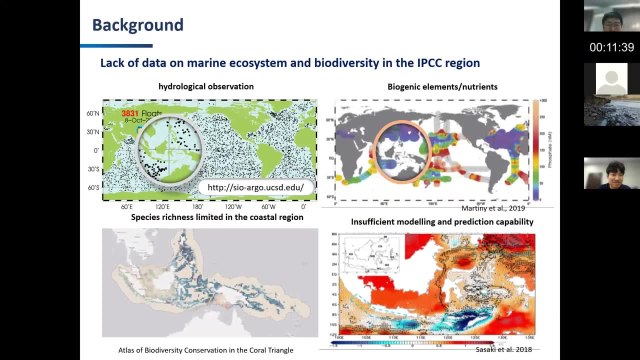 another session shortly after our session, But at this stage we don't have much understanding on the. we still have a lot of gaps in data acquisition, in observation and in investment of ecosystems. So we need to think about the future evolution of marine ecosystems. So all these gaps need. 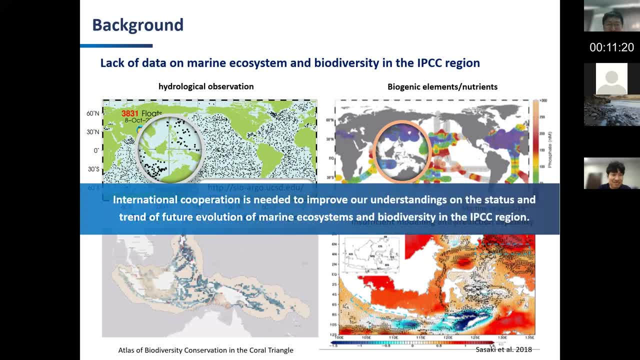 to be solved. But in this region we have many countries here, so we need a strong international collaboration to improve our understanding on the status and the trend of the marine ecosystems and also marine biodiversity. So that's the reason why we think it's important. 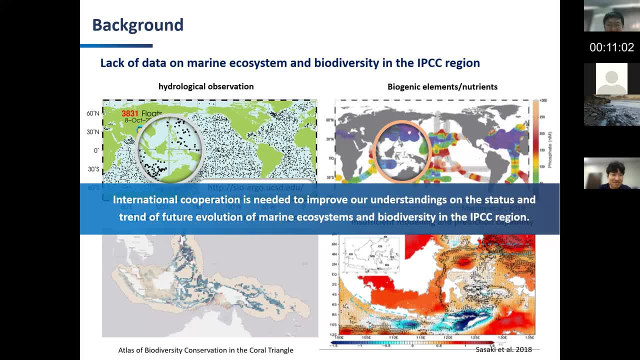 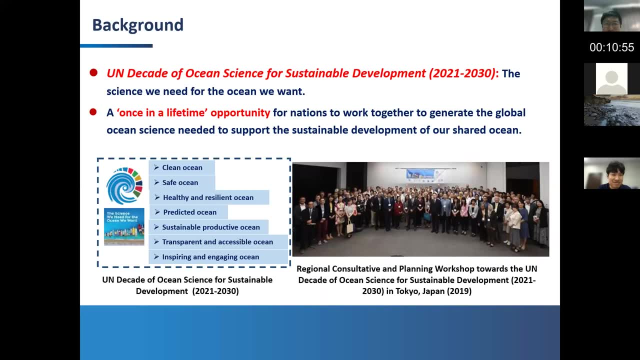 to put forward an international collaboration program, And I think the UN Decade of Ocean Science for Sustainable Development offers us a very good opportunity for us to carry out this kind of collaboration. It offers a once-in-a-life opportunity not only for the scientists working on marine science, but also for the other. 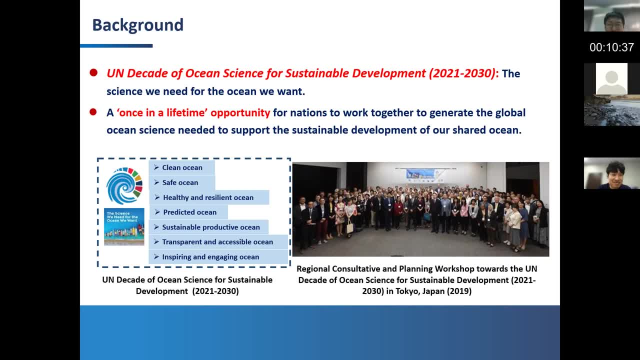 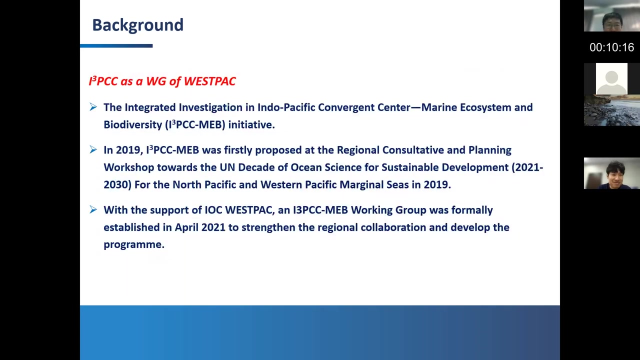 for the industries and for the students to join this kind of collaboration. So in the conference organized in 2019 in Tokyo, we put forward a primary idea on the organization of a triple IPCC MEB program in this region And fortunately this program was supported. 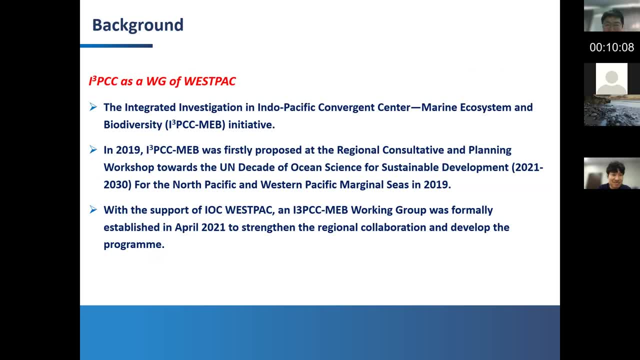 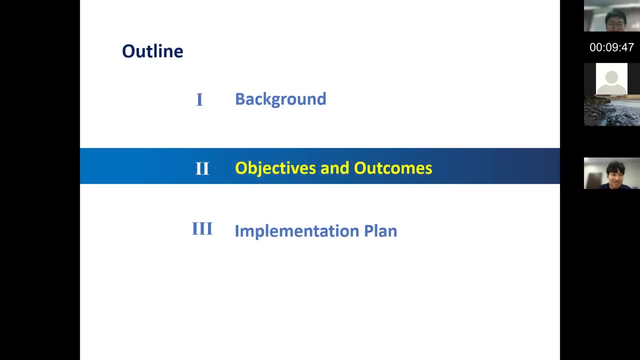 by the Westpac and it was listed as a working group in April this year. And this program, we hope, will strengthen the regional collaboration and for the development of the future international program. So I would like to give a brief introduction about the objectives and also the outcomes. 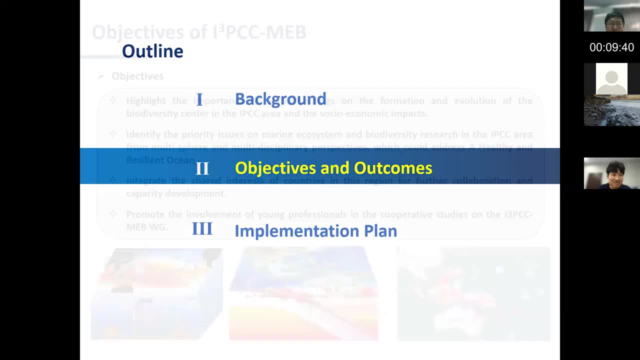 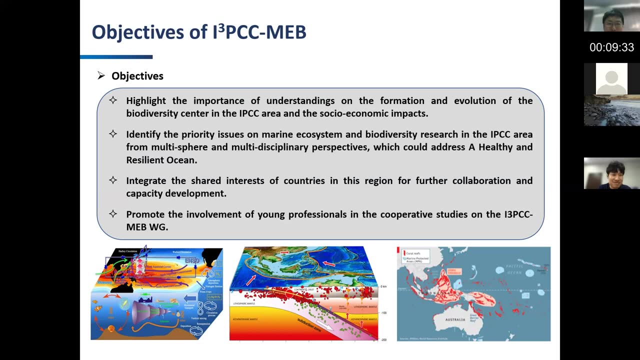 of the triple IPCC MEB program- I'm sorry, the working group. So we hope, through the implementation of this working group as well as this incubator meeting, we hope we could highlight the importance of the understandings on the formation and evolution of the biodiversity center in the in this ipcc area and also 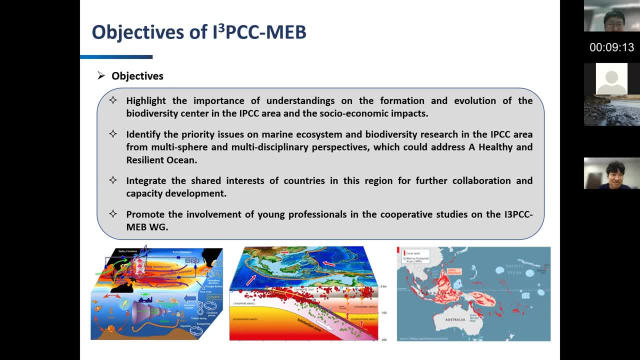 its social economic impacts. through the implementation of the working group and the discussion in this meeting, we hope to identify the priority issues on marine ecosystem and biodiversity research from the multi-sphere and multi-disciplinary perspectives, and this will help us to address a health and the resident ocean, and we also hope to integrate the shared interests of 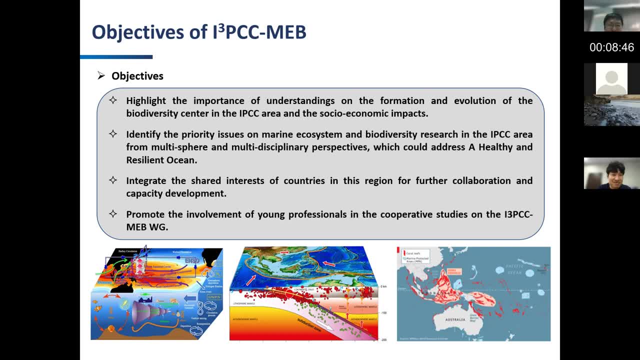 different countries in this country to promote further collaboration and also to improve our capability in observation, forecasting and the prediction of the marine ecosystem changes, and another objective is to help to involve more young professionals in the corporate cooperative studies on the triple ipcc map program, and there are many different aspects related to 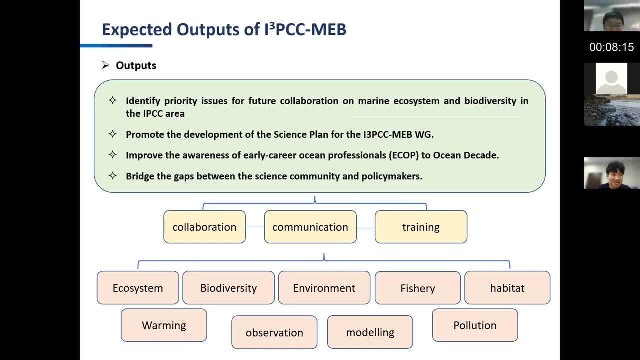 the marine biodiversity and the marine ecosystems in this region, for example, marine ecosystems, marine biodiversity, marine environment, fisheries, the habitat, the warming issue, the pollution issue and the also the marine ecological disaster issue, like humboldt or blooms. we need to integrate all the different parts through observation and modeling and try to develop them. develop them through integration. 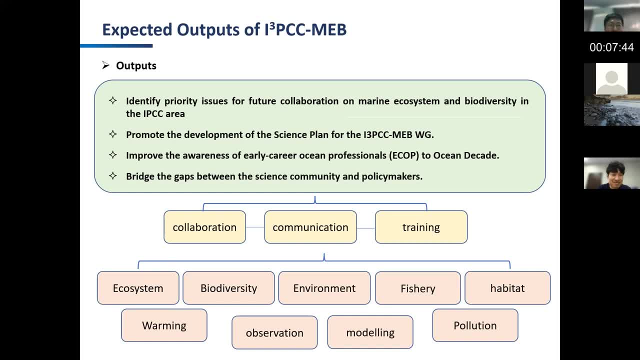 and collaboration, communication and training, to have some important outputs. the major outputs could be identified: priority issues for future collaboration and marine ecosystem and biodiversity. to promote the development of the science plan and also probably an implementation plan for the tribal ipcc web map program. and to improve the awareness of early career ocean professionals to ocean decade and try to bridge 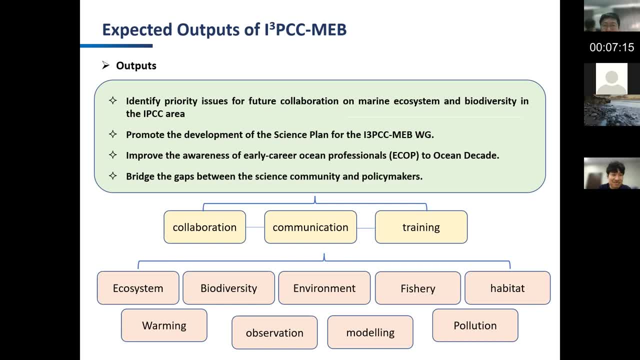 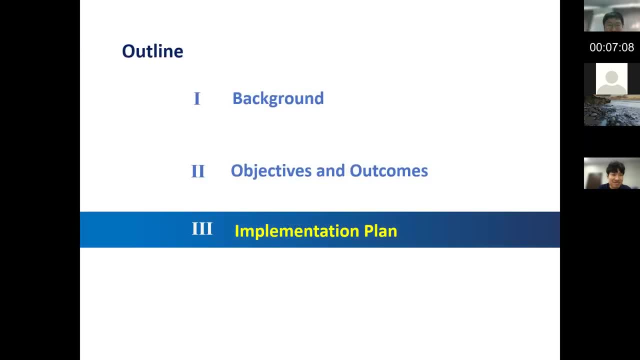 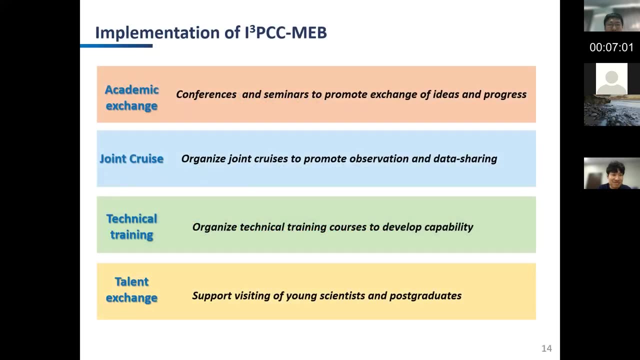 bridge the gaps between the science community and also the policy makers. so, um, i think it's the time for us to develop this, this uh program, and the how should we implement the the plan? there are several aspects we could working together. first is the academic exchange. we could organize conference and seminars to promote the exchange. 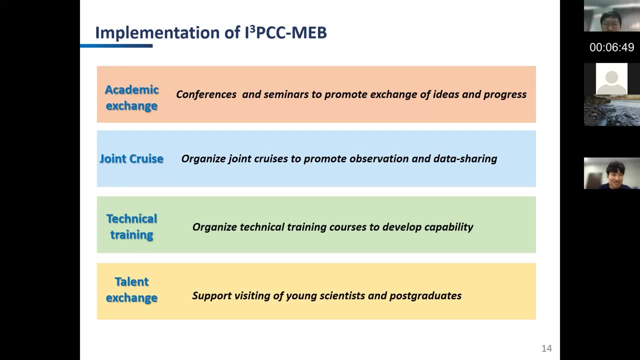 of ideas and progresses on marine ecosystem and biodiversity research in this region and we could organize joint crises to promote the observation and also the data sharing. and there will be technical trainings, uh for to develop our capability and reservation, such like the artificial intelligence and edna. 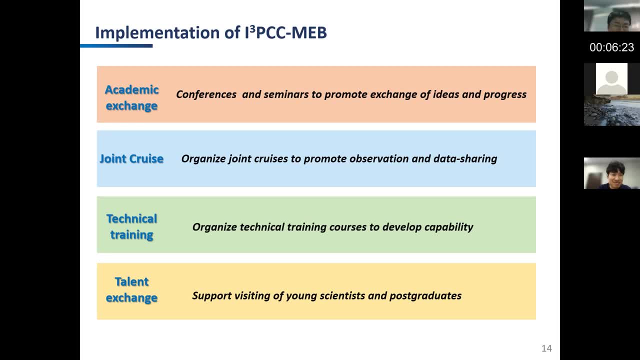 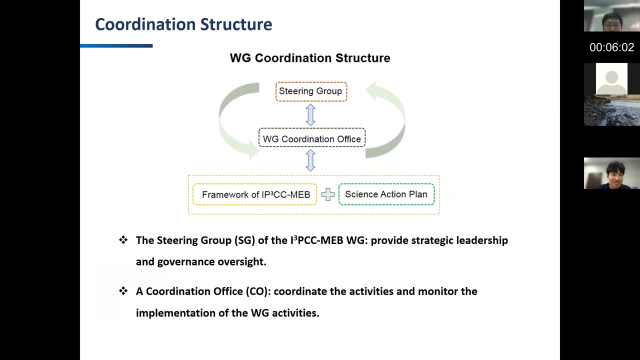 the new techniques could be involved in the future collaboration and also we could promote the talent exchange through the supporting of young scientists to waste to visit among different countries. to improve the the joint research, we have developed primarily a coordination structure uh through the establishment establishment of a steering group and also a coordination office. so this steering group, 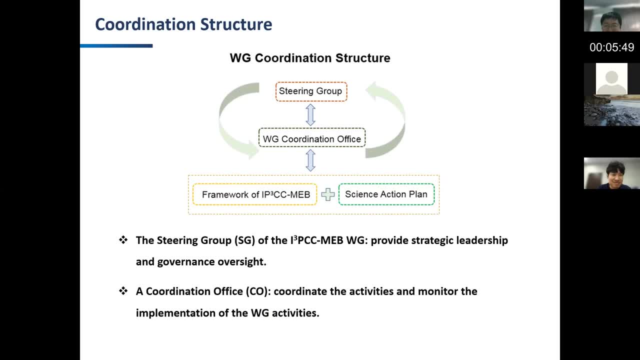 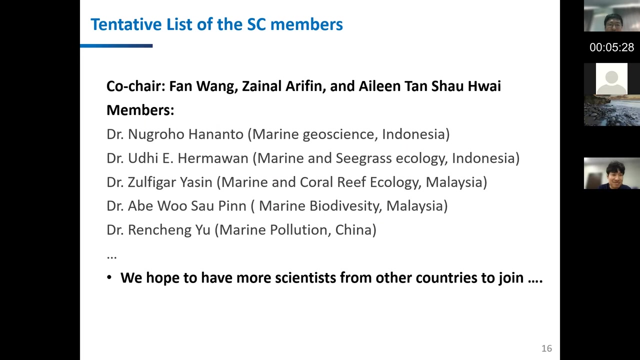 uh for the working group uh, the. its major responsibility is to provide strategic leadership and governance oversight, and the coordination office will help to coordinate the activities and monitor the implementation of the coordination and the coordination of the organization of this working group. so far, we have uh invited uh several professors uh to uh for this for this steering group. 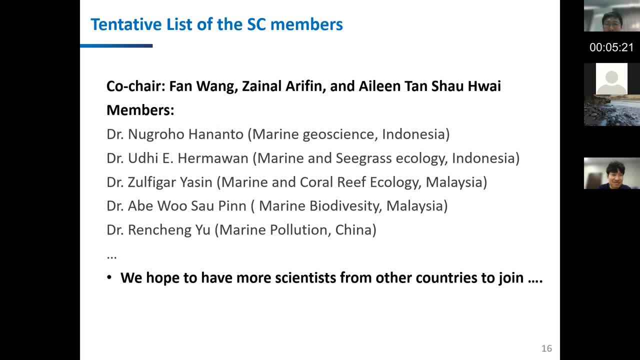 including professor fan one, uh patina everything and uh professor at in time, and also uh scientists from indonesia, from malaysia and from china are involved in this working group and we hope to have uh some opportunities from other countries to join our scientific steering uh group to help. 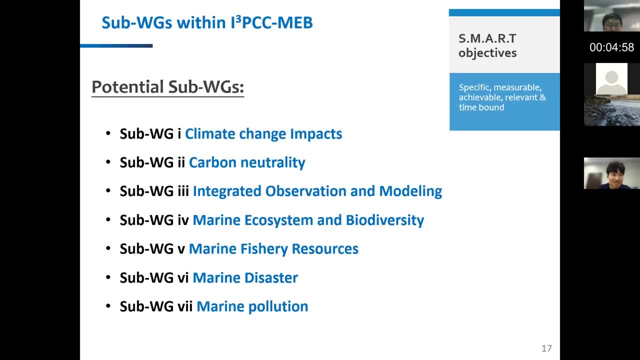 supervise the the working group, and also we think there are many different aspects related to this working group, such as climate change issues, carbon neutrality and observation modeling, marine ecosystem and biodiversity, fishery resources, marine ecological disasters and marine pollution issues, So we plan to develop different subworking groups. 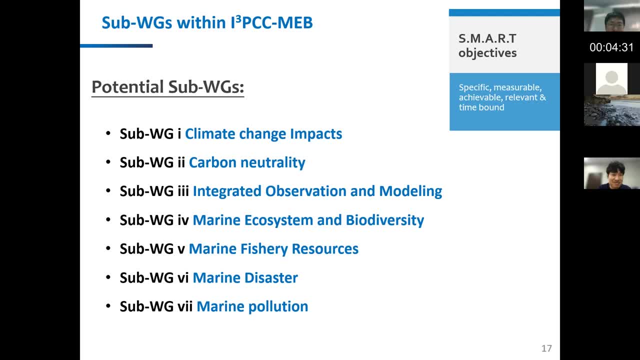 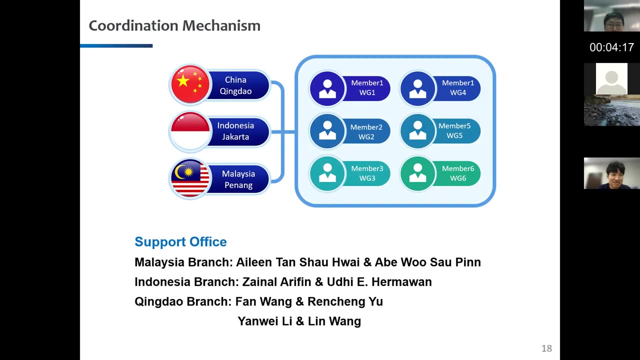 which could involve to have more young scientists get involved into this collaboration working group. To coordinate the operation of this working group, we also plan to establish a office for the coordination affairs. We plan to have three different branches: from Malaysia, from Indonesia and also from China. 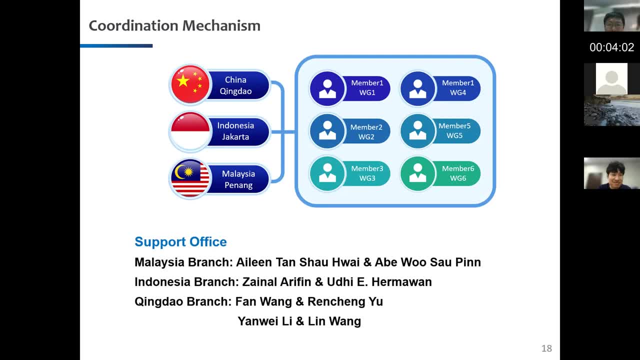 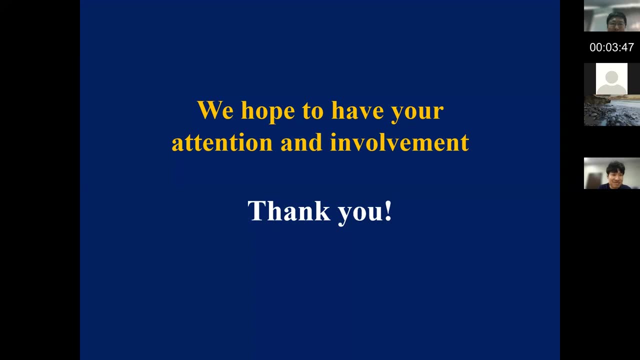 to coordinate the different subworking groups and try to organize the activities within this international program And that's a primary idea about the design of the TRIPAL IPCC MAP program And we hope to have all your attentions and the involvement from the scientists, especially the young scientists. 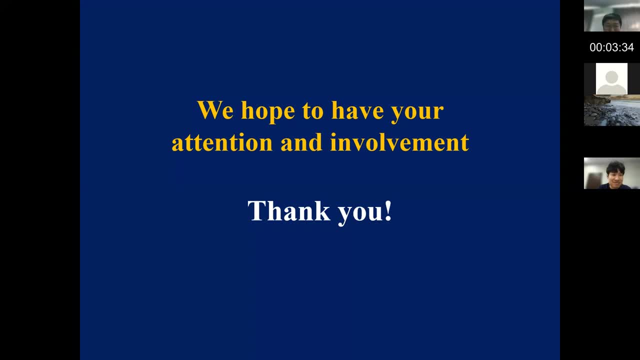 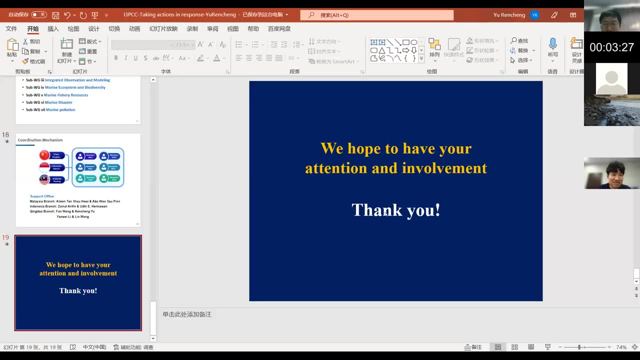 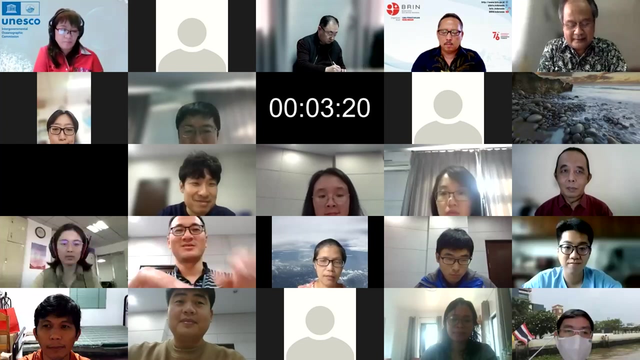 Thank you very much. Thank you, Professor Renxing Yu. I think this is a kind of, if I may say, the IPCC Indo-Pacific Convergence Center is a kind of a platform for working at a regional level. So, as Professor Fang Wang mentioned in the first talk, 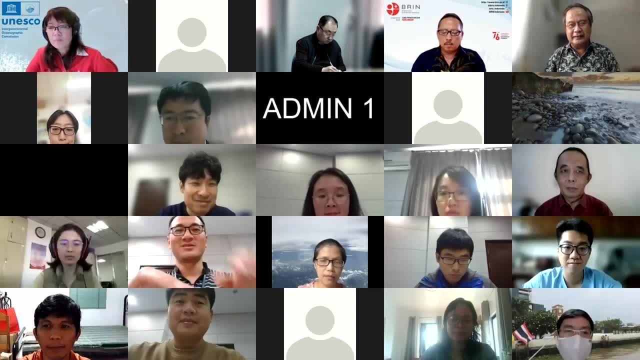 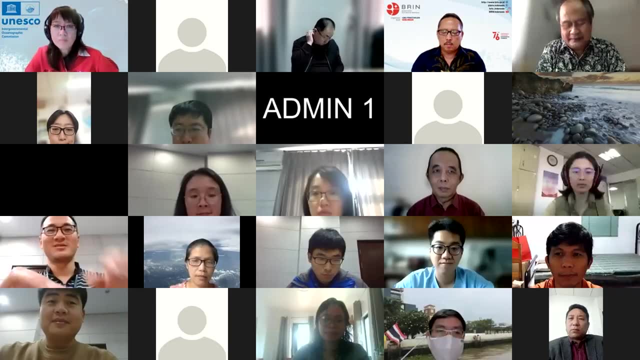 that this working group will focus on actually multi-layer activities at the level of hydrosphere. So focus on thermal center atmosphere issue, on advection and lithosphere. on plate convergent did a lot of a discussion today on biosphere, on biodiversity center area, so to move to the next, 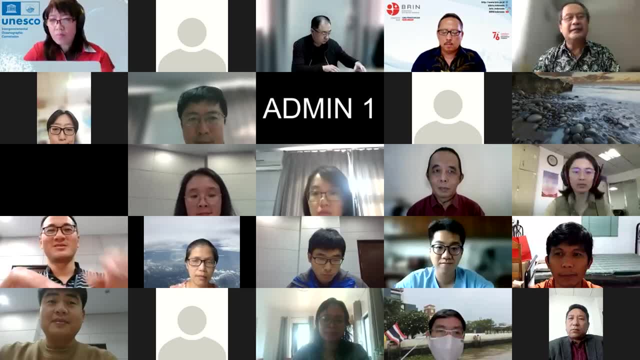 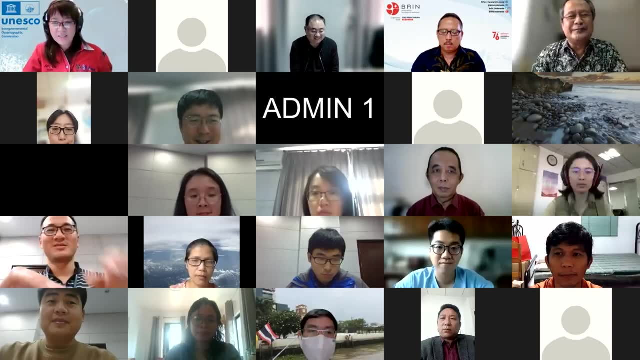 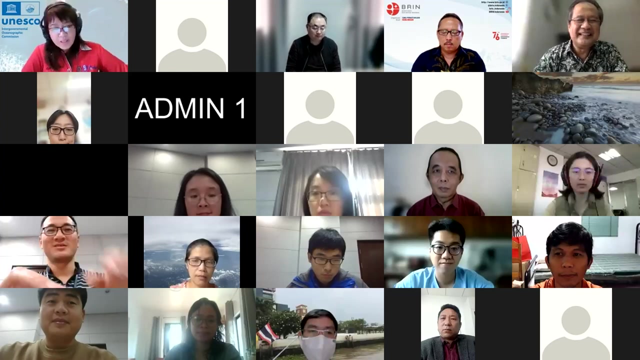 discussion. i transfer from indonesia to malaysia. ibu, prof eileen, to leave this discussion please, prof eileen, i send to malaysia now. thank you, thank you. thank you, pak zainal. you know, from indonesia to malaysia. earlier on was from china, indonesia, now now, lastly, to malaysia. thank you very much. so now we move on to the next session, which is the. 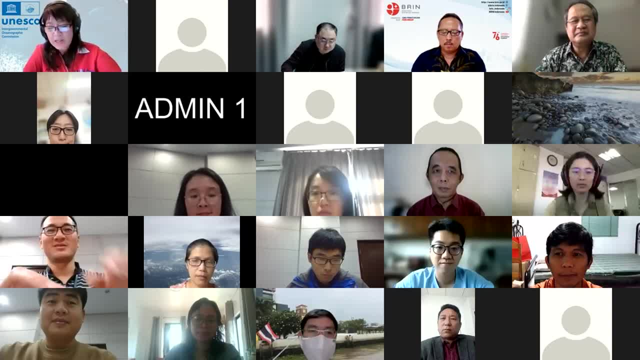 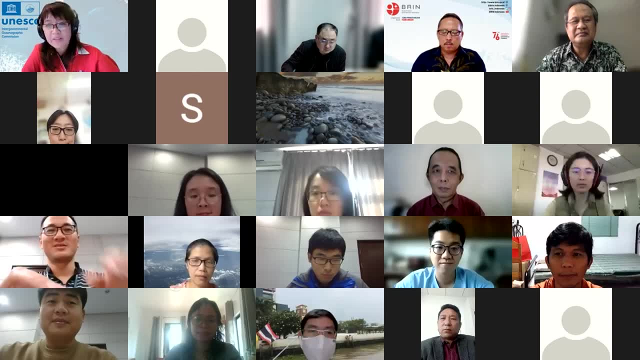 mini talks. yeah, we have three speakers that we have uh invited um. each speaker give a very short talk, about five minutes, so we have um enough time for discussion, hopefully. yeah, so uh, first i would like to invite dr christian, an earlier career scientist from wayanba university of sri lanka, his expertise. 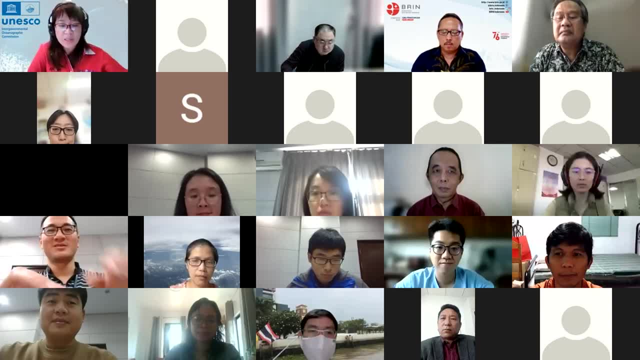 is in marine biology, focusing on taxonomic identification and presence status of jellyfish in the coastal waters of sri lanka. um krishnan's talk will be on the role of marine biodata in supporting industry. um over to you, uh, christian, christian, are you here? 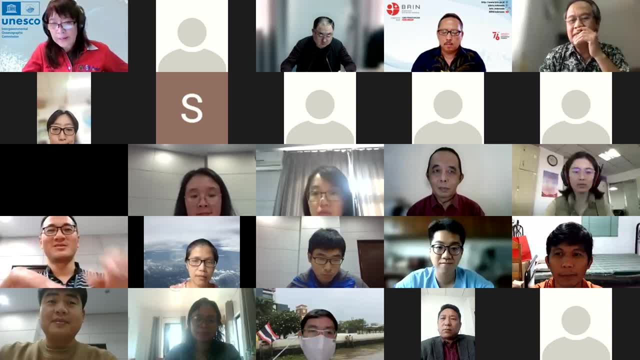 okay, i just got a message from our ti support team that he has. he was here earlier, but he has accidentally left while waiting for him. um and and without wasting time, maybe i will invite our second speaker first. yeah, uh, dr jay jeng, associate professor from the institute of oceanography china academy of science. 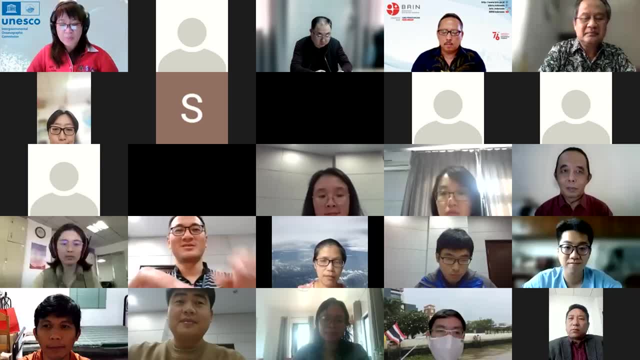 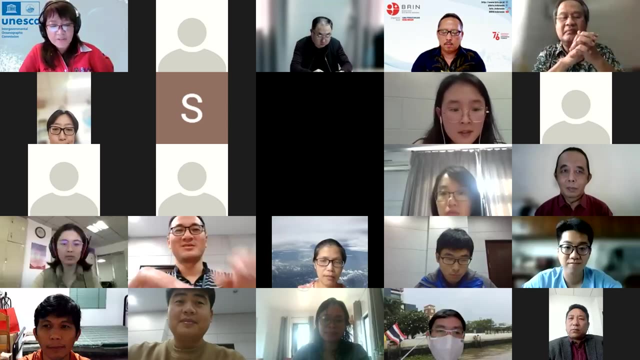 dr jay jung's expertise is on seaweed genomics, evolutionary biology and population genetics. Dr Zhe Zhang's talk entitled Phylogeographic Diversification and Post-Gracial Recolonization Patterns: the Case of Sargassum Species in the IPCC. 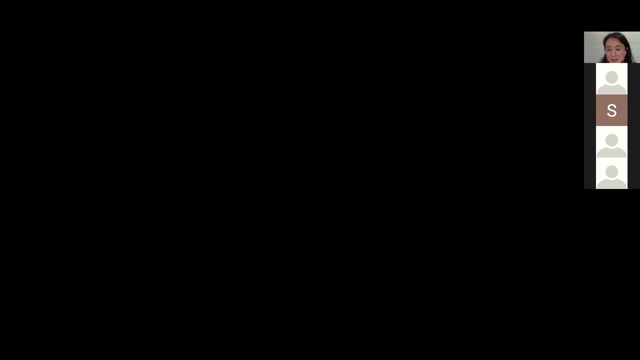 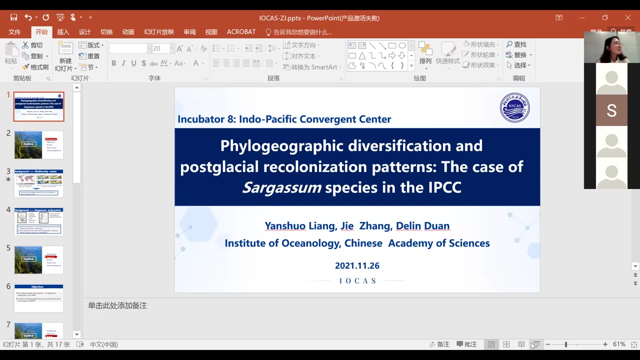 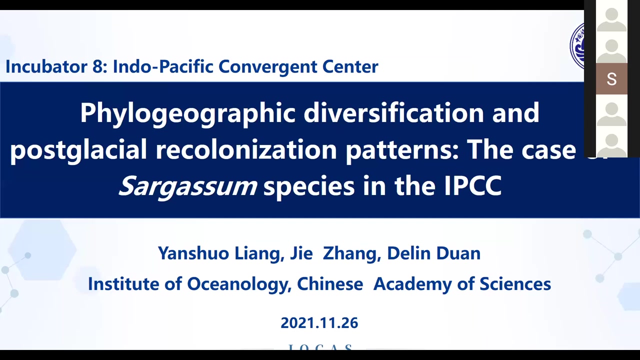 Over to you, Dr Zhe Zhang. Thank you, Yes, I think, Dr Zhe Zhang. I think you have to ask those surrounding you to move further away. Thank you, Dr Zhe Zhang, I think, for not speak. we have to turn it off. 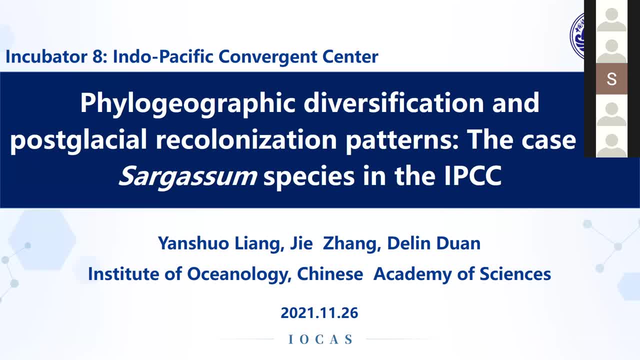 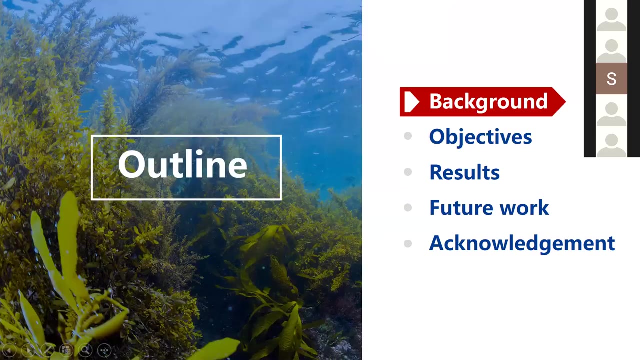 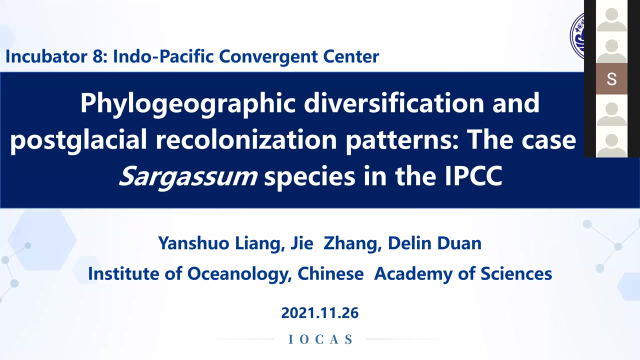 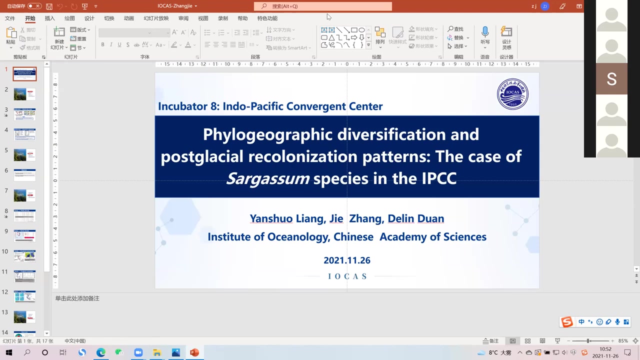 Dr Zhe Zhang. are you there? Dr Zhe Zhang, Your screen is already uploaded, is already on the screen. Thank you, Yes, everything is okay over there, Zhe Zhang. Hi, Professor Ali, Yes, yes, 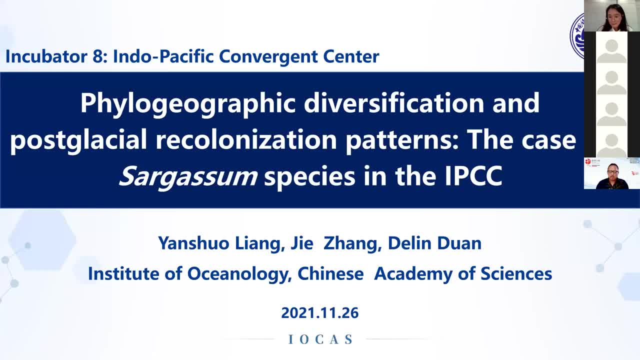 Can you see the slide? I can see the slide, but can you put it? Yes, yes, Thank you, Please. Okay, Good morning everyone. I'm Zhe Zhang from ICERS. It's my great honor to share our recent work with all of you. 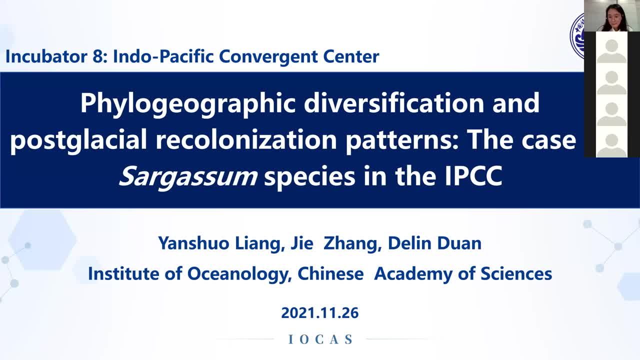 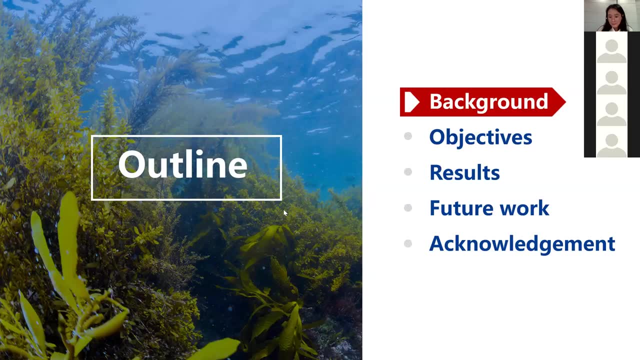 Our research work focused on phylogeographic diversification and the post-glacial Zhe Zhang. you're amazing Mute. you're accidentally unmuted. You're accidentally muted. Please unmute yourself. Yes, Can you hear? Yeah? 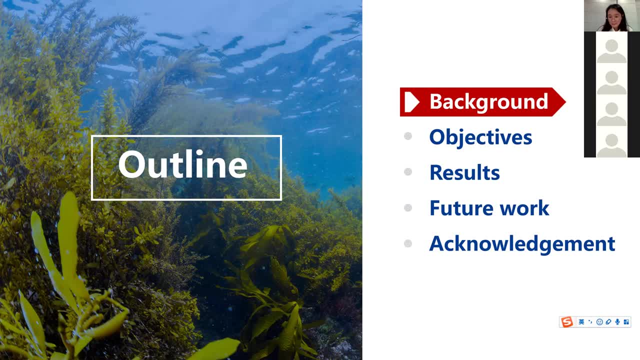 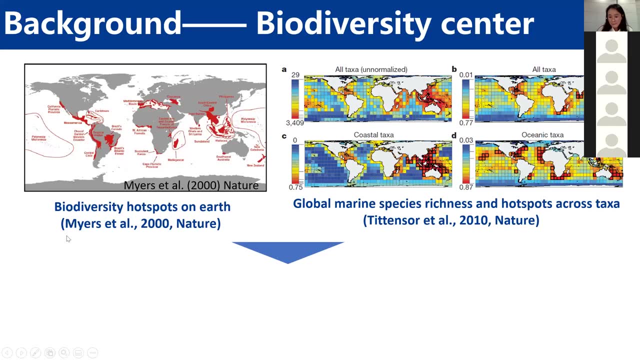 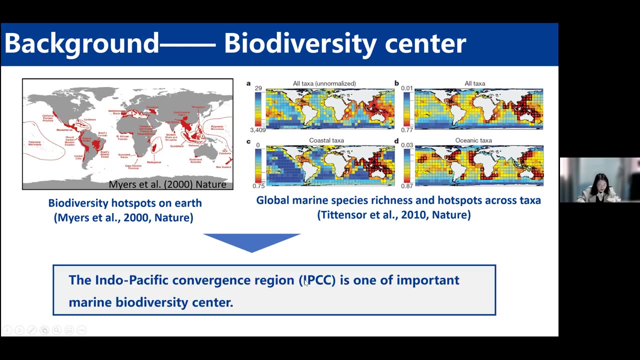 Yes, Okay. First I introduce the background of our research work. The left figure shows the biodiversity hotspots on Earth. The right figures show the global marine species' rich evidence. The right figures show that IPCC is one of the important marine biodiversity centers. 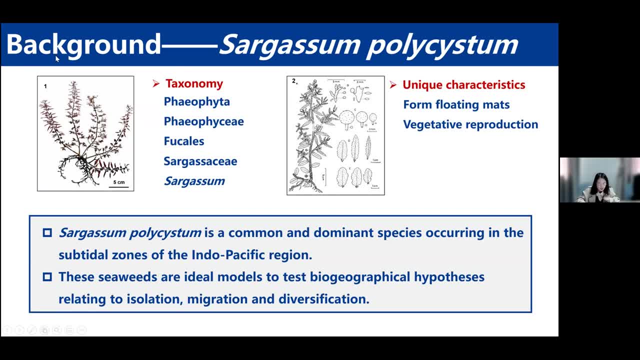 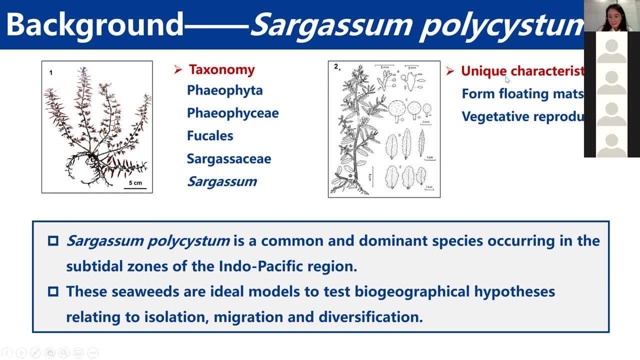 Our research work focuses on one important seaweed, Sakasama polysystem. The seaweed is a common and dominant seaweed occurring in the sub-tidal zones of the Indo-Pacific region. It belongs to Sakasama genus with some unique characteristics. 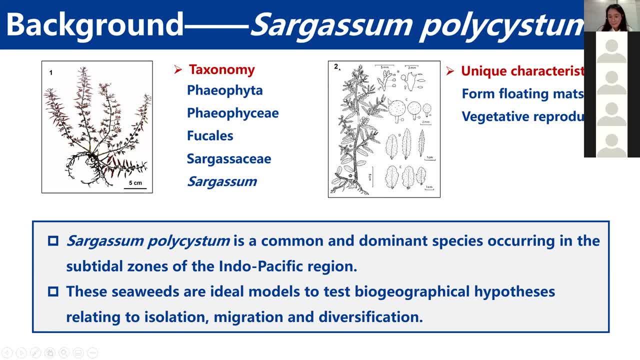 The seaweed contains vesicles. It's valley, so it can form floating mass and exhibit a stronger floating ability. Besides, vegetative reproduction promotes the seaweed to colonize and survive in the new habitat. So the seaweeds are ideal models to test biogeographic hypotheses. 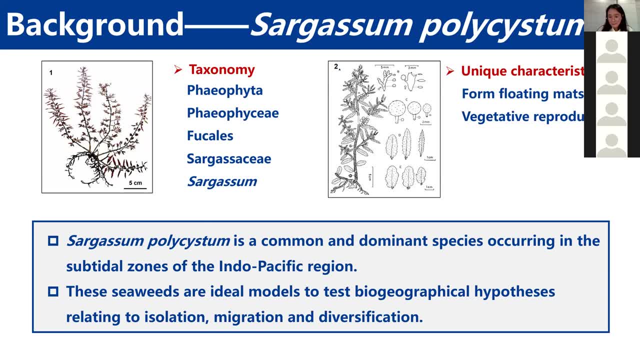 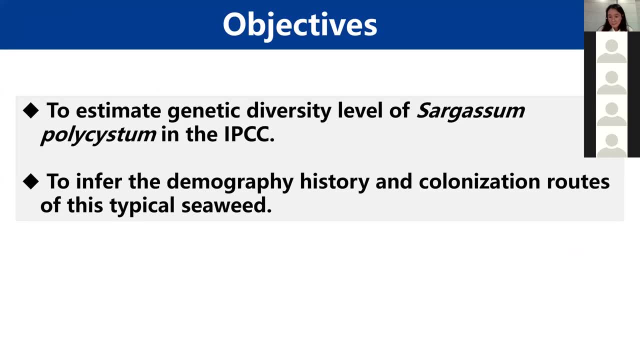 relating to isolation, migration and diversification. So in So, in our work have two main objectives. One is to estimate genetic diversity level of this seaweed. The other is to infer the demographic history and the colonization rules. 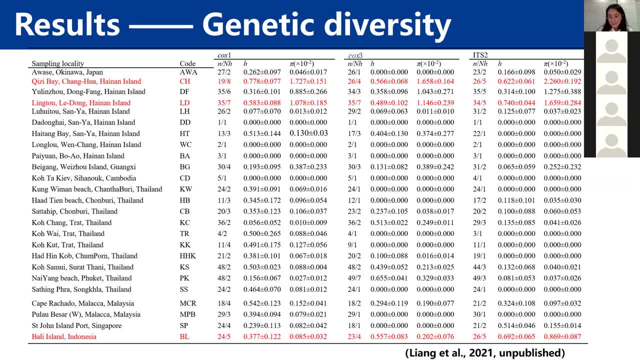 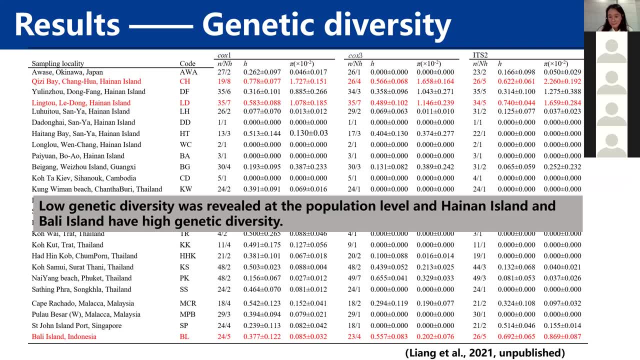 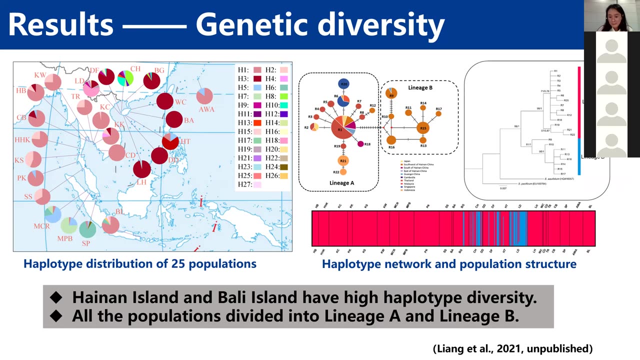 In our study we examined two important genetic diversity indices to evaluate the genetic diversity level. The results show that low genetic diversity was revealed at the population level, But Hannah Iceland and Bali Iceland have high genetic diversity. Furthermore, we also examined 27 haplotypes in all cow populations. 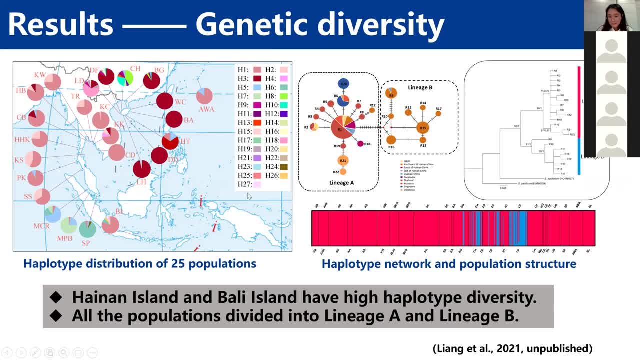 This figure shows the haplotype distribution. Different colors represent different haplotypes. From this figure we can say that Hannah Iceland and Bali Iceland have high haplotype diversity. Then we also construct haplotype network and conduct population structure analysis. 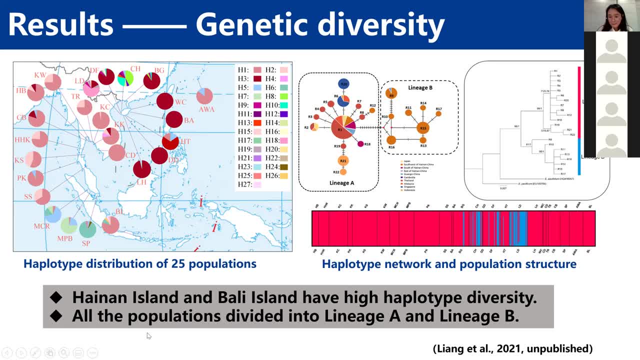 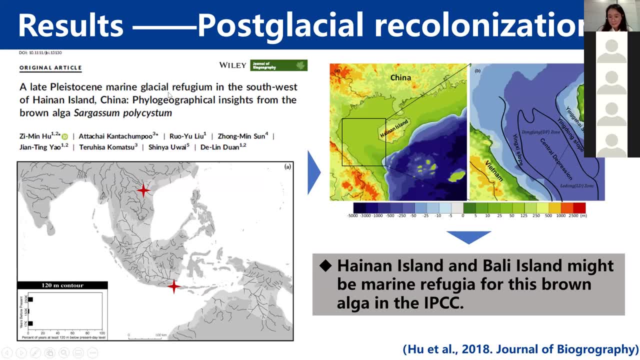 All these results show that all the cow populations divided two genetic lineages. As we know, glacial refugia is the area where animals and plants could survive during glaciation. Our previous work supported that: Hannah, Iceland, and Bali, Iceland, might be marine refugia for this brown alga. 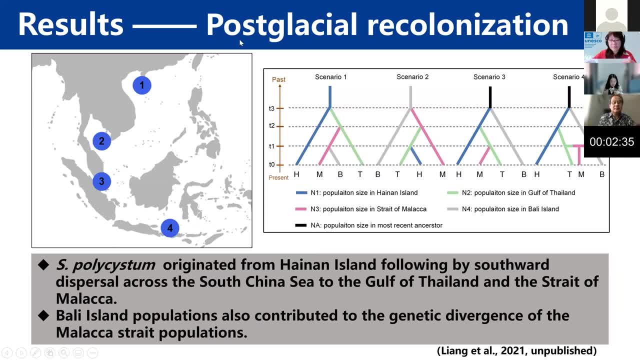 So in this study we want to investigate post-glacial reorganization process. So we designed four evolutionary models to test the reorganization rules. The results show that this cap was originated from Hannah, Iceland, following by Southward Disposal across South China Sea. 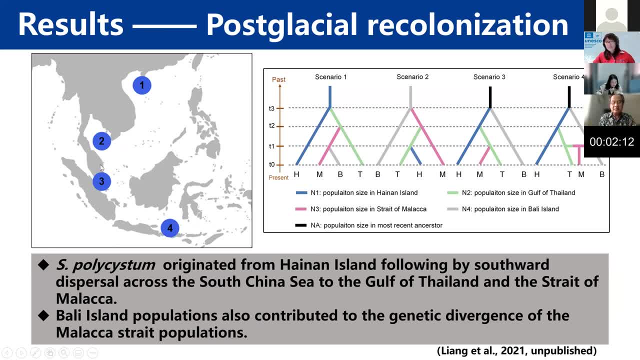 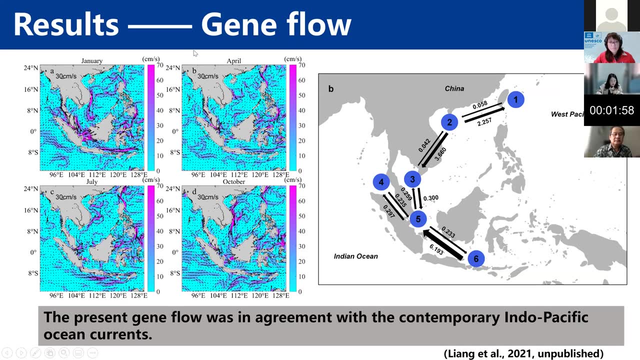 to the Gulf of Thailand and the Strait of Malacca. Besides Bali, Iceland population also contributed to the genetic divergency of Malacca Strait populations. Then we want to examine how ocean currents influence the gene flow between different cow populations. 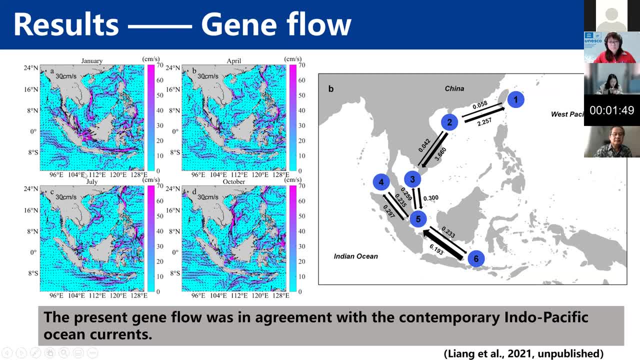 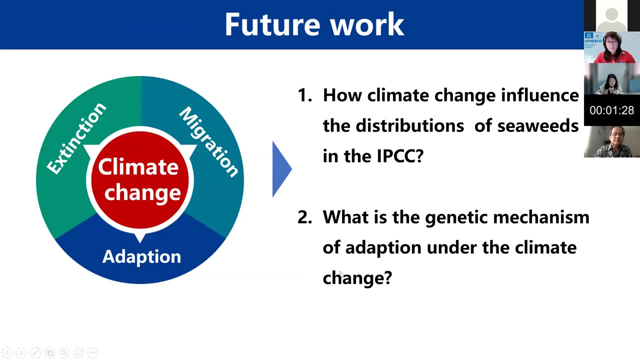 The left figures show the ocean current patterns in Indo-Pacific region. The right figures show the gene flow between different populations. All these results show that the present gene flow was in agreement with the contemporary Indo-Pacific ocean currents. Sorry, As we know, there are three common responses to climate change for marine species. 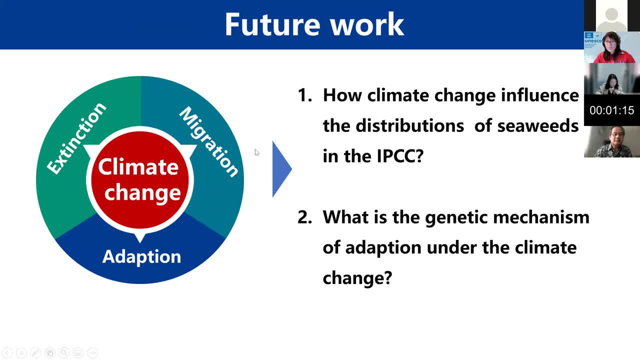 One is extinction, migration and adaptation, Then our future work will focus on two main objectives. One is how climate change influence the distribution of species. The other is what is the genetic mechanism of adaption under the climate change. Special thanks to our team. 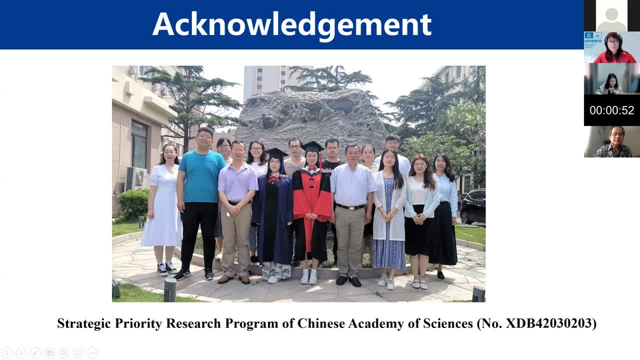 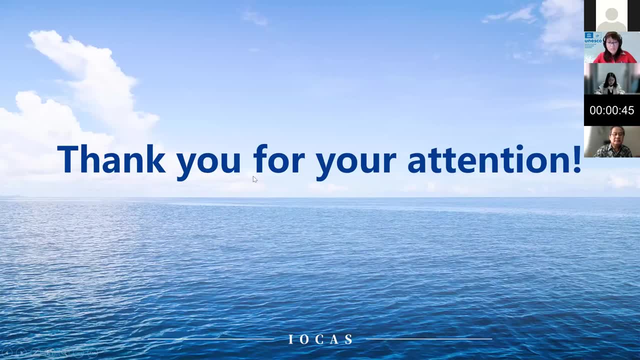 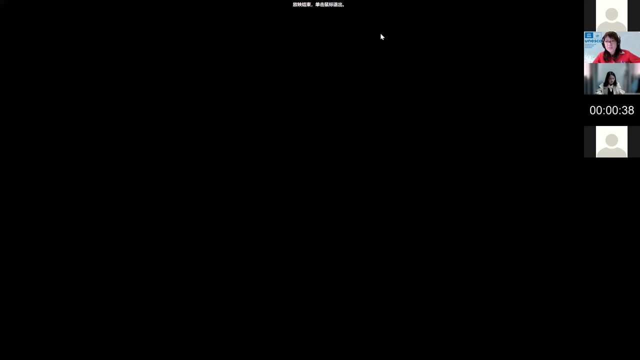 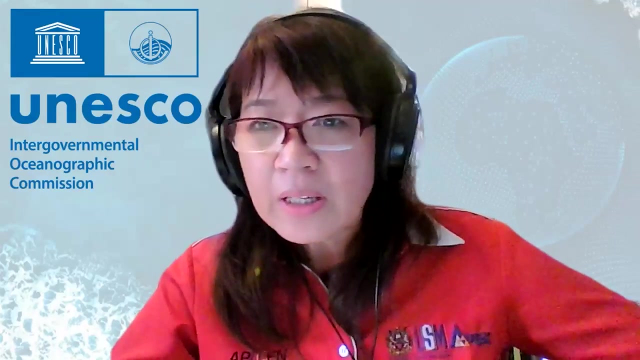 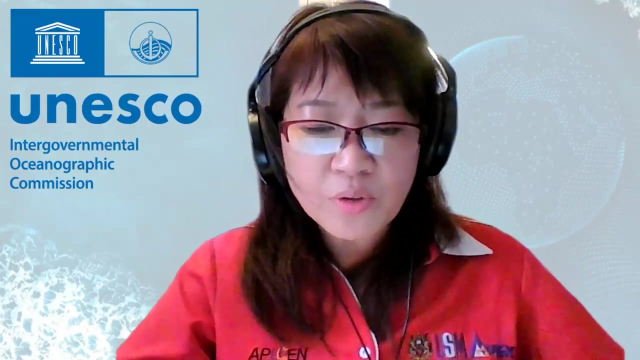 And this work was supported by Strategy Priority Research Program of CAS. Thank you for your attention, Thank you. Thank you, Jie-Zhang. Thank you very much for your presentation and keeping to the time. Very good presentation. Now, since Christian is not here, we will invite the third speaker, Dr Yong-Gwan Yuan. 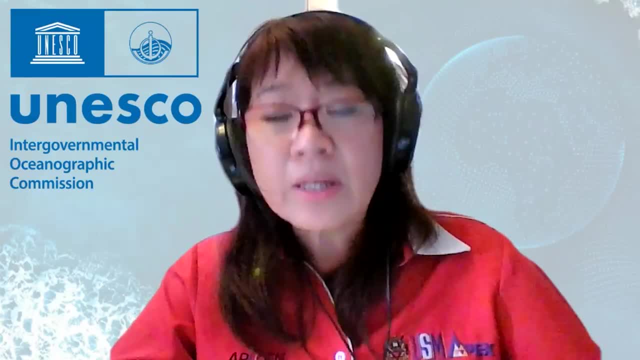 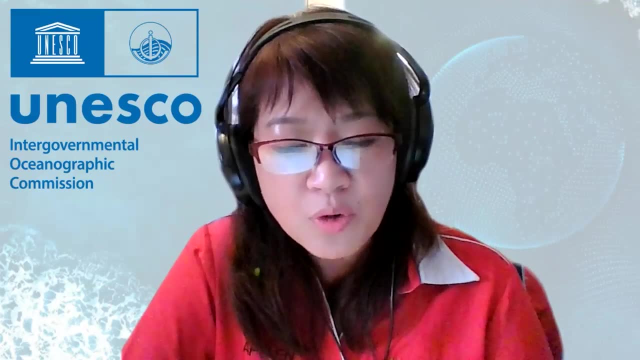 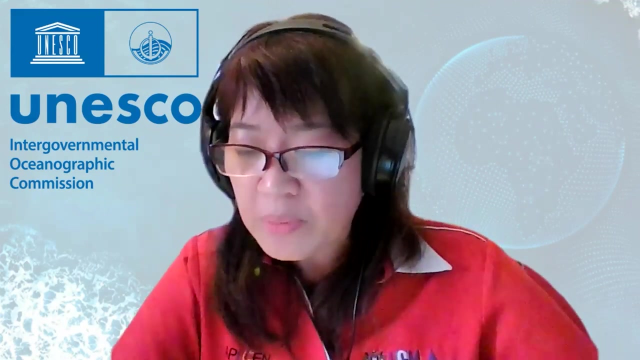 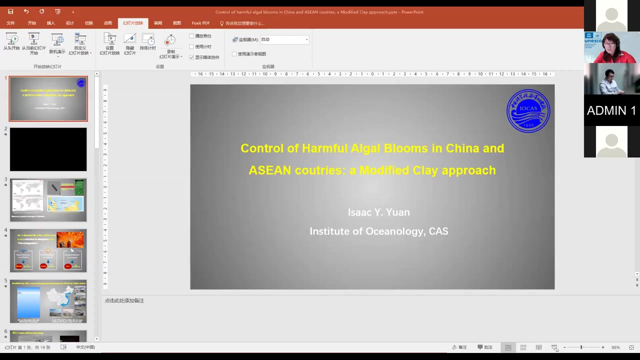 Associate Professor from Institute of Oceanography, Chinese Academy of Science. His expertise- Dr Yongguan Yuan's expertise- is on coastal eutrophication and harmful algae blooms. His title is Mitigation of Harmful Algae Blooms in China and ASEAN Countries: a Modified Clay Approach. 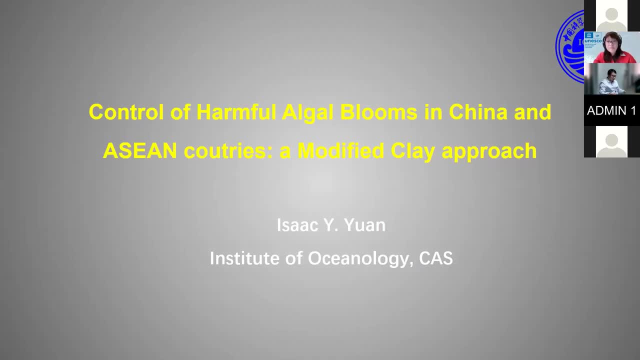 Over to you, Dr Yuan. Yeah, thanks, Thanks for you, Aileen, And just call me Isaac for your convenience. Okay, yes, Yeah, I'm for you, IUCS, And today I'd like to share a story about the harmful algae blooms control. 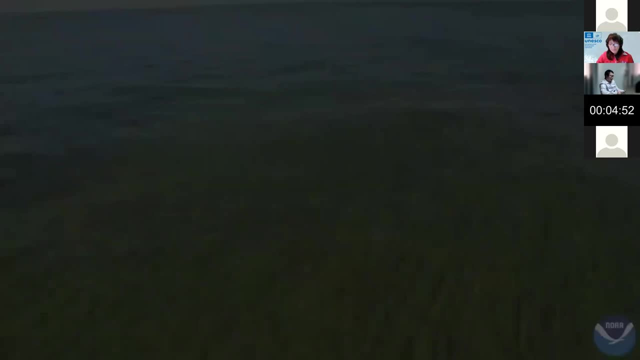 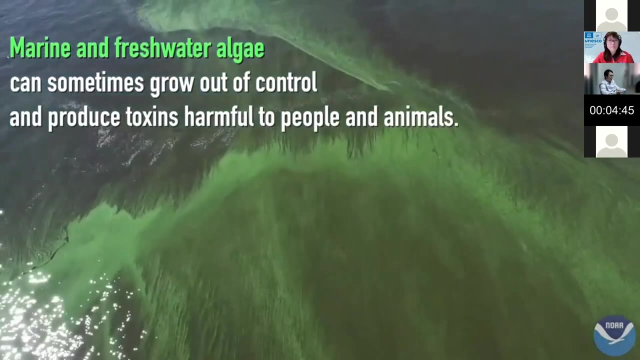 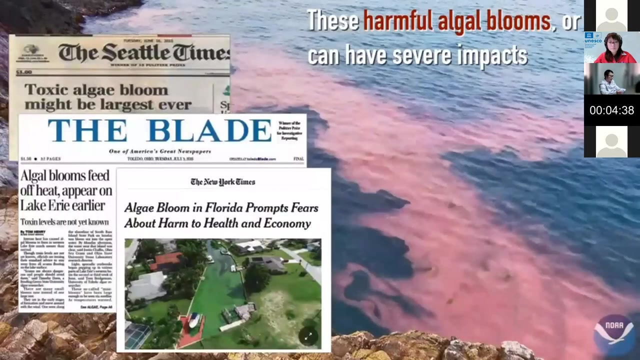 Well, let's start with a short video. So we know that the marine, the freshwater algae or phytoplanktons, sometimes grow out of control And this phenomenon we call the harmful algae blooms. It could have several negative impacts to the human health. 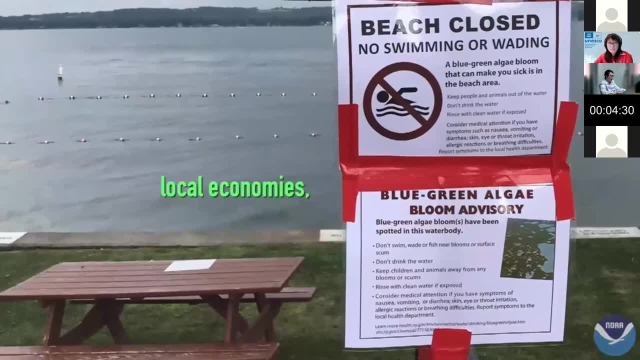 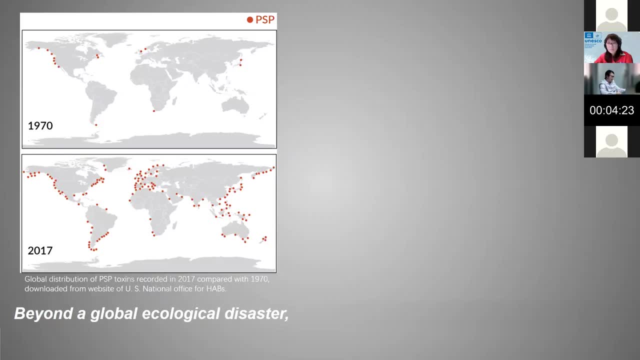 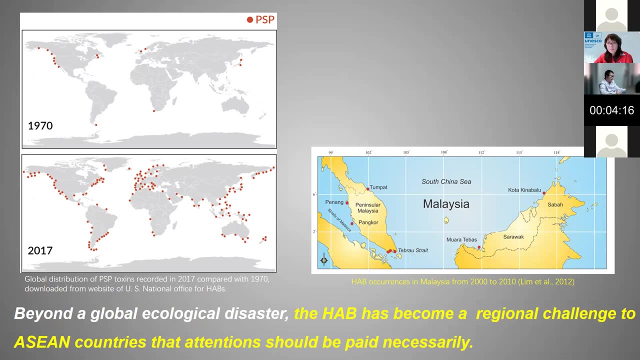 For example, it could be harmful to the environment, to the animals or to the local economies, such as the aquaculture, and to the biodiversity. Well, it's a global ecological disaster but, more important, it has been a regional challenge in the IPCC area or in the Asian countries. 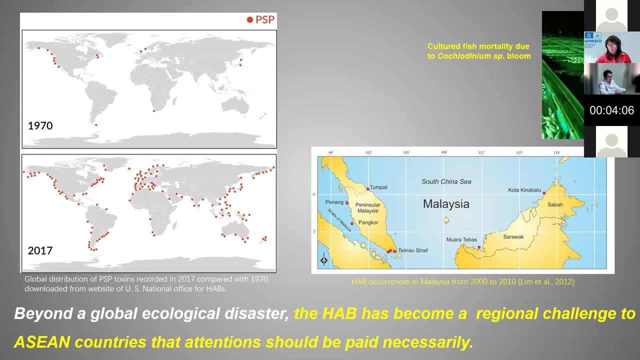 For example, the hapst caused by the crocodilian often induced some cultural fish molluscs, And this is the case in Malaysia last year along the coast of Penang. So the hapst is a disaster just like a fire. 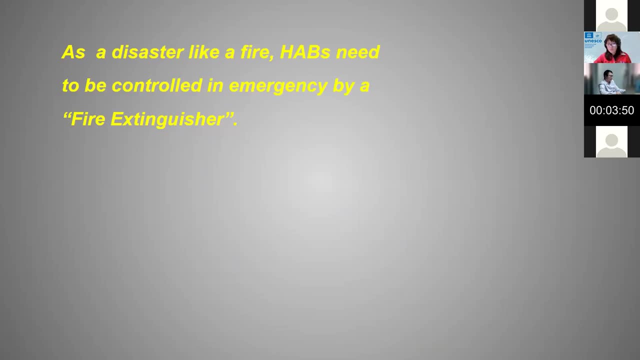 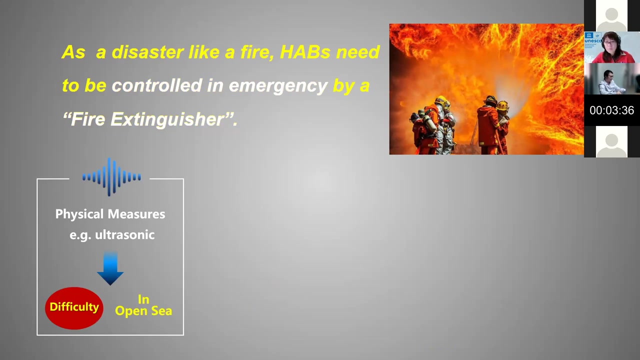 So to a fire, we have to do something and have something in our hand. We call it the fire extinguisher, or let's say some emergency control strategies. So in theory, there are several approaches that could be used to treat hapst. 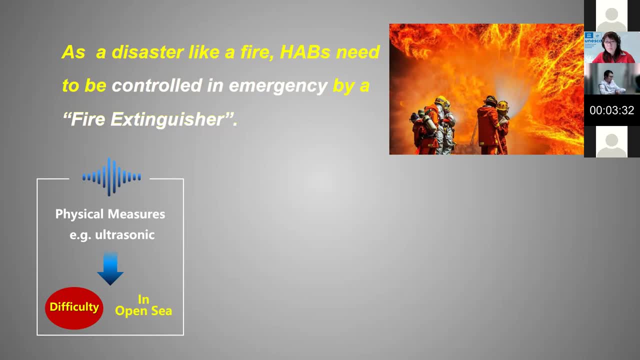 For example, we could use ultrasonic. So in theory there are several approaches could be used to treat hapst, For example, we could use ultrasonic. So in theory there are several approaches could be used to treat hapst, Or some physical measures. 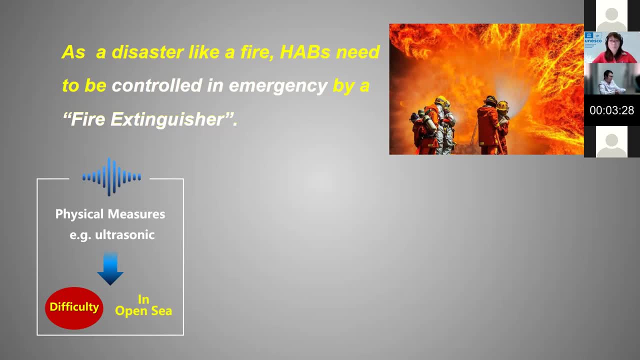 But you know, the hapst in the field is often dozens, hundreds or even thousands of square kilometers, So it could not be used in the open sea this kind of method, And people used to spray some chemicals like copper or algae cider into the field to treat hapst. 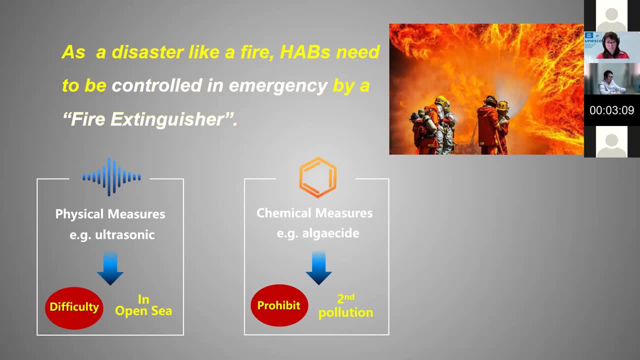 But it could induce the second pollution to the environment. So this kind of approach has been prohibited And people used to use some biological methods, but the effect is very slow So it could not be used in the field by now. In China we use a technology called the modified clay. 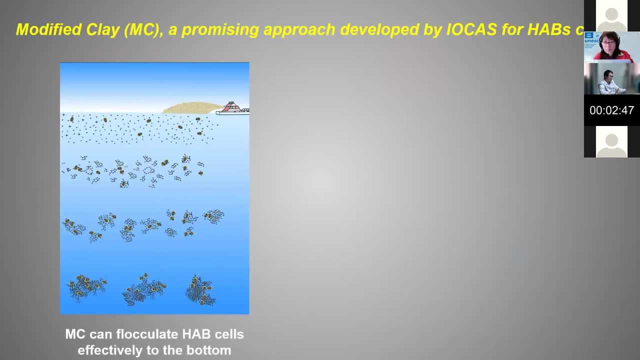 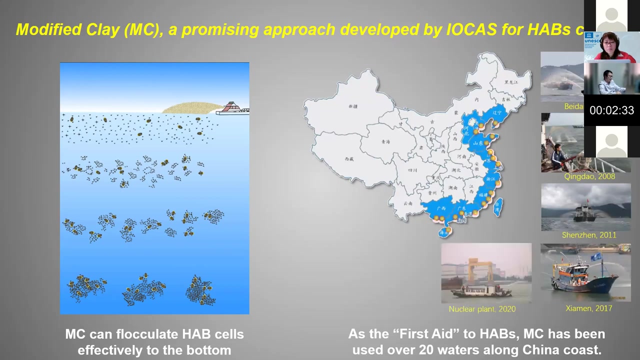 So the clay, the cells would be flocculated by the clay particles and settled down to the bottom. And it is very quick. And this method has been used along the China coast since 2012.. Since 2005.. It's a very promising technology. 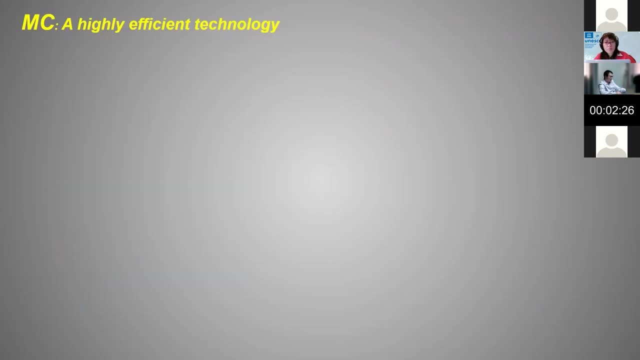 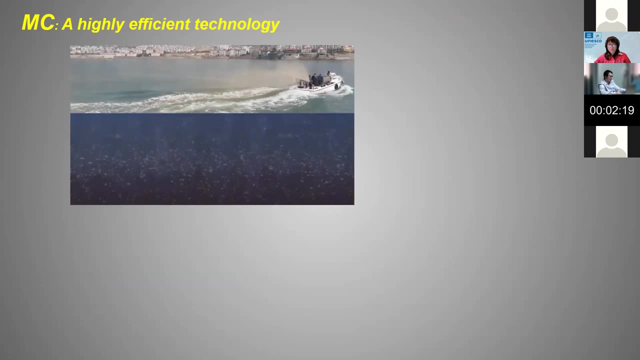 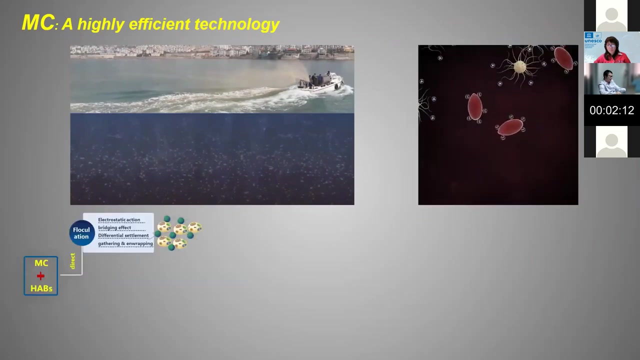 The advantage of it. initially, it's very effective to flocculate the hapst cells. Well, after spraying this MC into the field, the water becomes clean in maybe minutes or hours And in the microscope view the clay will flocculate the cells. 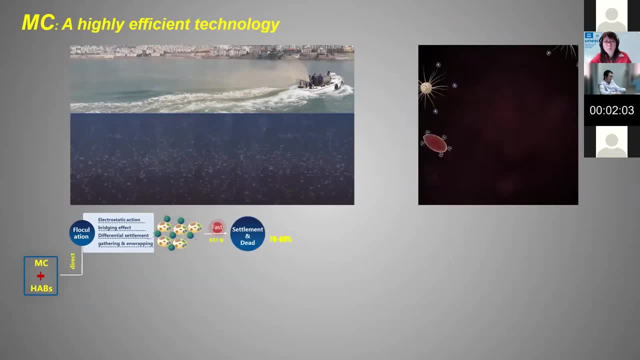 And settle them down to the bottom. And this action maybe takes only one hour or less than one hour, But this direct flocculations. maybe 70 to 80% of the cells would be flocculated to the bottom. And for the lucky residue cells in the water, well they will, just the growth of them will be inhibited. 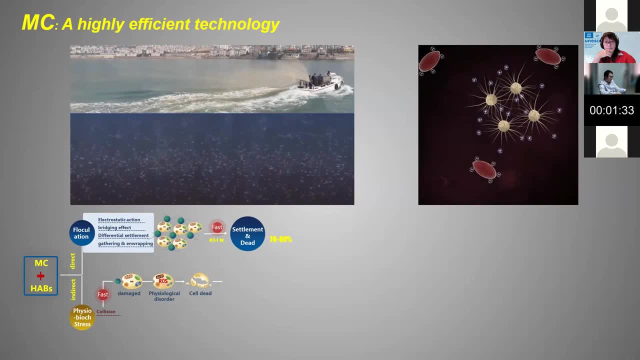 By the MC additions. Some of the progress is very fast And some maybe a little relatively slow, But it's the destination And by the growth of the cells will be inhibited by the MC addition. So the hapst could be controlled in the field. 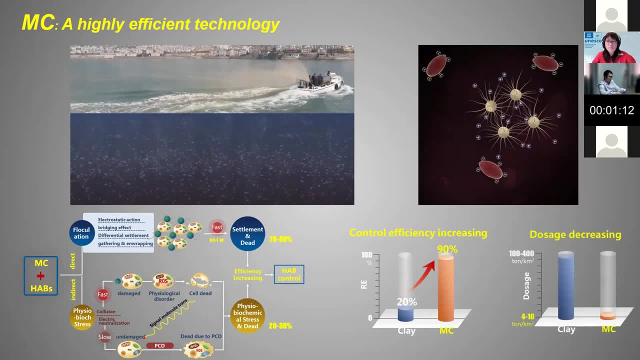 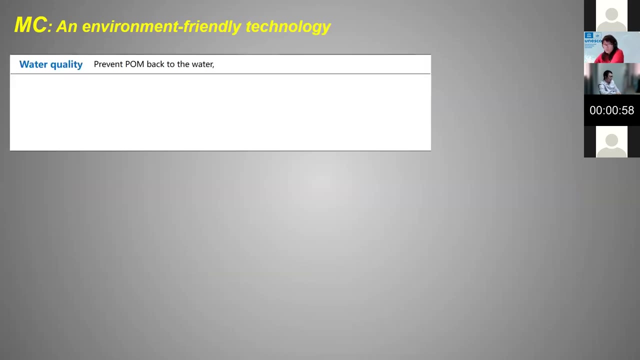 And the efficiency of this method is very okay And the dosage we use in the field It's only 4 to 10 tons per square kilometer. It's very low. And secondly, it's a very green technology. Well, the cells at the bottom to the cells at the bottom, the degradation of itself would be prevented by the MC additions. 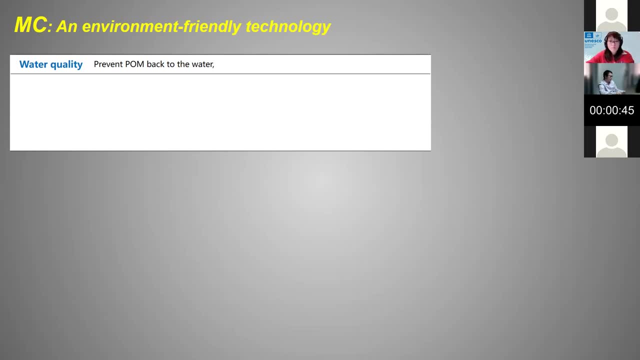 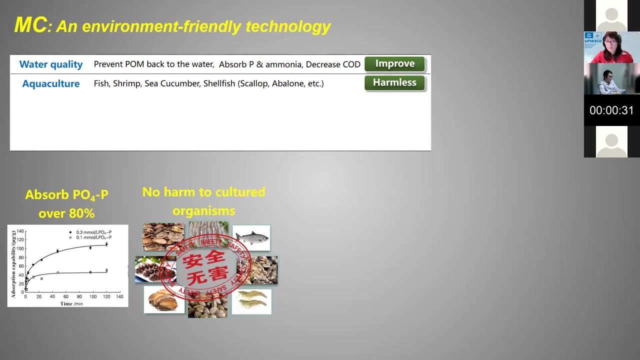 So it benefits the carbon burial And the nutrients in the water could dissolve, absorb, So the water quality could be improved. It is totally harmless to typical agricultural organisms like fish, shrimp et cetera. It could decline the toxins in the water. 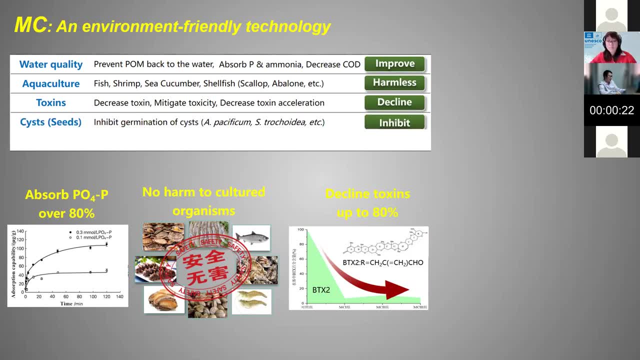 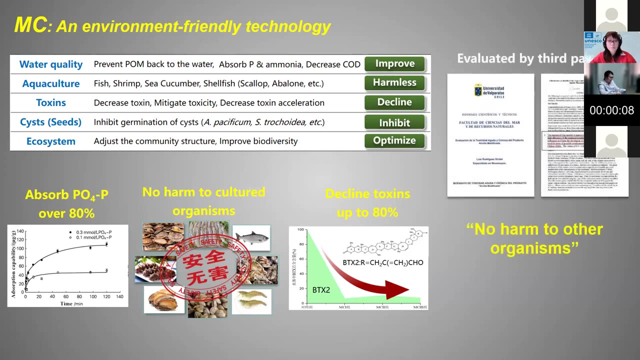 And inhibited the seeds, or maybe seeds of some specific species, And could adjust the community structure, Just optimize the ecosystem totally. And this material was further evaluated by Several third parties And it is indicated that no harm to the organism and to the environment. 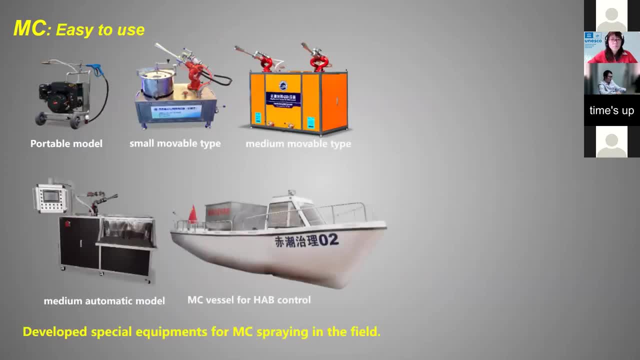 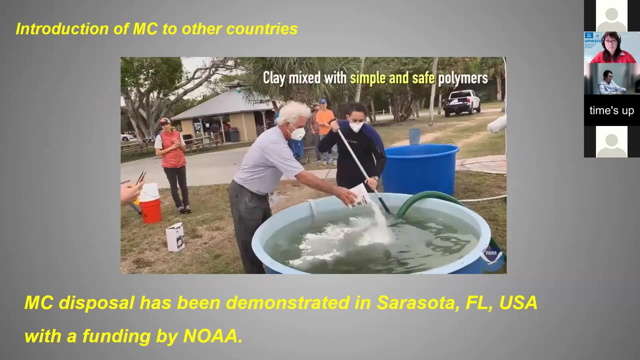 We also developed several types of the equipment that could be used to spray this material in the field. Some of them could be used in the culture ponds, And some of them is feed forward to be used in the open waters. In addition, this method is not only used in China. 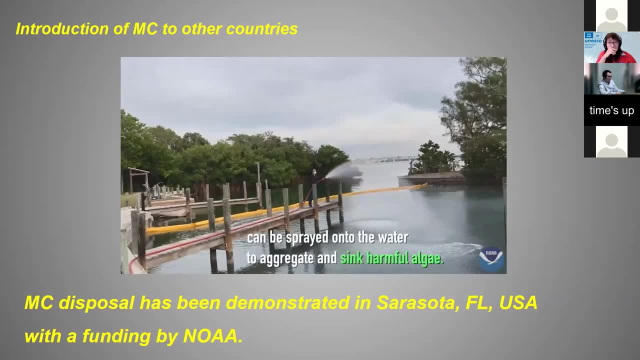 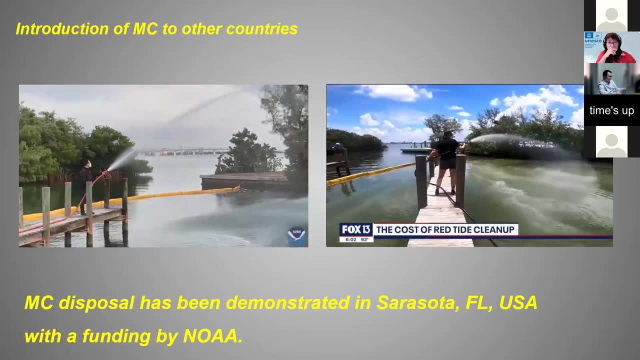 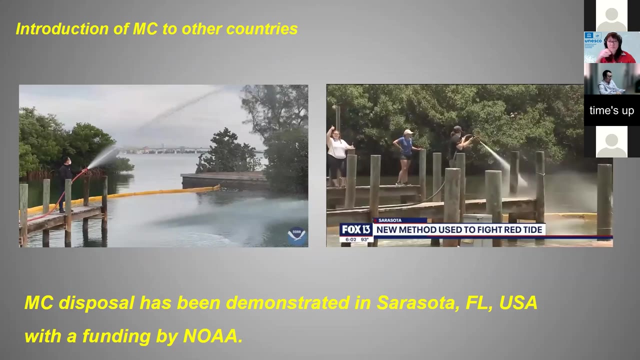 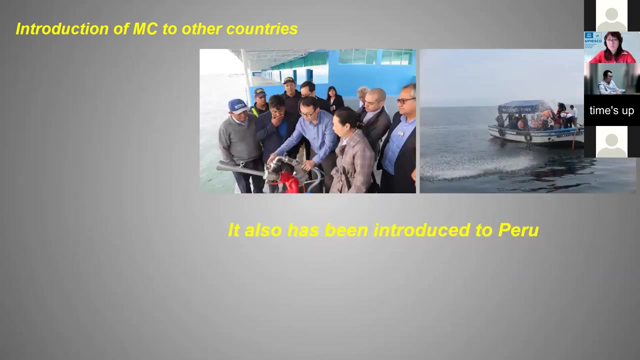 But also be introduced worldwide. For example, it has been demonstrated in the USA, In the Florida, So against the Florida. Well, perhaps there And such collaborations on the disposal of this method was just financial by NOAA and others, And we also introduced this method to Peru. 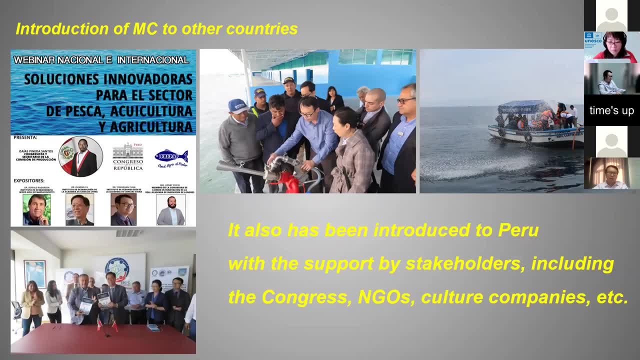 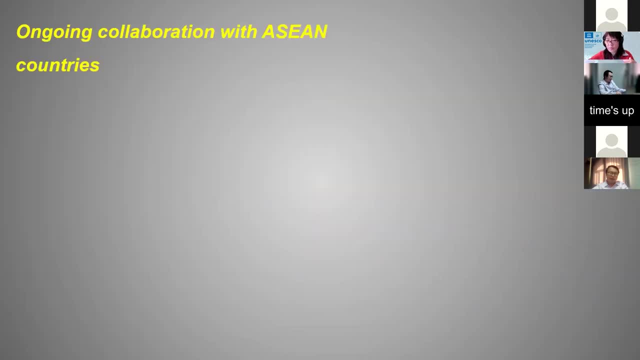 And such collaborations were supported by different stakeholders Like the National Congress of Blue NGOs And some cultural companies there. So can we use this? Is this method could be used, potentially, in the Asian countries? The answer is yes. I think This method is viewed by Princess Sherrington. 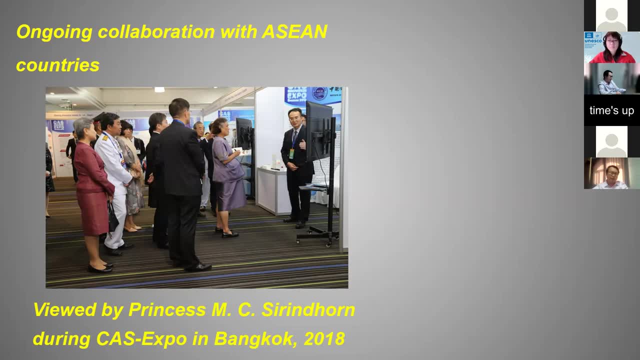 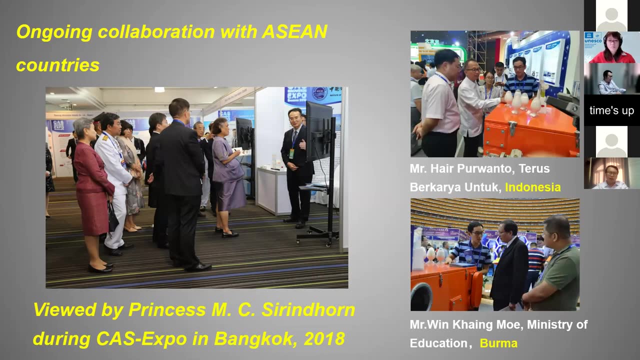 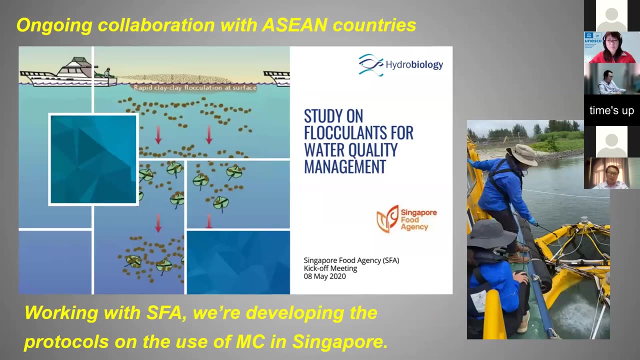 In Bangkok 2018.. During the CACS expedition And it is viewed by several officers from Indonesia, Burma and etc. By now, this method. we are working with the Singapore Food Agency, SFA, And to develop the protocols on how to use this method in Singapore. 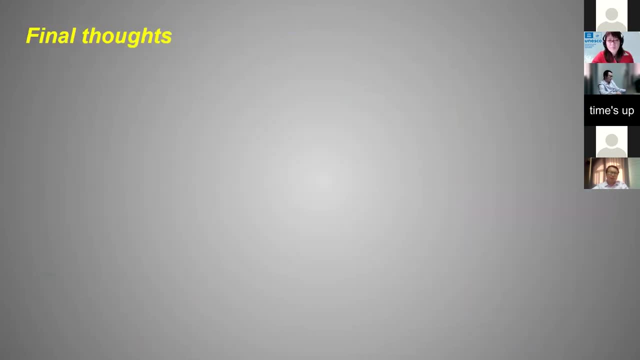 In the Johor Strait. So here we go, The summaries. So many types of disasters And should be treated as special disasters, And people, including the public authorities And the agriculture industries, They want some levels of CACS control. So is there any strategies to control CACS? 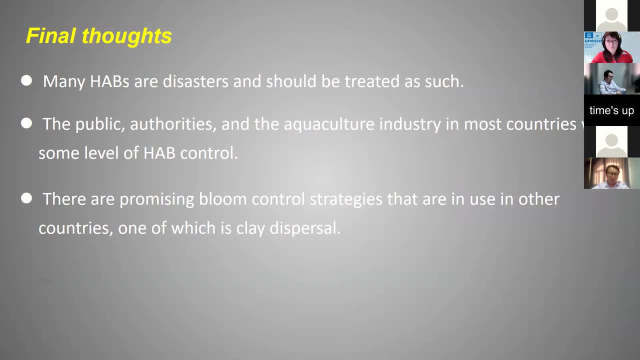 The answer is yes. There are promising blue control strategies in use in some countries- Maybe not in your country, But in some countries outside, So one of which is the curry disposal. In this area, MC, the modified clay, is widely used in China. 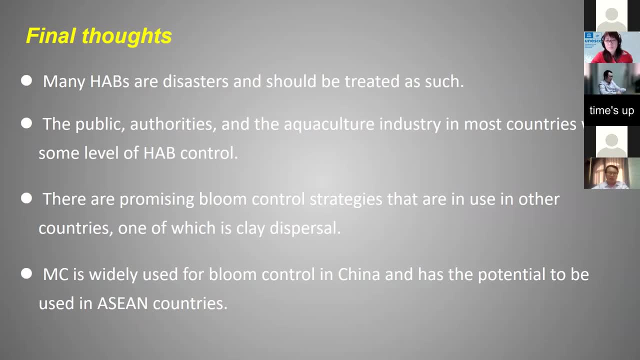 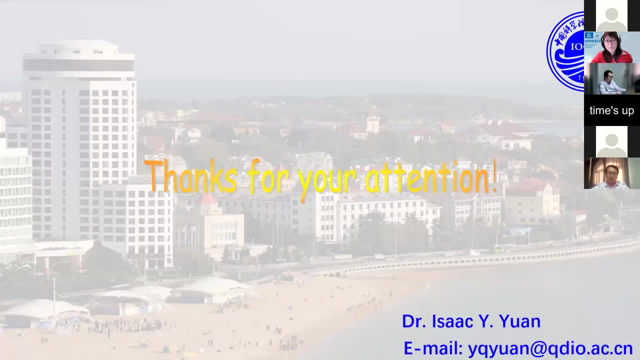 It's a promising technology And has the potential to be widely introduced in Asian countries. So here is my talk. Thanks for your attention. I'm Isaac And I could be reached by this address, Thank you. Thank you, Isaac, For your impressive presentation. 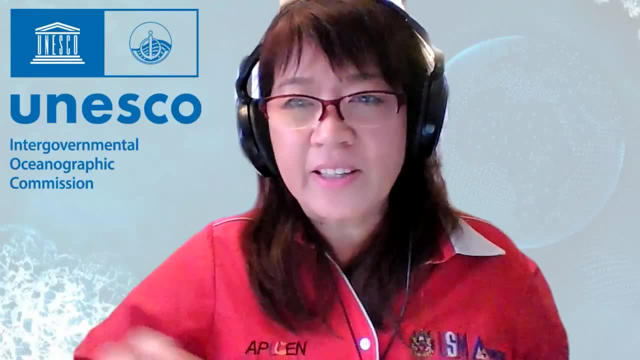 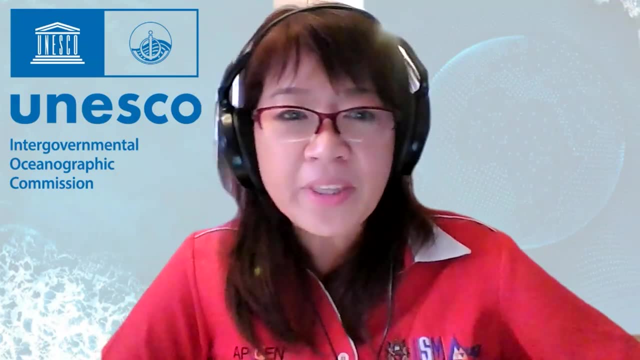 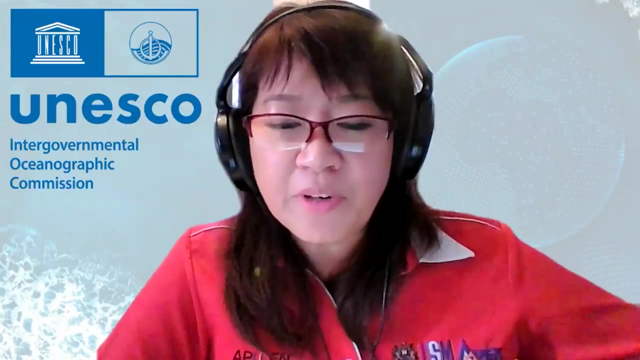 I'm sure there will be some questions for you later. Let's move on. We have found Dr Christian. I think he's here with us already. So again I'll introduce Dr Christian, An earlier career scientist from Wayanba University of Sri Lanka. 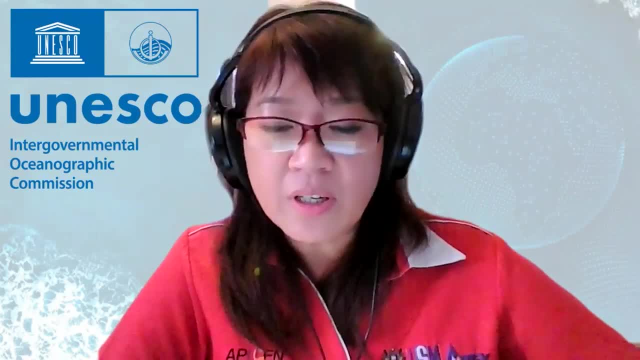 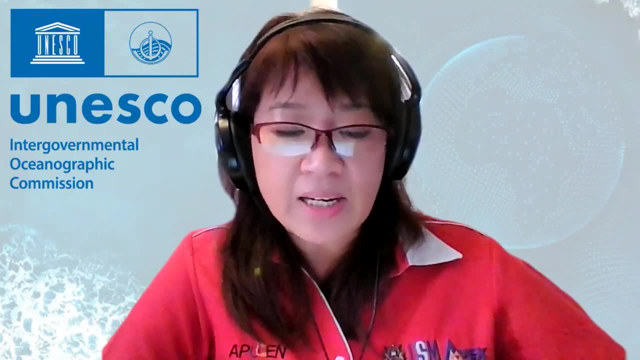 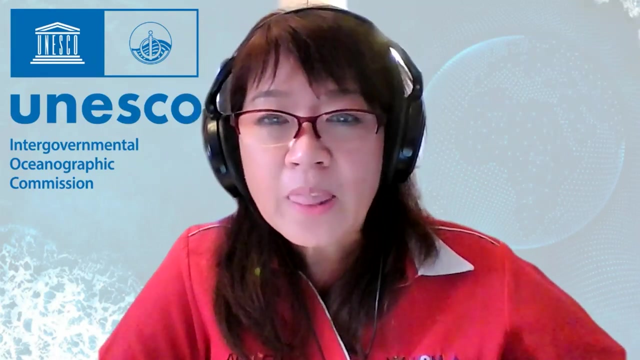 His expertise is in marine biology, focused on taxonomy, identification and present status of jellyfish resources in the coastal waters of Sri Lanka. His talk will be on the role of marine bio data in supporting industry. Over to you, Christian. Welcome back. Thank you, Professor. 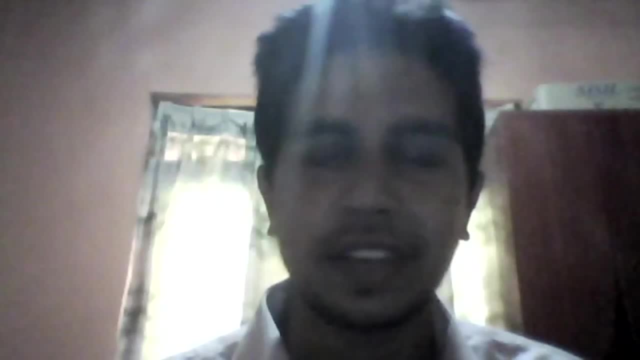 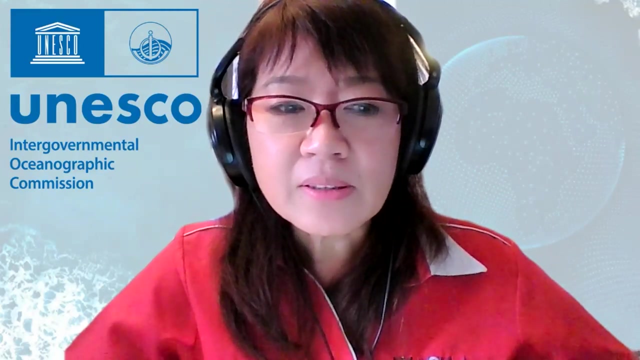 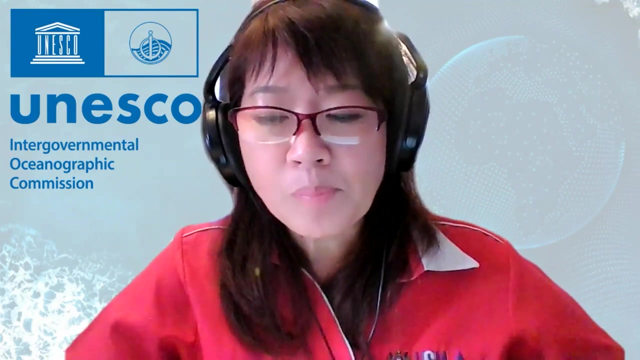 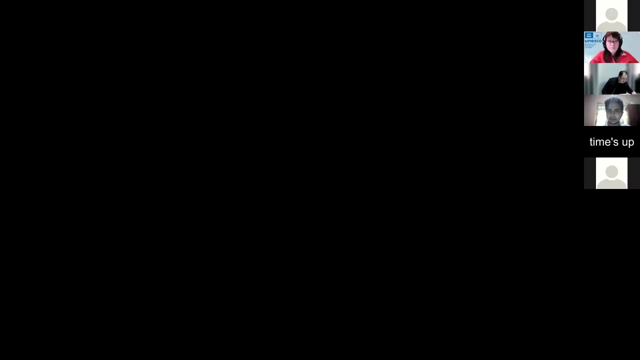 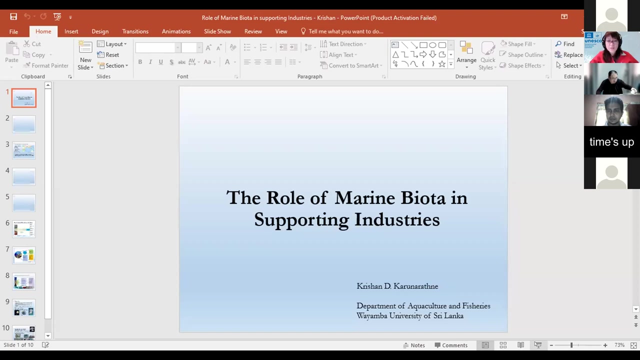 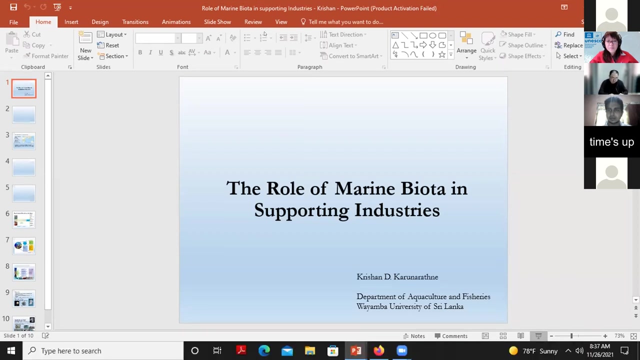 Thank you, Professor Eileen. Yes, There was a small technical issue So I couldn't participate on time. Do you have slides to share? Yes, Yes, please. Okay, We see your slides now. You just need to put it into slideshow. 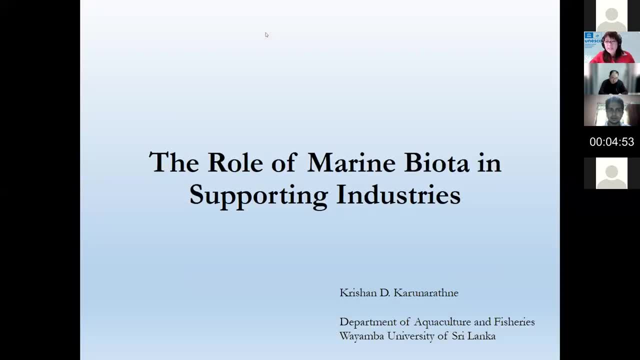 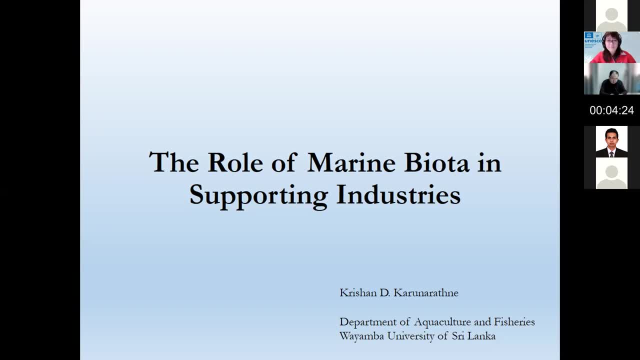 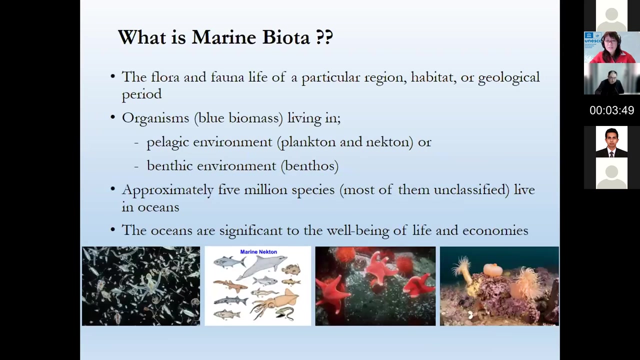 Okay. Yes, Your slides is not moving, Kishan. I don't know what's going on Now. it's okay, Okay, okay, Right. The plants and animals of a particular region is called a biota. The marine organisms economically called as blue biomass are pelagic or benthic. 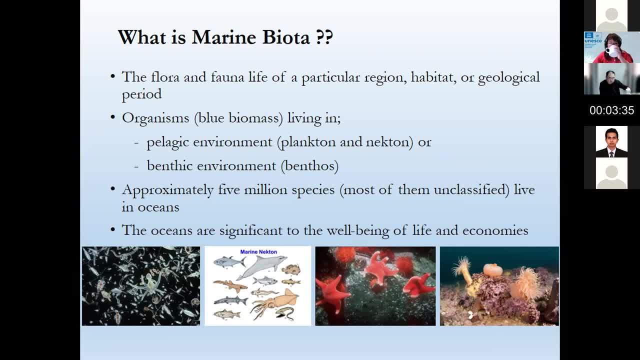 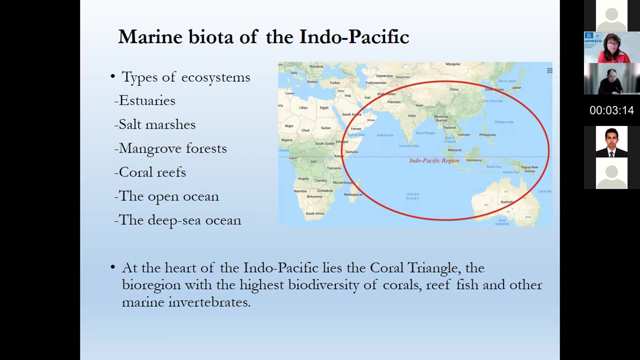 There are about 5 million species in oceans, but so far most of them have not been classified, And these oceans are really important to the well-being of life and economies. Marine biota in the Pacific is significant because it is the biodiversity hotspot in the world. 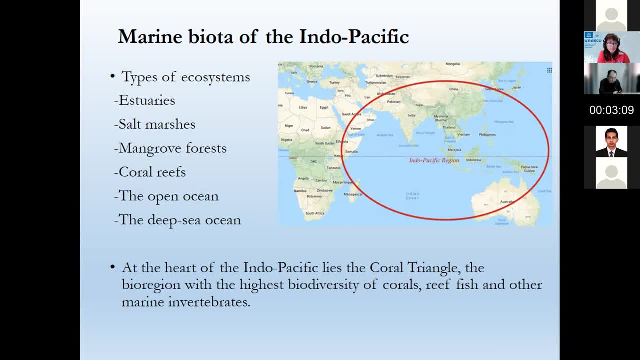 The Coral Triangle is also located here, And there are several types of ecosystems, like estuaries, short masses, mangrove, forests and open and deep sea oceans. A range of organisms dwells in these ecosystems, such as bacteria, fungi, other microorganisms, cyanobacteria. 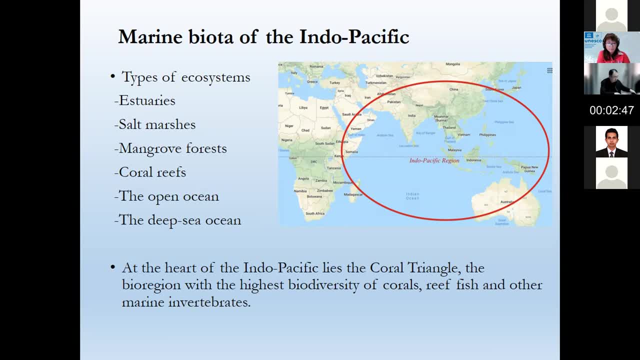 micro- and macroalgae, sponges, mollusks, other invertebrates, fish and plants are called as marine bioresources or blue resources. The sustainable use of those blue resources for economic growth improves livelihood and jobs while preserving the health of the oceans. refers to blue economy. 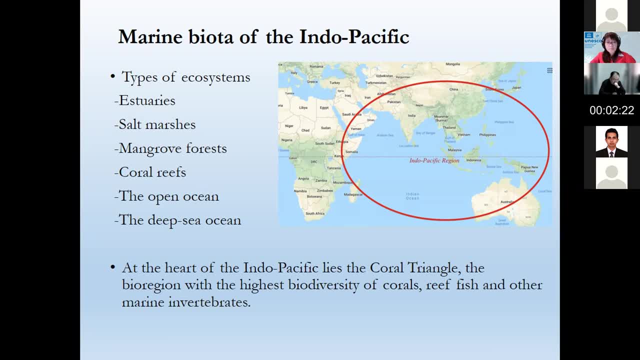 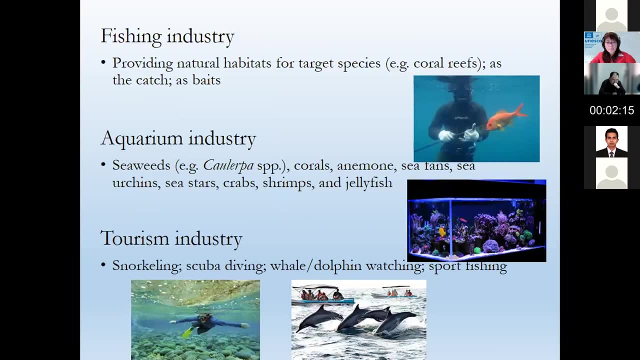 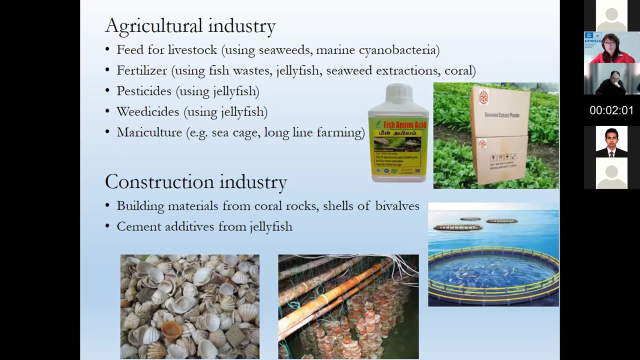 Thank you. As you know, the Indo-Pacific region is very popular for the several industries, such as fishing industry, aquarium industry and tourism. Also, various marine resources harvested from this region are important to produce feed for livestock, fertilizers, pesticides and natural resources. 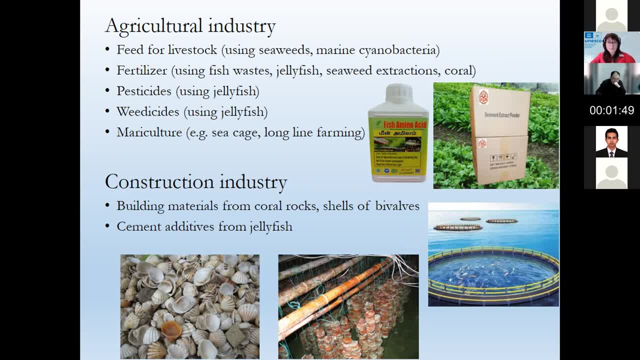 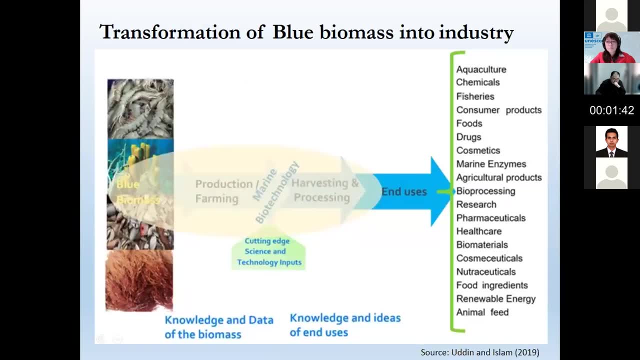 The building materials and cement attitudes are also produced by using invertebrates. The biotechnology that utilizes molecules and substances of marine origin refers to the blue biotechnology. The growth of the blue economy in the Indo-Pacific region could be enhanced on the European and Western part of the world. 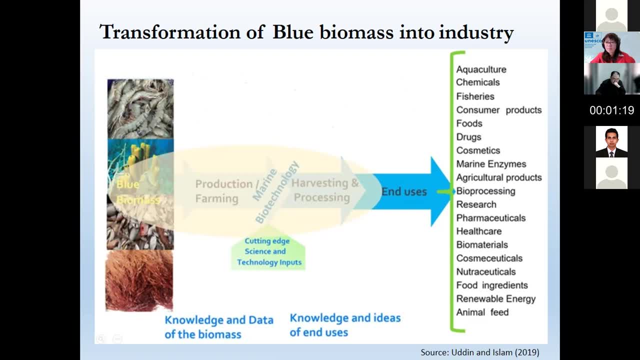 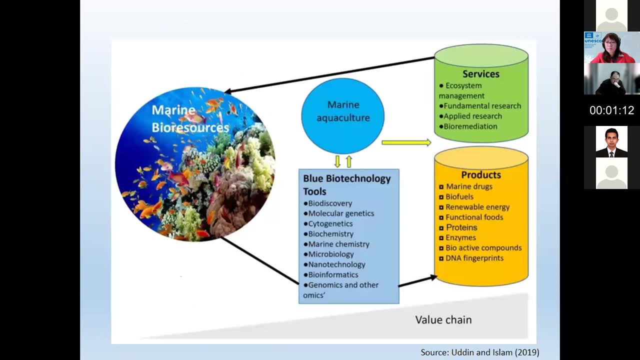 the transformation of marine bio-resources into food, medicine, animal feed and related bio-based items. The blue biotechnology can be applied for mariculture and highly valuable various products can also be produced, Incorporated services such as ecosystem management, both fundamental and applied research, and 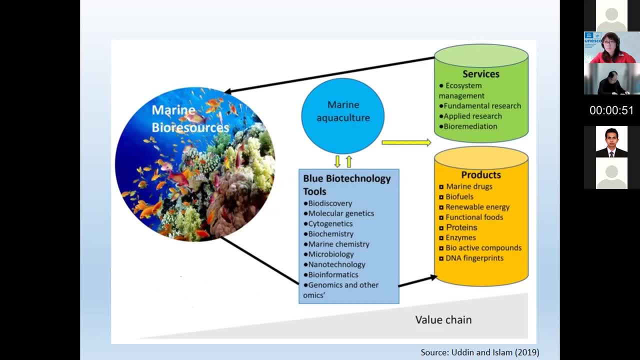 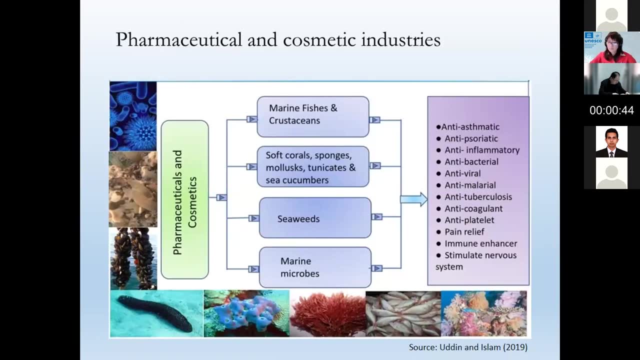 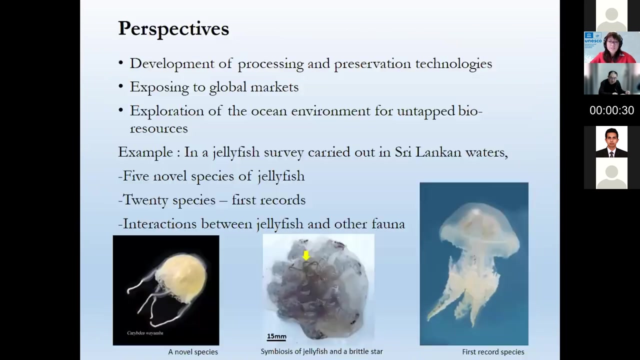 bioremediation can be used for sustainable utilization of marine bio-resources. The blue biotechnology is essential for the development of the pharmaceutical and cosmetic industries. Various kinds of therapeutic drugs are produced from marine bio-resources by using blue biotechnology. Perspectives of the blue economy in the Pacific. 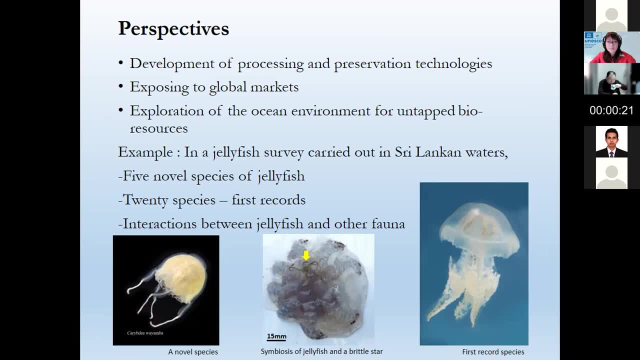 It should be upon the development of processing and preservation techniques of marine bio-resources. Also, the products should be exposed to global markets, And exploration of marine environment for NTEP or underutilized bio-resources is also essential. There is an example from Sri Lanka. 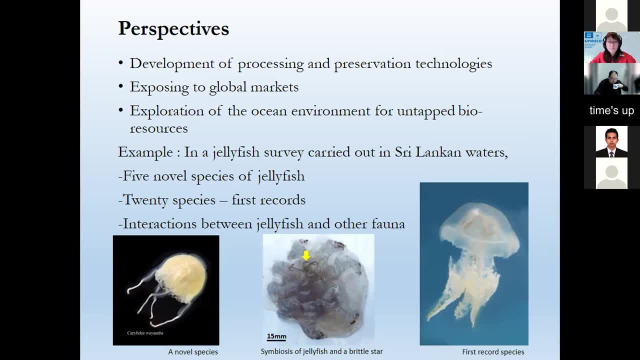 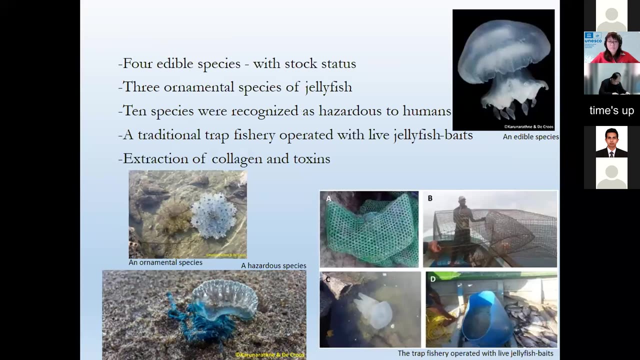 There was no comprehensive study on jellyfish resource in Sri Lankan waters. Thus we carried out a survey. A lot of Question, Another one minute. We obtained which were important: biology, fisheries, toxinology, some other applied sciences. Based on our findings, some other Sri Lankan researchers were able to extract some important 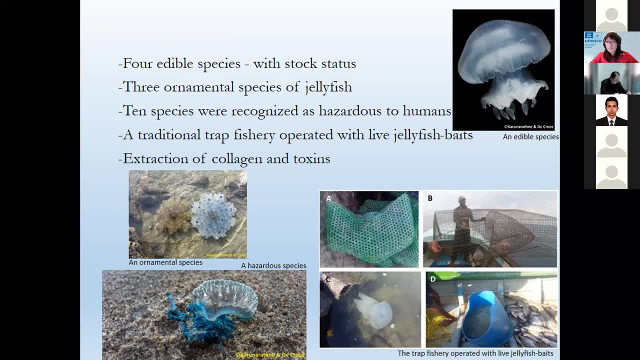 substance from jellyfish for the first time from Sri Lanka. By the presentation, I wanted to tell that exploring marine bio-resources is very important. We need to expand the industries and the economy of the Pacific nations. So thank you very much. Thank you, Christian. 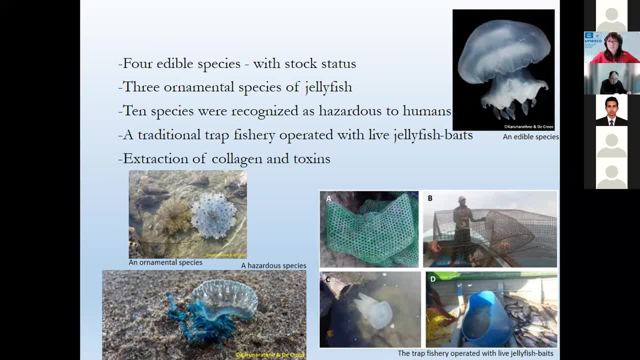 Thank you for your For keeping the time And, Okay, Let's, Let's move. Let's all of us move to the discussion. I would like to invite all the speakers and back on stage to us answer the Q&A session. 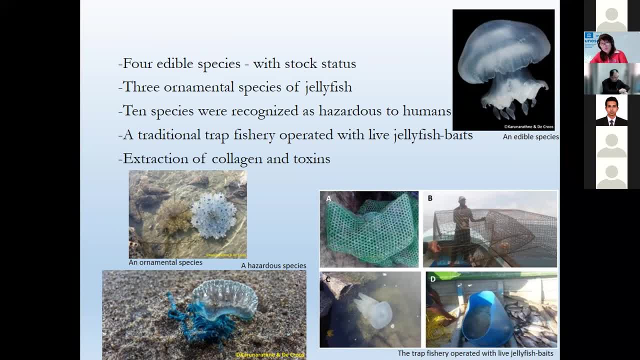 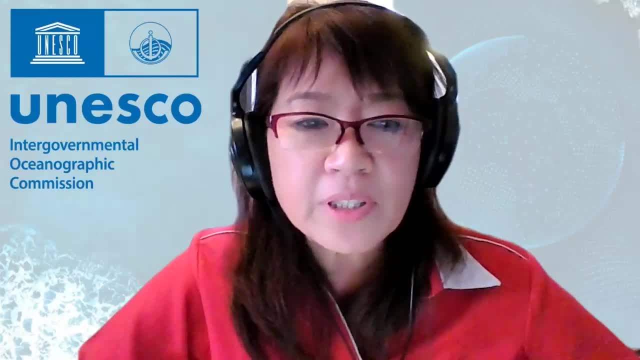 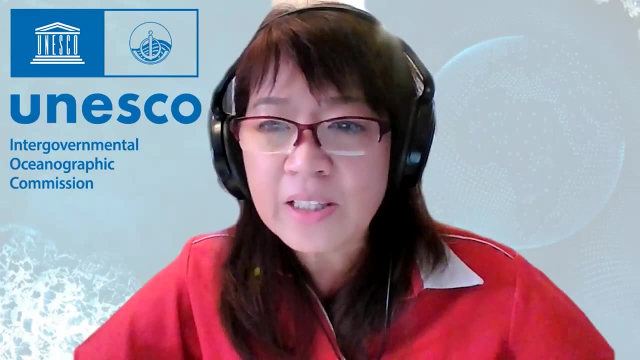 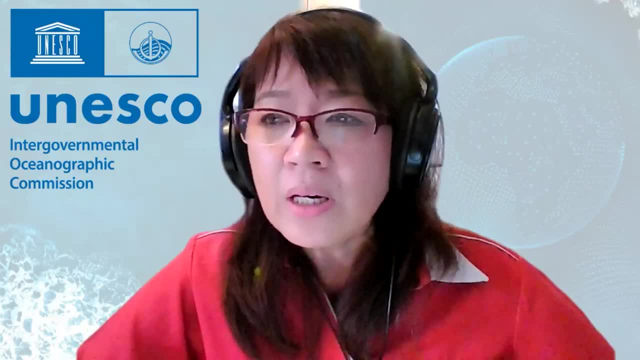 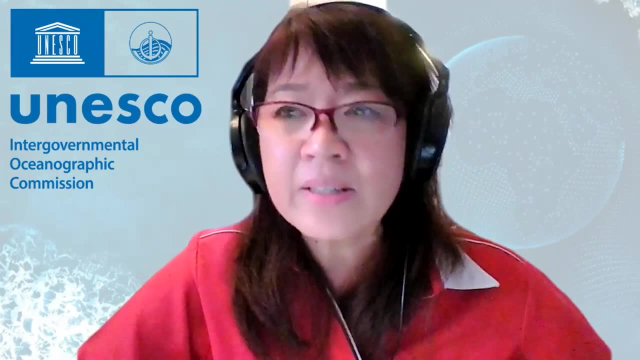 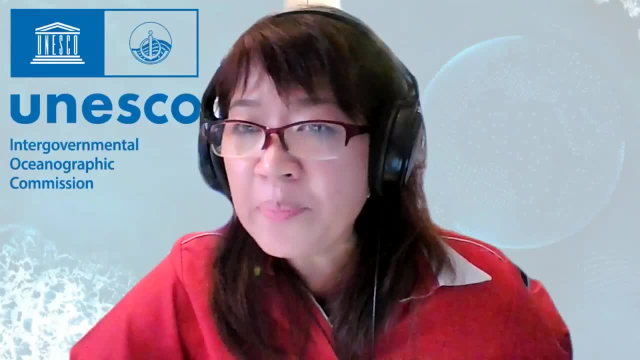 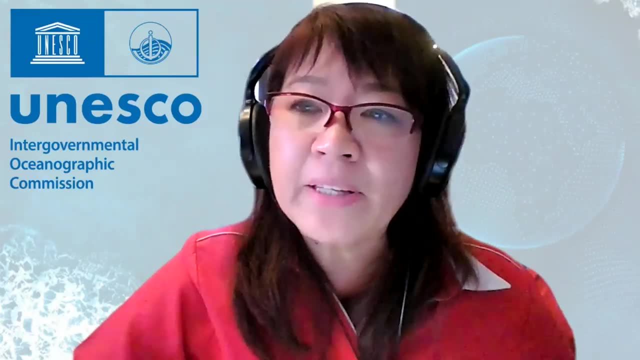 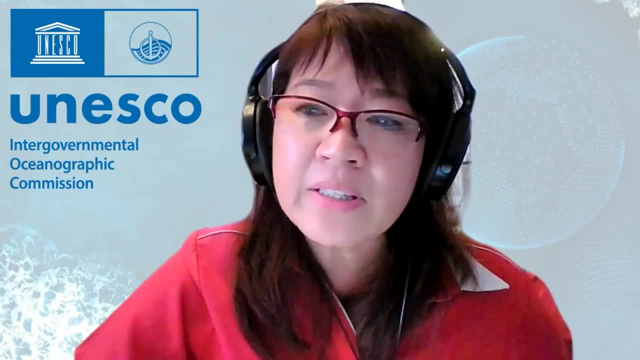 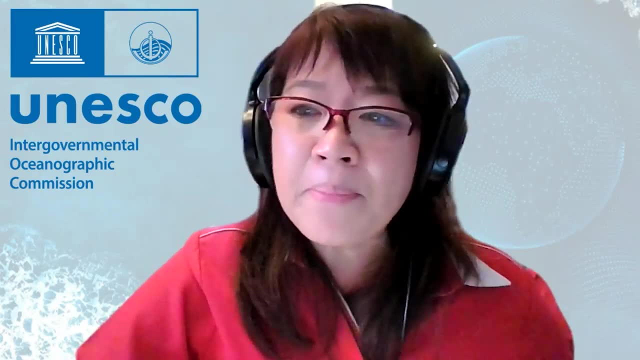 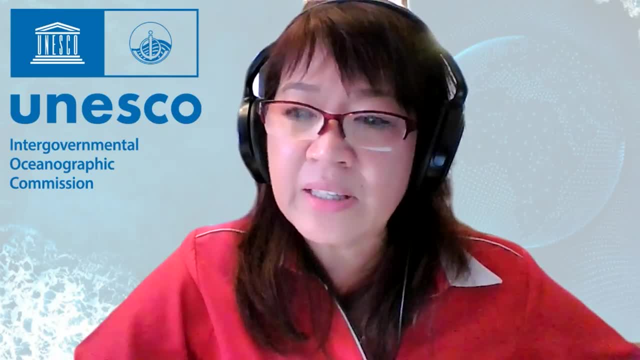 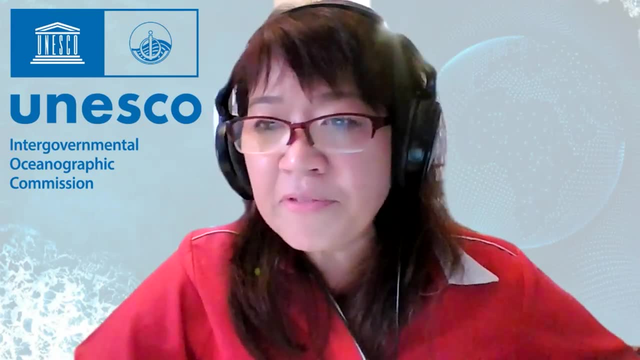 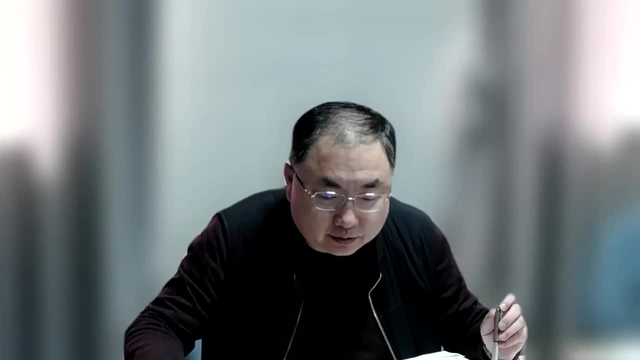 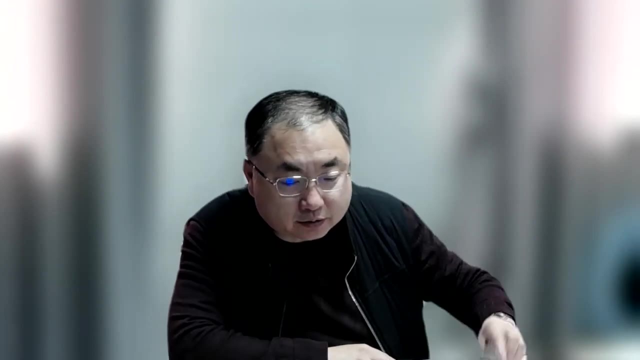 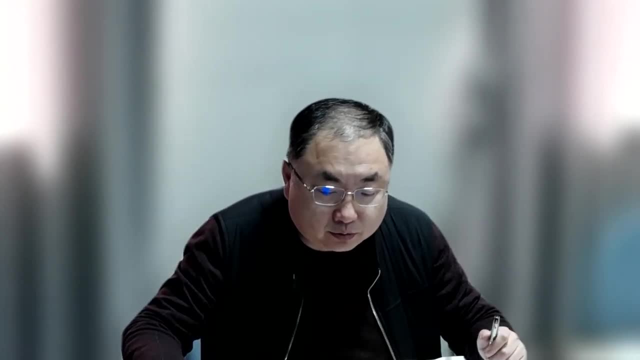 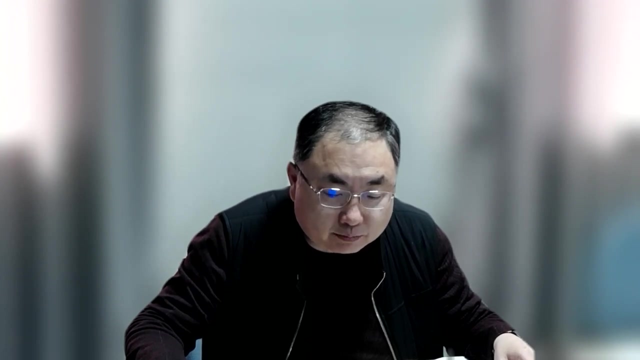 We will, We will and I do think, in the future, if we want to address this question, we need to organize some basic investigation with better coverage, not only in the coastal or the surface sea, but also some offshore area and subsurface, intermediate or deep layer sampling. 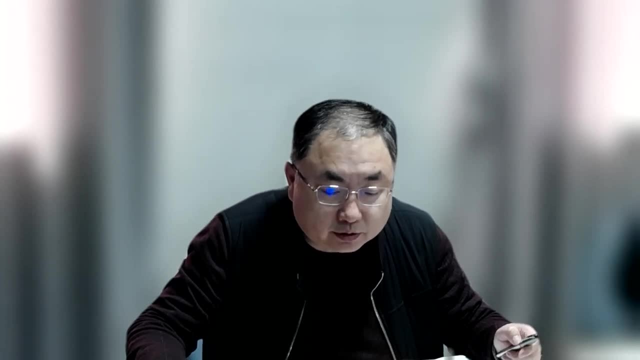 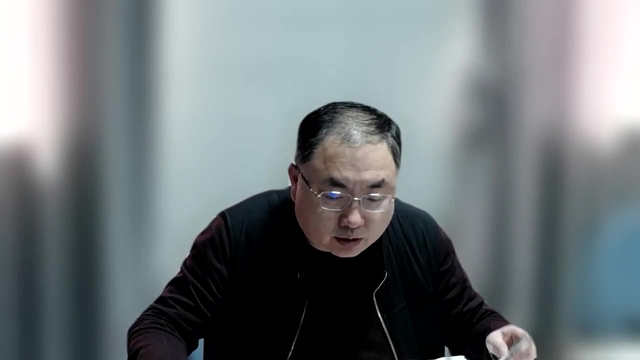 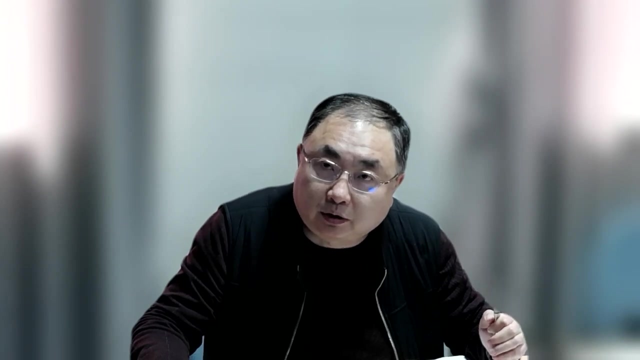 And also we should follow the international standards so we can combine the data and sample analysis results together from the different channels. And also I do think that our traditional method of sampling and analysis can hardly fill the gap of sampling the spatial and temporal sampling. 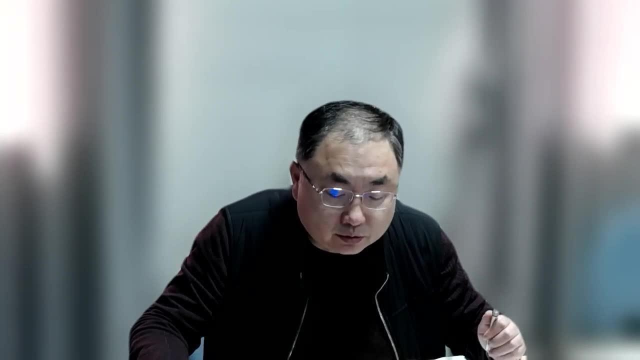 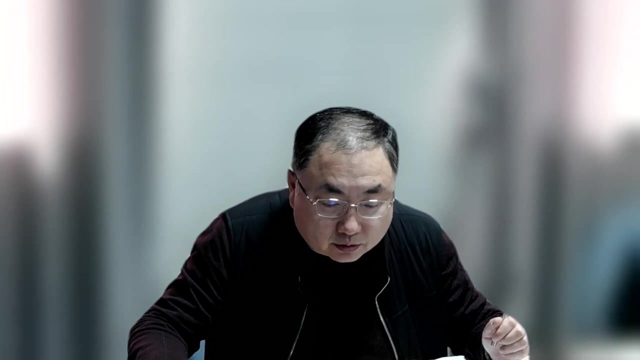 So maybe we need to use some new methods, such as the environmental DNA. We can use the water sample Sample to recognize or identify the species, instead of we have to use net or multi-layer net, which cannot give us enough sample. And also we can use the artificial intelligence analysis method to help us to establish the 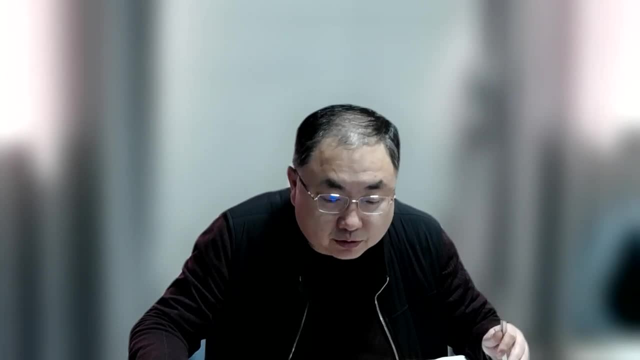 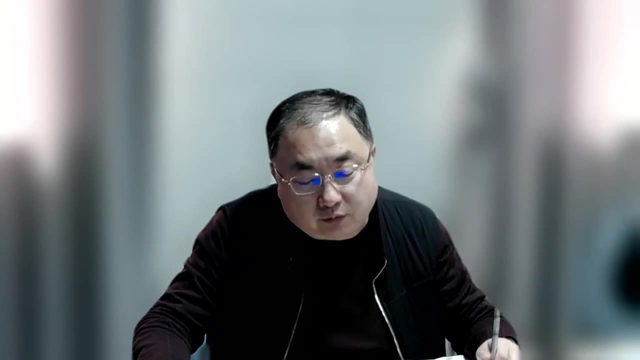 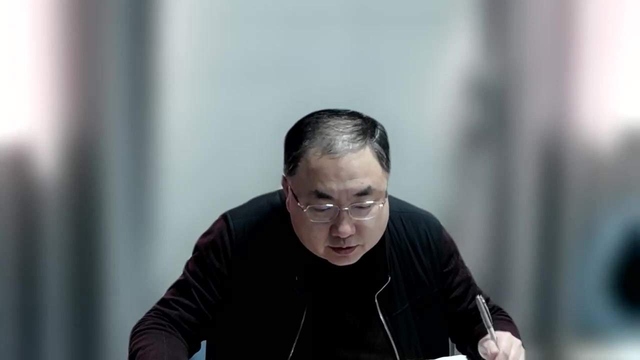 relationship. Okay, That will make the relationship between physical, chemical and biological—or ecological—parameters, And also, if we want to protect the future trend of the biodiversity pattern in using and outside of our region, we definitely need to develop a proper coupled model to give. 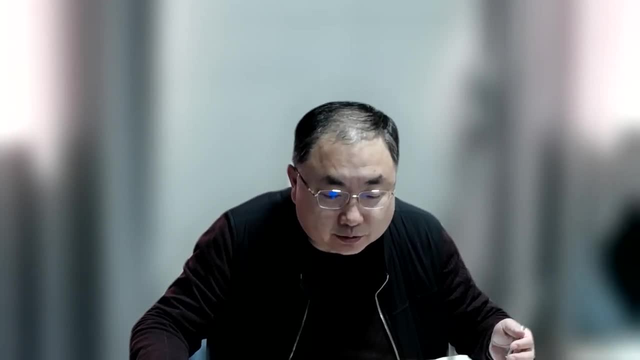 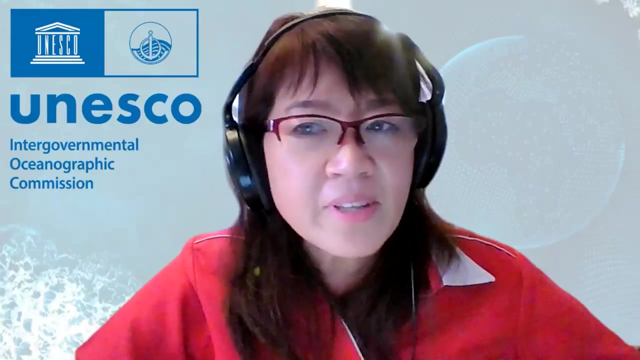 us a much more reasonable. Okay, I'll stop this scenario of the future environment change. That's my preliminary thoughts, Thank you. Thank you, Professor Wang. Let's move on. Is there any questions from the floor themselves? If you have questions, 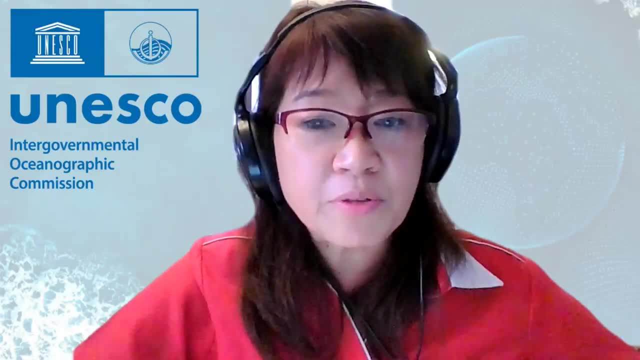 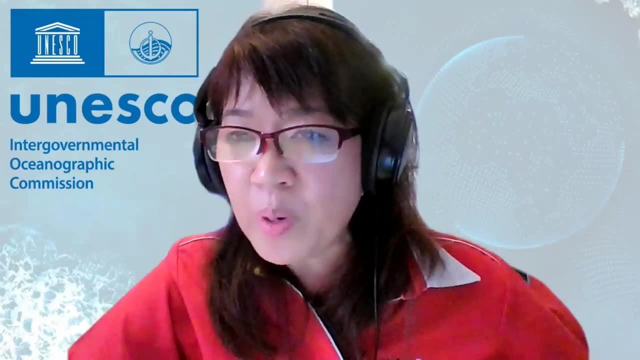 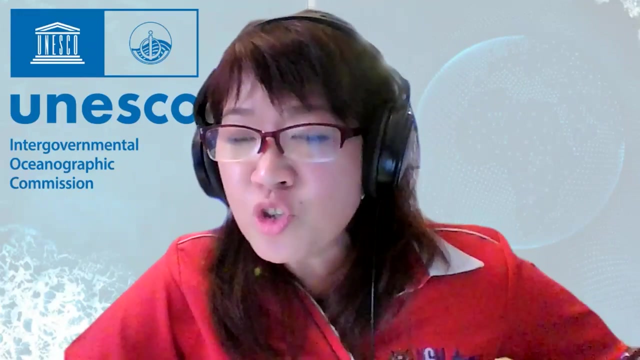 please raise your hand and unmute yourself to ask the question. While waiting for you to raise your hand, I will go back to the chat box. There's one for Isaac. Even though it has been answered, I think it would be good for Isaac to share it with the crowd. The question is: 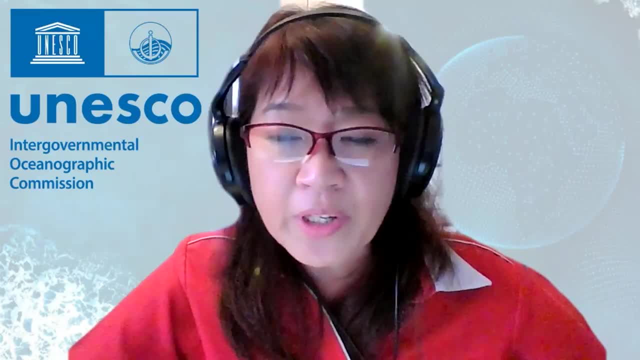 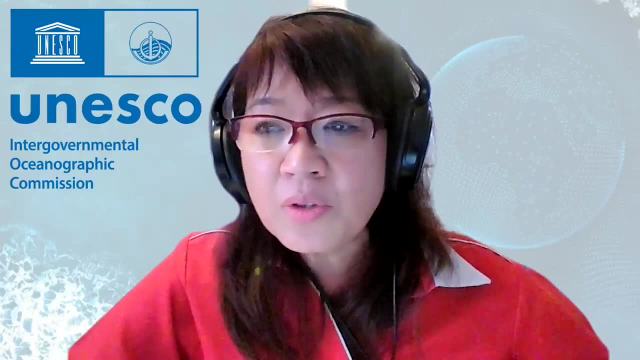 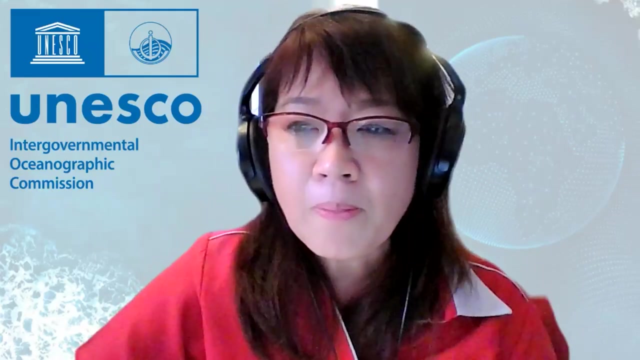 could you explain a bit on the chemical components of the modified clay? Is it just clay or is it mixed with other chemical compounds so it fluctuates easier or can kill or stop phytoplankton growth? Isaac, please, Yeah, I'm in that concern. 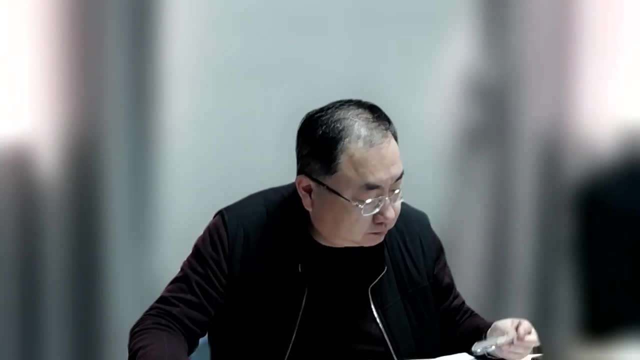 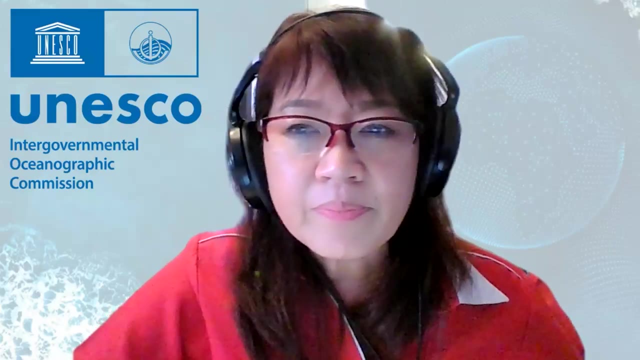 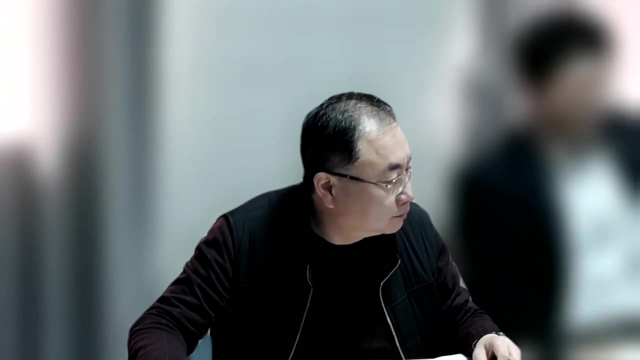 The components of the modified clay is just a natural clay. Isaac, we could not hear you clearly. Can you go nearer to the mic? Yeah, I'm coming, So is it much better? Yes, much better, Thank you. Okay, so the main components of the modified clay. 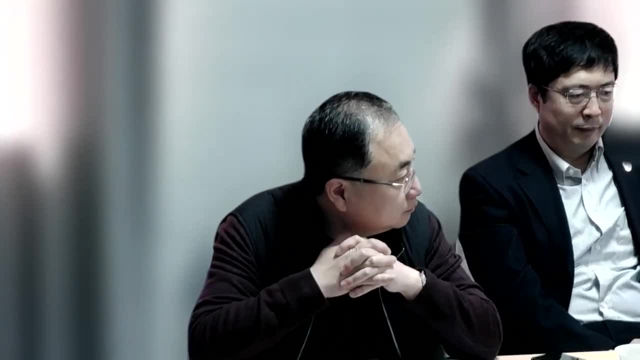 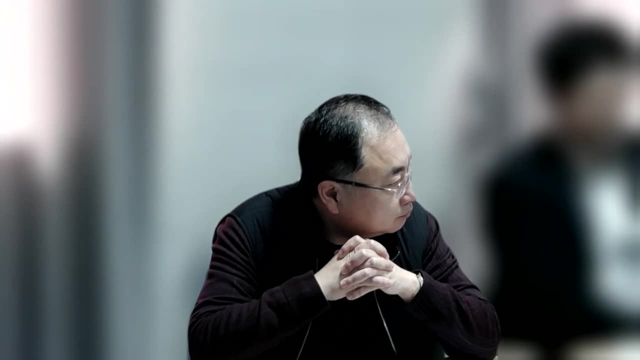 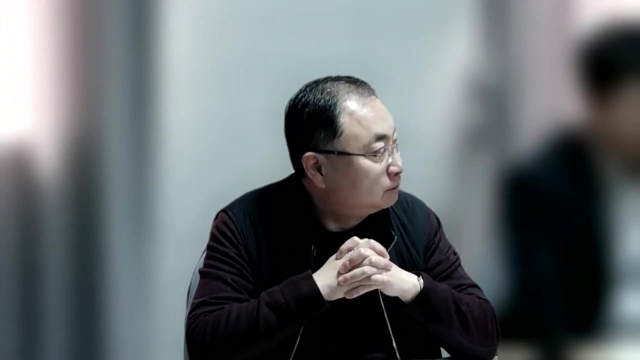 it's a natural clay, so it is very green and environmentally friendly technologies And we just modified the surface to improve the removal efficiency of the clay and to the cells. And for your concern about the basic organisms. initially, the dosage we used in open water is extremely low. 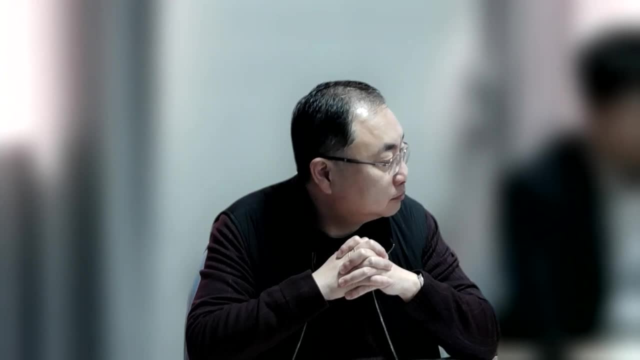 which is only four grams per meter, a square meter. So it is equal to We just spray a sugar bag of coffee onto the surface of one square meter. So it is very, extremely low. So the turbidity: we didn't see the turbidity changes in open waters. 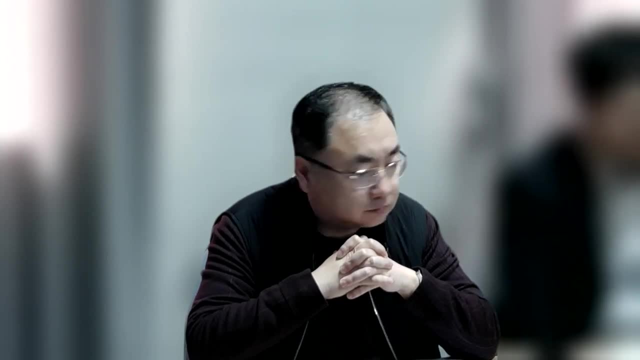 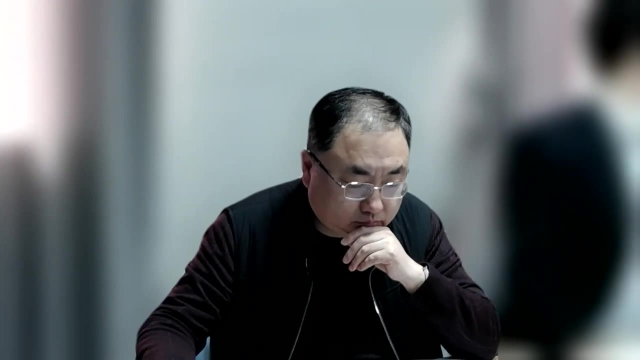 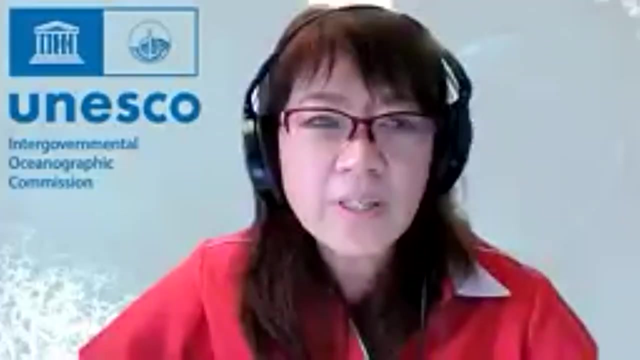 because of the water exchange, But for a careful reason. it also has a potential impact on the modified clay. Yung Wei, can you please off your mic, Sorry, sorry, Yung Wei, can you unmute yourself? Okay, back to you, Isaac, Sorry. 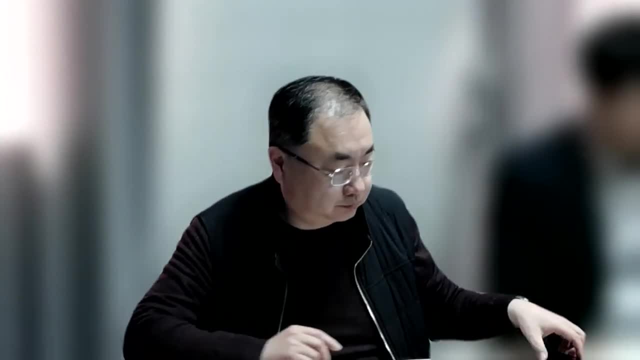 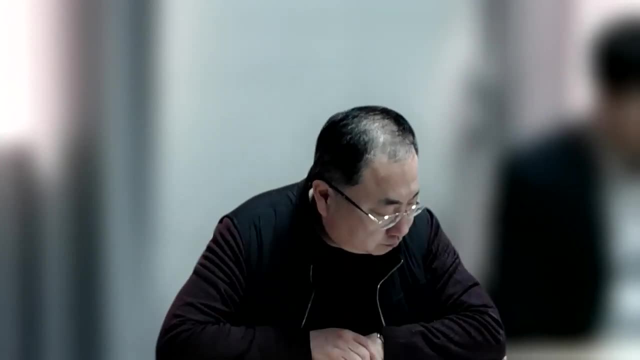 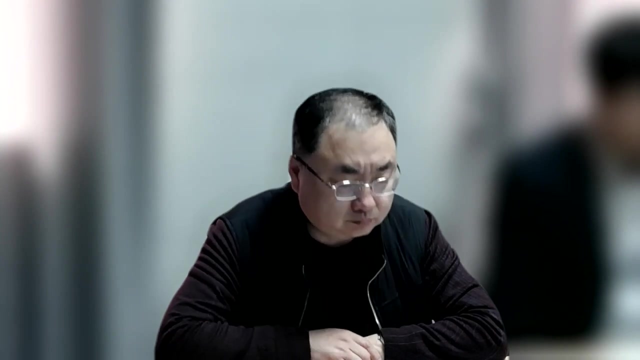 Yeah, no problem. Yeah, so let's back home And to the basic organisms. we also test the potential impacts of this method to the basic. The simple answer is no. There is no obvious changes of the contribution of the control group and the MC addition group. 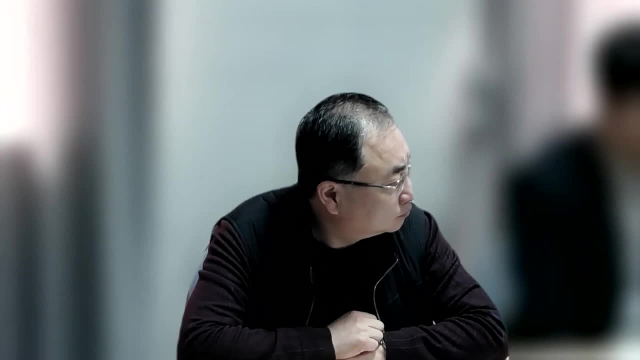 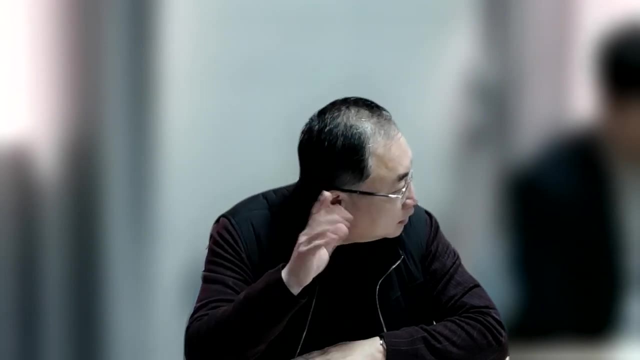 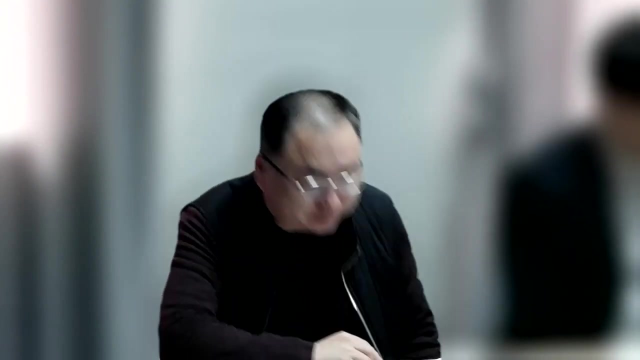 So, all in all, it is very green and environmental friendly approach to mitigate or to treat HABs in field, And is it cheap comparing to other tools. Well, yeah, thank you, Professor Wang. yeah, You know, this method has been widely used. 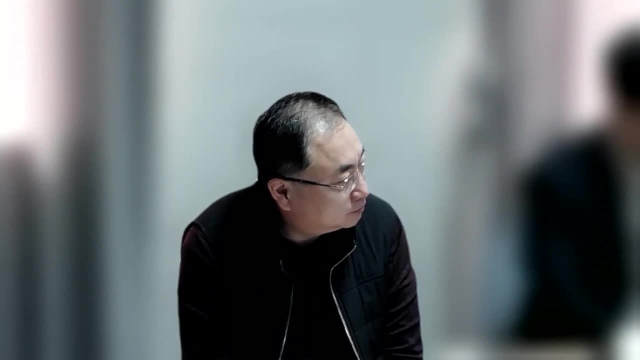 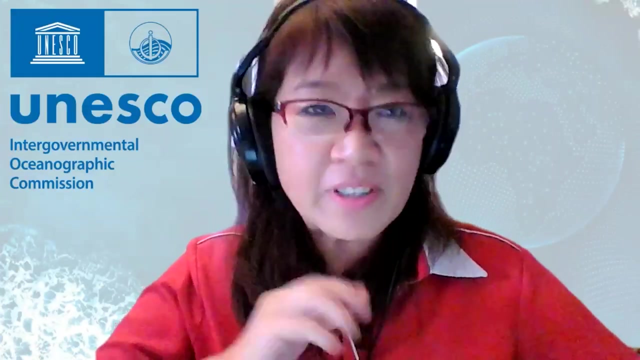 along China coast. We treat, we control HABs in thousand square kilometers or thousand square kilometers, So the cost could be accepted? I think yeah. Thank you My own curiosity: This modified clay is designed to actually capture the HAB. 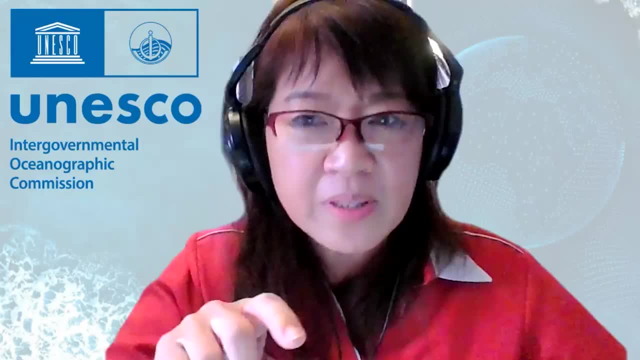 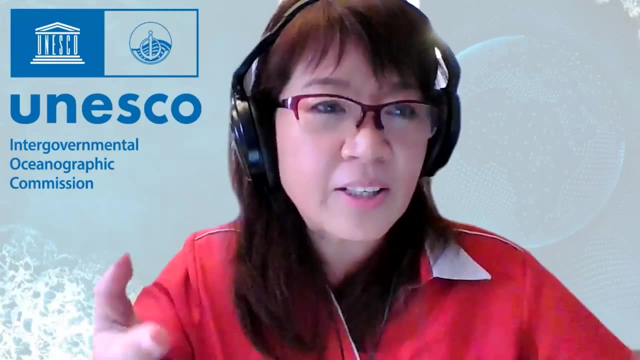 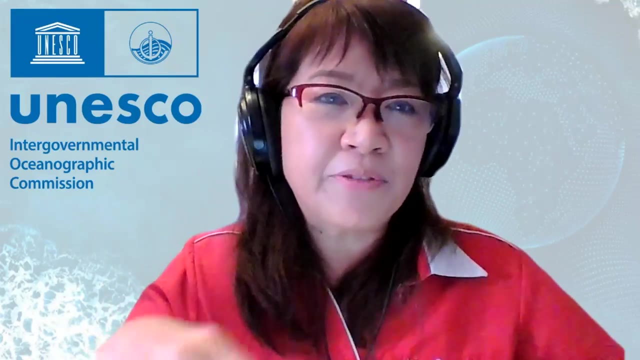 My question is: what if the HAB happens in a mollusk farm and the mollusk is filter-feeded and they need the algae to feed? Does the clay also absorb other plankton also in the area? if you were to put in the clay in a mollusk culture farm? 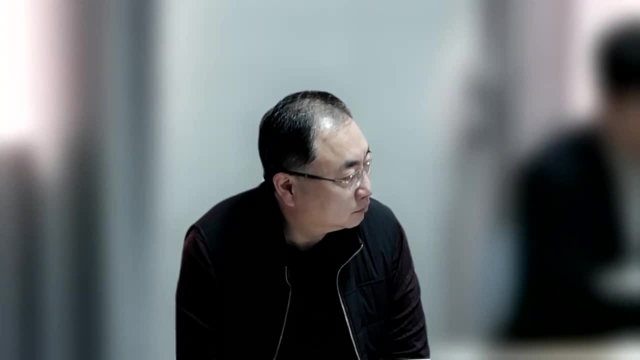 Initially and it's a mechanism. this method controlling HABs is the flocculation between the clay particles and the HAB cells, So it could flocculate This is the HAB cells and settle down them to the bottoms. Yes, and to your own concern. 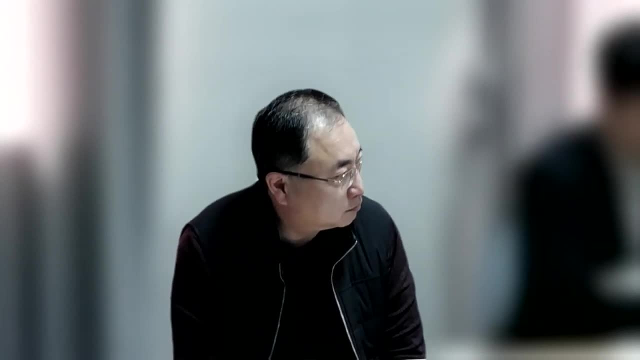 and I wish to share a story we used in a shrimp culture ponds. We spray this material onto the surface of a shrimp culture ponds and the shrimps may potentially- you know- to eat this clay particles or all the flocculants. 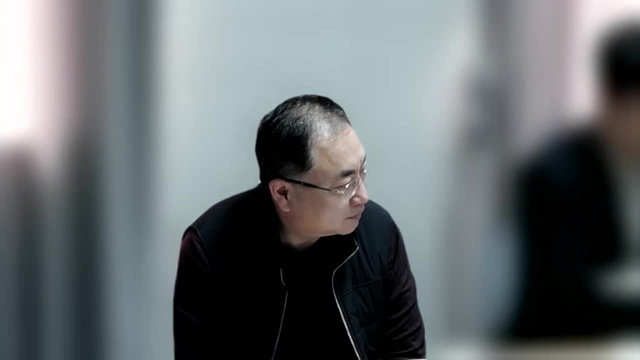 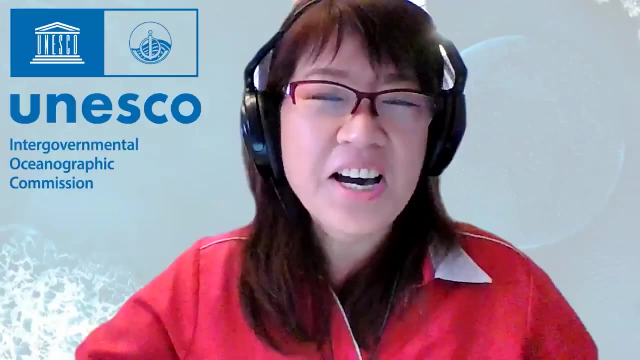 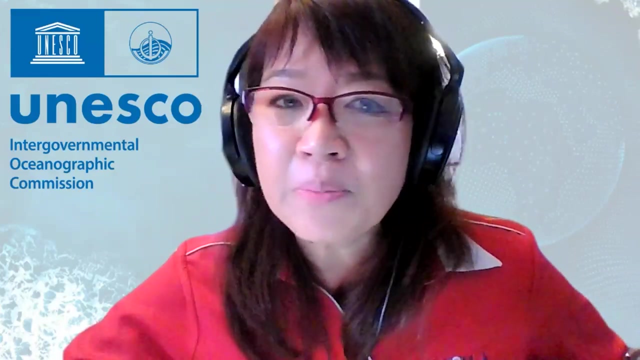 And do you know the results? Do you know the results? Do you know the results? And the shrimps grow much bigger and the taste is much better than before. Then you know, does it actually in a way eating also the HAB also right? 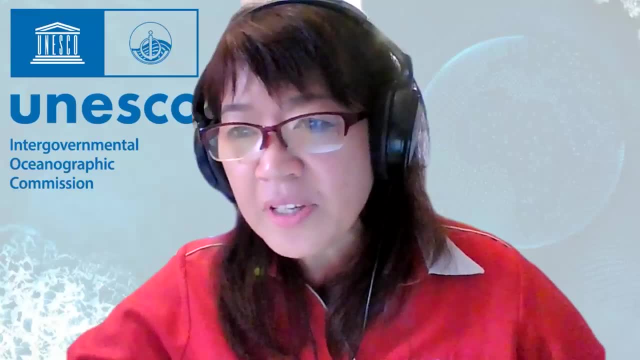 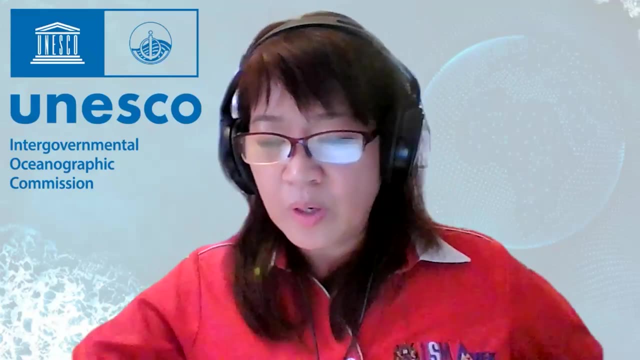 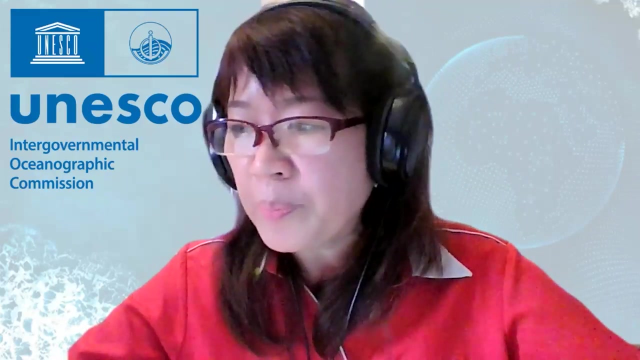 Yep, Okay, I have. you know, I don't see any burning questions in the chat. I have one question for Professor Wang, or Ren Zheng. I have one question for you to address. you know, with this, triple I, I, triple, triple P-C-C. 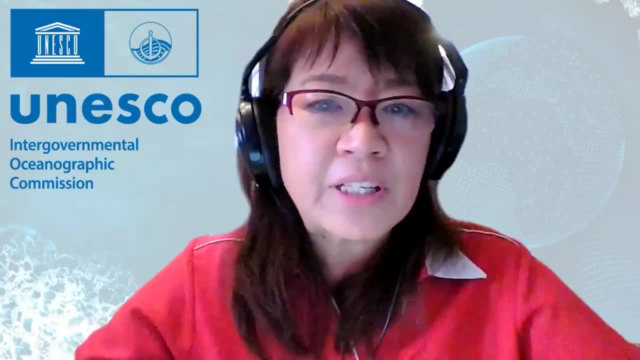 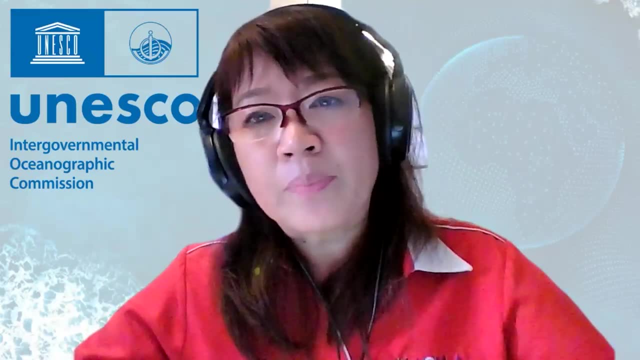 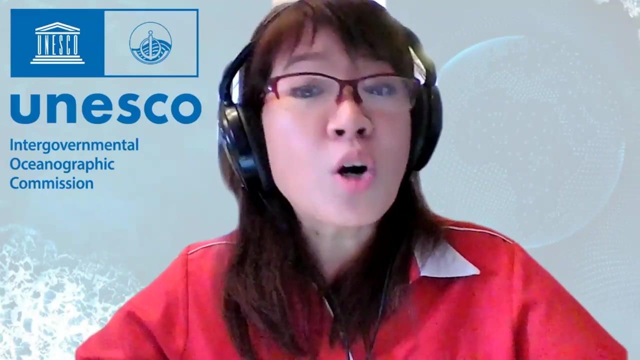 we are just initiating A lot of- I see a lot of interested participants and audience here that we can actually invite them to join. The burning question that they have is fundings. You know, fundings if there's, there is opportunity. 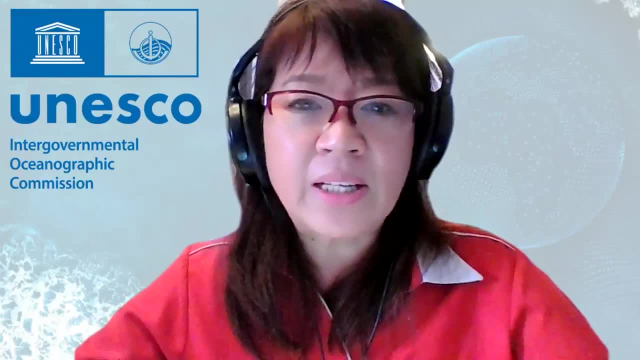 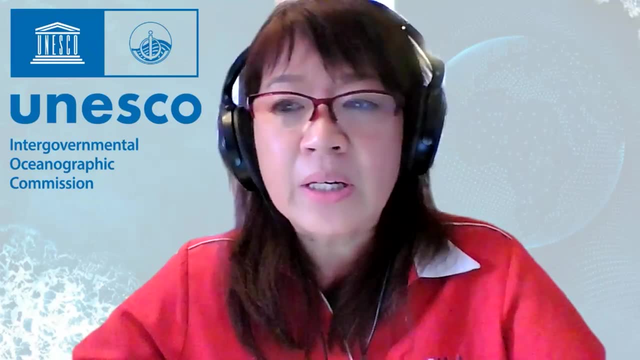 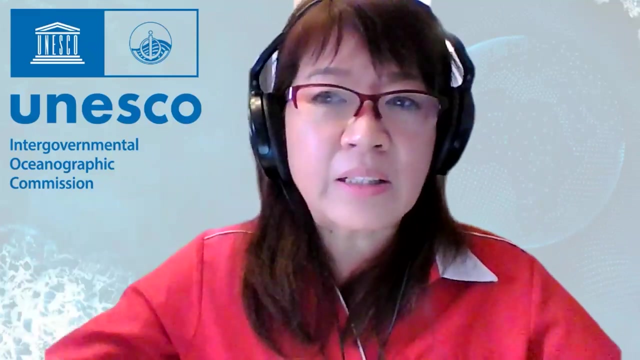 for training, for joining the Experts in Pearson excursion and training and workshops, you know, and also learning how to do the research together. But most of us would like to know what is your directions in terms of sustaining this program, in terms of funding. 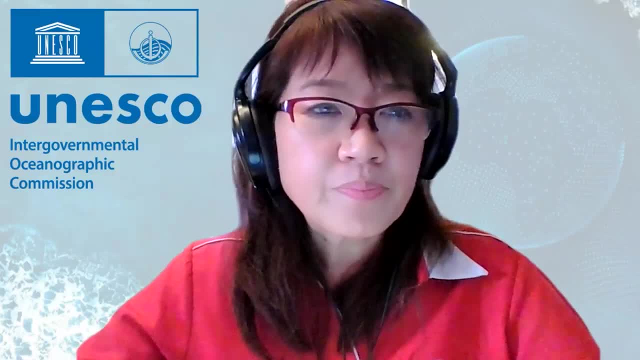 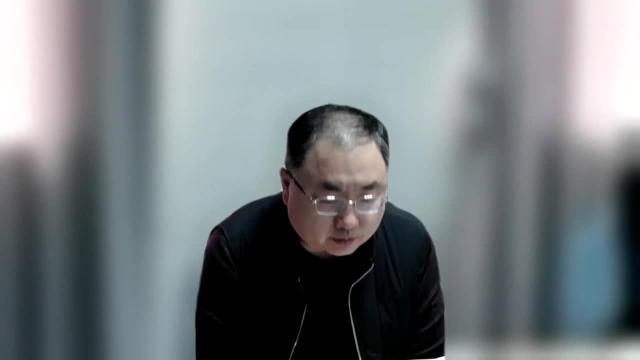 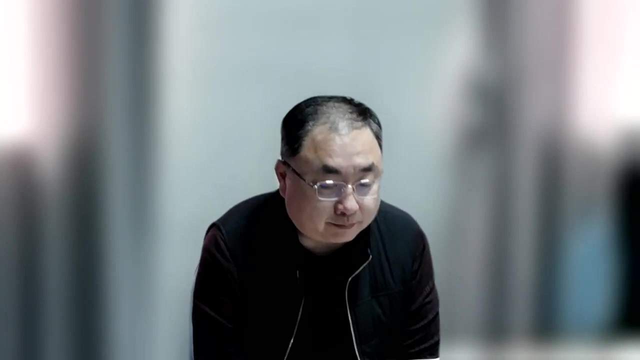 Yeah, over to you, Prof Lam. Thank you, Eileen. I think the international program can play a role as an umbrella or platform where we can apply the funding from our own national funding agency for the members' activity, And meanwhile IUCAS have already get some initial fund. 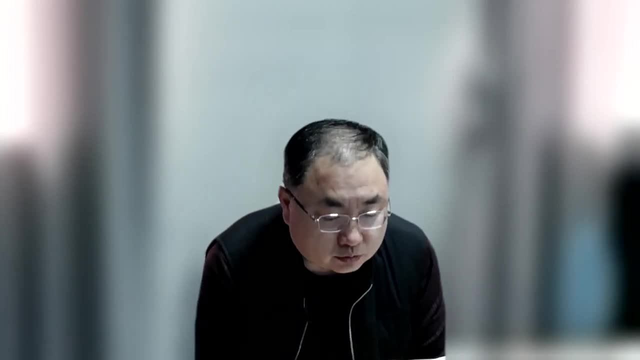 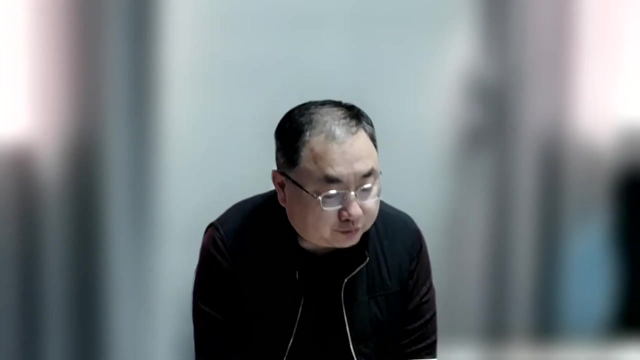 which can be used to organize some seminar and the training course and the young scientist exchange in a couple of years And based on this and I think we can design a very good implementation plan including the field experiment and the internal experiment. So, yes, the membership. who has the member institution? 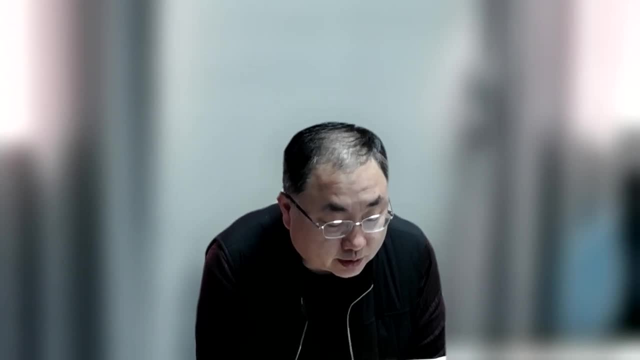 who has a research vessel. okay, we can organize some joint crews, but with their own funding and for the partner institutions without research vessel. or we can invite the scientists on board or research vessel, or not even on board, or no. 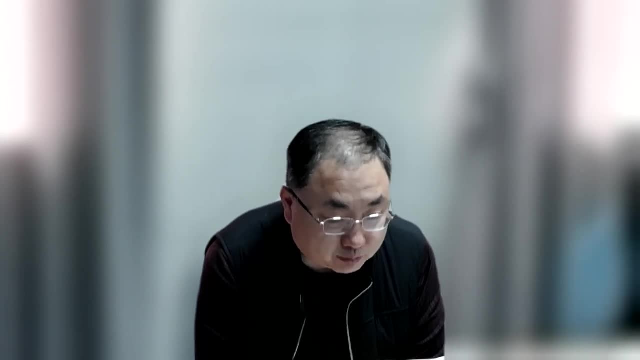 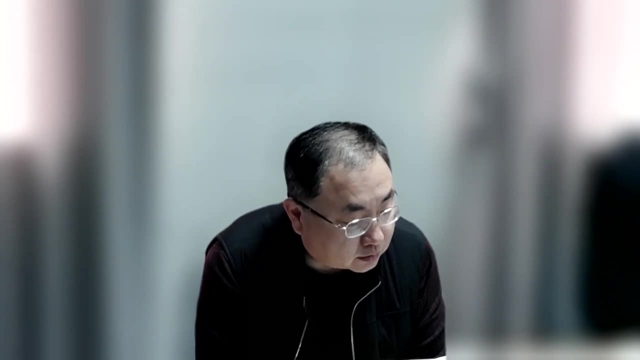 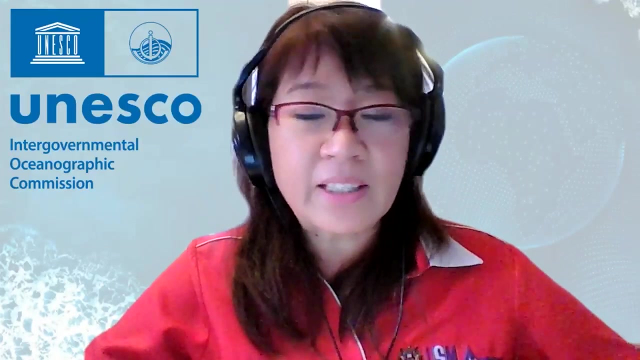 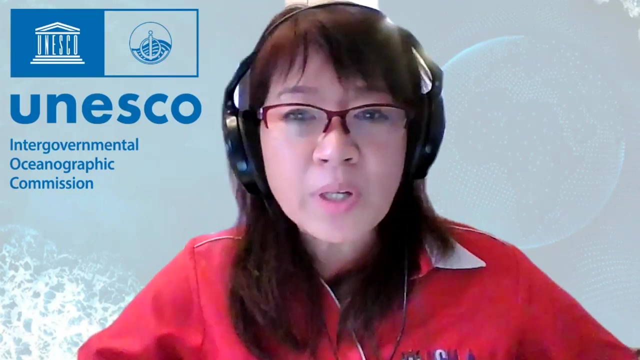 we can share all data and the samples And do some joint research and jointly submit and publish our papers. I think that's wonderful. thank you for enlightening us with some positive notes on how we can move this program. I would like to suggest to Ren Zheng Yu: 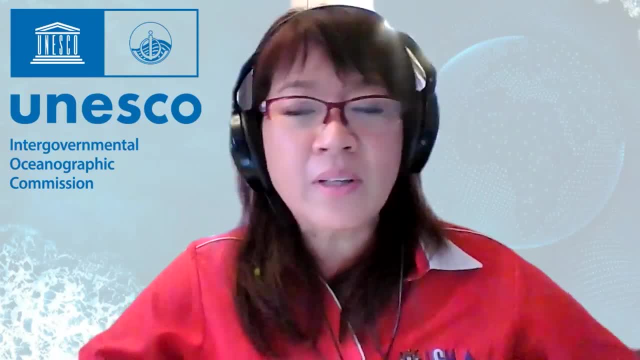 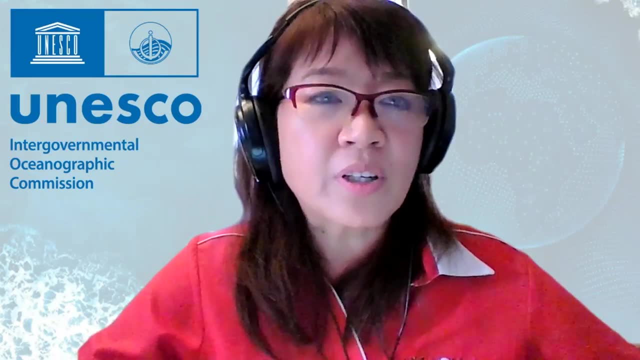 can you please kindly put the secretary email onto the chat box? So I'm sure there will be more interest. so I'm sure there will be more interest, so I'm sure there will be more interest parties that is going to contact. 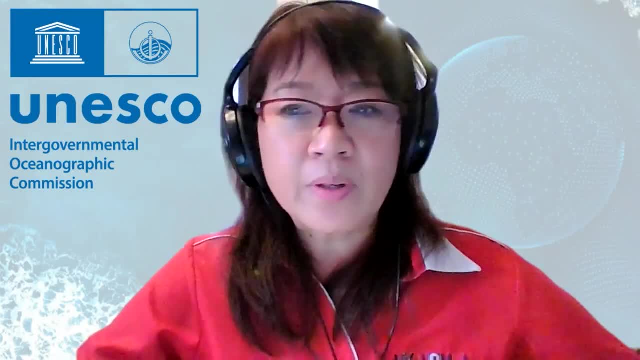 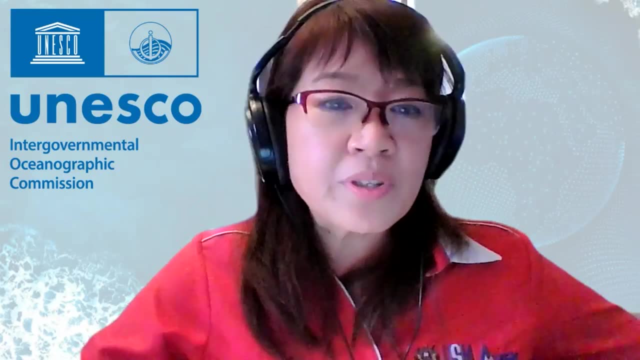 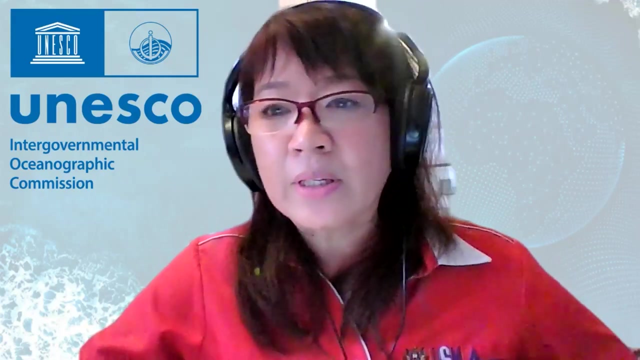 contact the main secretary of this program? Okay, Ren Zheng Yu or Lin. can you please type your whoever contact number so those who is interested to join or to participate in this program can actually email to our team. All right, For those who are interested, please look at the chat box. 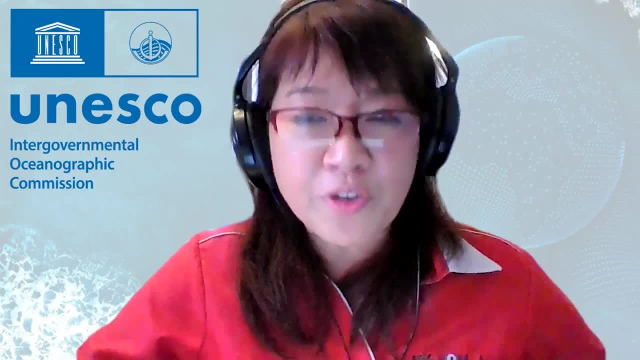 for the email address that you can write to to show your interest, for the email address that you can write to to show your interest, your interest. so i think time is not on our side. i will pass it back to professor fang wang for for. 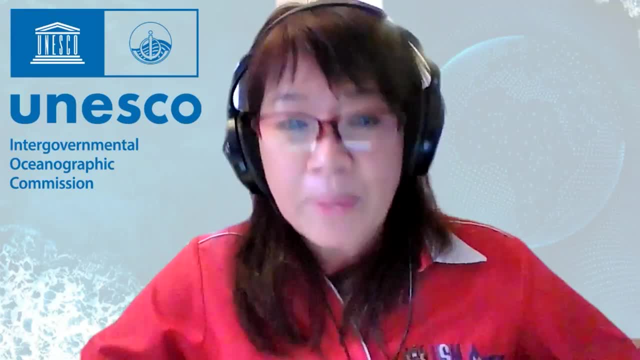 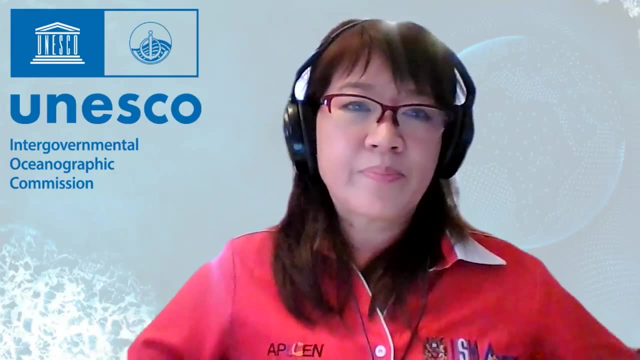 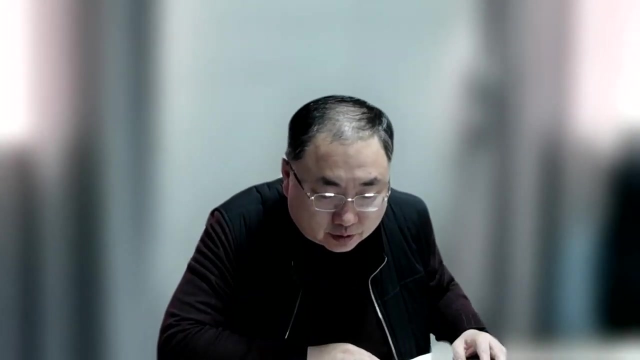 your closing remarks. thank you very much everyone uh for participating and and and uh be part of the program. thank you very much. back to you, profan one. thank you and uh. yeah, maybe, maybe. thank you and uh. i i just uh reading the uh the message at the chat room to me uh, but maybe i can uh answer. 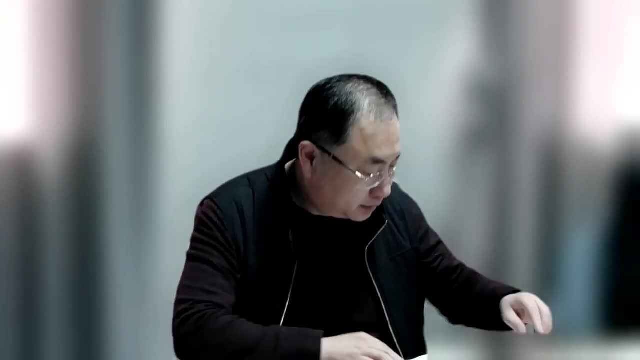 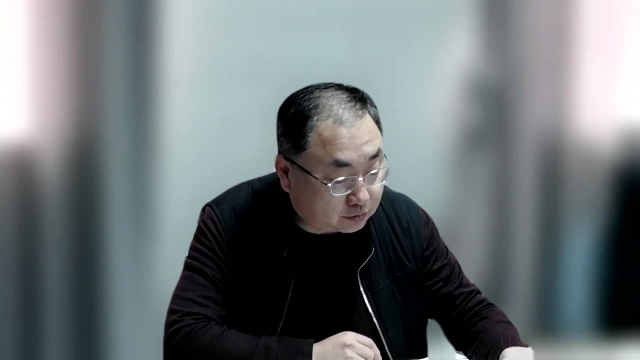 the question uh later. uh, okay, the dear friends and the colleagues, uh, we are very close to the end of this meeting. i believe, uh the uh, our meeting is a great success. we have already uh listened to four invited talks from senior scientists and three mini talks from young. 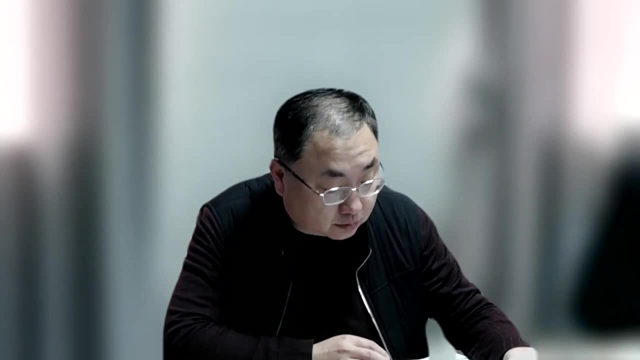 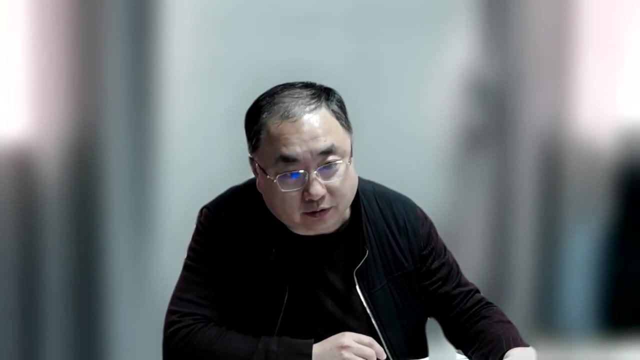 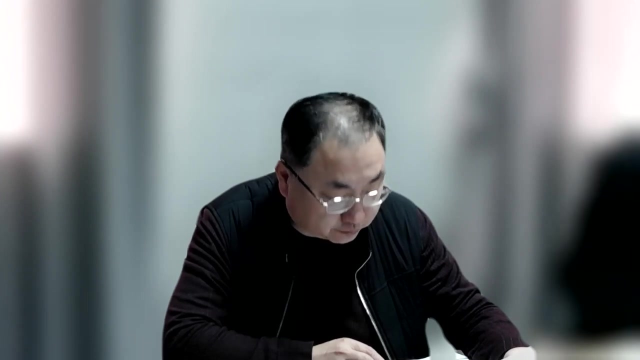 scientists and all presentation were very uh, informative and the discussion, uh even not time enough, but it's very uh, i think, is fruitful and constructive. on behalf of all members of our organizing committee, i want to thank professors zena and ellen for hosting the meeting and uh. 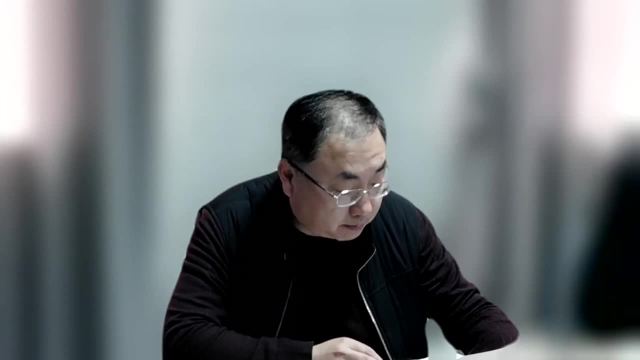 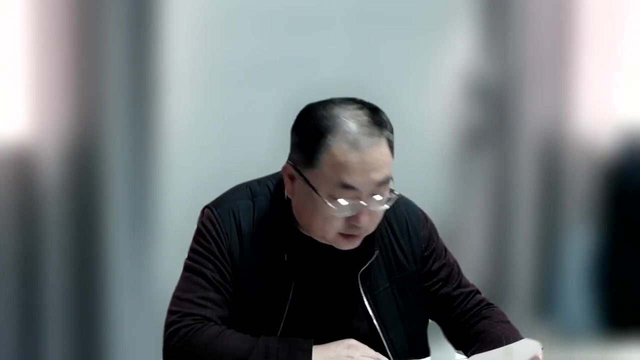 sincerely appreciate the all participants of the incubator aid today to engage in developing the knowledge of marine biodiversity in this area and funding finding the solutions based on our joint effort. and you can see from uh regional youth park there's many vacancies of uh of the our working group.